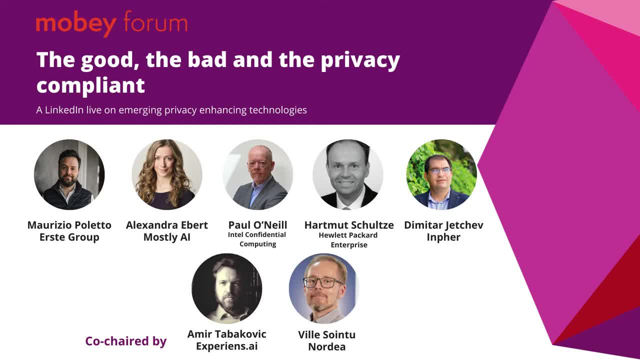 these privacy enhancing technologies and see what it actually means for them, And I also work with financial institutions like Nordea. whether they are a threat or an opportunity, I can certainly say that in case of this, it is definitely an opportunity to actually collaborate. 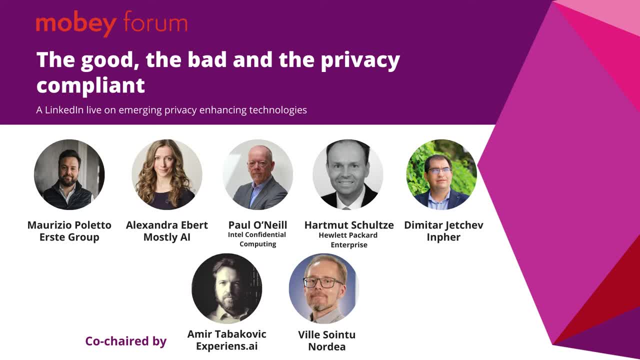 in a much more effective way. But, Amir, maybe a few words about the expert group itself. Yes, sure. So before let me just say introduce myself, because I forgot to do it in the beginning. So I'm Amir Tabakovich. I'm an independent advisor in the area of privacy, enhancing technologies and 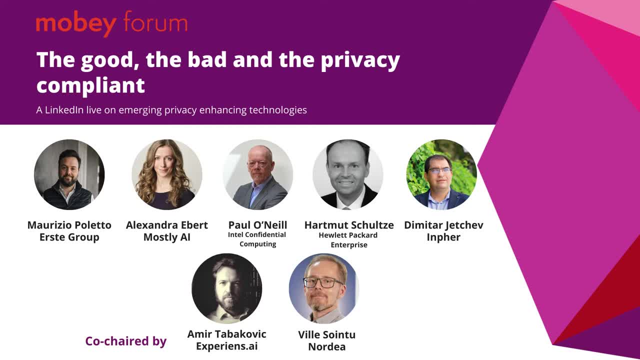 artificial intelligence, And I'm also an honorary member of MobiForum and the co-chair of this expert group. So we started this expert group some one and a half- two years ago, I think- by discovering that the privacy is one of the major challenges when it comes to introduction. 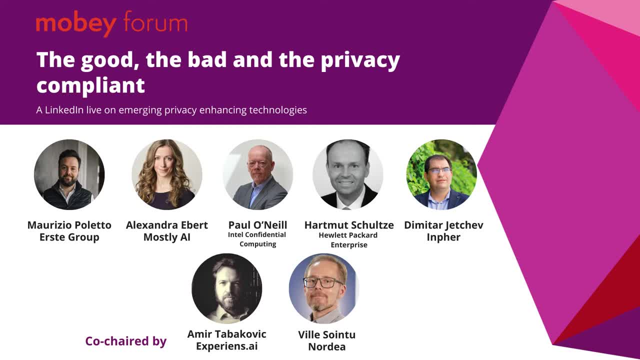 and deployment of predictive AI applications in banking. We started with the work, and in the minimum, a few years ago it was the first time to do so, So we started with the work, and in the minimum, the first time to do so. So we started with the work and in the minimum. a few years ago it was the first time to do so, So we started with the work and in the minimum. 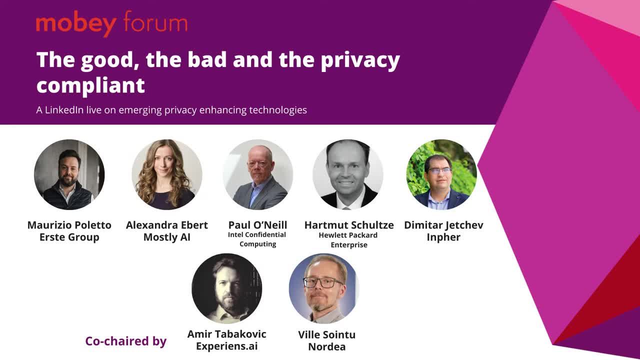 In the meantime, we have different members joining from different banks and solutions providers within the MoBay Forum family. This work resulted, for now, in the first report that we published in June of this year. Maybe you want to say something about our first report. 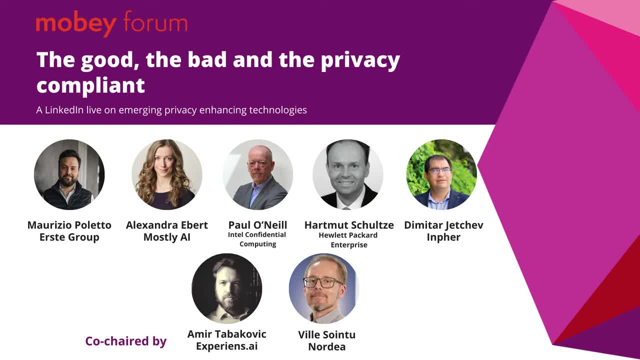 Yes, of course. So the first report that we again. it was a long time writing, but it turned out pretty well. It's kind of a good way to explain that we're really looking at a sweet spot between how to be compliant in terms of all the privacy regulation. that is especially important for. 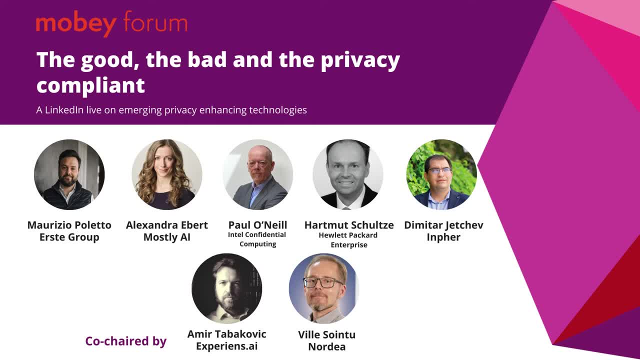 institutions like banks and yet to be able to leverage all the opportunities of data. Now we, especially in banks, we feel the pain that we perhaps are not able to be like Google or Facebook and use all the customer data in the same way as they are doing, for obvious, 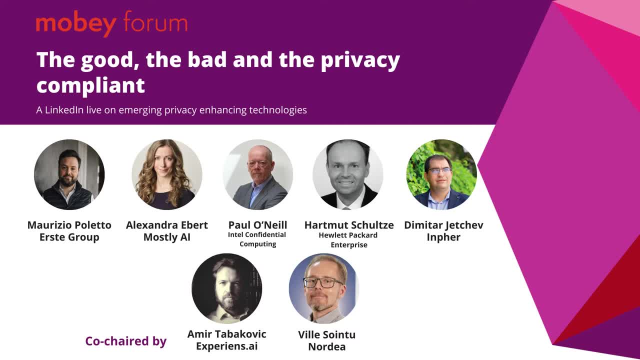 reasons. There's regulation, there's supervision, but, most importantly, there is the element of trust. If we cannot reach the trust elements that we have towards our customers- and this, of course, means that we also need to be trustworthy as custodians of important customer data points- 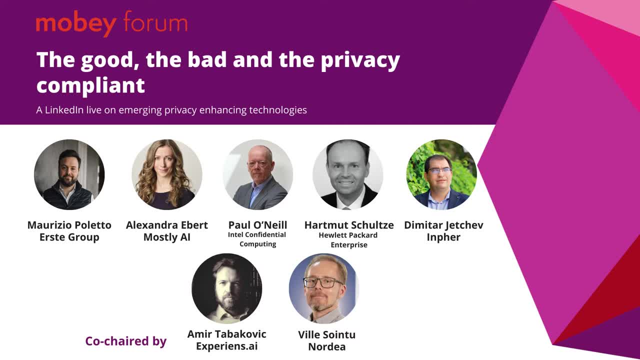 So, again, looking at these ways to make sure that we have the integrity of the data, the privacy of the data is maintained, by using these technologies. it is a great opportunity for us to move forward in a data driven innovation department Now, before we go into this kind of new format that we're experimenting here. this is actually 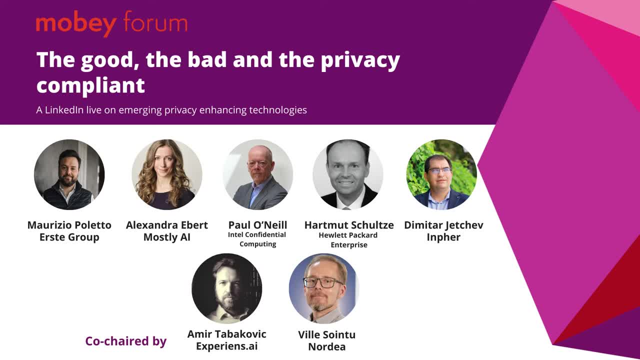 our second thing in life on this topic. we have some pretty hilarious technical problems in the last one. Let's see if we can manage through this one without any unintended nudes or weightings of hands like we did last time, but it was anyway a memorable moment for all of us. 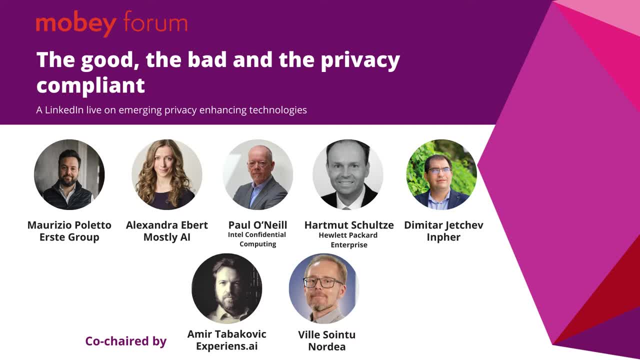 But before we go into that all of that, a few words about MobiForum or any of the other audience who might not know about MobiForum before. MobiForum is a global not-for-profit industry association working in connecting banks and financial institutions and vendors working in this space to create better digital financial. 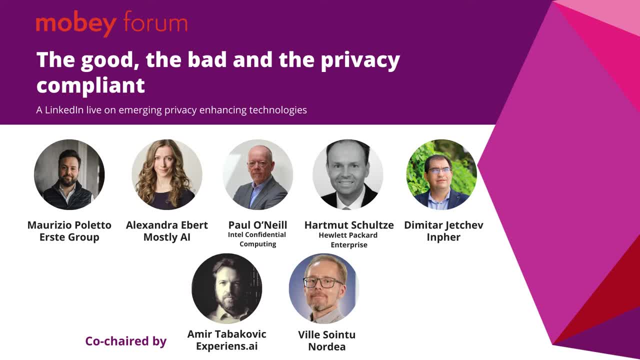 services for the society at large. And again, we have been together since 2000,. so it's one of the oldest industry associations, especially focused on digital financial services, and we intend to stick around for another 20 years, So looking forward to all of that. 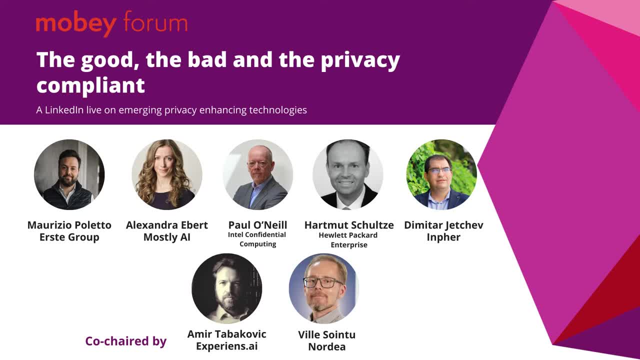 So good, Amir, about today. So what are we going to do now? Exactly Like, MobiForum, is basically very good in exploring uncharted areas in financial services and the whole digital space, And I think, with this new format that we are introducing today, with this open expert group, 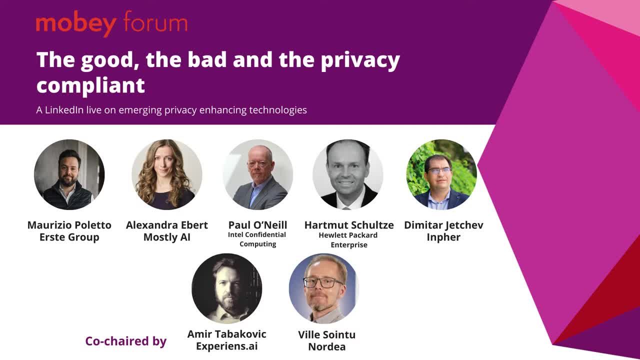 we are also exploring an uncharted area, not only when it comes to the format of our expert group, but also when it comes to the topic. I've been following what is basically happening in the privacy and hence in technology area for a while, and I have to admit that I never witnessed event with a combination of such 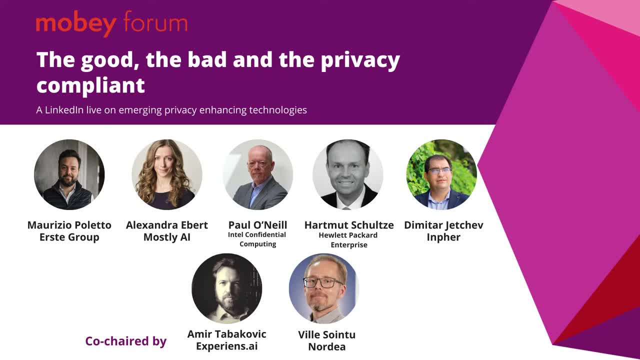 an interesting speaker, like we managed to get today, to share with us their vision when it comes to privacy, And so that's why I would just briefly want to come back to the agenda. We will have four minutes of time, So if you have time, please have your questions. 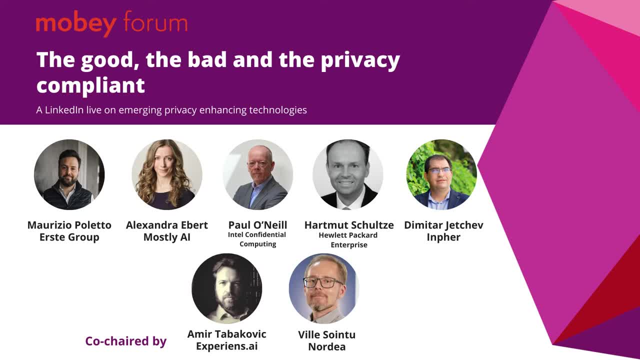 uh, four presentations of four, uh, excellent speakers, excellent experts in this area, followed by the panel. and after this panel, uh, we will have also um representative of a bank. we'll have an interview with maurizio poletto from the erst group, and then that should basically. 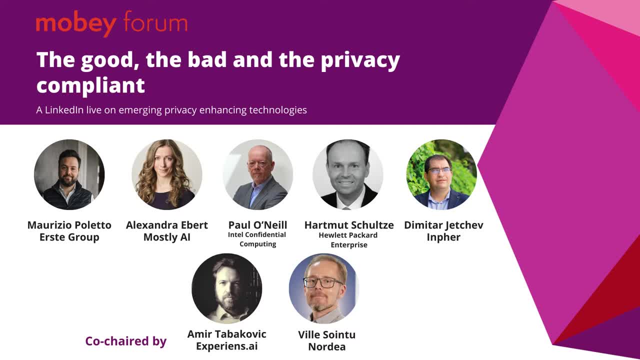 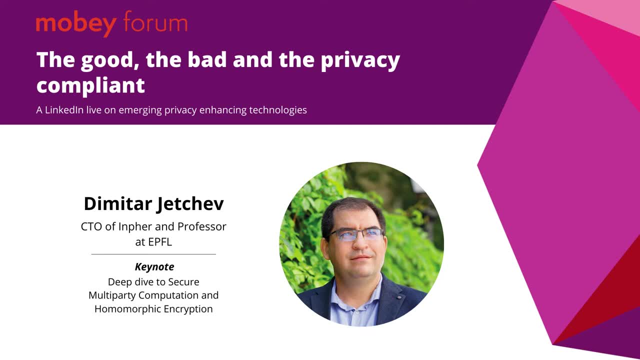 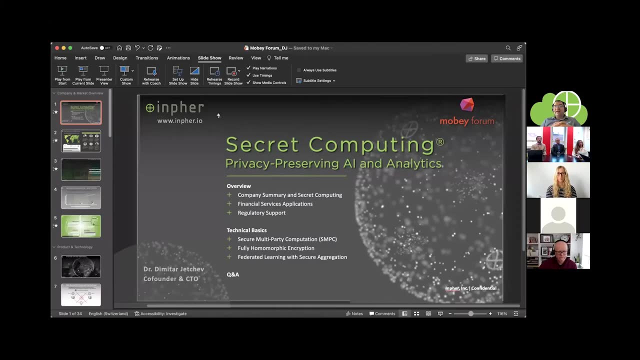 we then will be able to conclude this event in a little bit less than three hours, say that our common vision is that, indeed, these are all technologies that some people might think are competing, but actually they are not. so the optimal usage of this technology for me is really in a hybrid combination, as you will see, so hopefully that creates very interesting. 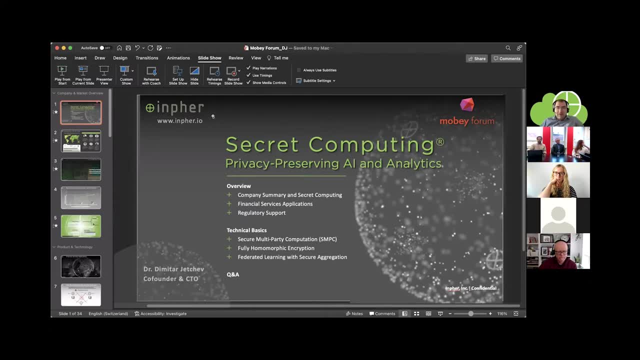 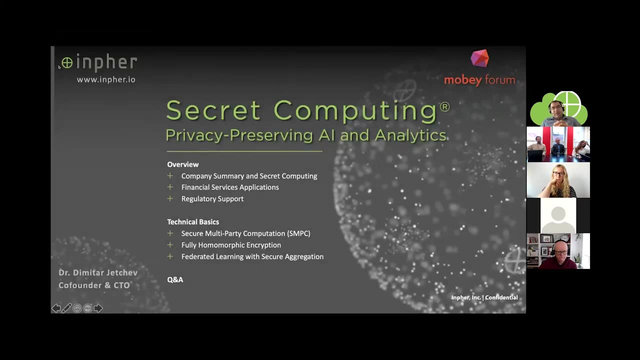 discussions with the other speakers who obviously develop and work on different complementary technologies. so today i'm going to talk about, i'm going to give you just very quick overview of infer and then i'll switch to the technical basics. but before i do that i'd like to talk about some 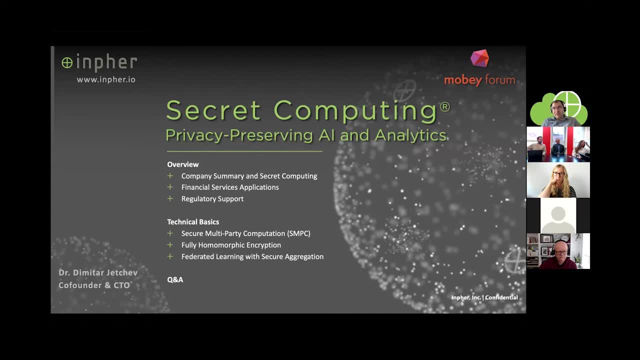 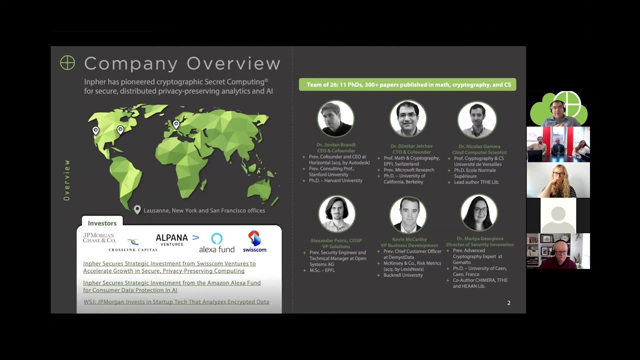 financials services, applications and regulatory support coming from these technologies. so infer was created in 2015- about six years ago- and includes multiple expertise in cryptography, machine learning systems, distributed computing, etc. so we have a large set of publications in the space. we're coming from: background in mathematics, cryptography, machine learning. 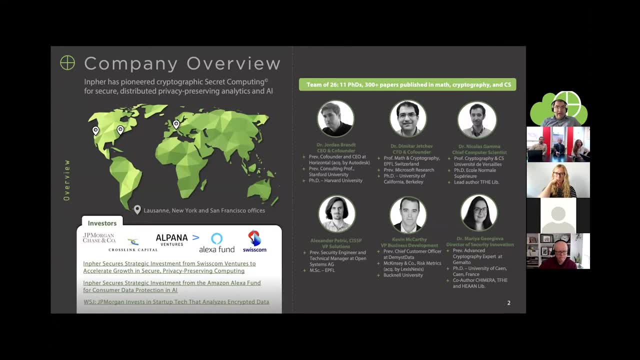 we are funded? we have been funded by various investors, including jake morgan chase, crosslink capital, alpana ventures, alexa fund, amazon. alexa funded most recently swisco. so some of these, as you see, are institutional, some of them are strategic investors, so the company is based in. 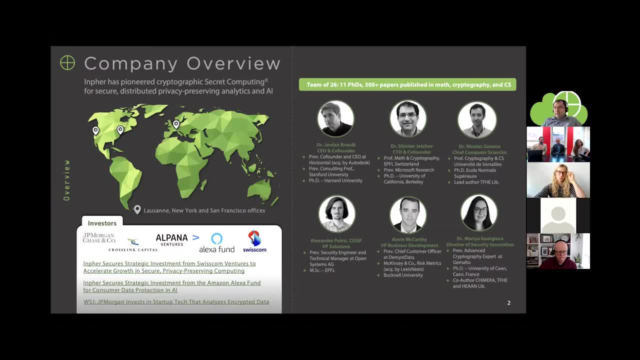 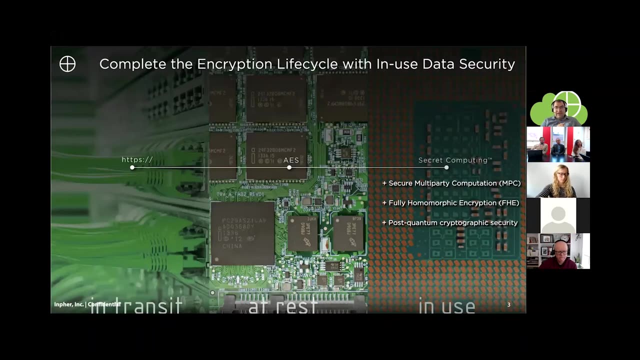 both- i forgot to say- in us and in switzerland. technical team is in switzerland, business solutions team is in the us. so, uh, to begin with, the problem that we are addressing is, uh, as we call it, the three pillars of uh, uh, of data security. so, on one side, you, uh, you have. 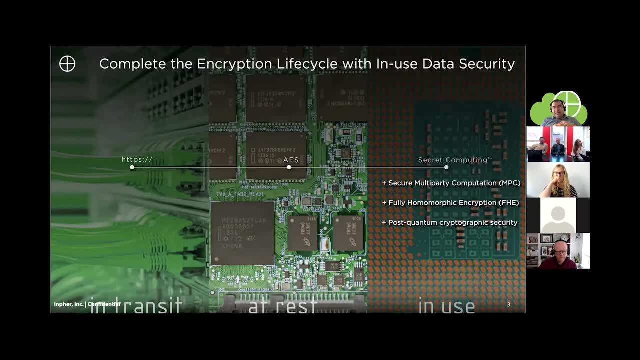 securing data in transit, uh, on the other side, you have securing data at rest, and most interesting is securing data in use. so, when your data is secured, the question is, how can you actually do you's and useful computations on this data? and here, uh comes the two major cryptographic technologies. 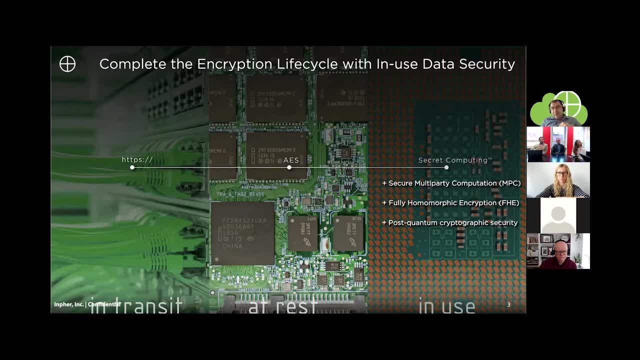 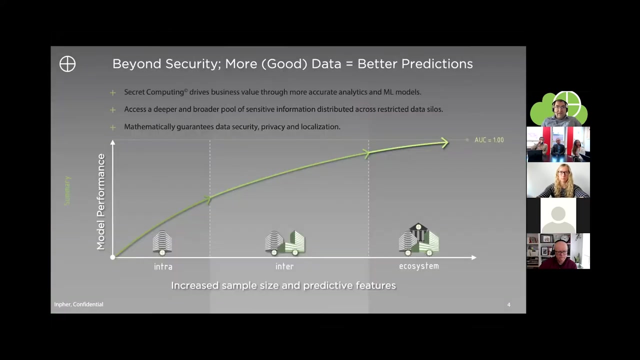 uh, so secure multi-party computation and fully homomorphic encryption that presumably enter the long-term vision of providing this post-quantum cryptographic security as well. of course, these technologies are complemented with multiple other technologies, as i will mention in my in my talk. so, uh what? the major idea here is that you use this type of computing with essentially enriching your 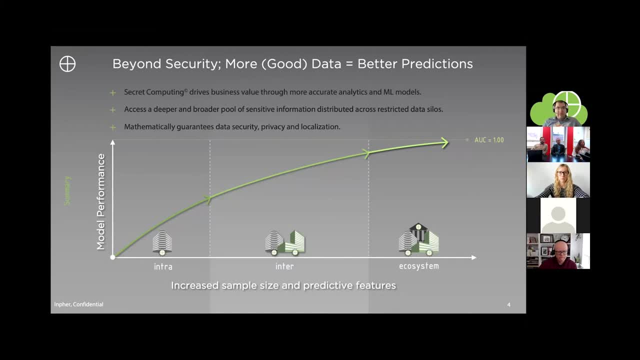 data. so if you're an organization, a bank or a financial institution, you may have limited data to just train or build or compute your model. so if you compute model with only your own data, the performance of this model may not be very satisfactory. so what you could think about is: can i enrich my data using other data sources? 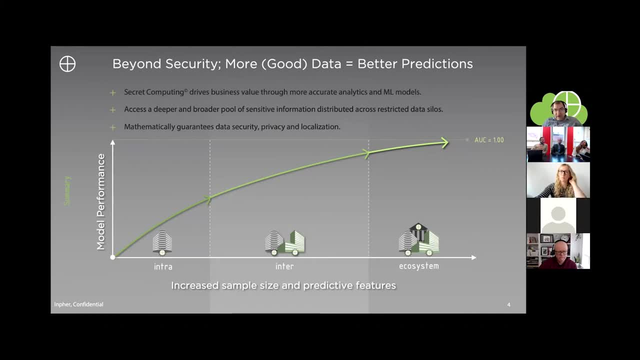 that i a priori don't have access to due to privacy constraints. the simplest possible scenario is when you operate in multiple jurisdictions and you use private data for, say, your customers, and in that case you can't really aggregate that data in one place. so that's. 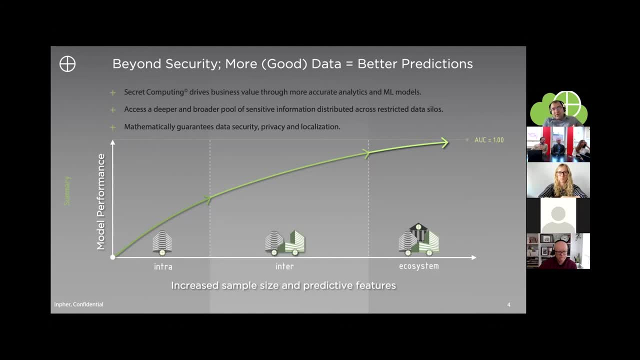 a very significant constraint, uh, you can. you can talk about collaboration between different institutions, uh, in the ecosystem as well, in which case, potentially, you bring extra data that give you extra features in your model. so the question is that, instead of bringing all this data in one central place, which is impossible or constrained, uh, due to privacy regulations- 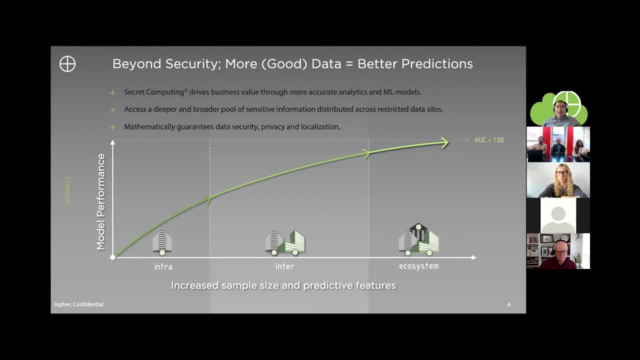 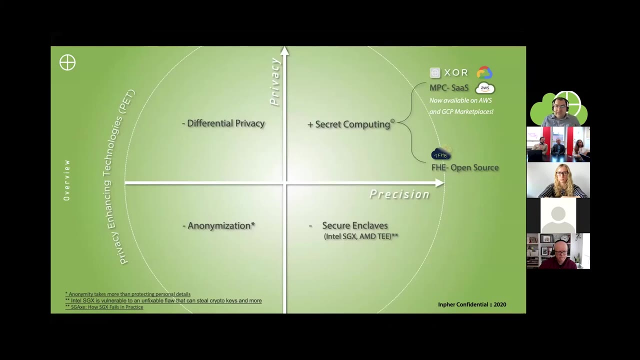 what you want to do is you want to compute uh without actually bringing uh the data outside these institutions. so you you do a distributed compute, but with strong mathematical security guarantees. so there are different approaches here and they sort of, as i mentioned, they complement each other. so some people might think that they compete. i don't want to think that way. so in the 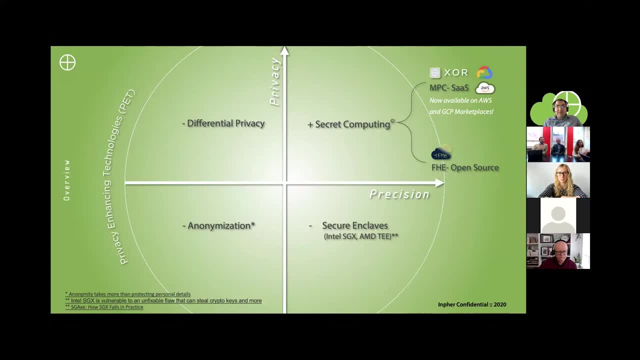 first, uh, in the lower left quadrant, you have an anonymization, and we know that anonymization uh is sufficient because, on its own, because, um you, you risk a free identification. so, on the lower right corner, you have secure enclaves, and we're going to talk about this more at this forum today. so 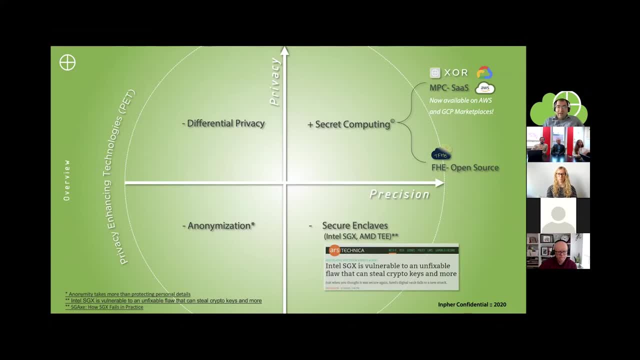 uh, secure enclaves, including trusted execution environment, uh, uh, so intel, uh, hgx, amd, trusted execution environment, etc. so i will show you how this can be useful. so, in a in a sense, that hardware can complement- uh, what? what we are going to talk about today, which is secret computing. so 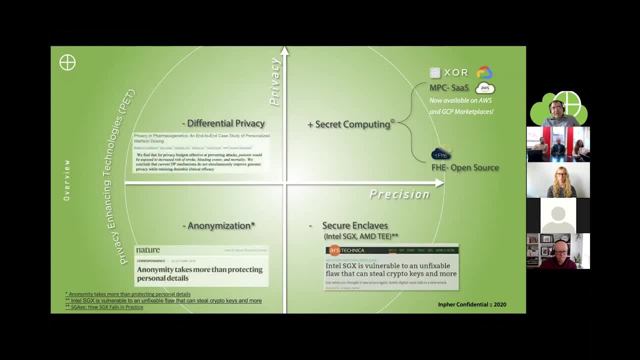 differential privacy on the other hand is introducing noise in the data, and by doing that you lose precision in the computations. but you could preserve the privacy of your original data, and in fact here you have to be very careful of how much computation you can use on the data. 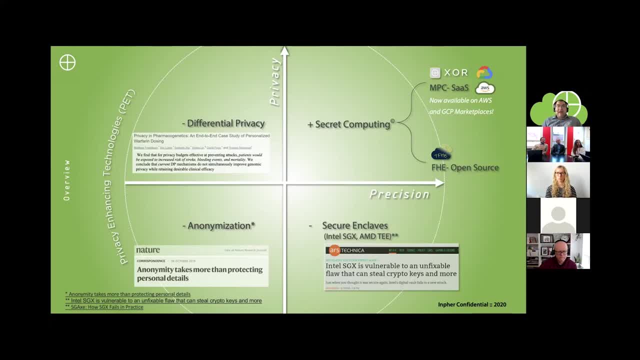 so usually this is another technique that uh complements the other ones and uh, the one that i want to talk about today is secret computing. so secret computing relies on mathematical, mathematically proven uh security, proven security proofs and uh. so the two major uh techniques that 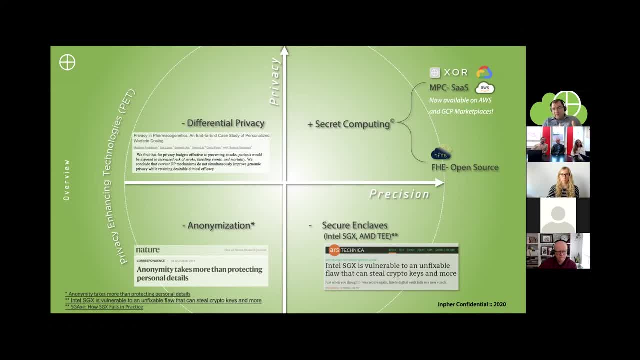 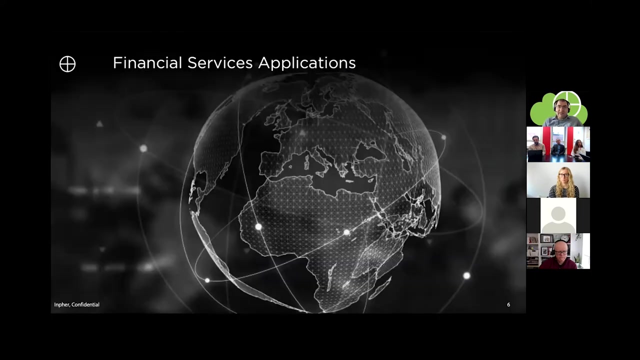 we will discuss are secure multi-party computation, fully homomorphic encryption. so infer as a company commercial product called xor secret computing platform that is based primarily on npc and it provides a open source library called tfhe for fully homomorphic encryption. so let's look at the 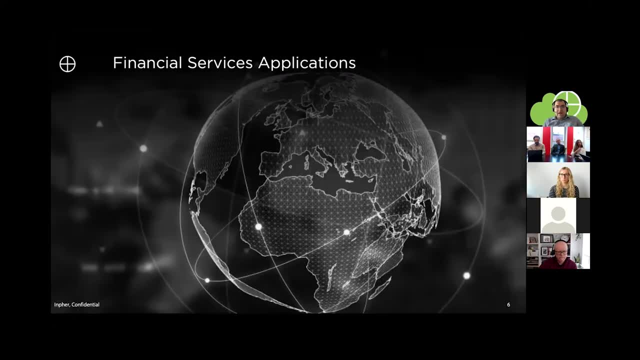 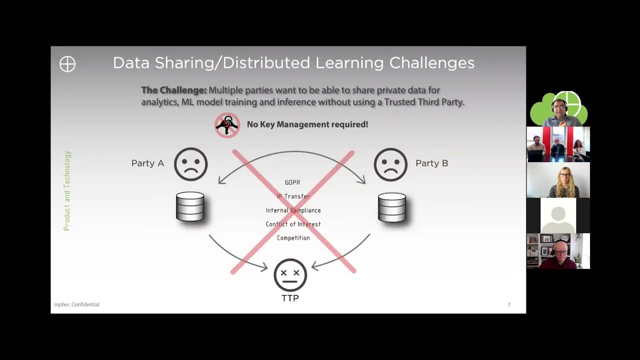 applications now, uh, so the first of uh the uh, the first and most uh common use case that we already saw was, uh, the situations or the scenario when multiple parties want to be able to share private data for analytics- uh say, machine learning, model training or inference- without interested. third, 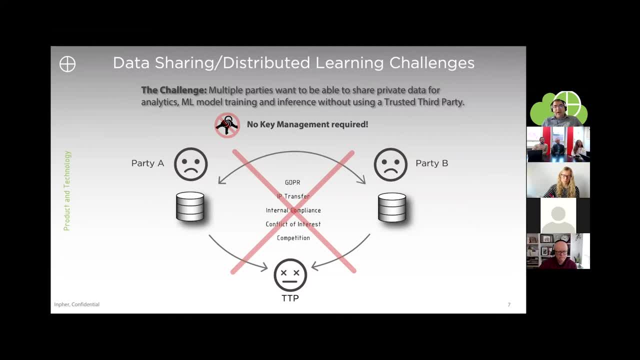 party. so, uh, if you have private data for party a and party b, you can't really bring it to a server- central central server. so in that sense, uh, like gdpr essentially prevents you from doing that. how solve this problem with secret computing? so here is the typical platform and tile. describe it in. 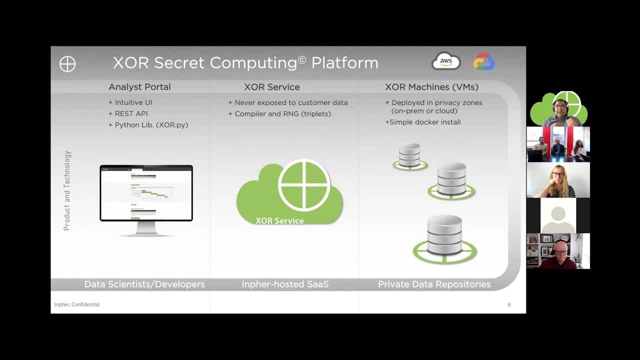 detail. on the left, you are seeing the analyst portal. this is how a data analyst interacts with the platform. so, with this analyst portal, what you have is you have an intuitive ui, you have a python module that you could integrate in your python data science code, and then you have also 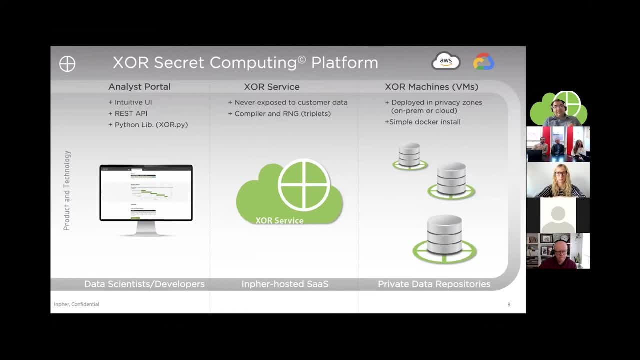 another rest, api. the idea is that data scientists need not understand the internals of cryptography, yet they need to trust that what they use is secure. in the middle, uh, infer hosts an exor service. so this service sees no data, and so it only runs a compiler that compiles the program. 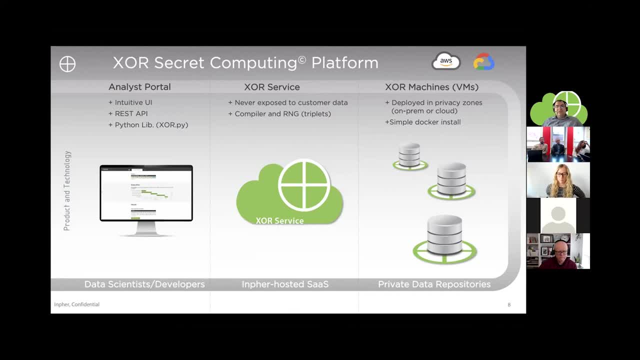 provided by the data analyst and also it runs a random number generator. on the right you have the so-called exor machines. so these exor machines are running on the different data sources. uh, so they are deployed in a in a different, in different privacy zones. they can be deployed very easily, obviously. this is the entire. 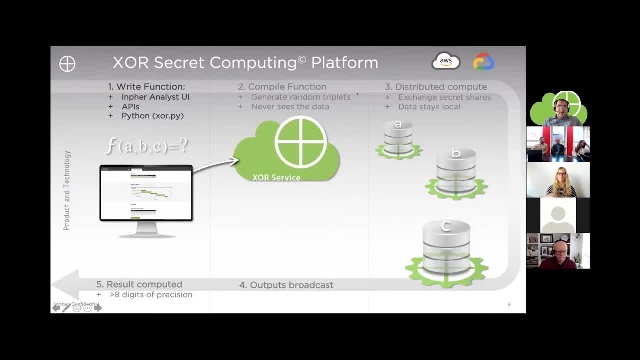 setting of the of the platform. so now what happens is the data analyst writes a function. function gets compiled and distributed across the data sources. the data sources are computing. so this is the actual secret computer: multi-party computation and secret shares, for the results are returned back to the data analyst to reconstruct the result without seeing anything. 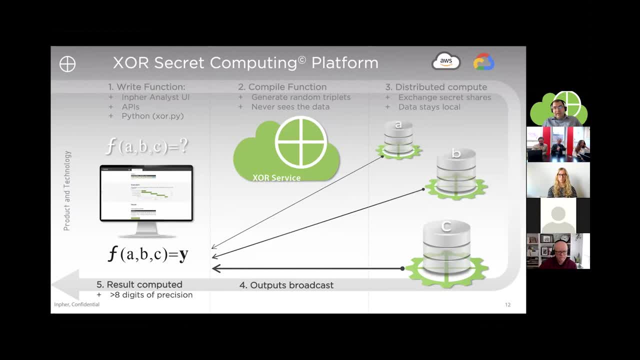 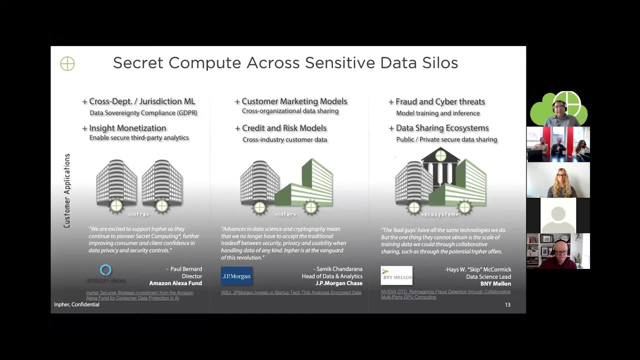 more, but the result about the original data at data sources a, b and c. so uh again. uh, examples of the secret compute across sensitive data silos, cross departmental or jurisdictional jurisdiction. machine learning- uh, insight monetizations, so enabling secure third-party analytics. here you're seeing some of these cases. customer marketing models, where you build models. 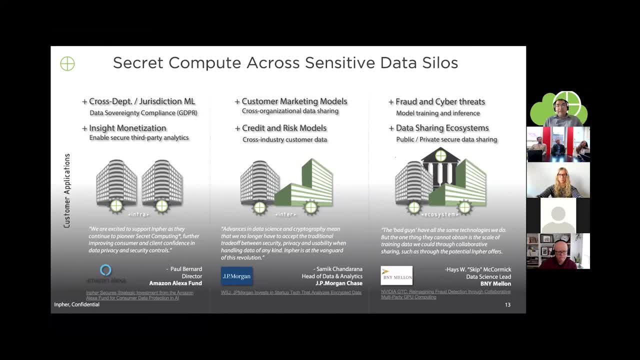 across cross-organizationally, and this is typically used in a production scenario. we use this in credit and risk models and then, on the right, what you see is fraud and cyber threats. so this is important when you want to do fraud detection or, even more generally, anti-money. 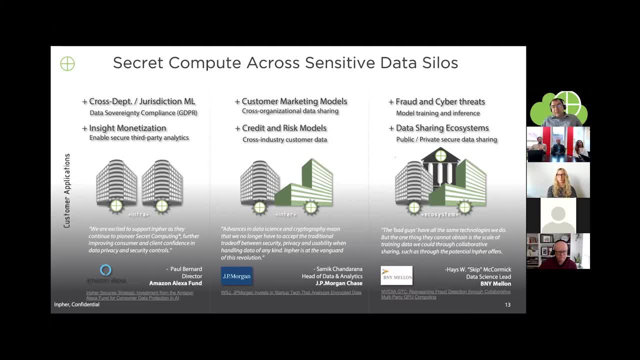 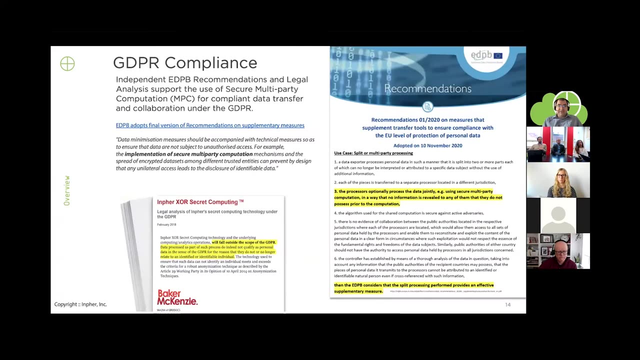 laundering detection when you want to include multiple financial institutions. the use case that you will see is a public one that we did with bank of new york melon, and it is about detecting fraudulent transactions. so, before i move to the use case, just to tell you a word about 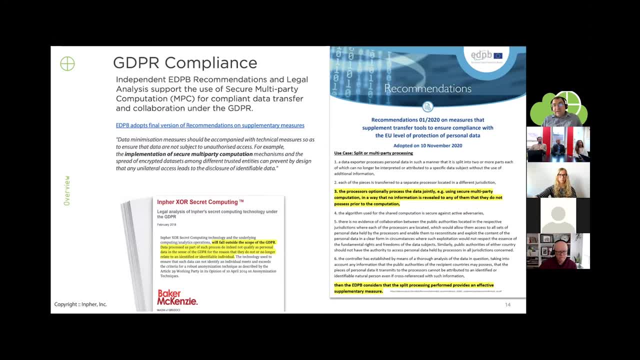 gdpr compliance and regulations so recently. on the right you're seeing the recommendations of the european data protection board on the use of secure multi-party computations for compliant data transfer and collaboration under gdpr. so that's an official document from about a year ago. on the left, there is an analysis of 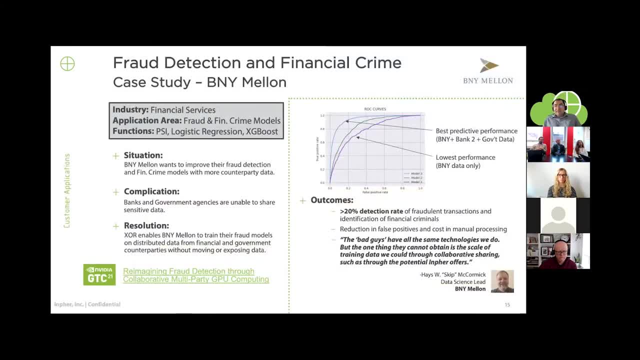 baker mckinsey. so this is the use case i'm talking about and i'll go very quickly over over that use case. so it's a use case in financial services where you want to build a fraud detection model for transactions. so that's that's use case, led by the bank of new york melon. 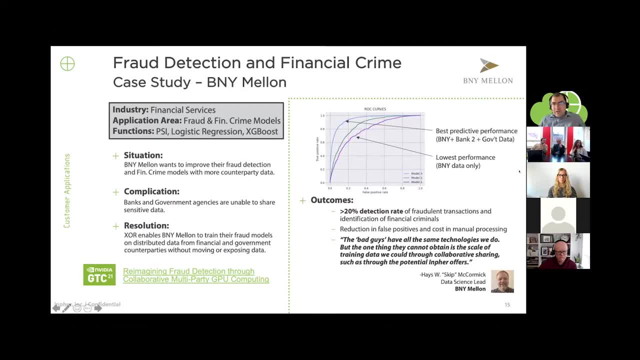 and the idea is that, if you, what you see on these curves is that if you just use the b and y data only you're getting this roc curve, that's the uh purple one, and so secret computing is capable of improving that performance of the model by more than 20. 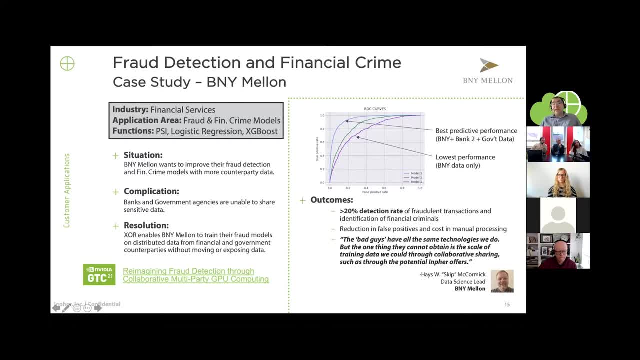 by including uh data coming from a second bank and some uh government data, as you can see on these roc curves here. so, uh, the outcome is that by doing secure data collaboration, you could actually improve significantly machine learning model that detects fraudulent transaction and thus reduce the false positives. 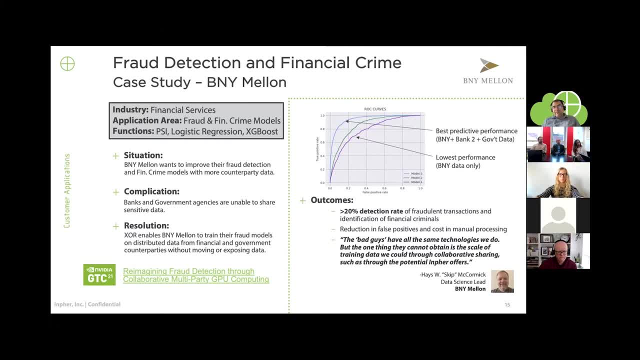 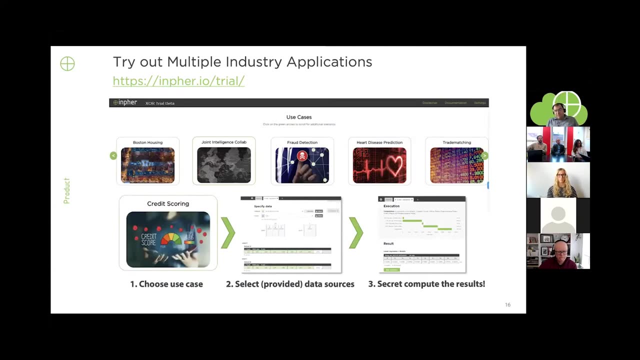 and also automate this process. That's the other advantage. So you're gaining in cost in actual manual processing of transactions. So that's the major use case And what Infer is doing is Infer is providing a simple version, simplified version of this use case. 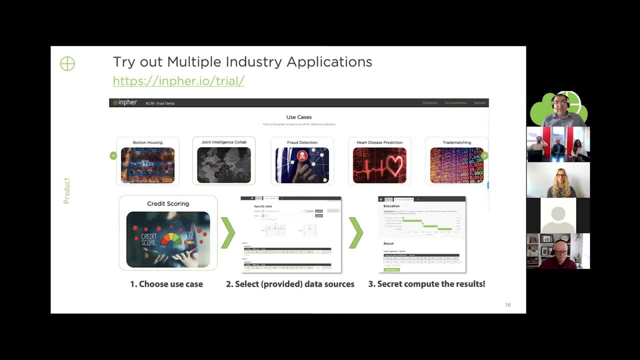 in our trial environment. So here you can see among that use case also multiple other use cases. in finance, For example, you could see credit scoring use case. You could see a use case for predicting housing prices on the right using different data coming from government. 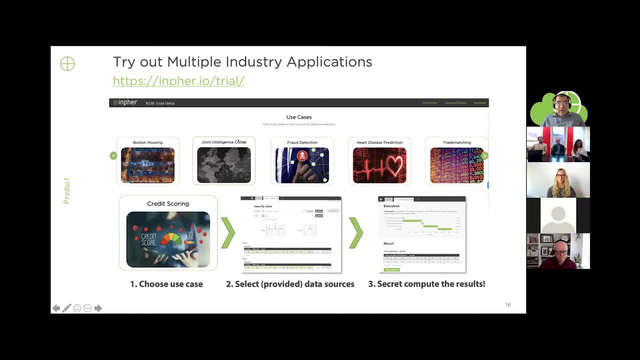 coming from real estate state agencies. You could consider a use case in joint intelligent collaboration. You have also use cases in healthcare, So that's a very different vertical. And on the right you have yet another FinTech use case on double-blind trade matching. 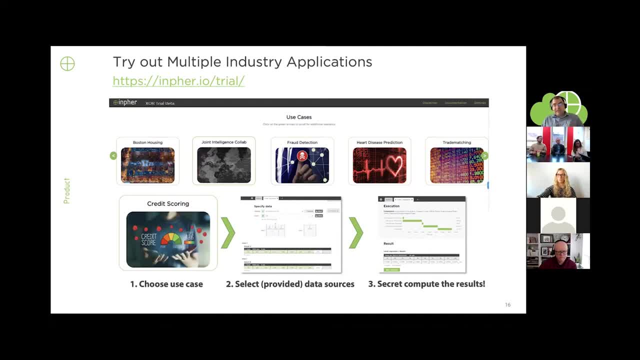 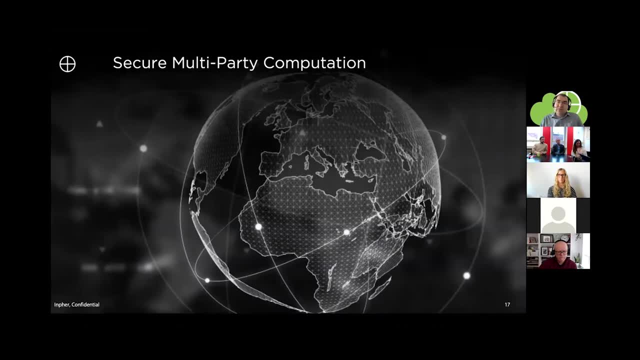 So all of these are powered by secret computing and one can actually play with them at this website. So now let me switch to the internals of what's going, what's being used in all of these technologies. So, starting from secure multi-party computation, 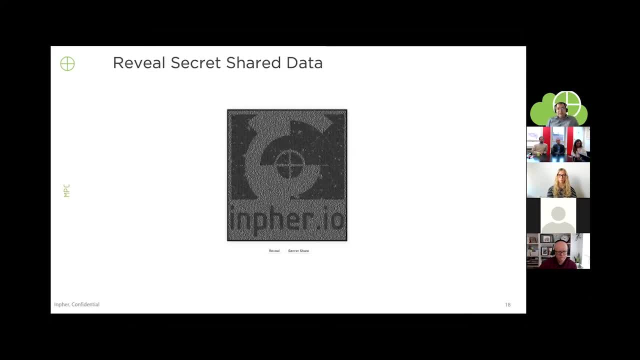 the main idea is secret sharing. So you have some data like the image that you see here, and what you could do is you could secret share that data across multiple parts. In the simplest case, these are two parties, So what happens is I'm giving each part. 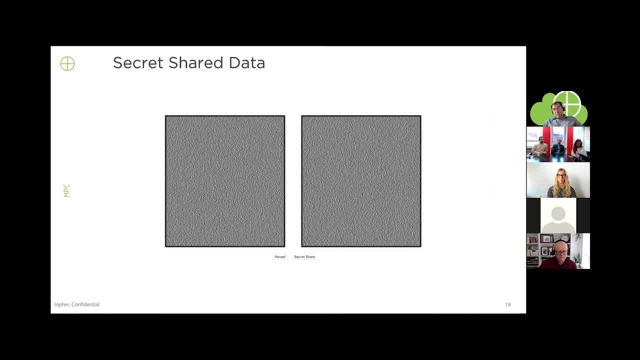 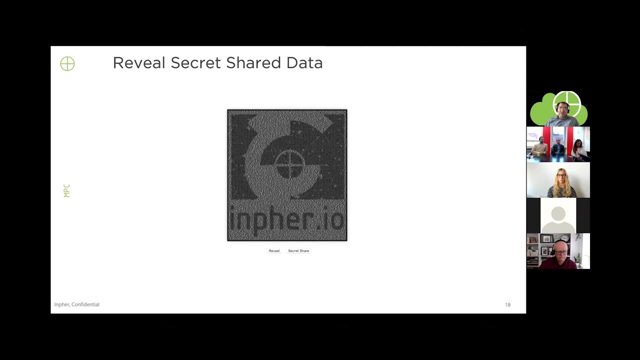 each party a random image. So this image, you can deduce no information about the original image. Yet when these two parties collaboratively use the two images, they could reconstruct the original secret, but no party could individually gain even a single bit of information about the image. 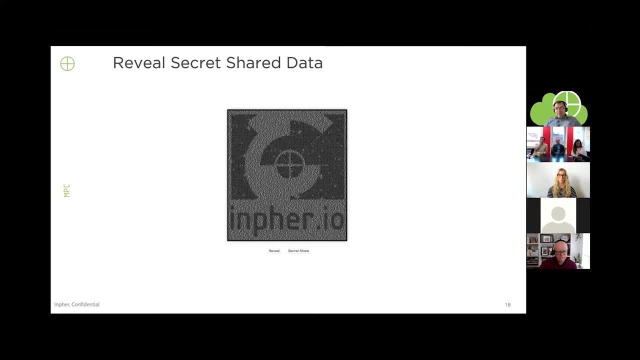 So that's the basic concept that is used in secure multi-party computation. Essentially, you secret share all of your data, that you all of your private data across a set of parties, So that way, no coalition- proper coalition of parties- could deduce anything about this data. 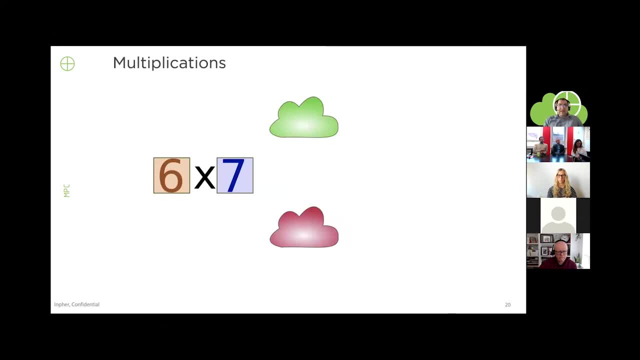 Now, how does this work in computations? So imagine that now I have to do a simple computation like a multiplication. So what I do is: my first number is secret, shared across two parties, two or more. Here I'm showing just two. 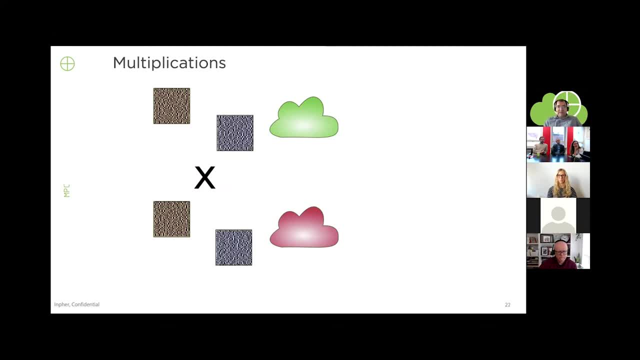 And my second number is secret shared across these two parties. So what happens is these secret shares are used by the two parties in a collaborative computation- distributed computation. However, during that computation no information is revealed about them And on the output of the operation. 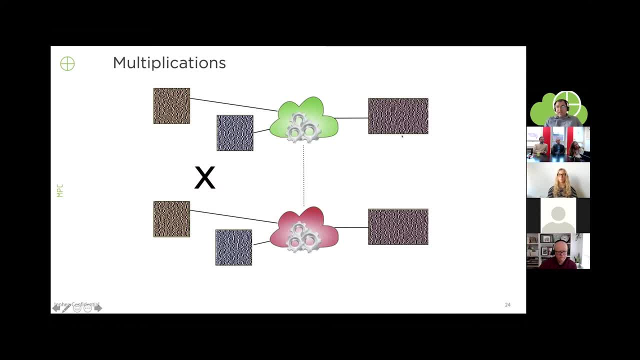 you get two secret shares as well, And these secret shares are called two secret shares as well. they could reveal the results. so if, at this point, the parties collaborate, they could get the result. but they don't have to, they could just go and continue the computation. so that's the very basic. 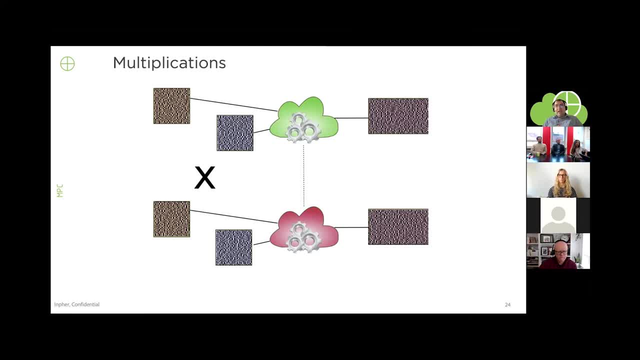 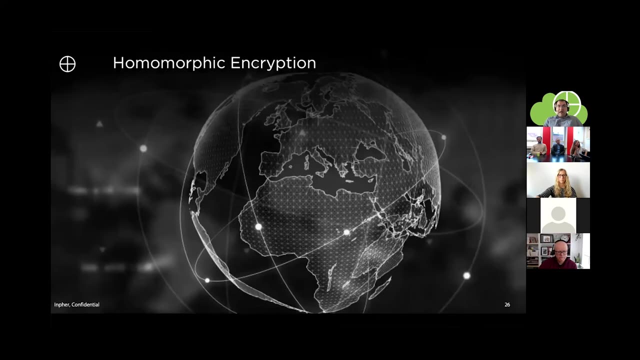 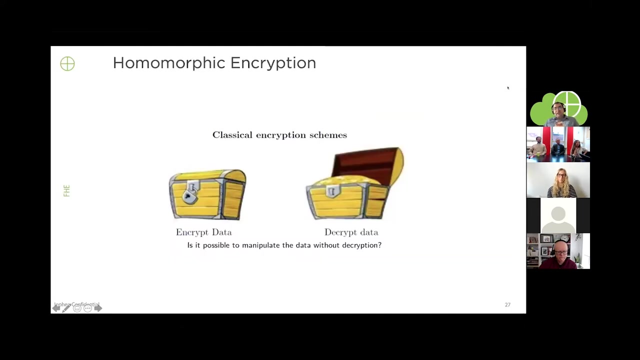 description of secure multi-party computation and the cryptographic protocols that enable you to support these operations, which is which is which is what infer has has developed, that's, that's it on a very high level. so now i have to tell you about the other cryptographic technology called homomorphic encryption. so homomorphic encryption is is very different than the secure. 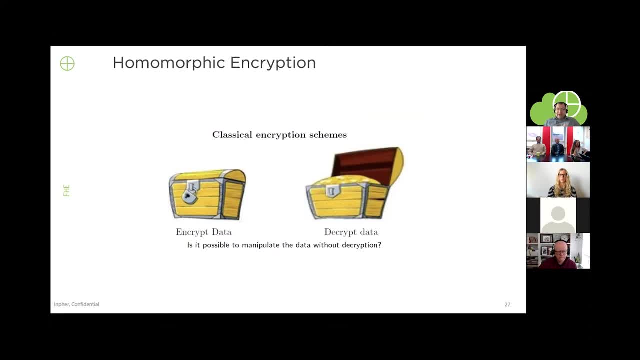 multi-party computation. so it's type of public encryption, where you encrypt some data. in this case, i've locked, uh, i've locked, uh, this, this box full of gold, and you can decrypt it with a key. so, um, what is important here is that: can you actually, while your box is locked, can you do? 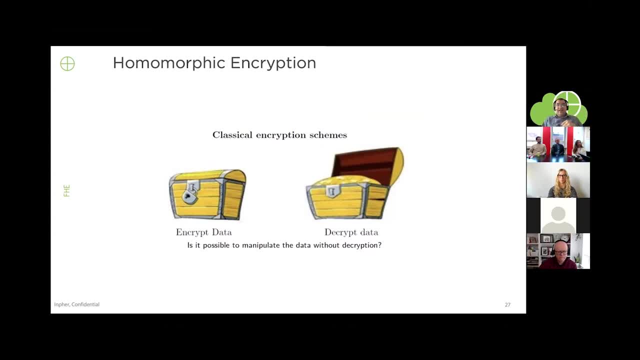 an operation on the content that's inside. so that's the typical uh like scheme that i want to show. so imagine that you have some gold inside. can you actually produce a crown or a ring without opening the box? so that's really homomorphic encryption and uh so. 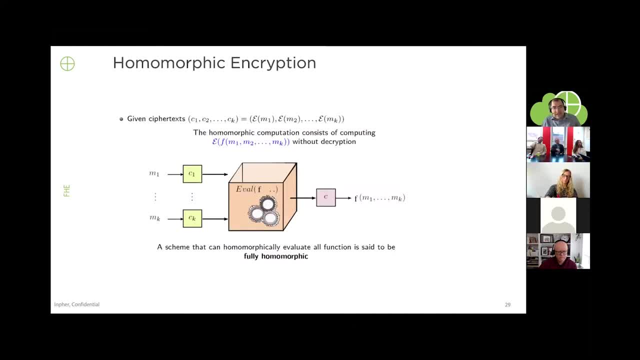 more formally: uh what? uh, what we do is: uh, we imagine that we have plain text data, these messages, and then we encrypt them. and then what we do is we imagine a box that is operating only on the ciphertext and producing a valid ciphertext of: uh, the result of the function that we, we want. 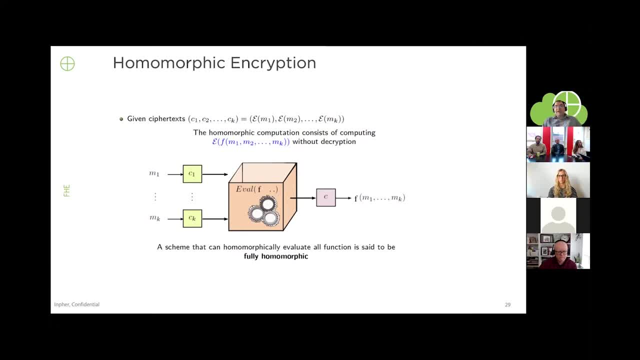 to compute. so if we support both basic arithmetic operations, then we are talking about uh, fully homomorphic encryption. otherwise it can be the additive homomorphic uh. so only, only additive homomorphic encryption. some applications require only additive, but for most of the generic computations that we want to do we require fully. so, uh, some examples of how this is used. 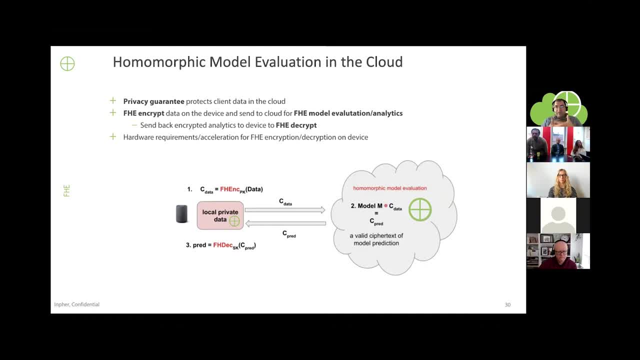 so imagine that i want to do a model prediction in the cloud. the cloud contains the model, but the data that i want to run the prediction on it's a private data sitting on a client, so it's a local, private data. what you could do in the case of fhe is you encrypt. 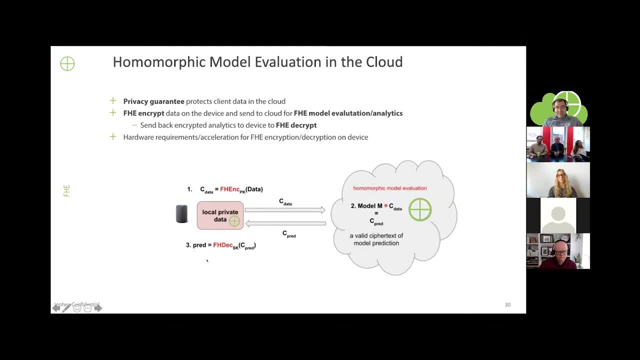 the data locally with this homomorphic encryption scheme. so you put it in the box and then you lock the box, then you send the box to the cloud and the cloud doesn't want to give you the model. it's going to run the prediction on the model and then return the encrypted 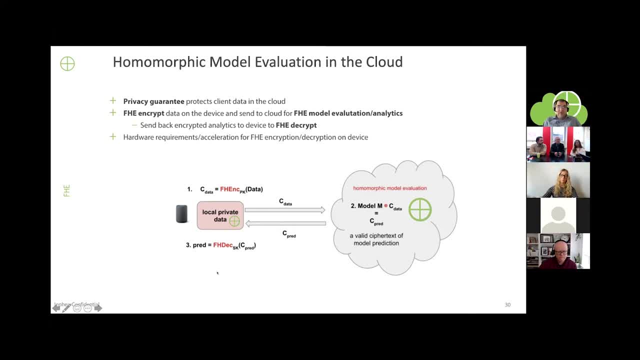 data and then you decrypt with your secret key locally on the device. so this guarantees that the client data is protected. so no plain text data is sent in the cloud and what you run on the device is basically only the encryption function. the actual model evaluation, the heavy lifting here. 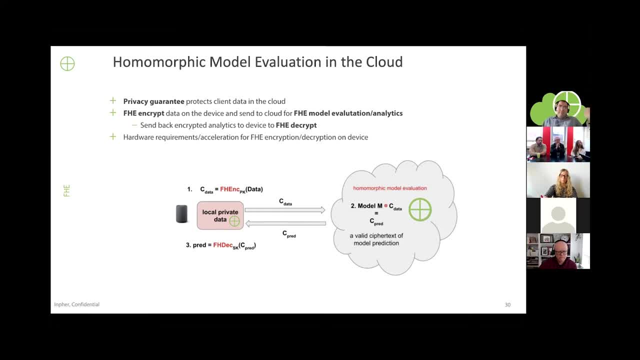 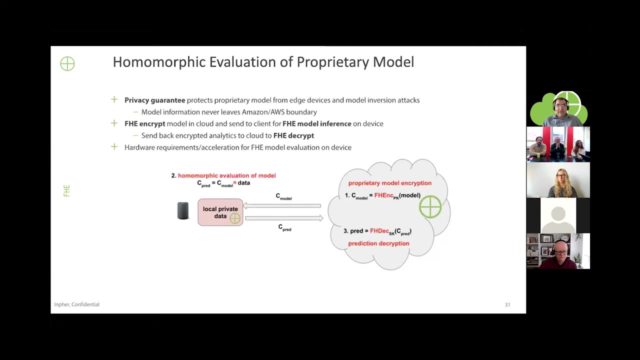 is done on the cloud and then back on the device you run the decryption. so if you want to make this efficiently complex with complex machine learning models, then you probably need some hardware accelerations, as we we at infer 2.. so the other scenario is is a bit different. 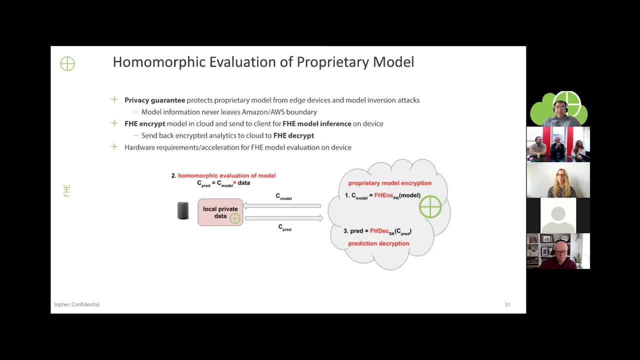 so you have a proprietary model that you may want to evaluate locally on the device. that's also a possible scenario here. we've given an example running on the amazon cloud aws. so what you, what you do, is you, you have your data locally, you don't send it to the cloud, but essentially the 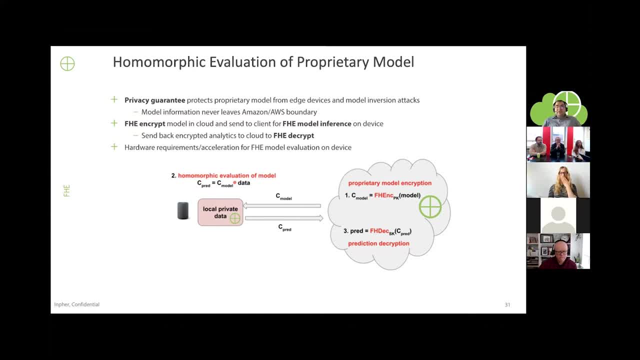 uh, the cloud asks for a prediction, so the it encrypts the model. it wants to preserve the proprietary model, and then sends the encrypted model, which then gets applied to the data locally. and uh, you get uh, the the, the prediction, which the cloud then decrypts with its secret key. so uh, 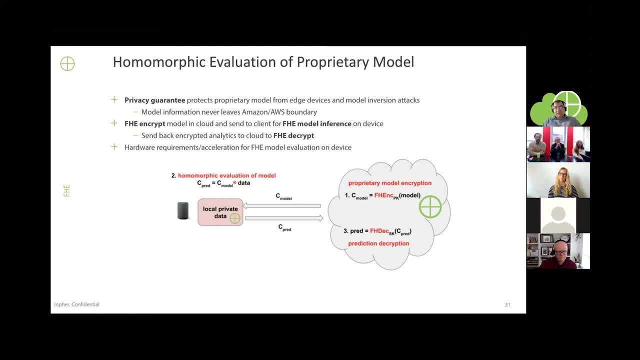 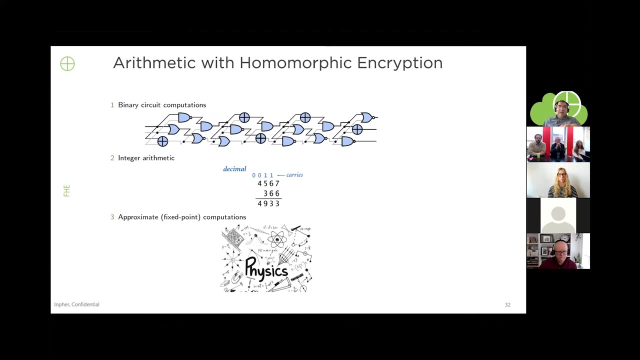 this is an orthogonal scenario of homomorphic encryption. of course, these are very typical scenarios that, uh, you could, uh, you could talk about. these are not the only ones i should mention. so, uh, now getting a bit more technical, obviously, uh, in homomorphic encryption scenarios, you may need to do different types of 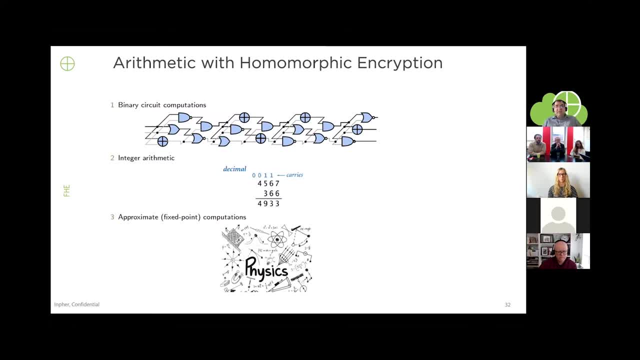 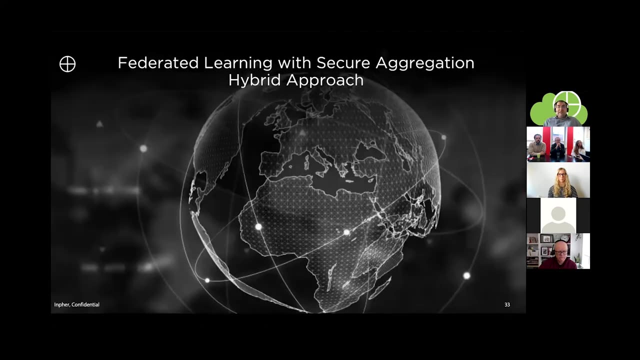 computations. you may want to compute with numbers. you may want to compute with, uh, real numbers or fixed point computations, as in physics and others sciences, or you may want to also evaluate binary circuits. so this is all that i wanted to say about homomorphic encryption, and now 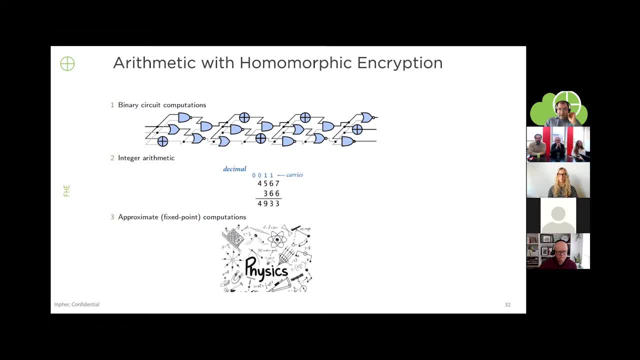 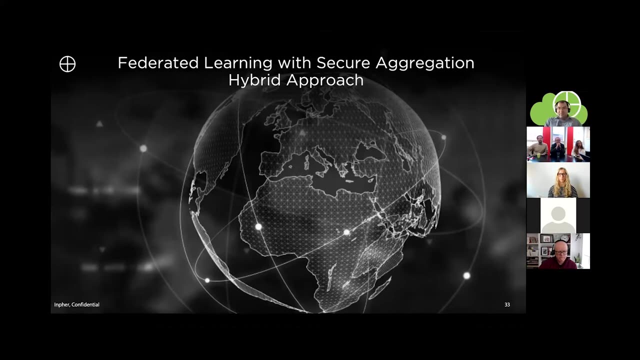 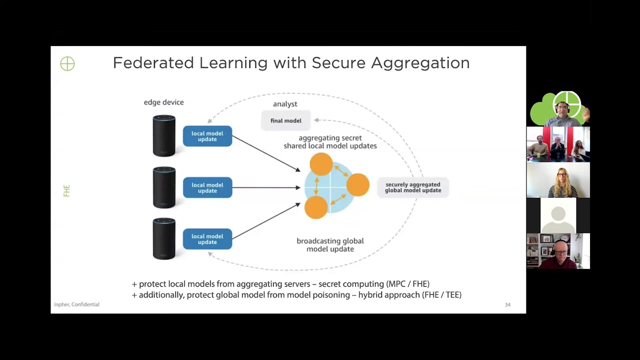 in my last slide, i'm going to talk about a hybrid combination of all these technologies, which could potentially also include other technologies, such as trusted execution environments. so this is the type of technology that you commonly see as a federated machine learning, uh, with secure aggregation. so the goal here is that you have multiple devices. 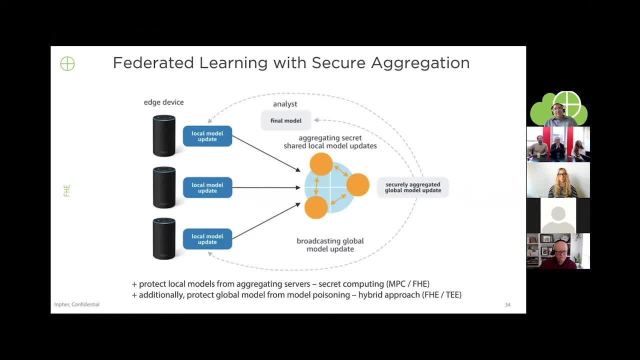 you can think about thousands of devices or even million of devices. we typically with limited computational capabilities, and what you want to do is you want to. you have data on each one of these devices, but you can't really send it to a central server for aggregation. so what you do is you do minimal. 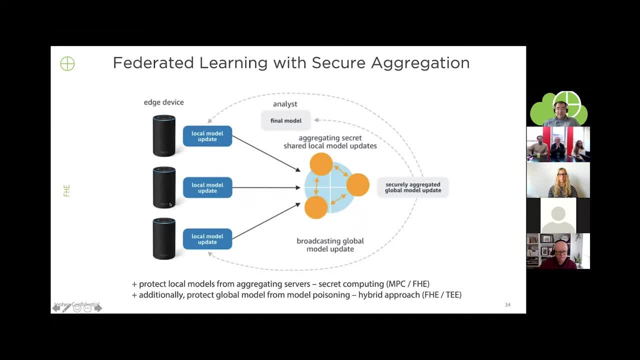 computations. with this limited data on each of these devices and you get some local models that are not at all exact, so not at all accurate. they they can't solve your real problem. but when you send all of them to a central server, aggregation server, then the server can actually aggregate. 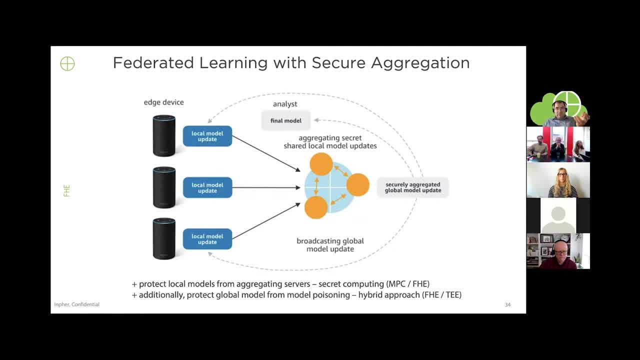 these models and get a meaningful global model. and then you iterate this process just as you do in any any meaningful machine learning training algorithms. so what? what happens with that is at the end of the computation. at the end of the computation, the analyst gets a high quality model. 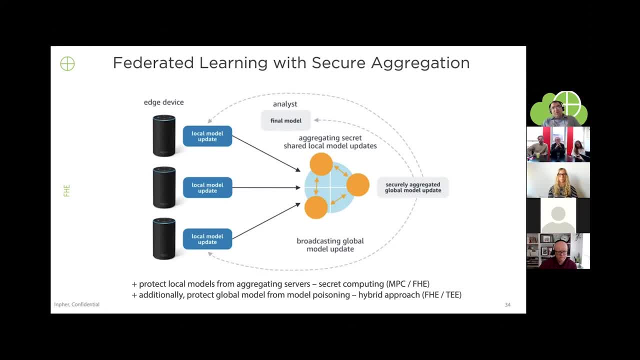 now. federated learning is very popular in many areas of machine learning these days. what is less obvious is how do i protect my local data from the aggregating server? if you just send the local model updates to the server, the server is going to learn. in many cases it can. 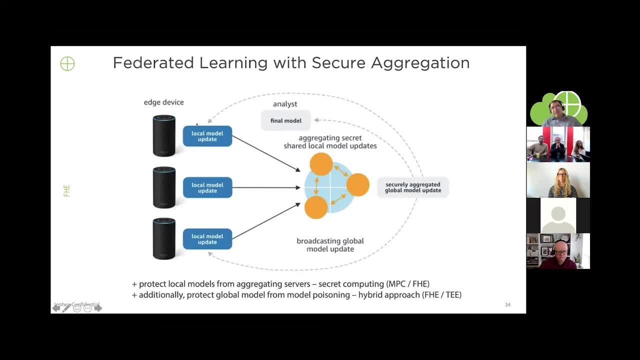 learn even all of your local data. so you don't want that. these are called model inversion attacks. so what you do in this case you use secret computing, npc and fhe to actually protect these models from the server. so the local models, the local model updates, are protected from the server. 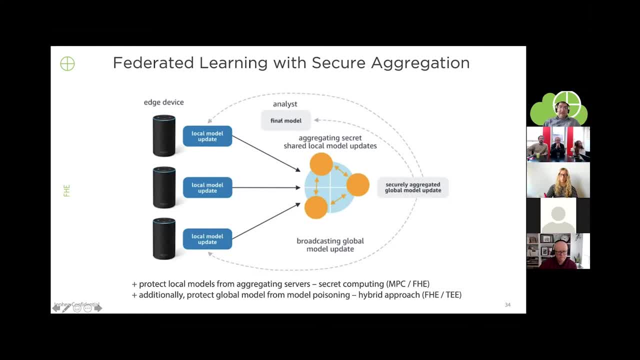 additionally, if you're a data analyst, you may ask a question of how can i protect my global model from being poisoned by some of the clients? imagine that you have a malicious client that is trying to poison a model, so bias the model or make it put some intentionally some, some biased data. so this is: 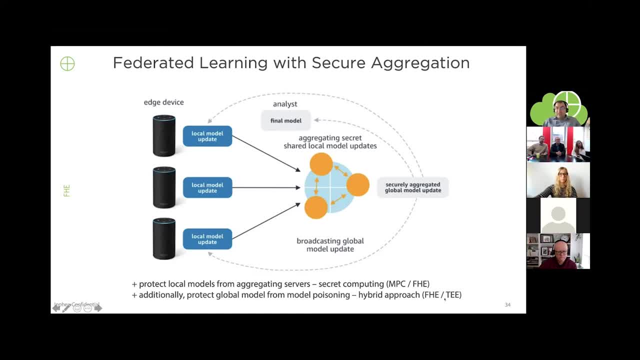 where the other technologies, like combinations of fhe and trusted execution environment can, can solve your problem. so in a sense, that's a typical example of how hybrid computation could occur, and orchestrating this hybrid computation is a non-trivial task. in privacy, enhancing technology infer as a company. 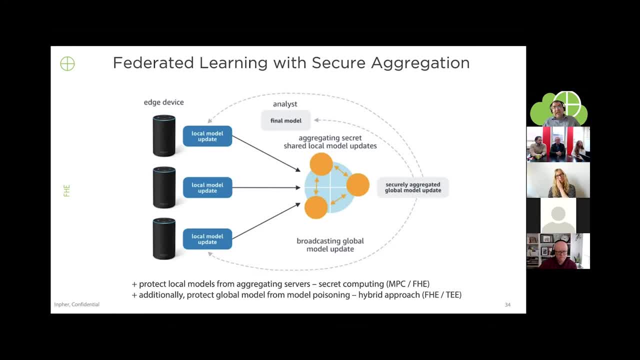 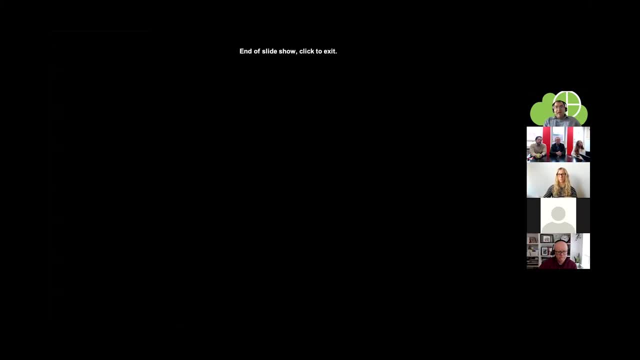 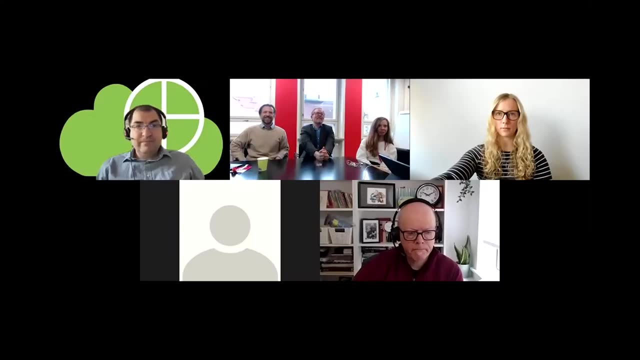 for example, is building non-trivial development tools that allow you to orchestrate this whole computation yet make it very intuitive to the data analyst. i'm going to stop here and ask for questions. um, um, uh, really really great first presentation. uh, people here are cheering us. 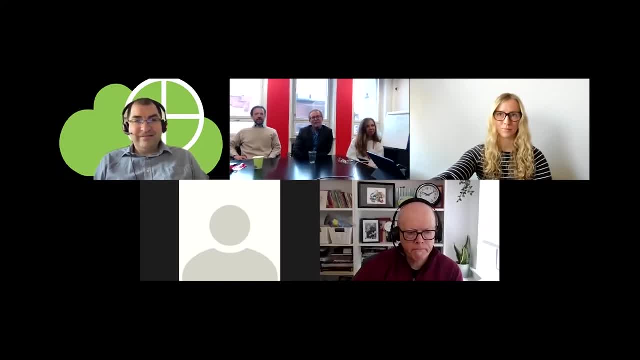 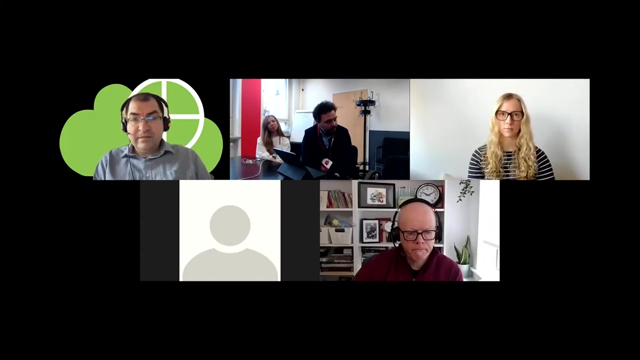 uh, it was a real nice overview. um, and first, before uh coming up with the questions from from from this round, uh, mia, are there any questions from linkedin live? no, um, um, So the first one is the how to deploy our products on AWS, uh, on the AWS environment, so we could use standard AWS services to power. 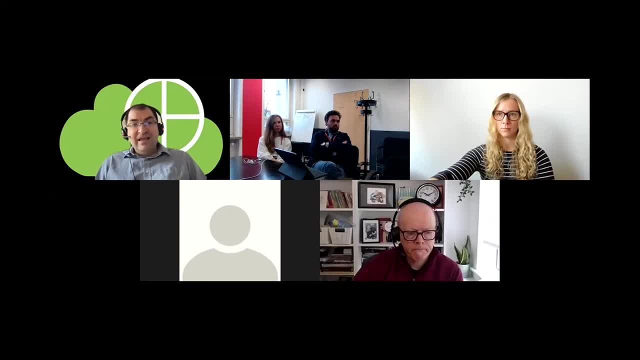 our orchestration. that's, that's all that i said. of course, infer is- you would see in the press that team for is funded by amazon alexa fund, uh, so here what i'm saying is is very generic. so what i'm saying is that you could deploy, uh, infers, uh, you could use the AWS services to power. 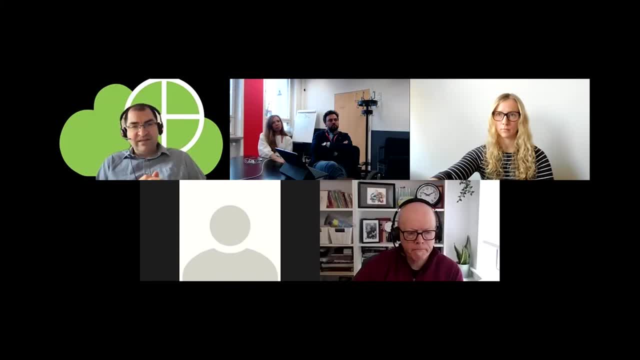 of infra-private sequencing capabilities. I may first of all say that this was a very, very impressive presentation, What you have done, and also the way that you described it to a less technical person like myself that I can catch up with the bits and pieces. 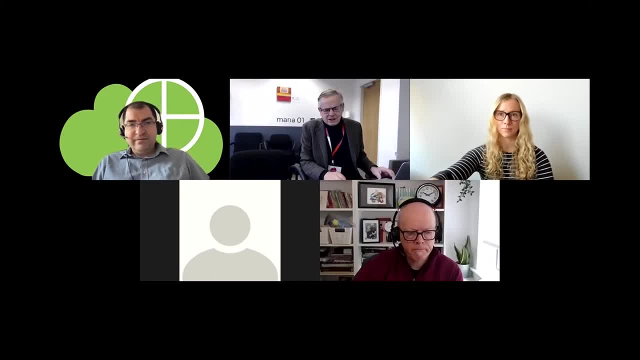 of it and see the potential. Here in Finland we are just in the process of updating the legislation for against money laundering And it's obviously, as we know, the way it has been done in the past has been outrageously expensive and silly and inefficient and so forth. 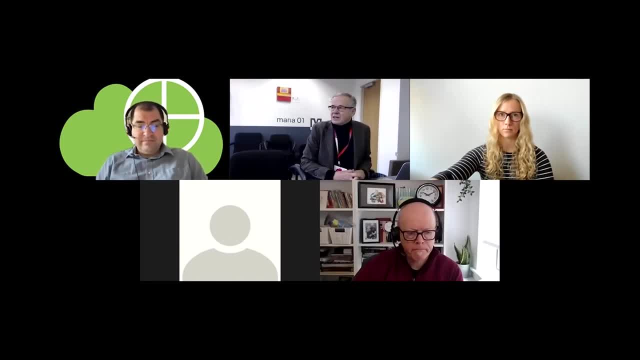 And what you are really showing here is a kind of a key to make it both efficient and, about all cost efficient. So the banks in the world should- should grab this right away. Thank you, Thank you, Thank you. So just a comment on money laundering. Infer presented a money laundering. 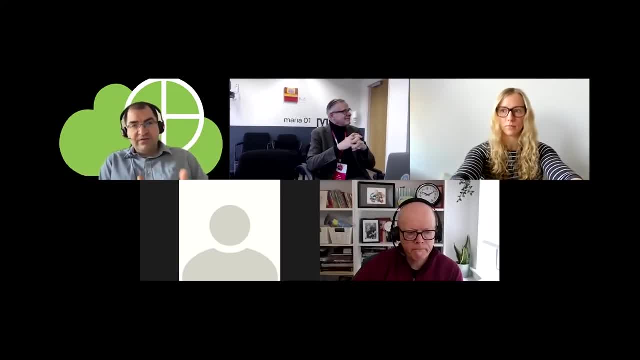 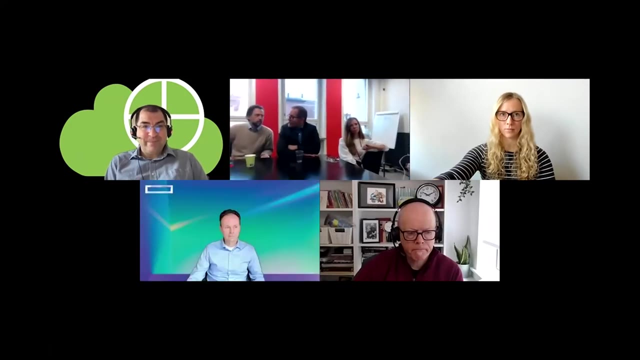 QC case two years ago, a big money laundering use case in one of the biggest conferences in applied cryptography- real world cryptography- in New York. so there is a whole presentation on that. So final question from Ville: Yeah, So we have a lot of banks, of course, in the audience, myself included. 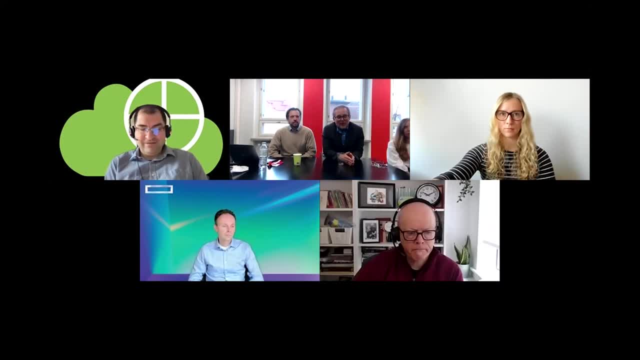 Now one of the things we realized when we started working with these emerging privacy enhancing technologies. But sometimes they are quite difficult to explain, especially articulating how to get started. So a simple question: If you, if you would talk to a banking audience right today and the banks 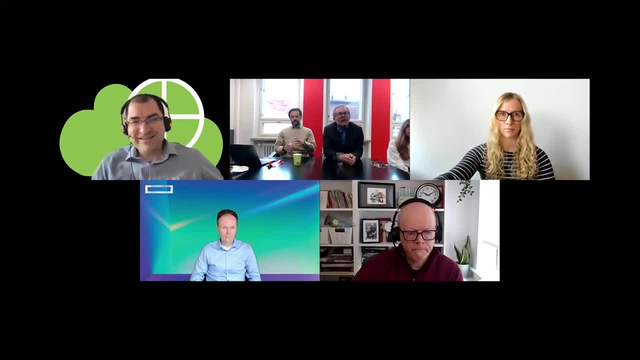 would like to get started on something like anti-money laundering based on these principles. how would you kind of tell them to get started? So the very first step is go and subscribe on trail. So that's why we put trail. I should say that, from a business perspective, trail is. 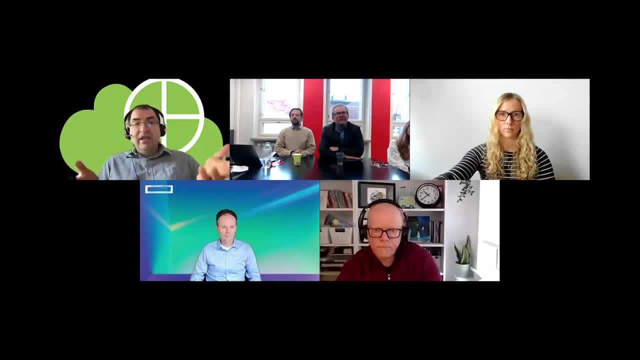 the uh, an excellent educational tool, And you can even tell me how this works. So, uh, for obviously, uh, the, the, you're absolutely right. So the education takes most of the time and uh, and effort, and this is very important. 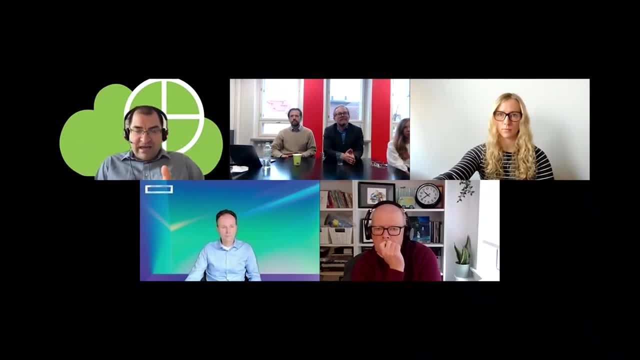 So people should understand what the security implications are. but the first thing to begin with is just getting your hands dirty with this technology. is is very important And that's why we built trial. it's free and people can use it. Yeah, Thank you very much. 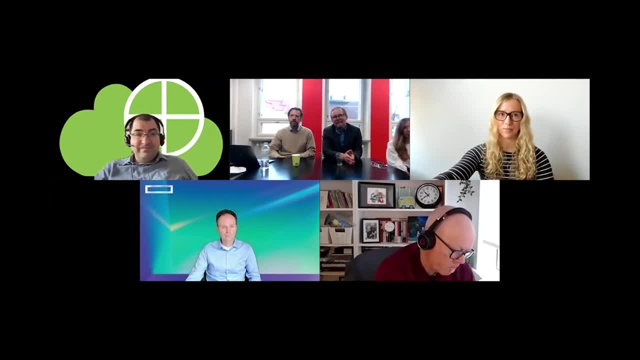 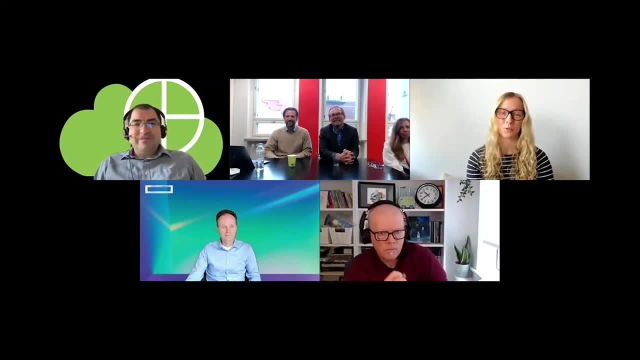 I think we should also. there is a one question from Alexander Uh for mostly AI. So, Demeter, thanks a lot. I can only second what was already said. super great introduction to this topic And I really liked this analogy of creating a necklace without opening the box. 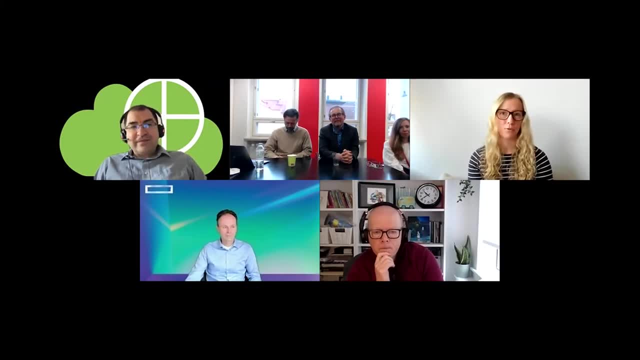 One question Uh in regards to state-of-the-art performance of fully homomorphic encryption Uh. last time I looked into the topic it was said that oftentimes computation takes 1000 to 1 million times longer than when uh computation is done on clear text. 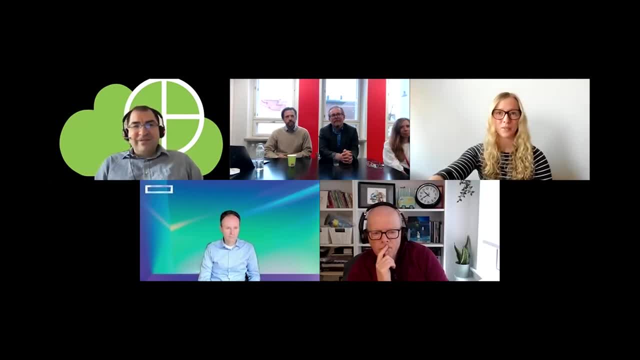 What state-of-the-art when it comes to performances. So thanks, Alexander. That's an excellent question that I should have commented on earlier in my presentation. Uh, so fully that's. that's exactly the point where we uh need to uh think. 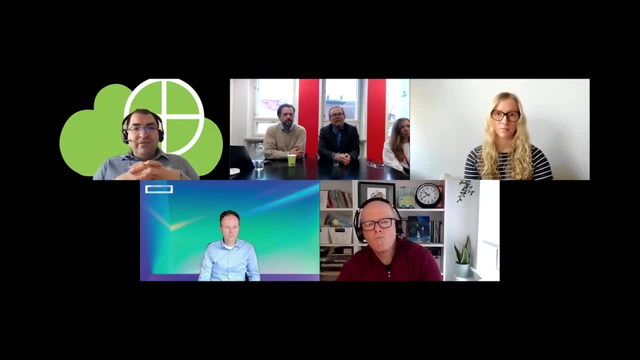 about these hybrid approaches. So, uh, basically, fully homomorphic encryption on its own is not going to scale to the point where uh to the to the complexity of the models, as well as the complexity of the data that you, you put into training these models. 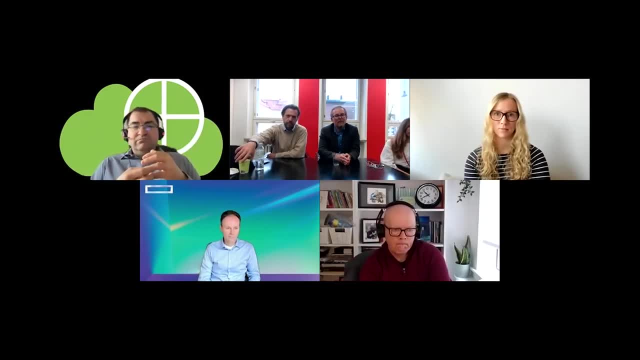 So, uh, fully homomorphic encryption, Uh, so so nowadays there are lots of uh improvements, hardware accelerators, uh, hardware acceleration efforts. We at TRIMFER we do a lot of that. Uh, that's a lot. 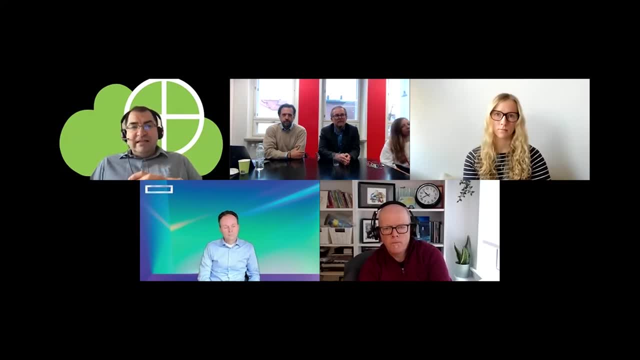 We do a lot of that work, uh, but what we've identified really is that, uh, for each application, there is a trade-off between the scalability and the technology that you use. So, for instance, secure multi-party computation these days scales much more. 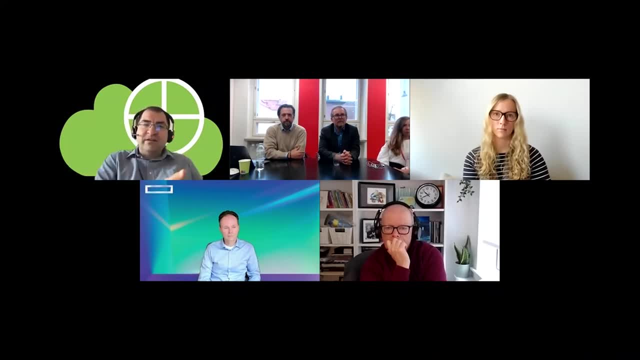 than fully homomorphic encryption. Yet secure multi-party computation cannot solve all of the problems that FHE can solve. So even further, uh, for cases where secure multi-party computation cannot scale, that's why we use this federated learning, and that's the excellent example of how you put together. 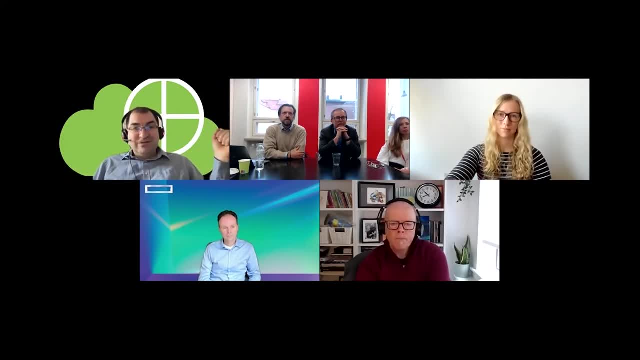 all these technologies in a hybrid solution. So, yes, your, your question is very important And according to the size of the data and the complexity, for example, if you're building a neural net model, then you have to think about really, uh, how you put a hybrid approach. 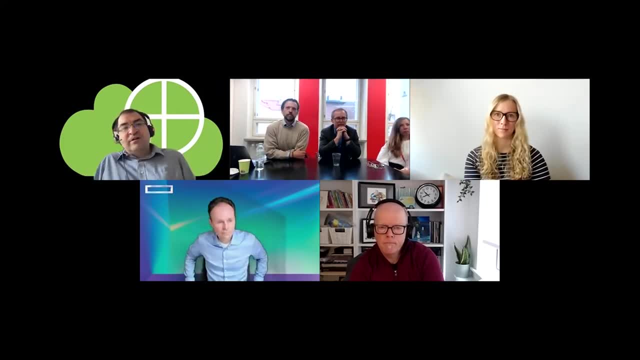 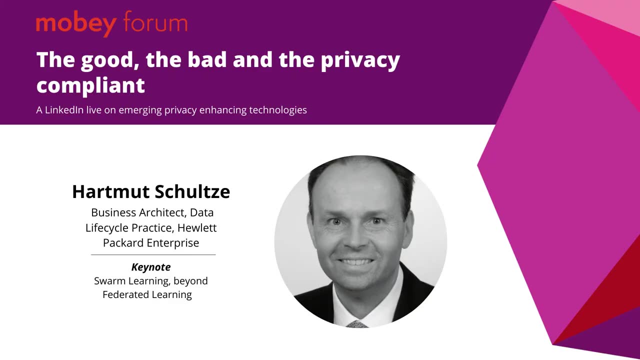 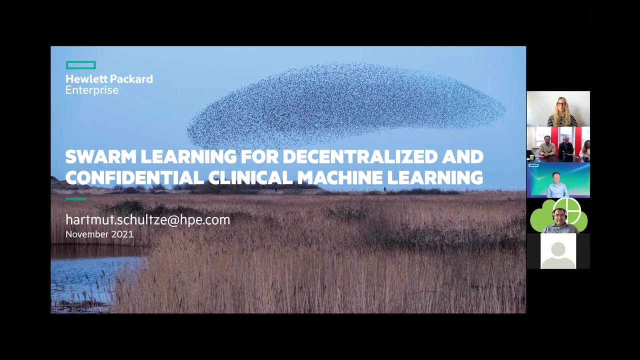 This is achieved also by, like very sophisticated developer tools that that need to be built. Thank you very much. Yes, I would like to talk about decentralized and confidential clinical machine learning, And now I have another field, Uh, so, as Dimitar was uh talking about, 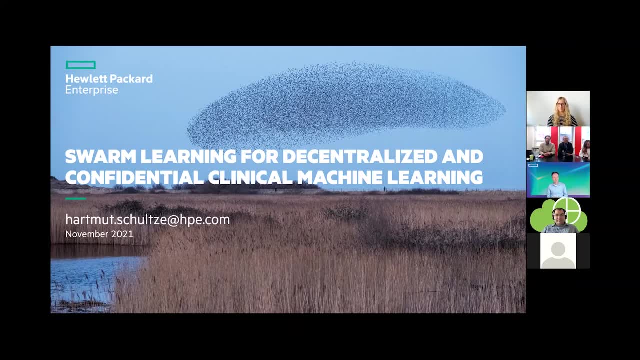 Not only banking has the problem of privacy and uh confidentiality also. medicine does have it and I have a use case in medicine. but I'm I'm pretty sure that you will immediately and very fastly uh also connect to this as well, as this is pretty much the same topic. 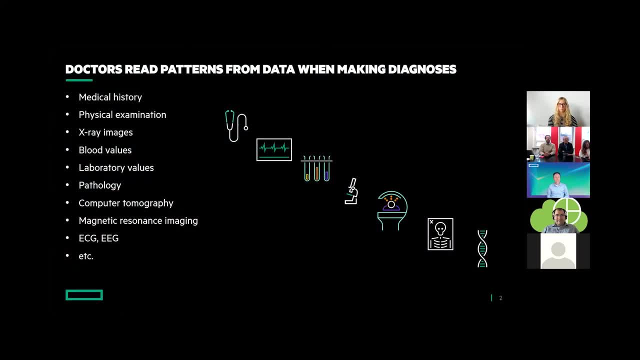 what we're trying to reach here. So so let me go through this role. Uh, I started, so so what does just do doctors do? now I, we, we got an escape. We're trying to, we're trying to shift it to another field and into another domain. 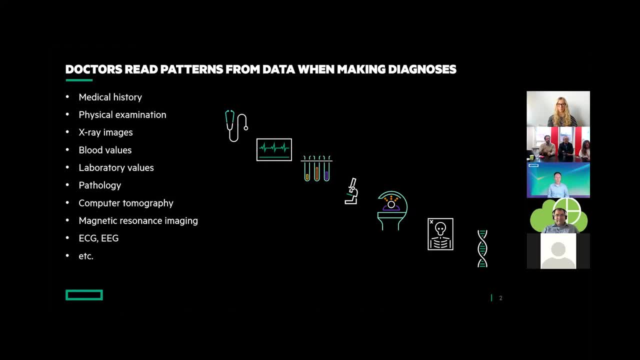 Uh, doctors read patterns uh from data when making diagnosis. um medical histories, which are privacy, uh information. So PII data, physical examination, X-rays- If there's no metadata added, it's a well anonymous data as well already. or histological. 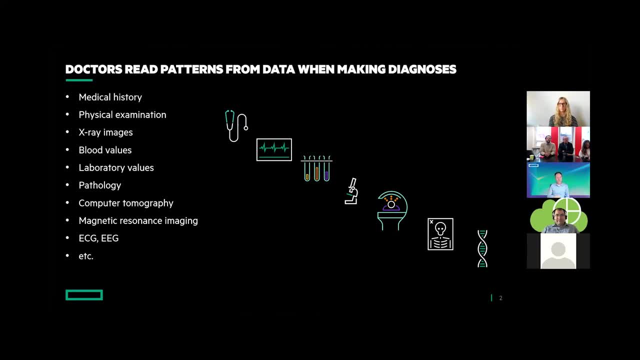 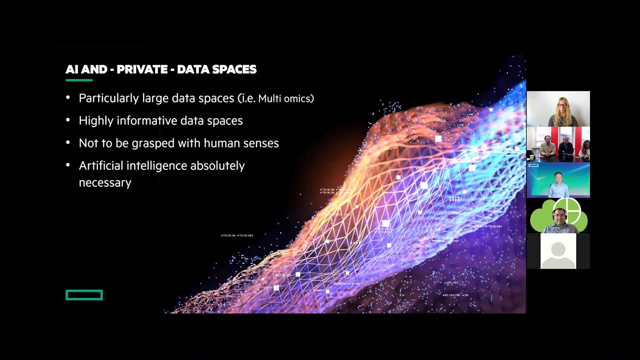 diagrams, computer tomography, pathology, MRIs, which is computer vision, which is NLP of patient records. So it's patterns within data, And basically that's the same thing we have in banking as well. So there's another notion, though: if we go into the future, we're seeing: 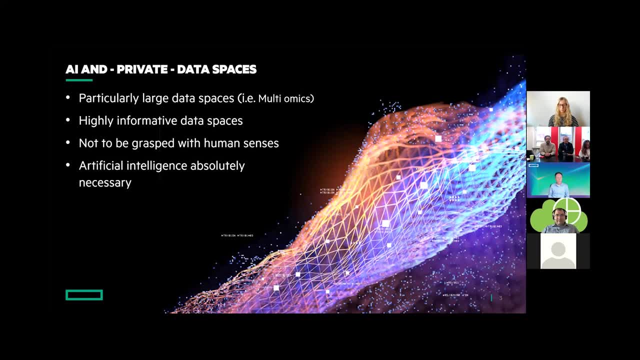 that we're especially going into extremely large data sets. For example, if we're talking about the highest resolutions of MRI data in computer vision, then we're talking easily in the terabyte space, where we have a one single picture which is then to be analyzed in conjunction with a lot. 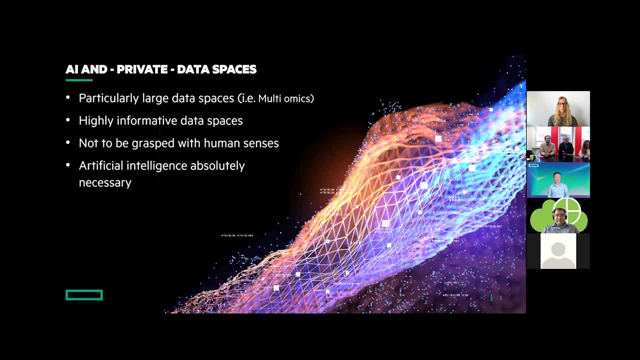 of other pictures or scans what we actually do there. Same thing happens with omics data. So omics data as the raw data, very private raw data which has to be analyzed. It's highly informative, but it's not easily to be seen. So, for example, a human sensor: we, as humans, we cannot sense this. 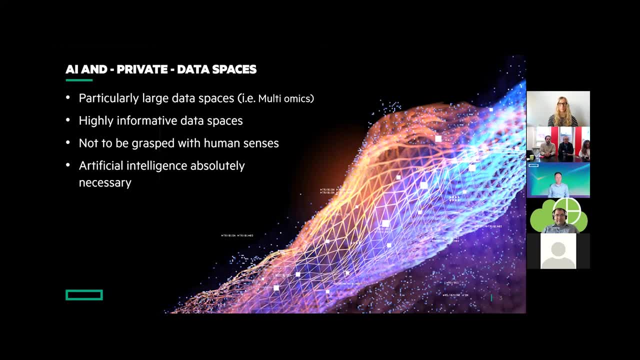 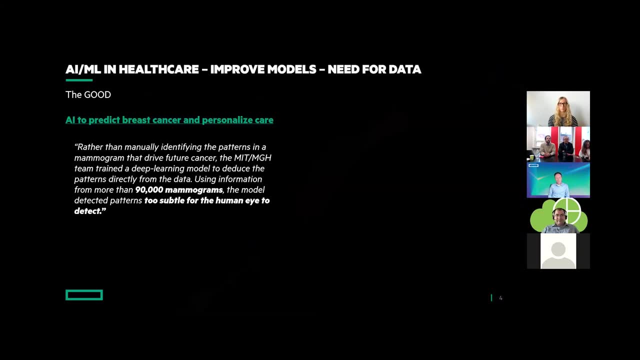 So we definitely need artificial intelligence, which is a way of getting patterns on heavily private data and to create those data spaces, to get patterns out of that, To actually make this usable. we've seen some different studies. So, for example, what you see on the left side, there was a study in 2019 where a professor at MIT took 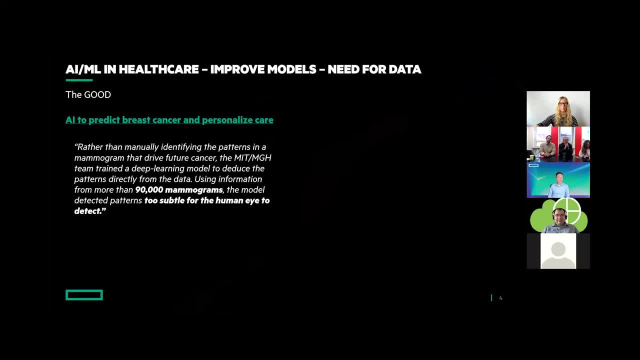 together 90,000 mammograms and they detected in the model actually patterns which were too simple for the human eye to actually detect. And that was exactly like Dimitar. I like this picture you just shown about. if you only have one. 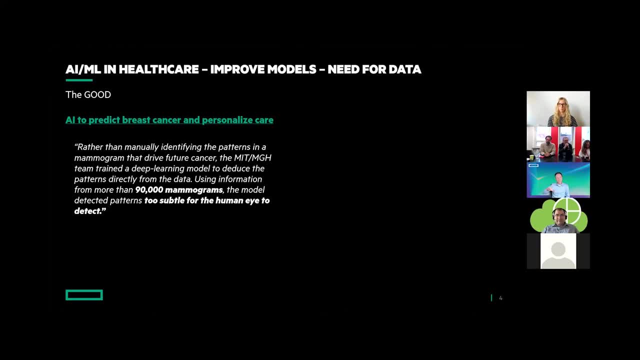 and then you go across and then you have a large data space. then you get a better area under the curve which is potentially going to the accuracy towards one. So the more data we have in excess, the better we actually can get. The other thing is which then might work in a scientific setting. when you get all 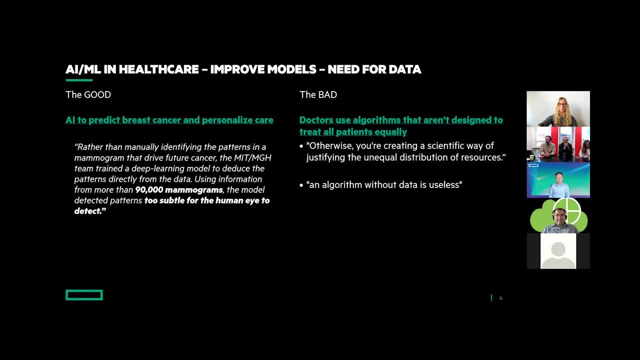 this data together to make this happen. If you don't have access to such data, each model is going to be pretty much useless, And that's exactly the curve which was shown there. So what we actually need to get out the real information out of that, we need to have the right access to the right data And, of course, 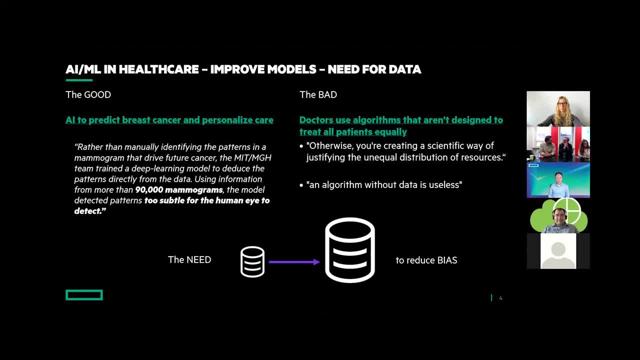 it needs to be privacy preserved. There's another topic here which is extremely important is bias in the data. We, as humans, we have a bias And nevertheless, each doctor has a bias because his experience is within what he is actually doing. 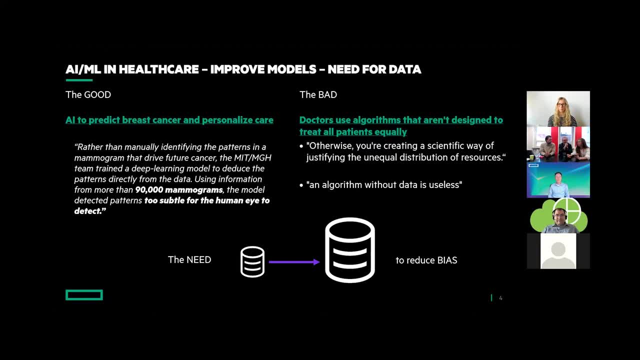 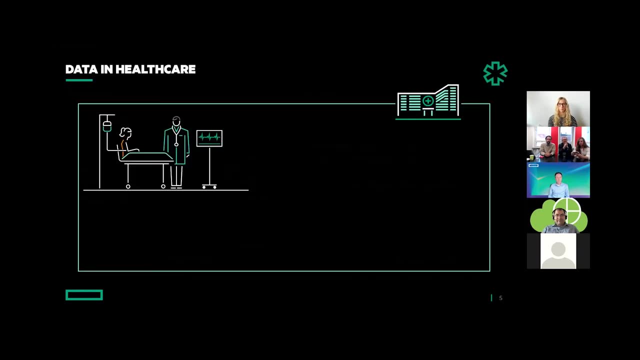 So if we would like to go into a data driven perspective, to get this more in depth, of course- then we need to have this access to this data silos, which are definitely across entities, So it's not under control of a single part. So when we're looking at a data pipeline in the hospital, 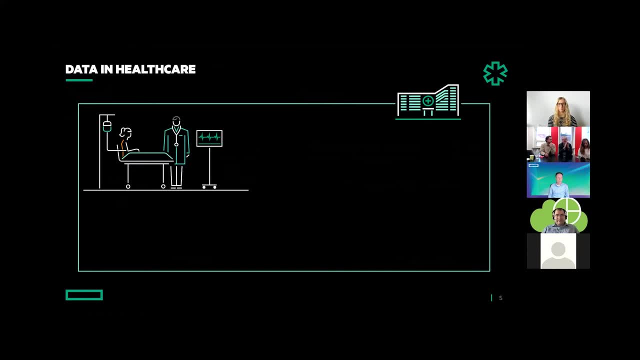 you pretty much have to have a data pipeline in the hospital, You pretty much have a patient. then you have different diagnosis instruments like microscopy, MRIs, blood tests, genomics. You generate data which is private, as said. You apply algorithms. 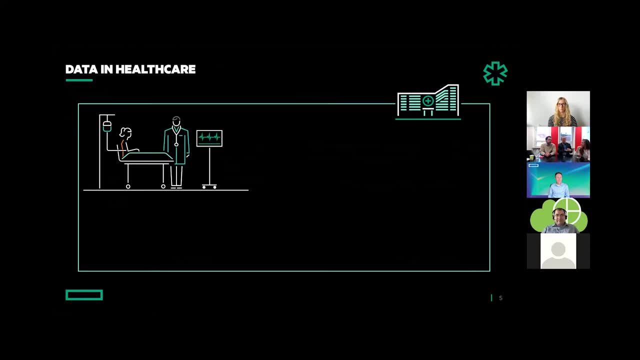 to it, And then you have this within, for example, one hospital, one clinical hospital, or within a consortium which brings this together, what we see in different countries, for example also in Switzerland with the SPHM. So now depicted here is a hospital. 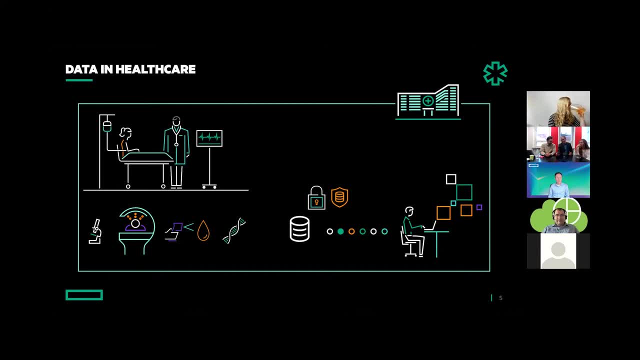 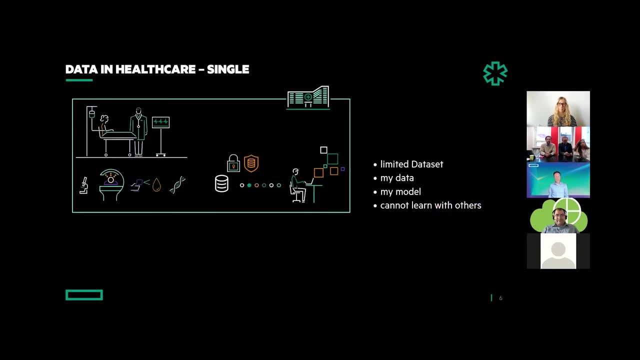 But it could be, of course, the same thing with a bank, And that was the intra versus the inter. So if we look at that, it's only a limited data set. It's the model a certain hospital has or can actually work on, and they cannot learn with. 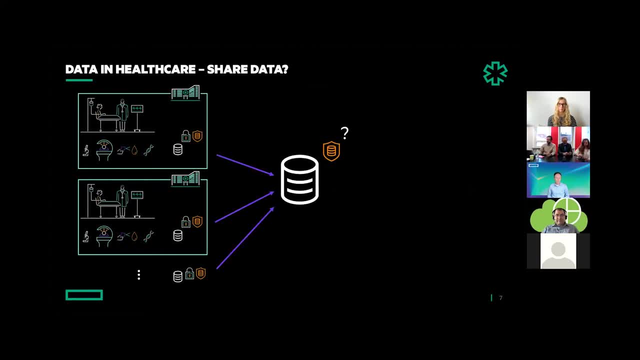 others. So that's, if we do that, single on a single space, So putting this data together. that's the initialized model, where we then potentially apply homomorphic encryption to the source data, which is large. We just heard that scaling this is not necessarily the way to go. 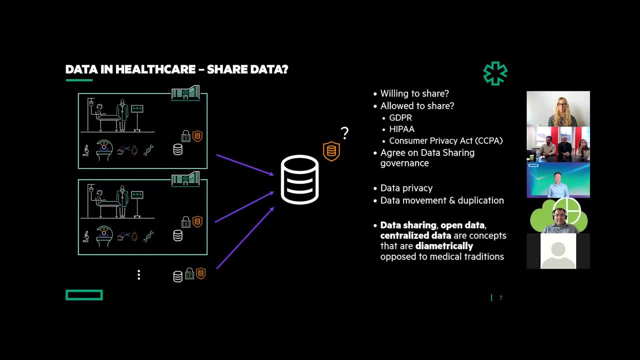 Then we could put it together in a secure way on secure multi-party environment. But then we have the topic of the governance, which is on top of that, And of course there's GDPR, And in health space we have HIPAA or the CCPA, And we need to have 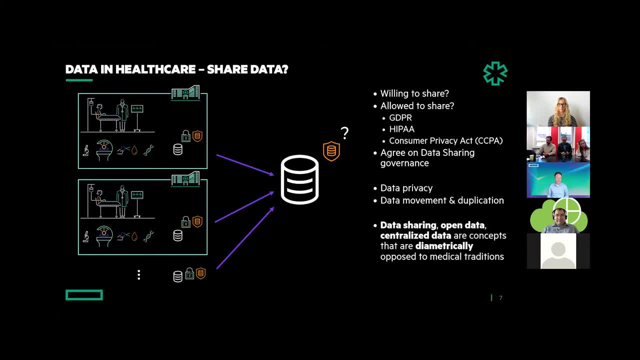 the data sharing agreement. So the willingness to share is also a topic which needs to be solved across the data privacy. Now you heard me saying about the large data set. There's another notion- might not be as much applicable to banking data. 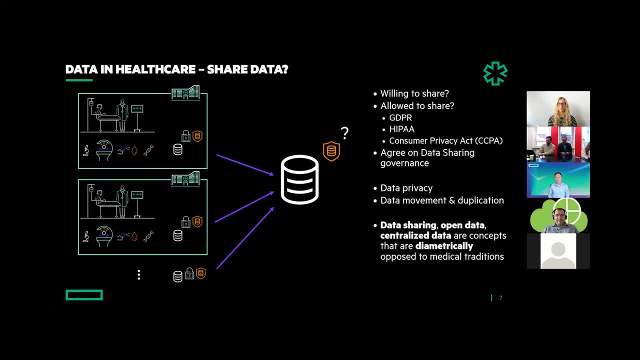 because that data is, per nature, not as large as it would be in the medical field, But there's a notion of data movement. As soon as I start to move data, I of course need a lot of energy. So, for example, if you just look at the computational space and everything, what we 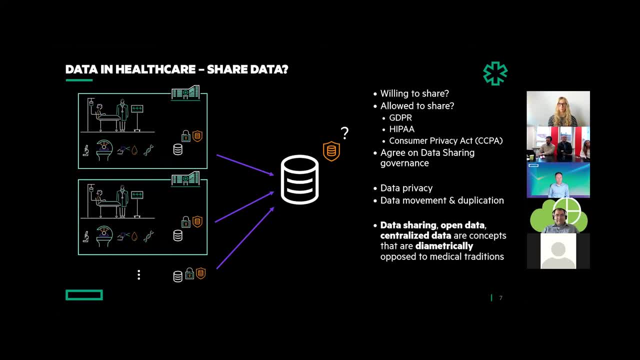 would like to do. in AI, a lot of energy is actually used- Not as much as we need it currently in the crypto area, but nevertheless. about one third is only to do with data movement, So the more data we are going to have. 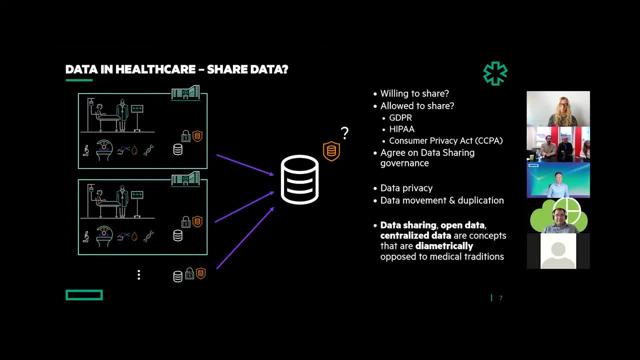 we should prevent data movement And also, of course, data duplication, Because as soon as I duplicate data from any kind of whatever enclave, it is then in the wild. So as soon as I have a duplicate data which is then decrypted, of course I cannot control it anymore. So, being really 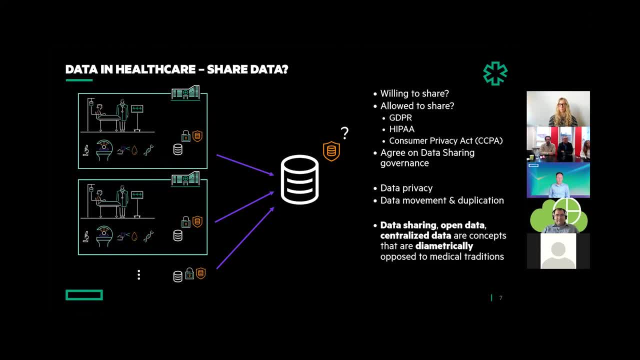 sovereign on your own data. you need to take care about duplication And, as such, data sharing and open data should not be done, at least not in the medical field, And I was just in a conference and we had the notion of, or the title was, share without sharing. So what can we actually do? 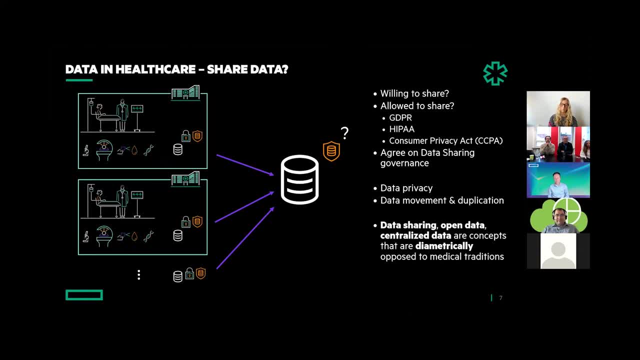 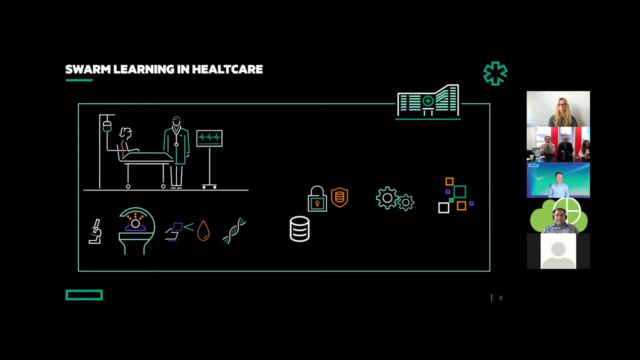 to make this happen, to actually get or share the insights, get the insights of a consortia of working together, collaboratively working together, without sharing the raw private data. So how can we actually approach this? So, same procedure in the medical field. So we start this, but now we do it differently. We 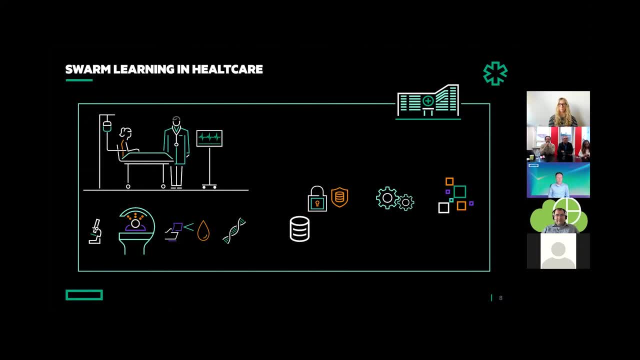 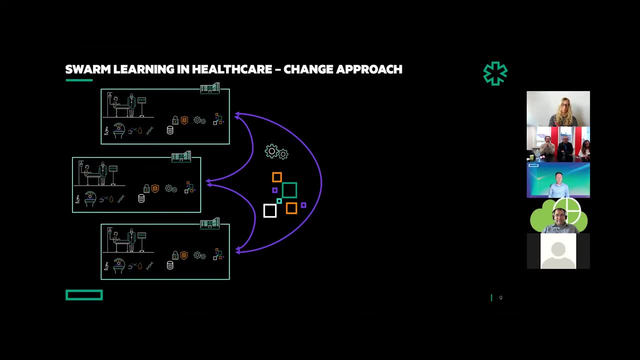 bring the algorithm to the data. So send the model, send the agent to the data instead of vice versa, And that reduces the following thing: So, looking at that, hospitals can work together. That is exactly the federated approach to that, And so we share only the insights, We share the results. We 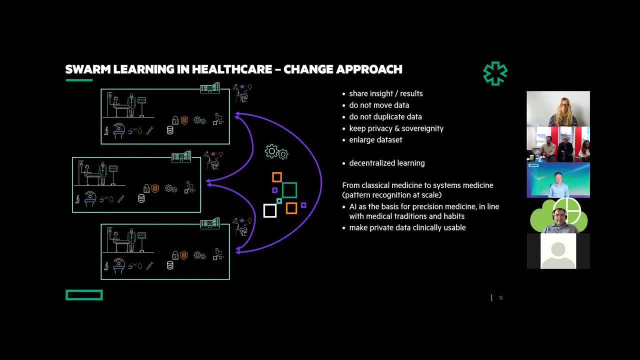 do not move data, We do not duplicate the data, keep the sovereignty but at the same point in time enlarge the data set. So that is a decentralized learning Here in the medical field. we can then come from a classical field of medicine into the systems medicine. 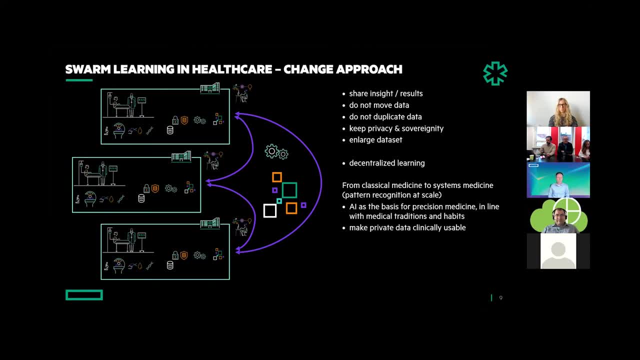 So AI is necessary. We need to have access to a lot of data. We need this collaborative approach and make clinical data also usable. Now there's one additional thing where we say we have to do on a governance perspective: the right abstractions layers. 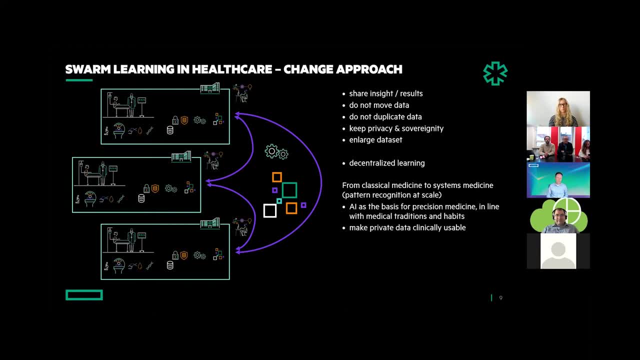 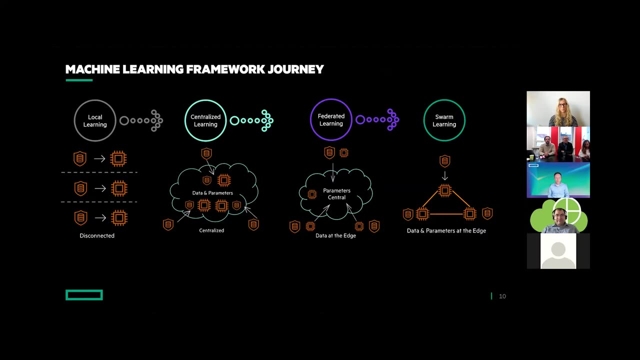 so that we can apply the models, which are then from one party, and have the data. maybe is from another party to do the automated decentralization and keep the data private in such a swarm. That's why we call it swarm learning. So now looking at the different frameworks and the 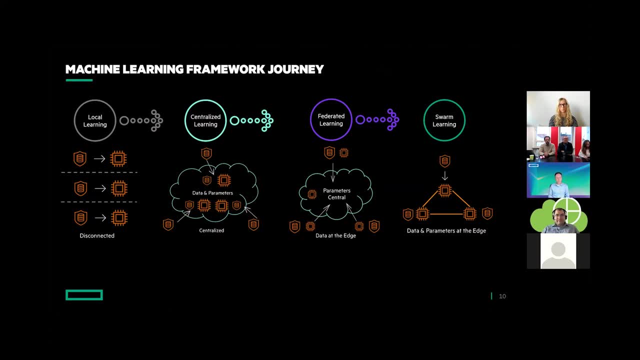 journey we're currently seeing. That is something. local learning, of course, separate. as said before then. typical notion of how we approached AI in the beginning was centralized learning. So we put all the data together, We did move the data, have the parameters together, do the results, And now 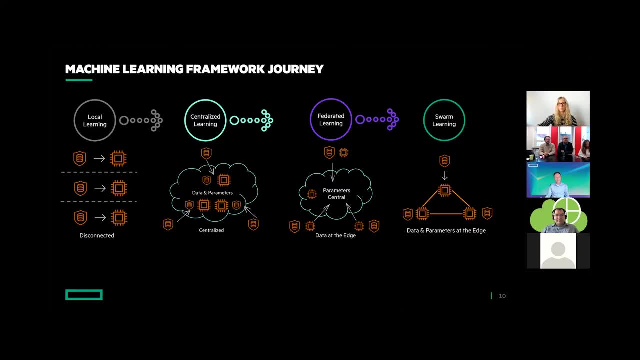 of course. if I have that, then I might apply directly homomorphic encryption, So I have the data safe, but still the data comes together. And then we have the federated learning approach, Like Dimitar was just mentioning in his last slide, And the typical notion, and that was also. 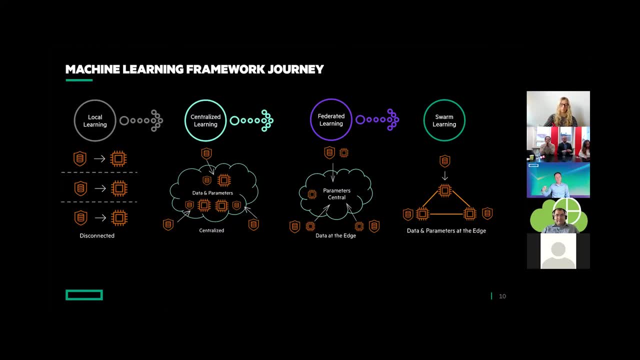 and this is about the almost overall situation- that we do the computation at the edge, at the data source, so that the raw data is not leaving that. Nevertheless, from a consolidation of the parameters, this has still been done centrally. And now I ask you one question. 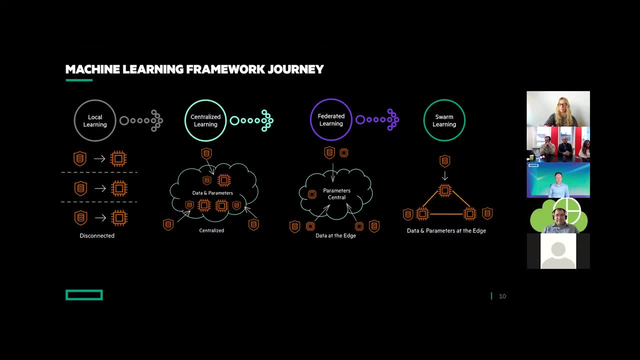 If we have a certain situation where, let's say, 10 banks work together, who is going to be the bank who is leading the central server? And there I'd say we will not be having it, because there's no primers under Paris. So we're not. 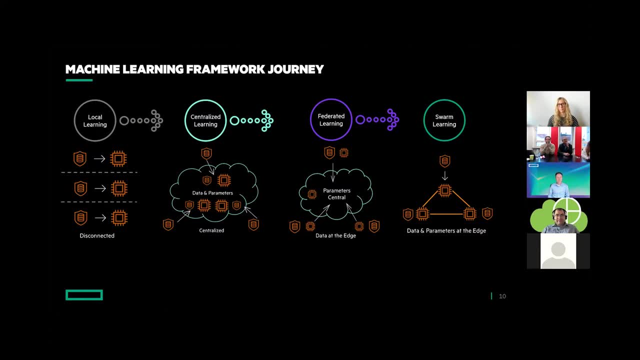 seeing this one bank who has done the power to actually do that- And that's why we say swarm as a function- now decentralizes that as well. So the consolidation of the parameters and the data is going to be at the edge, And that implies then also that we have a privacy enabling leaving raw data at its source. 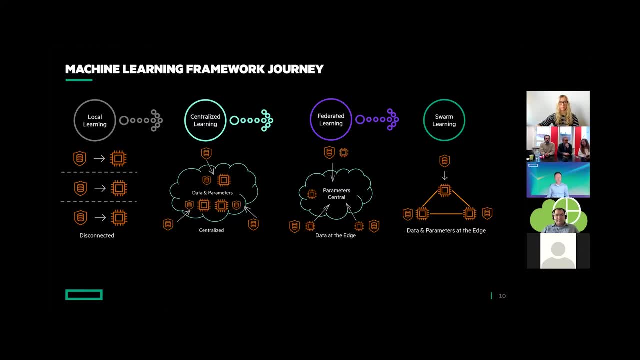 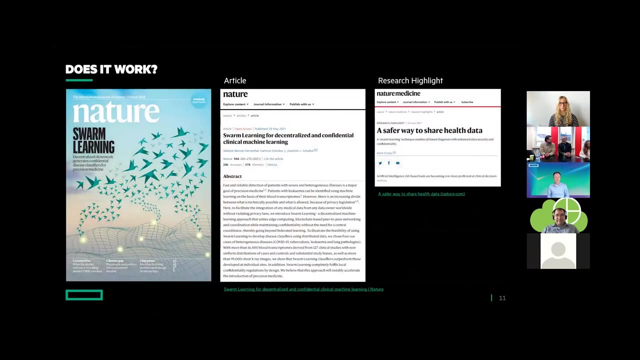 a collaborative machine learning and then training all parties equally in sharing the results And based on a common agreement on how to actually do this. So how does it work? Well, let's see, or did it work? So we just published this year a paper in Nature where we applied this technology to a setting of 16,000 data sets in different diseases. 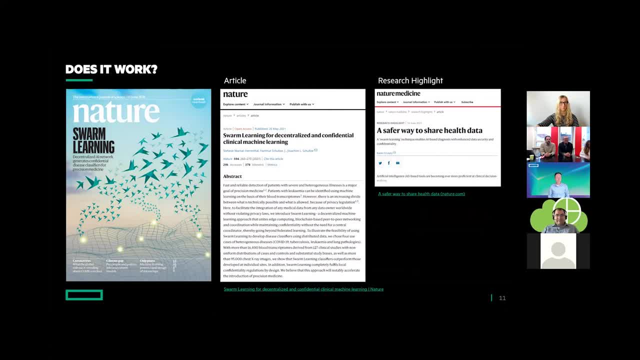 So we wanted to make sure that this technology actually works. Also, we applied it to x-rays- 95,000 x-rays which are publicly available- and then we split up this data set and see: is it the same thing what we get from a centralized model or from a decentralized model? 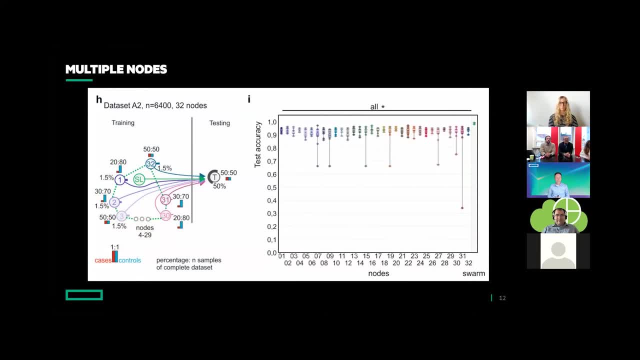 What we actually could see, and that is what you see here. it's mimicked. It's that we split out in different permutations a lot of permutations on different nodes, So each of these nodes had a subset of the data. and I must say one very important thing is we knew exactly what the result was going to be. 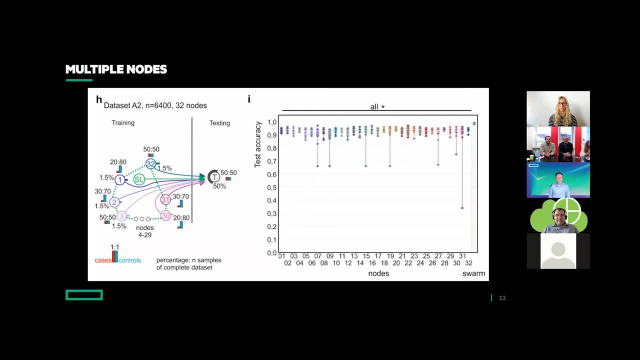 So we knew exactly what the accuracy was, because it took about three years of data curation before and, with classical linear regressions and classical models, that we knew what we would like to see or what the result should be. And there we applied this swarm so that we could actually see and prove that learning together in a way to spread out all the information is equally as good as a central model or better. 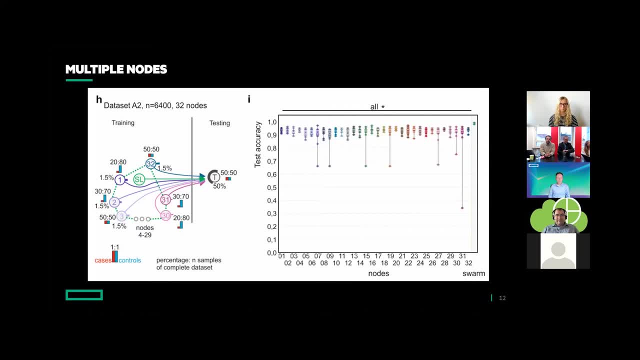 So what you see on the left side here is a training phase. You have 32 nodes. in this way, You have 50 or different prevalences on the different nodes, So they have different information about that. We applied this to a global testing set. So typically what you would be doing in an inference phase as well during your then applying of the model- 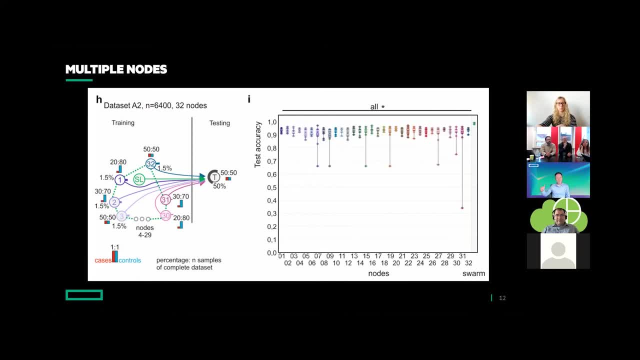 And what you see on the right side is the different nodes, different permutations on that, And what we see throughout our 50,000 runs we did is that swarm was always better or unparalleled. And what we see throughout our 50,000 runs we did is that swarm was always better or unparalleled. 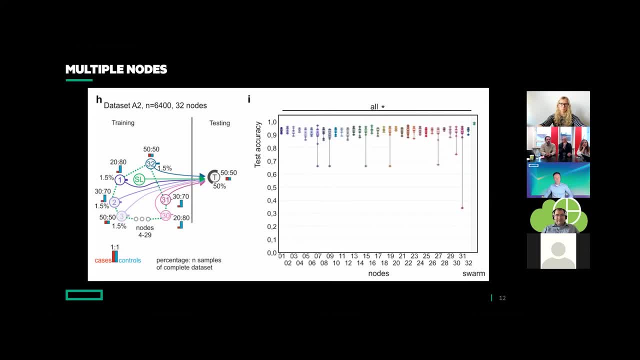 So it doesn't matter if you push all the data together or you leave it where it is. So there's one thing to this notion that you have now the choice just splitting this. Well, to be known, if you don't move data which is private and you leave it with the data controller at the source, the raw data, at the source of where you actually have, Well to be known if you don't move data which is private and you leave it with the data controller at the source, the raw data, at the source of where you actually have. well to be known if you don't move data which is private and you leave it with the data controller at the source of where you actually have. 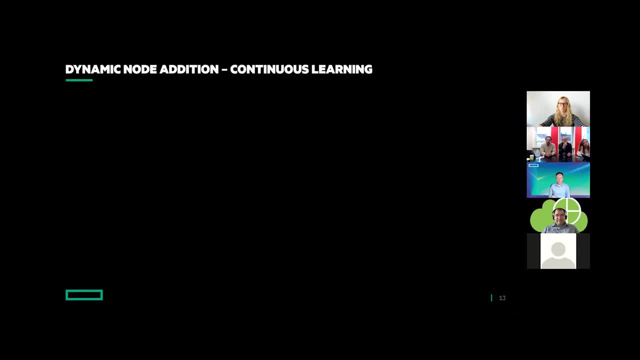 you've grab the data and stopping them from moving to the source of where you actually need to actually view this information with the data controller, this one, And actually it's ramping up place sacrificies for this one, we realize. So there's another notion here. 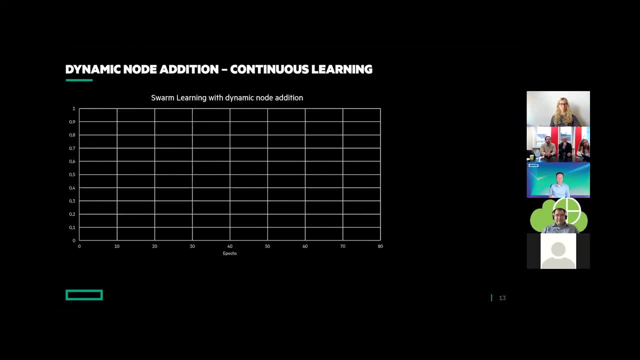 What we tested them as well, And what you see is is the pox on the, on the, on the bottom's and the accuracy on the vertical line. And what we did, we took some dynamic addition of different nodes. So, for example, we had a probable council right. 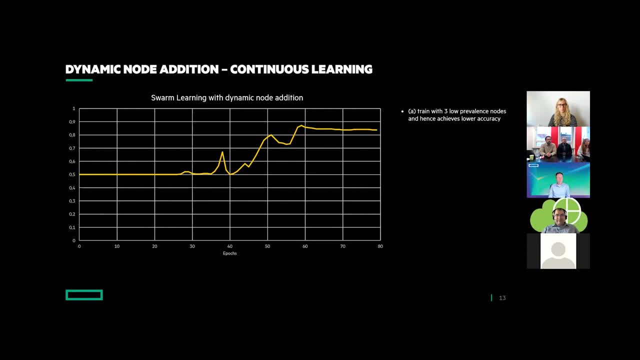 training node which had a low prevalence between the nodes, And we of course, as expected, generated a lower accuracy. So we took the same thing with different nodes who were better in training, so they could converge to the better accuracy throughout these epochs And the epochs. 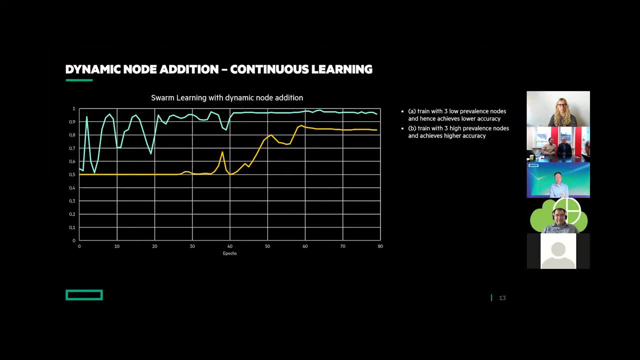 is always a certain time frame where the nodes by itself train on their own. So they have their data set where they train locally and then we combine this. So if we put this together- so low prevalence nodes and high prevalence nodes- we then saw we could throughout the 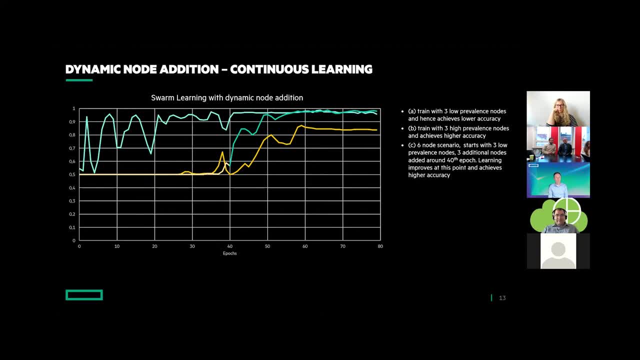 training phase, add additional nodes and still learn as the swarm together in a much better fashion and reach the right accuracy we were striving for. So that means that you can dynamically add additional nodes throughout the learning phase to actually create better predictors on what the different patterns on. 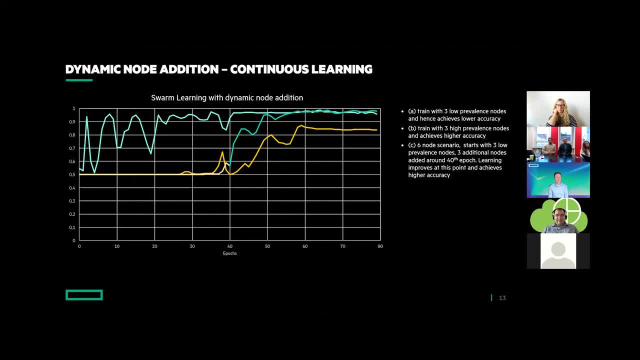 the underlying data structures is. The same thing works as well with the learning phase. So if we put this together, we can actually add additional nodes if, for example, in such a network you lose certain nodes throughout the training. So even if 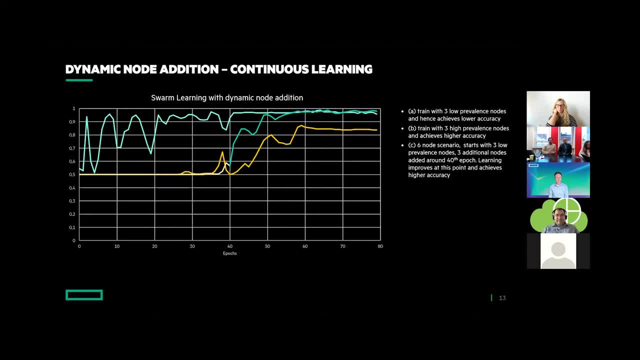 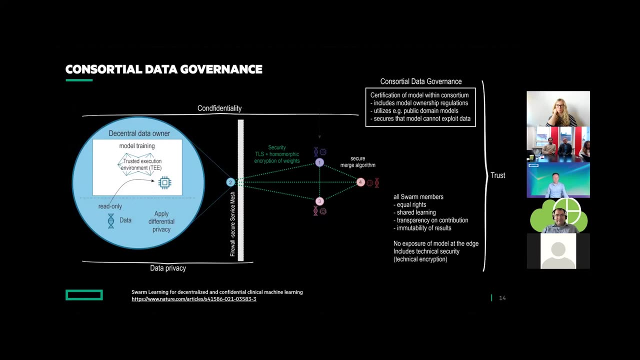 you have whatever a failure in the communication between those nodes throughout the training. actually, it picks up from the other nodes the results which are then on the overall scheme. Now I come to a point which pretty much reflects also what Dimitar was already mentioning. It's the combination of different notions. 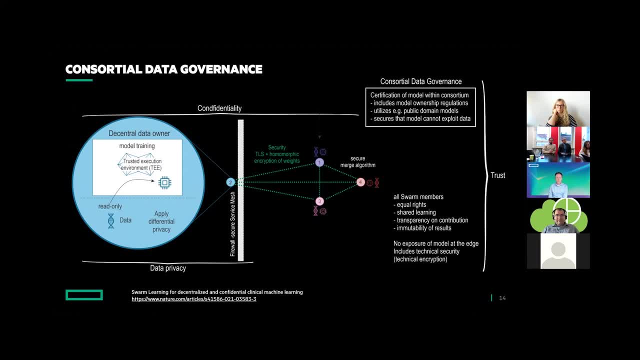 So we have also here the data at rest, data in transit and data in use. So it's a combination from blockchain technology or it's a distributed ledger technology, what we deploy here, which is then doing the immutability of the results on this transaction log. 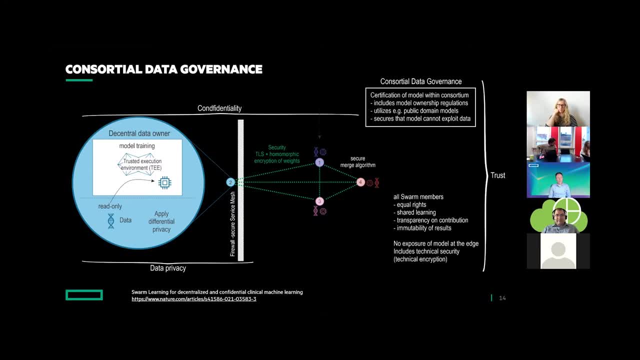 This has one notion: that in this blockchain you register everything and everybody can then look into that. So we have the transparency of the contribution of all the parties. So if there is a malicious party who is acting malicious in this respect, then we can identify this. 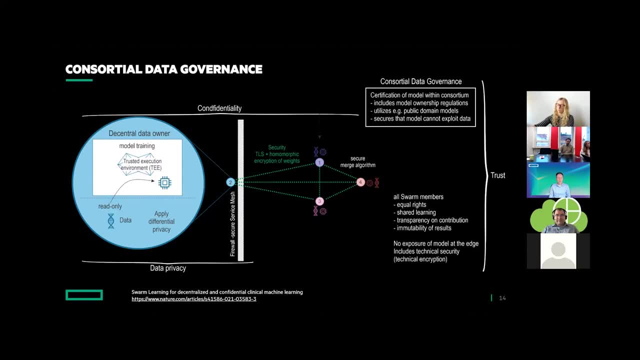 And this is one base for this very much important analysis we're talking about now in this workshop and very important notion of how do we actually enable trust, Because trust cannot be generated, It is only earned, And all the parties must work together if they want to work together and trust each other. 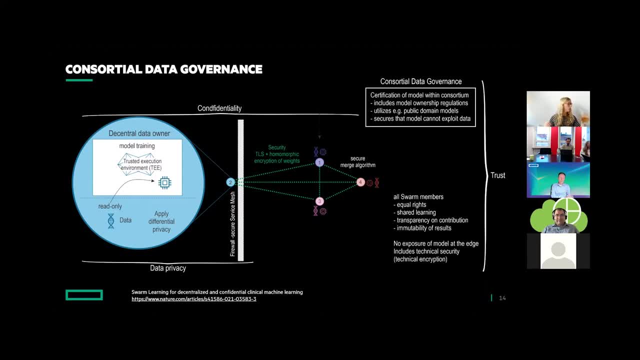 So, from a pipeline perspective, as I said before, we move the de-identification to the data owner. We learn on a read-only data point where the data is not going to be then moved out of the ownership and the controllership of the data. 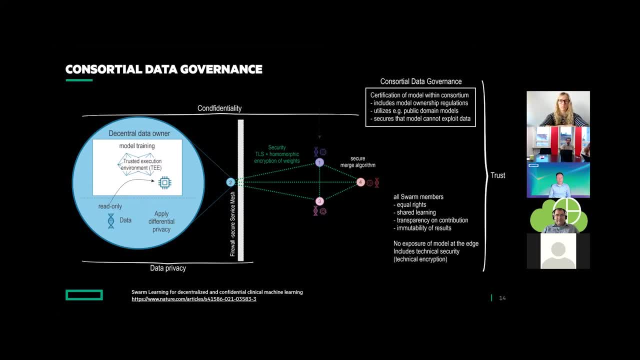 owner on the left side, A differential privacy. this noise we were just talking about can be applied locally. We have also a trusted execution environment which is locally, And then only through the attestation of access to such a data. So we have a very specific node. 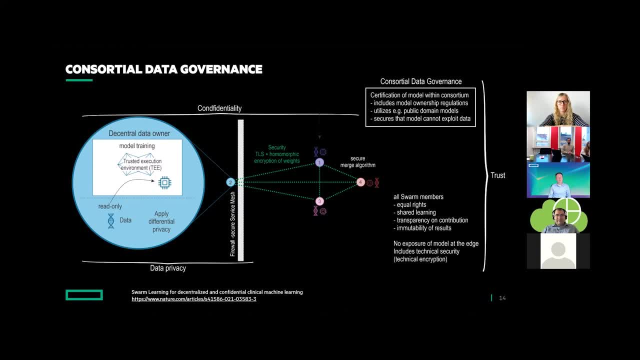 As you see here, it's one, two, three and four. This network of nodes have then also a homomorphic encryption of the weights within the distributed ledger. We explicitly don't use a public ledger, but explicitly use a private, permissioned ledger. 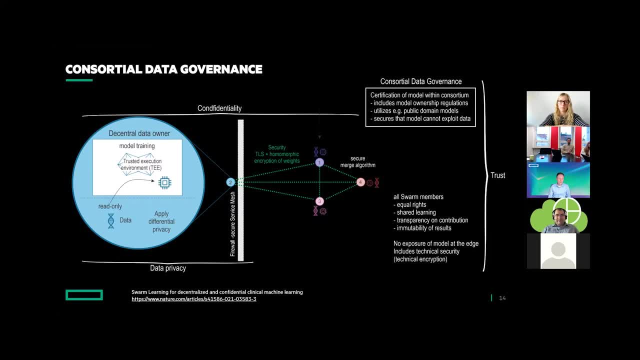 because we say, or we must actually make sure that we are not or are sustainable here. And this is optimal because, as you know, public ledgers from a consensus perspective is much suboptimal And as we need to have a consortia between those parties. 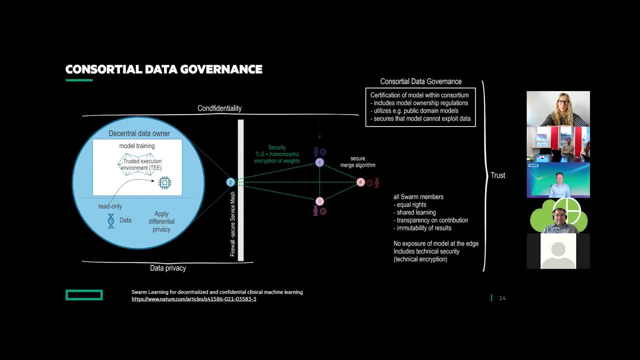 working together, which is basically again a swarm working together on a common goal. we have this notion of this collaboration based on contracts and persistent on a trusted ledger. So there's another topic, of course, of course, which is the model by itself which needs to be trusted, So not only the data which 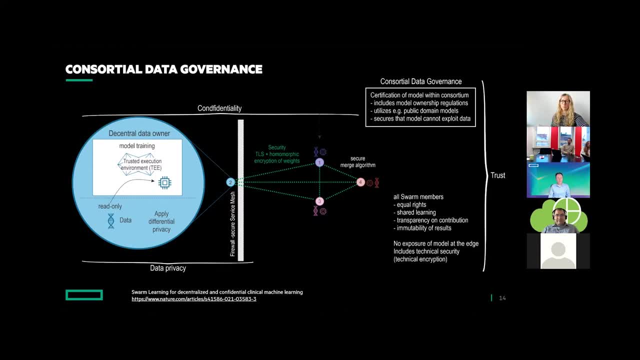 is fed into such a model needs to be trusted, but the model needs to be trusted as well by the parties that this cannot be inversively attacking the data and exploiting the data. So there must be a certain governance around it, which then also includes the ownership and regulations around it. 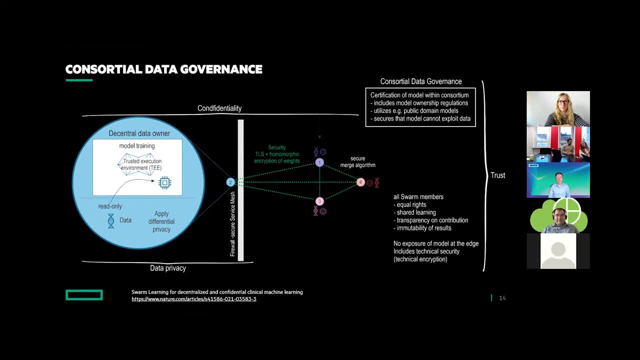 for the model by itself. So this is this notion of consortial data governance and model governance, which is then above. So the combination of those is what brings this. We have this also in our paper based on nature. Interestingly enough, there were different groups now looking into that and 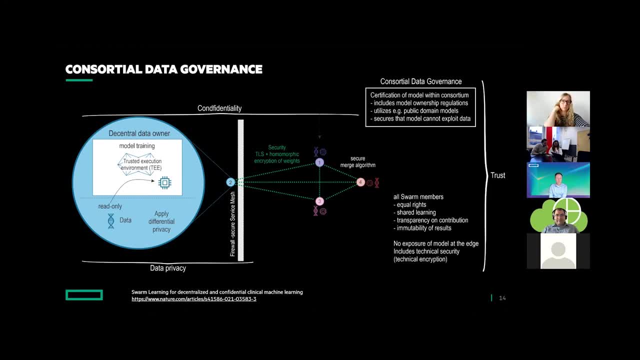 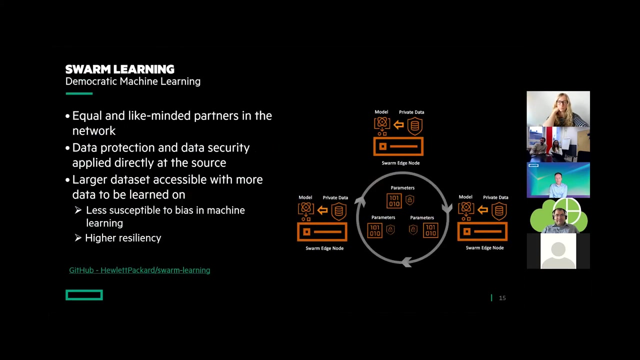 on histological data, they could see exactly the same results. So a central model has no improvement over a federated or swarm learning model as it is here, And the abstraction is then really on the model which is using standard machine learning libraries like TensorFlow or PyTorch or Keras. So what does it mean? Moving data, leaving raw data? 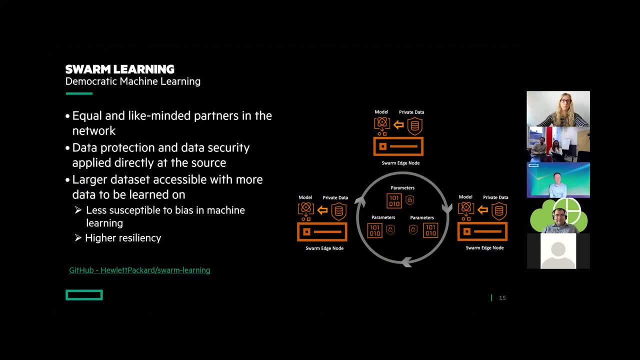 at the edge where the data is generated. have a like-minded partner network and leave the data protection and the data security at the source, getting larger data sets and less susceptible to bias in machine learning, while having a higher resiliency. moving out training partners or getting in training partners. 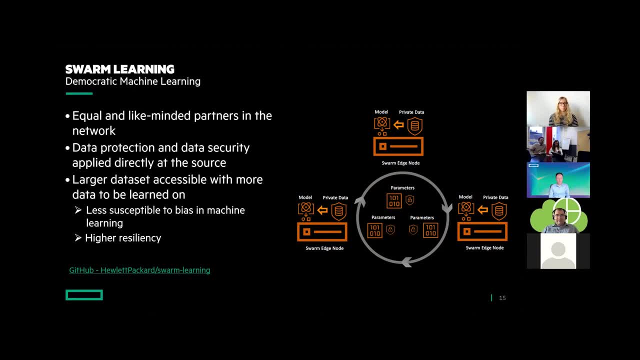 We also have this as a trial version, as an open version, so that everybody can apply it. It's also containerized on a zero trust elements so that we do attestations all over the place when getting these parties together. We, as HP, we don't deliver the model as such, because we believe that the model must be a domain. 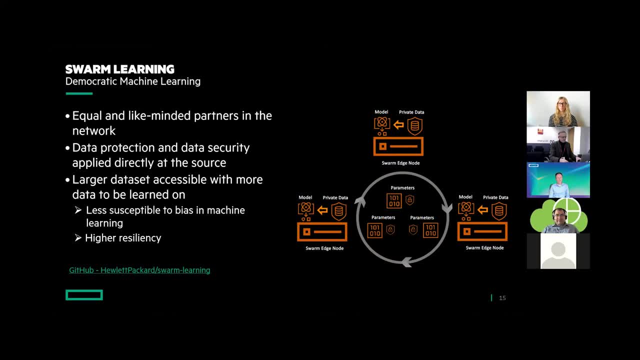 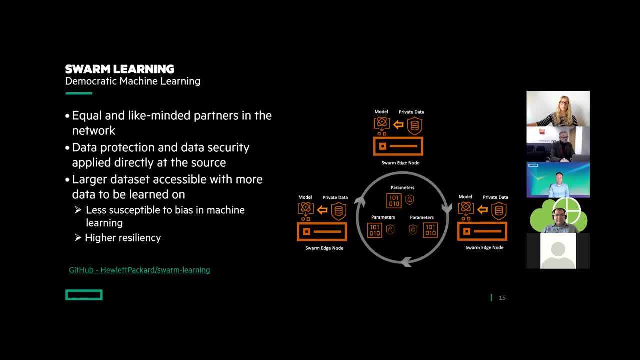 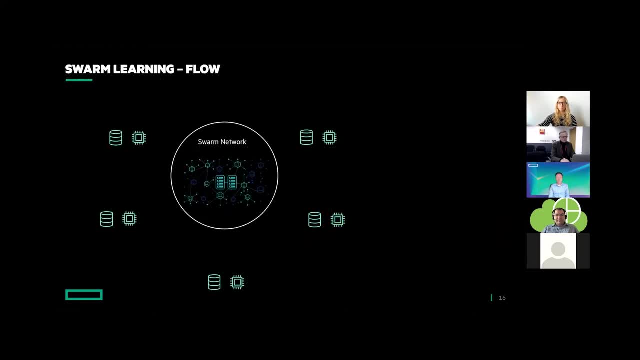 party can collaboratively work together. I have one slide on just how to show you how it actually works. So basically, you have a registration in a swarm from the models. you do a training, all the nodes do the training, they get their weights. 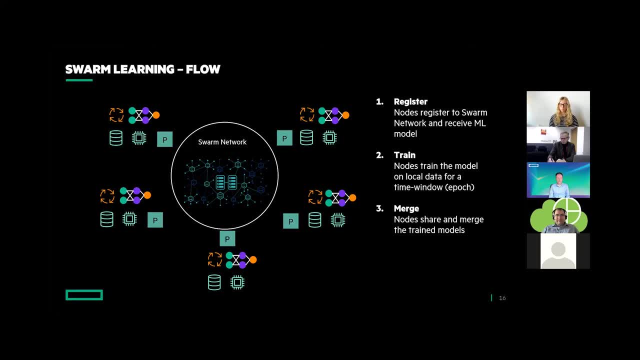 And then the aggregation of the weights throughout a single epoch is done at a certain node. So even if this nodes fails in the next phase, this training is repeated, but another node is being elected to collect the information. So there is no central server. 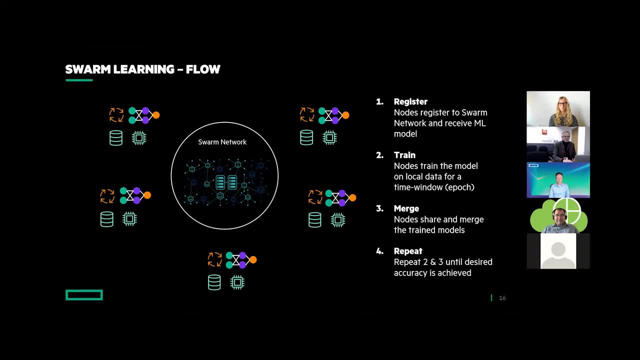 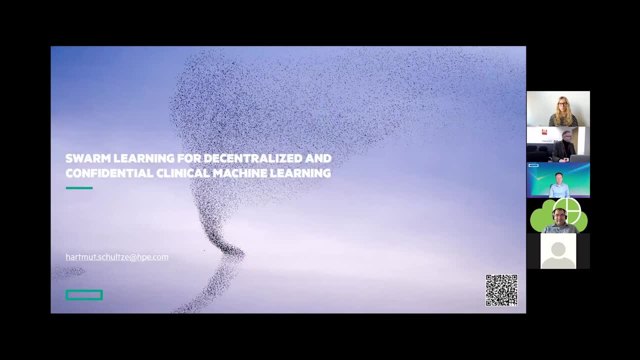 no central party of actually aggregating this throughout the training, And with that I would like to go for any questions you have. Thank you, Mr Harald. So we have many questions on the net? Yes, So shall we. we are now. 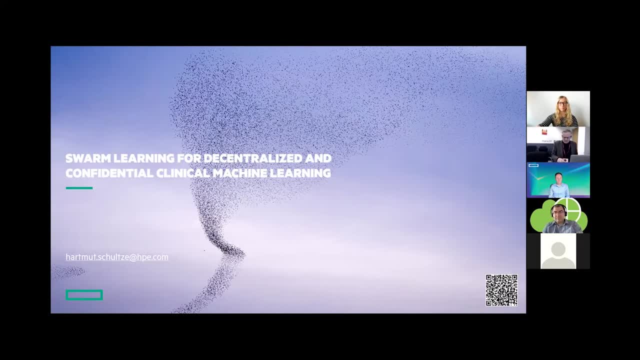 thank you very much, Hartmut, for the presentation, And we have one question from Bo. Thank you, Bo, Harald. here I'm on the steering committee for my data and obviously there we are pushing forward with putting the person in. 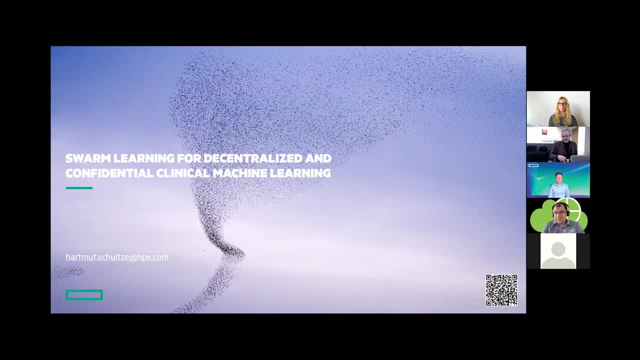 the human in the middle of the process, as GDPR in Europe is also doing, And there we have seen that trust of IP and SSI has been the way to actually make data travel in a safe way. So my question: how much is this supporting self-sovereign identity? 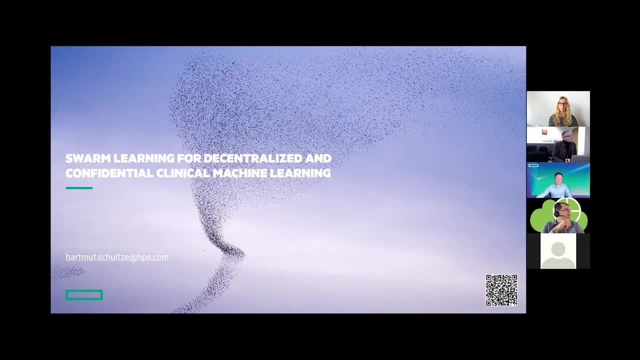 And how much are you participating in that work in trust of IP? thank you, Yeah, well, self-sovereign identities- uh, you're mentioning the the gaia x notion. that is one base to that, since the attestation of the collaborative parties should always work on the identities of such such ssis. so the attestation. 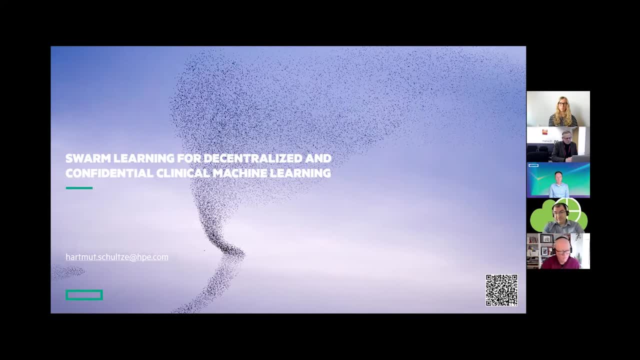 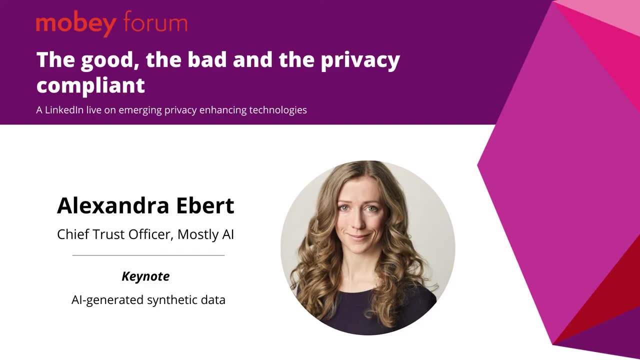 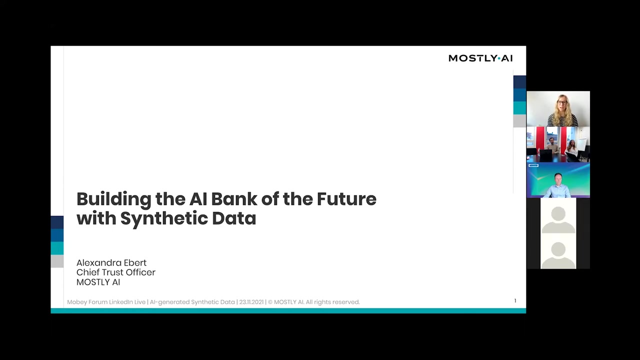 and the policy around who contributes to such a network is, then, a consumption of such a identity. so i'm alexandra ebert. i'm alexandra ebert, chief trust officer at the synthetic data company, mostly ai, and today i will talk about ai generated synthetic data and how it helps particularly with building the ai bank of the future. why ai bank of? 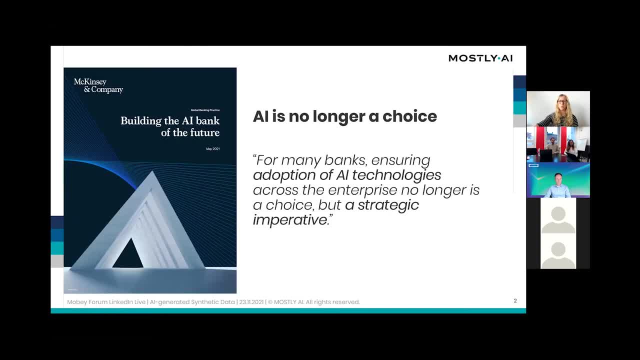 the future. sorry, my slides don't move as intended. now they do. mckinsey and basically any other consulting firm, professional services firm, is telling you there won't be a future for banking without ai. for example, from a recent report from this year they said ai is no longer choice, but it's. 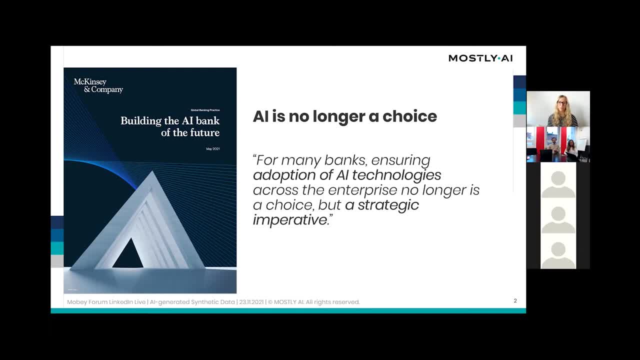 a strategic imperative to really ensure adoption of ai technologies across the enterprise. some of the reasons listed in this report are the increasing competitiveness in the landscape, with big tech players entering with innovative startups and then, of course, also changing customer expectations. one of the most important ones is that personalization really is key and that 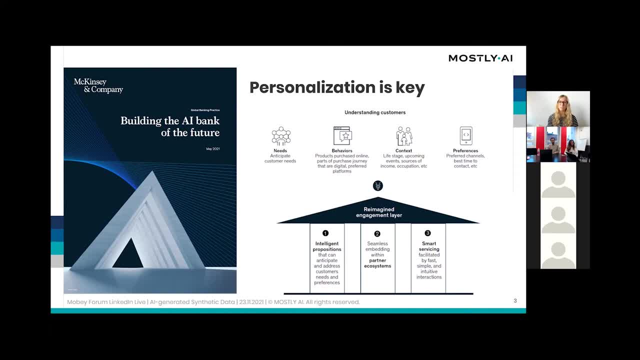 customers nowadays expect highly personalized services, so that you really switch from product centricity to customer centricity. and that's why ai is so important, because it's really important to make sure that your customers understand what you're offering and what you're offering to them. 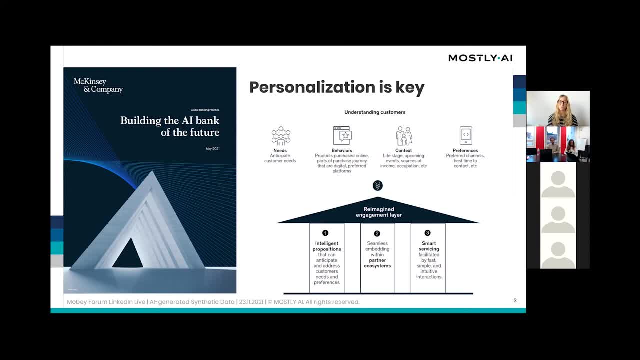 and that's why ai is so important, because it's really important to make sure that your customers understand what you're offering to them. so customers don't want, of course, the email that notifies them about a fancy new service offering, but they really want to be offered and 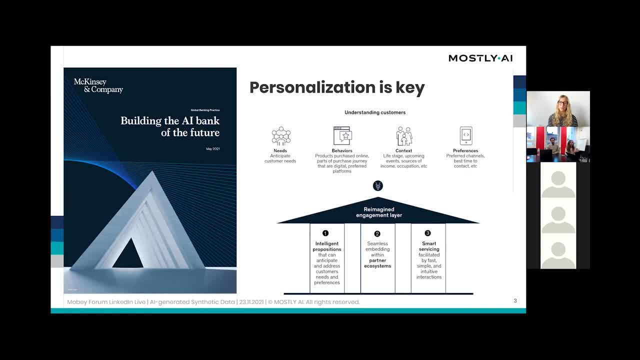 exposed to this offering right at the relevant point in time when they really could need this service. so this really means that, as an organization, you have to become in a position where you granularly understand the behavior of your customers, which, of course, requires access to data- and not only their behavior, but also. 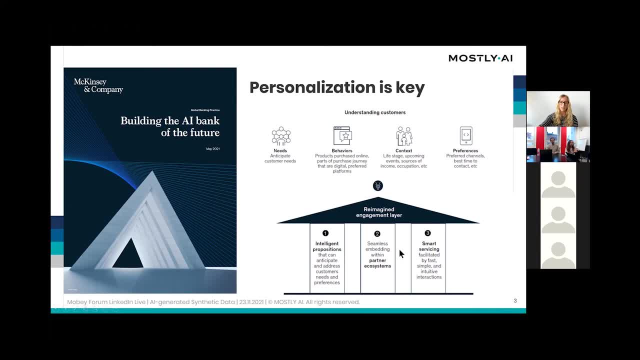 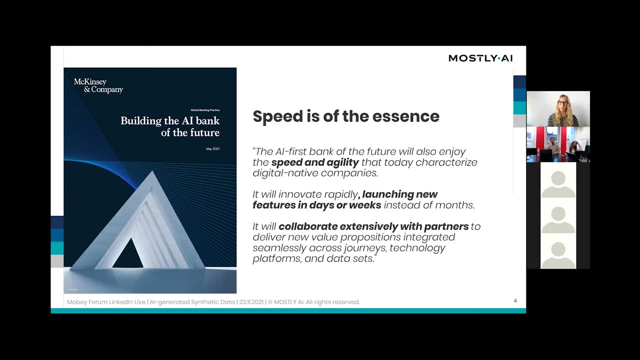 their context, and this then, of course, can lead to different intelligence propositions, but also collaboration with partner ecosystems, which is one of the other key pillars that's kind of in the future outlined by mckinsey. but also speed will become crucially important, because not only is it about speed and agility and being in a position where you can launch new features, 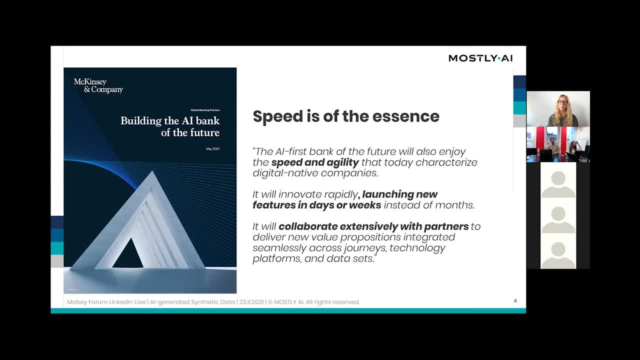 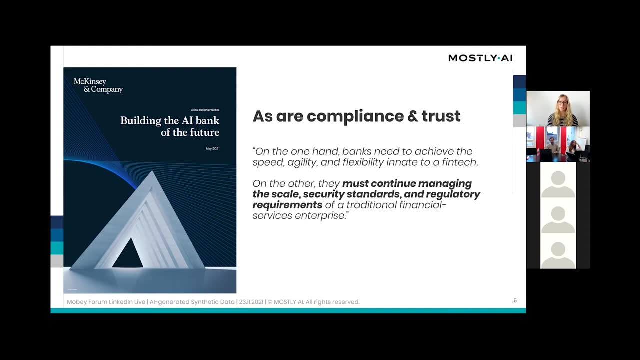 in days or weeks as opposed to months. you should also be in a position where you're able to collaborate extensively with existing partners, which again requires nowadays that you can share data. yet compliance and trust are still essential for financial institutions. we've already heard this: banking is a business of trust, and despite all the speed that's required, of course, 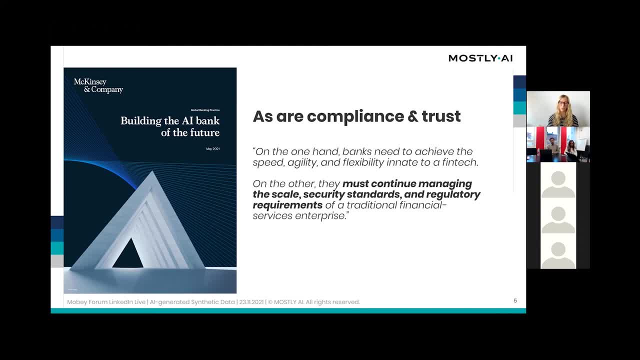 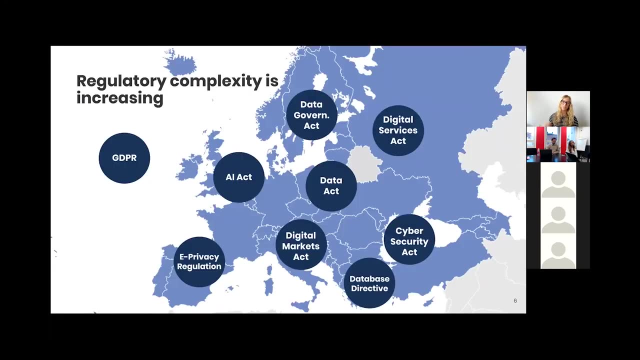 financial institutions can't afford not to comply with all the regulations that they have to comply with or to risk the trust that the customers have put in them for the last century. so for banks it's definitely a quite challenging environment nowadays. nowadays, and especially when we talk about regulations, we can see that regulatory complexity is increasing. i'm sure 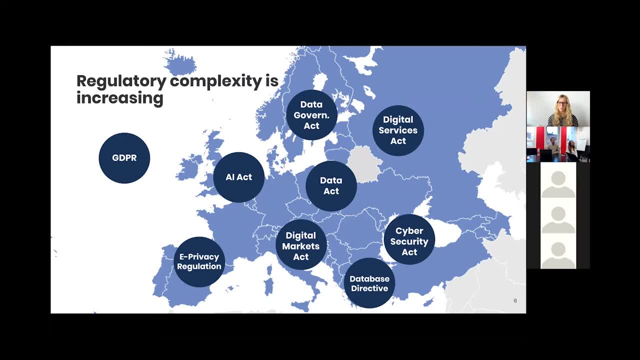 everybody's familiar with gdpr on the upper left. please excuse russia and britain here in my map of the eu. i was a little bit in a hurry when preparing the slides but in general the majority of circles you can see here are drafts of upcoming regulations which really show that working with data will. 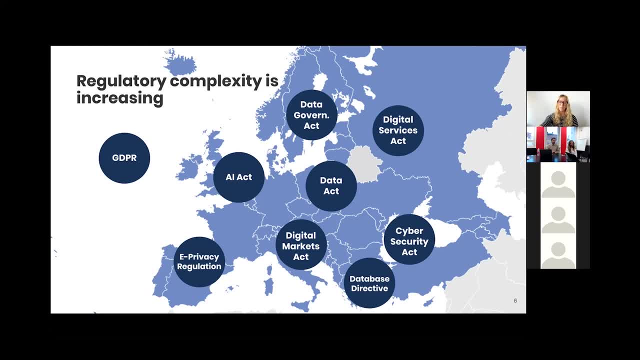 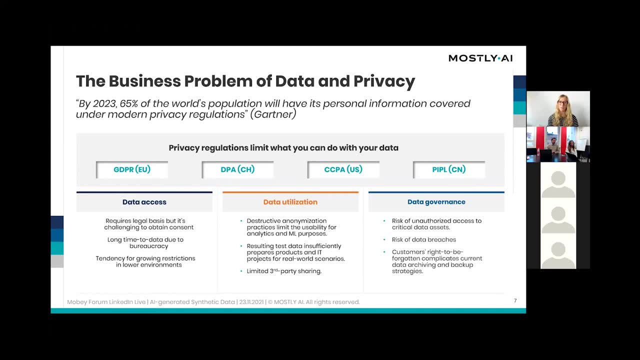 become even more complex than it already is, and that's what's the consequence of this. the consequence of this is that, as amy already pointed out in the introduction, privacy can be one of the major roadblocks for you to innovate with data and to build new services and product. 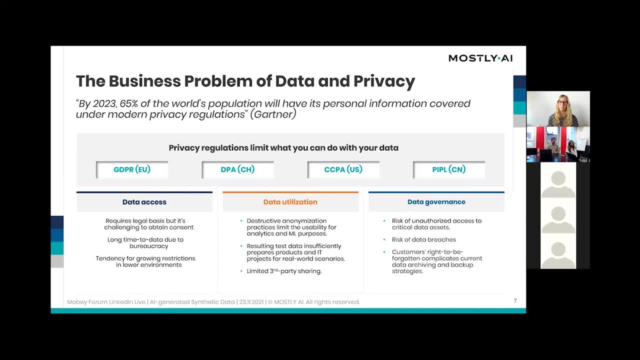 offerings. gardner predicts that already in two years, 65 percent of the data of world's population will be covered by modern privacy regulations, and it's not only gdpr, it's really also ccpa. china just recently introduced the privacy regulation, so it's getting more and more complex, not only in the eu, but also on a global perspective. what are the? 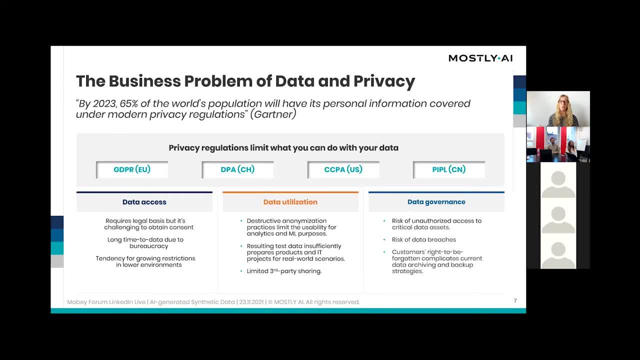 concrete challenges that we have due to these regulations. the first one is definitely data access. what we hear from our clients is that most often it takes them many weeks, sometimes even months, until they can access data for internal projects and as soon as they want to share data. 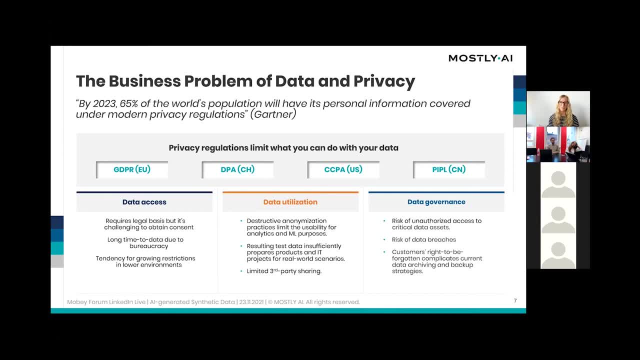 it takes even longer. then, of course, utilization is an issue for them because in the past, especially when it came to data sharing, they used legacy anonymization techniques like masking or obfuscating, which i will come to that in more detail in a few seconds- really limit the utility. 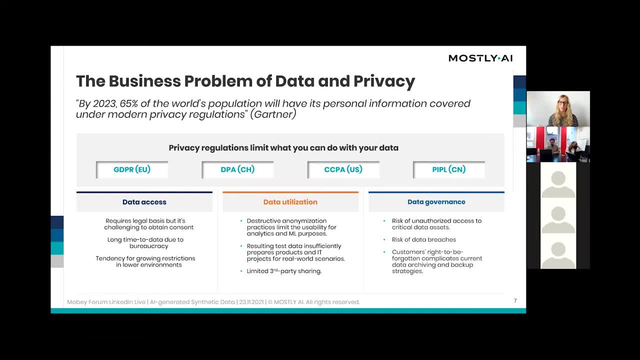 of a data set, especially when it comes to ai training and advanced analytics. and then also there are many data governance issues, the risk of unauthorized access, the risk of data breaches and also complicated regulatory requirements to manage, like the right to be forgotten, data retention and so on and so forth, and 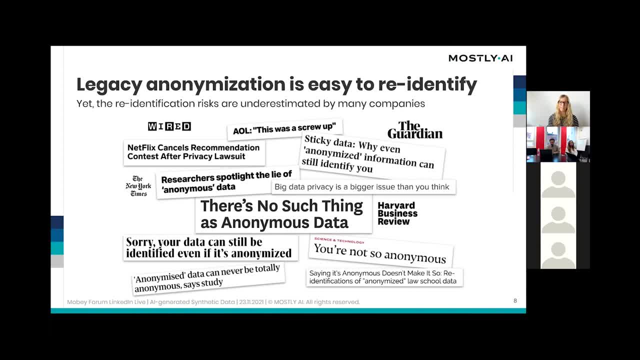 i already briefly talked about it: legacy anonymization. legacy anonymization was one of the way outs for all this regulatory complexity because, as we all know, anonymous data is exempt from the gdpr and other privacy regulations. the problems with legacy anonymization- so we already heard it in one of the earlier talks- is that it really doesn't work anymore for large data sets. 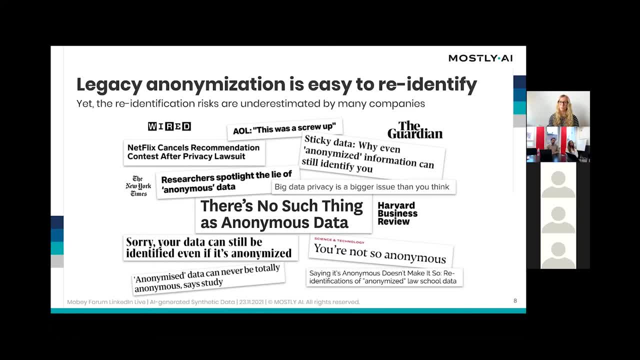 so there's a huge body of research out there that highlights that with these legacy anonymization techniques like masking or obfuscating, it's impossible to prevent the data to be re-identified, and therefore we've seen, on the one hand, a few nice headlines on these papers, but also from a 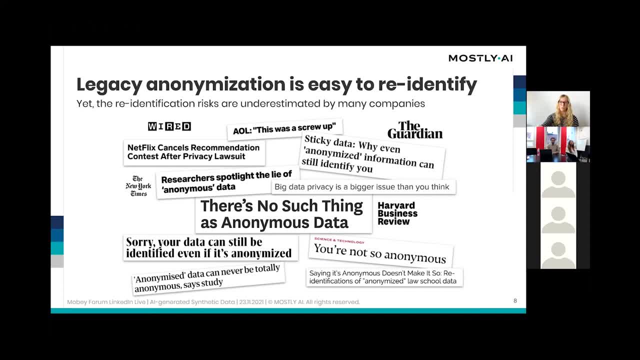 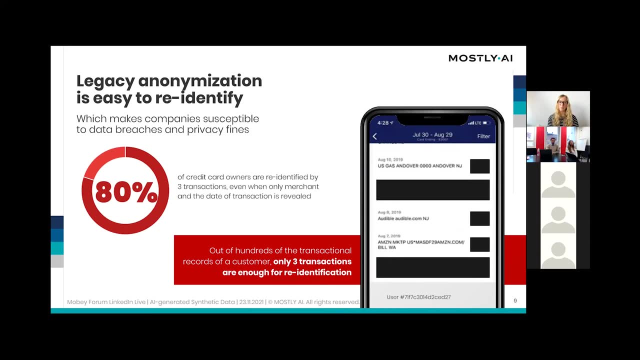 few companies that thought, okay, what they shared was anonymous, to then find out it in fact wasn't, and having to deal with privacy fines, regulatory and reputational damage. so this is definitely a prominent problem when it comes to legacy anonymization. to give you an example, one study: 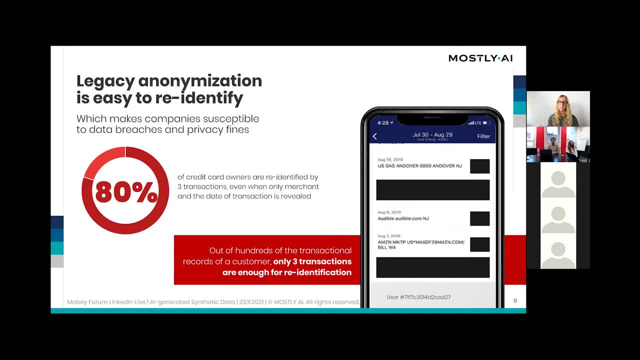 for example, showed that 80 of credit card owners could be re-identified by only three transactions and if you think about the amount of transactions that each customer takes over the course of a year, three transaction- the first place is not a lot of utility that you can preserve, and it wasn't even. 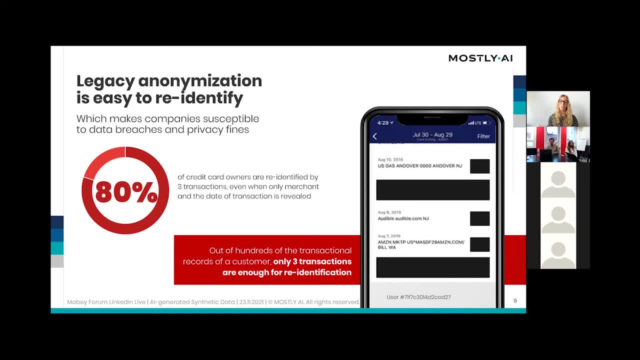 the full transaction and all data points from these transactions. it was only the information about the merchant and the date of the transaction, and these tiny pieces of information were sufficient to identify over 80 percent of customers, which really shows legacy. anonymization does not only help to protect. 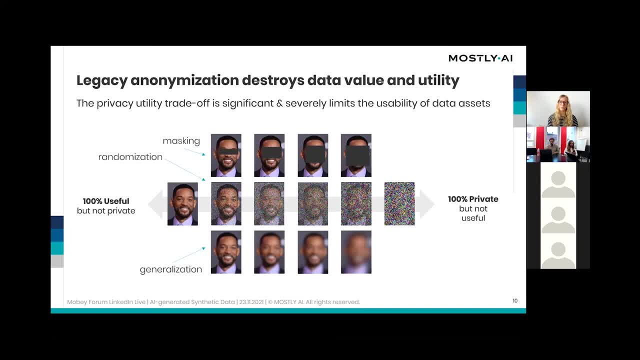 privacy or does not help to protect privacy. it also destroys all the utility in your data set, and a quite nice graphic to illustrate it here with different techniques is that you can see the privacy and utility trade-off. on the left side we have 100 percent useful data everybody will. 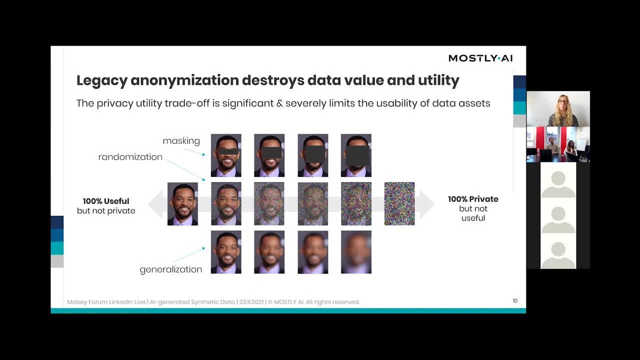 know that this is will smith, but of course it's not private, it's not protecting his identity. on the very right end we see 100 percent private data, super gdpr compliant, free to share, sadly not useful and anything in between: maybe um makes the day or definitely makes the data less useful. 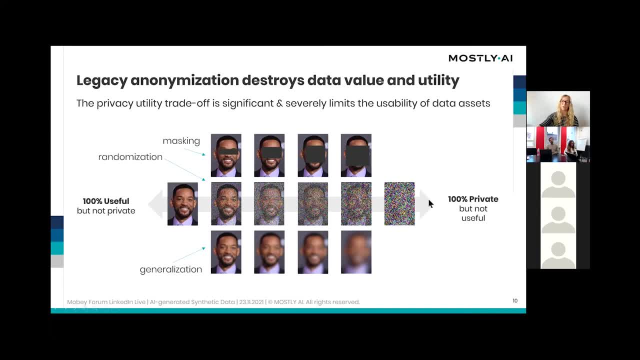 but, as the studies showed, doesn't protect the privacy. so only if you're somewhere here you can say, okay, i protected the privacy, but you can't do anything with this legacy immunization anymore. and to illustrate this maybe in a plot, we can see that we have this growing gap for innovation. 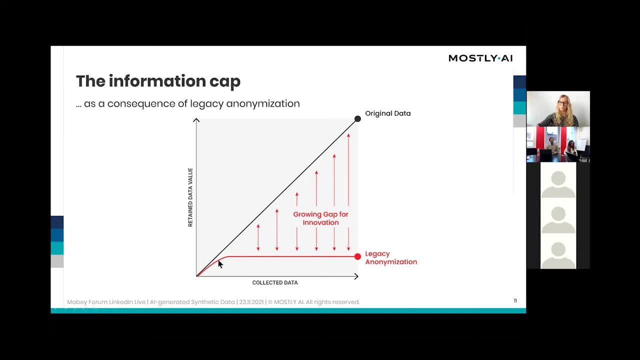 because we have more and more data nowadays compared to maybe the last 10, 20 or whatever years ago. but with legacy anonymization techniques there's always this hard cap, the ceiling that you can't retain more than just a tiny piece or a very few data points before you run the risk into the 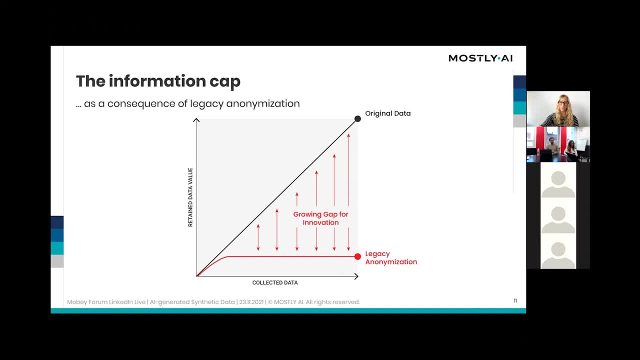 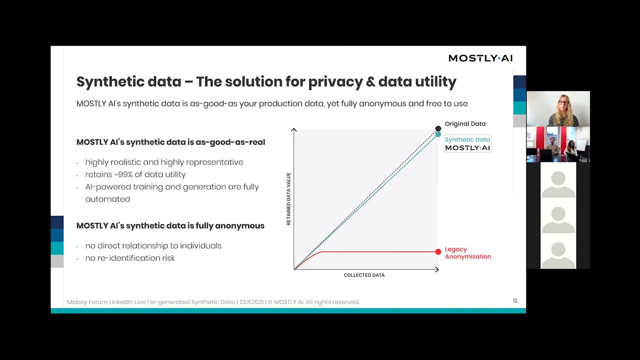 risk of re-identification and- this is the introduction- how synthetic data can help you come overcome this regulatory complexity and being able to innovate in a way that's privacy preserving and gdpr compliant. synthetic data, on the one hand, is data that's nearly as good as the real data, but it's still fully anonymous, so you get much, much closer to. 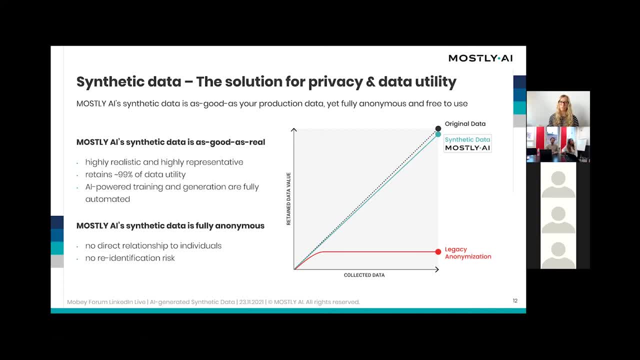 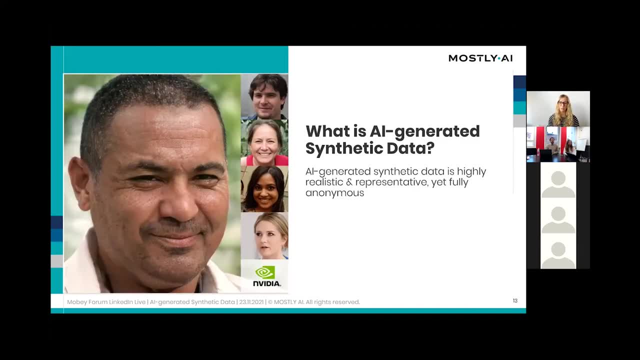 the original data, yet you protect the privacy of your customers. it's quite easy to understand if you look into pictures. the pictures you see here on the left are from an nvidia research project and they did back then was they trained an algorithm on hundreds thousands of human pictures up under? 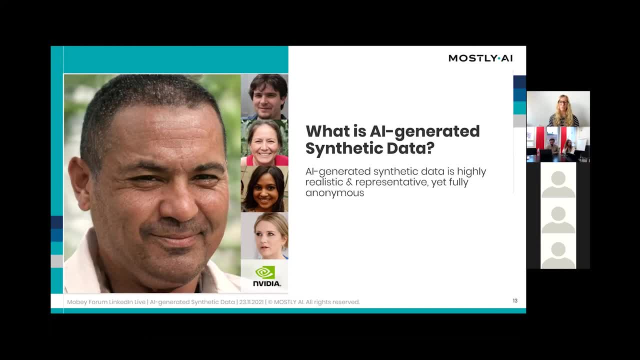 the point where the algorithm understood how a human face looked like that. humans have, i don't know, two eyes, one nose, one mouse. the eyes are roughly located in the middle of the head. it really understood how a face is constructed and once this training was completed, you could generate: 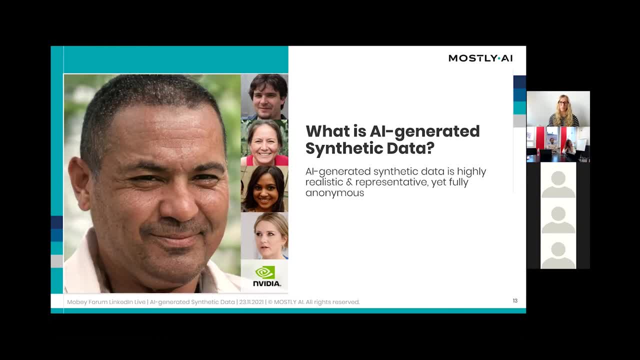 new synthetic photos of humans from scratch and these are the results that you can see here. so i would say everybody would agree with me that this is a very important part of the research and this is the first step into the study. so i think it's important to make sure that everybody 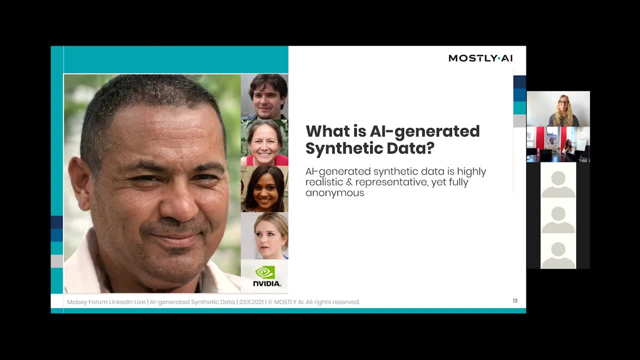 would agree that these are highly realistic photos and everybody would expect them to be real photos, but in fact, the people here have never existed before. they're synthetic faces, and the approach to anonymization when it comes to synthetic data is so sophisticated that you're not just shuffling. 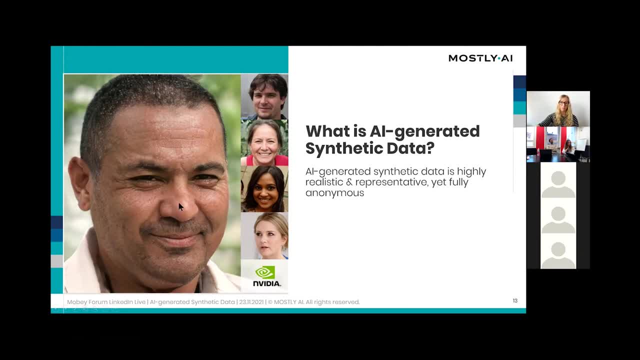 around some parts of the data. so it's not that, for example, the algorithm saw one training image with this type of nose and took then the eyes from another training image and the mouse from another together, but it's really just learning the logics, the statistics, the rules behind human faces in 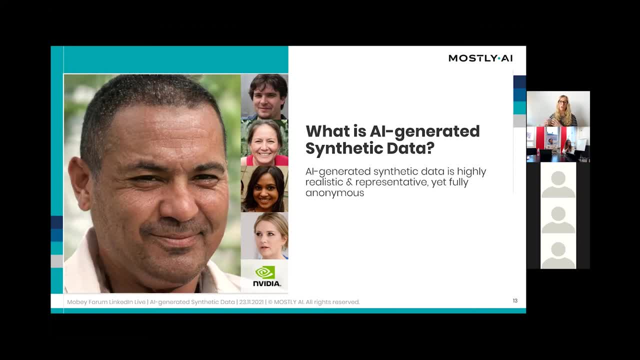 that example and then use this information to construct completely new data points, completely new images from scratch that don't have any one-to-one relation to real humans. And this is what we at Mostly AI do, but not for unstructured data like images or videos, but really for. 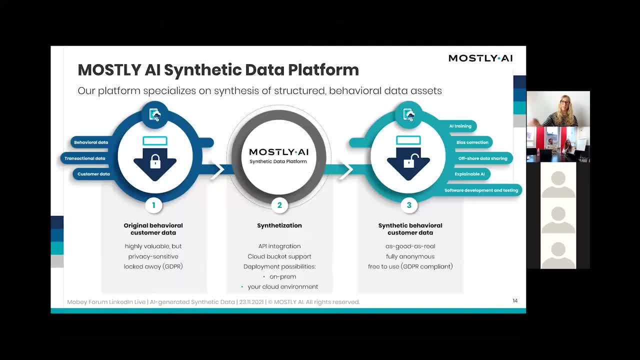 structured business data. So think of your customer databases, your financial transactions. How does this process work? We provide our software to our clients, so we, as a company, never get access to any sensitive customer data, and they use it internally to synthesize their data. 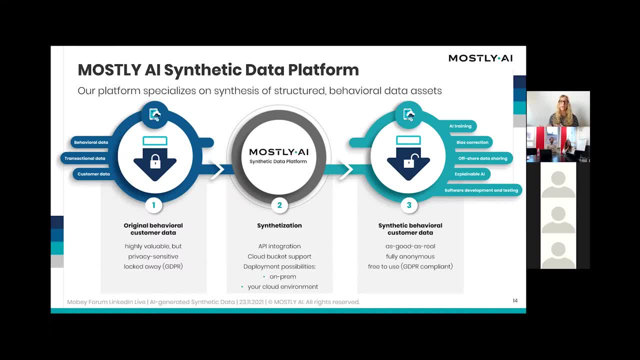 assets by selecting the data that they want to synthesize and then automatically, a deep learning algorithm learns all the patterns, all the structures, all the correlations, all the time dependencies in the data. To say it's simple, it understands how your customers think, act and 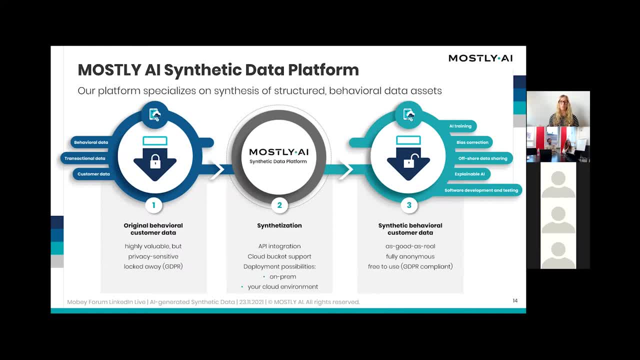 behave. And up until this point, when the training is completed, or once this training is completed, you can generate an unlimited number of new synthetic customers that have all the same statistical distributions, correlations, time dependencies, behaviors, just as your original customers have, But the benefit is that they're. 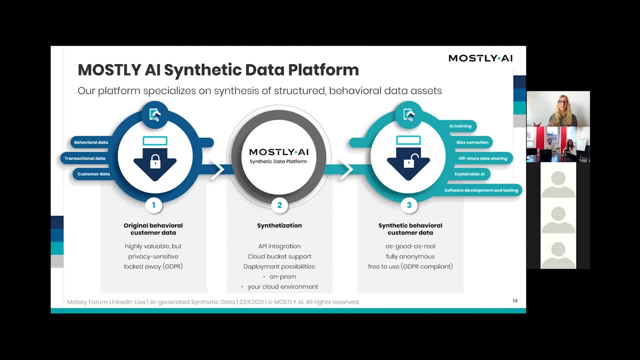 created completely from scratch and that you don't have any real customer data in there. so you're out of scope from GDPR, but still retain the utility of your data set. To give you a few examples: with some of our financial clients we saw, for example, that still all the ratios of how the customer basis 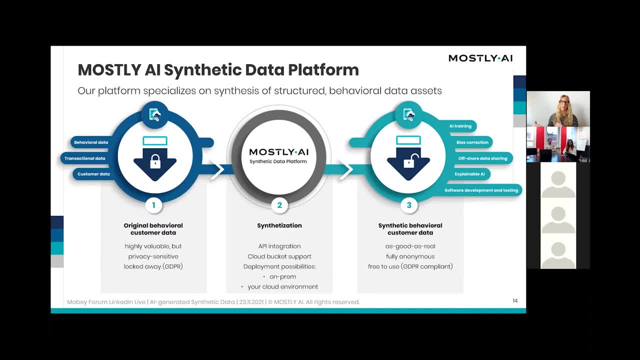 looked like were retained, but really to a very granular level. So even behaviors like I don't know the old granny going to the cash machine just once per month but always retrieving the maximum amount of cash, was preserved, as well as, for example, that 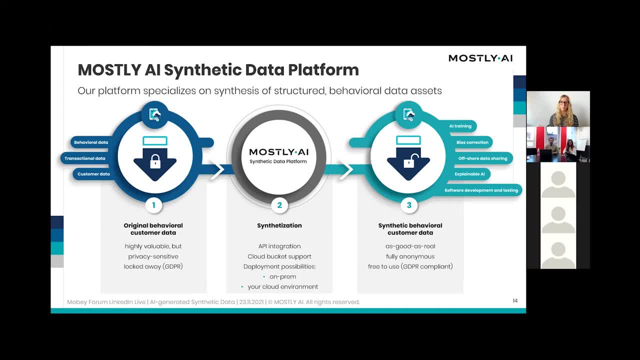 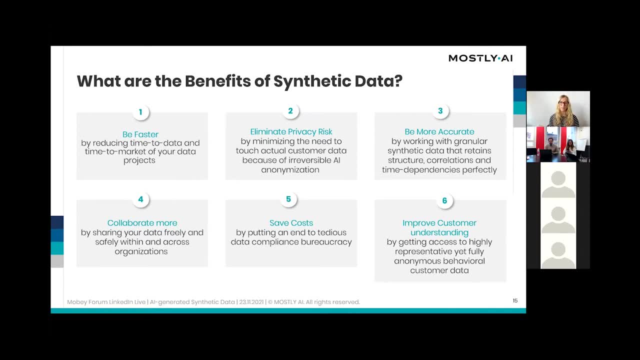 different age groups have a significantly different spending behavior and financial behavior. So what, concretely, are the benefits of using synthetic data as opposed to legacy anonymization? On the one hand, you're significantly faster and can get to data much, much faster. I can come to. 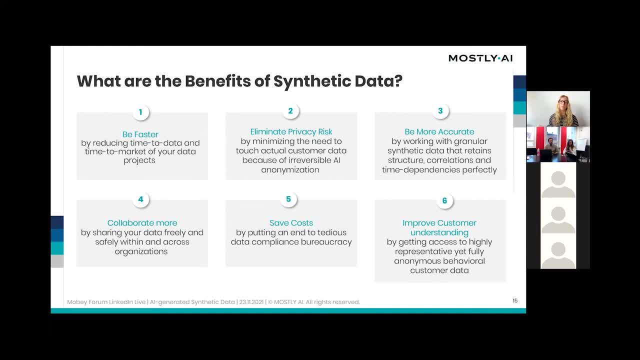 this. we'll come to this later, also with the use cases, But up until now, legacy anonymization was always a case-by-case basis. So what we heard from many of our clients was that these data access requests really took months, whether it was negotiation between the different parties. 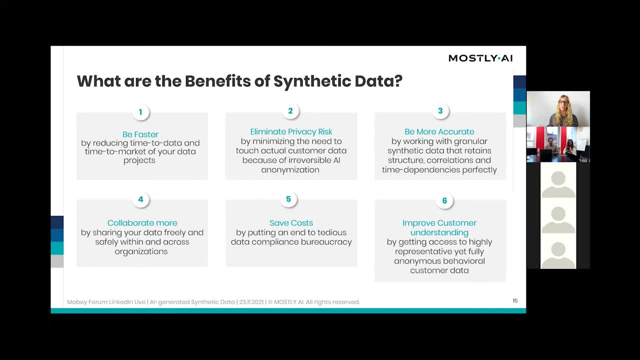 privacy department, DPOs and so on and so forth, And so you know, there's a lot of things that you can do to make sure that you're not just using the same data, but you're using the same data and you're using the same data, And so, of course, whether they really need all the data that they. 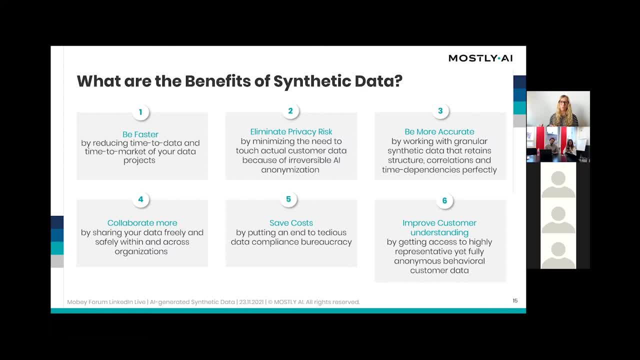 requested or could maybe make do also with little data and less data that they actually requested. And once they finally got the approval, the data was legacy anonymized on a manual or on a case-by-case basis, manually, which again added a few hours, weeks or sometimes even longer. 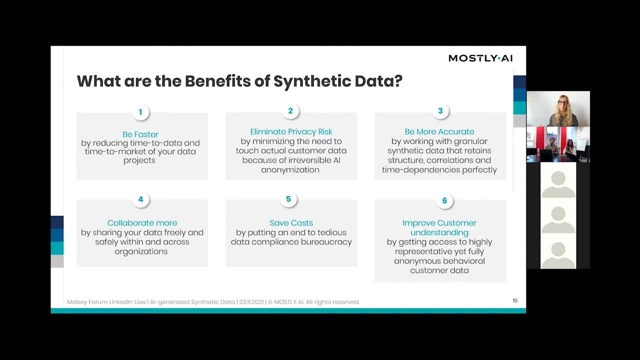 to the already very stretched time budget. So oftentimes it was really three months, six months that the department received the data that they needed. With synthetic data, the whole process works automatically. So you don't have to change something for specific data assets, You just 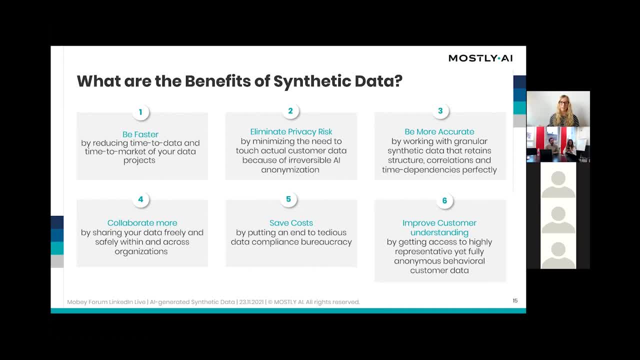 select the data, push it through the system and can get to your data in a matter of hours or days, So significantly faster, which comes back to the speed that was highlighted in the McKinsey report and how important it is going to be forward. Then, of course, you eliminate privacy risks. 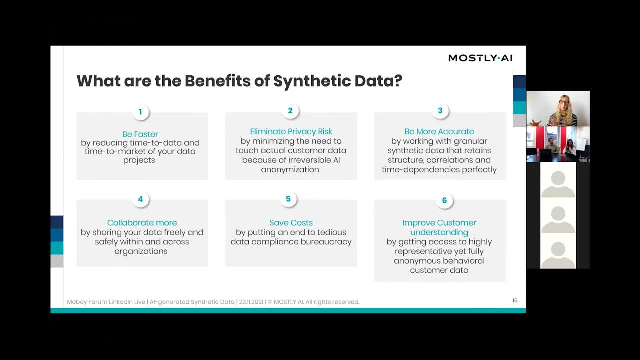 Since synthetic data is artificial data that's generated from scratch, and not original data where you just shuffle a mask or obfuscate some existing points, there is no way to come from the synthetic data back to any real data points of your customers. So you don't have privacy risks through risks of re-identification. Then you can retain much more. 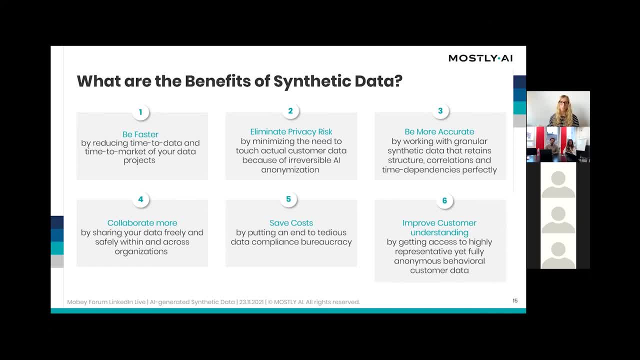 accuracy. We saw it already on the graphic. Usually what we hear from our clients is that we retain approximately 97%, 98%- 99% of accuracy and that even machine learning models they train on synthetic data, but they don't retain much more accuracy. 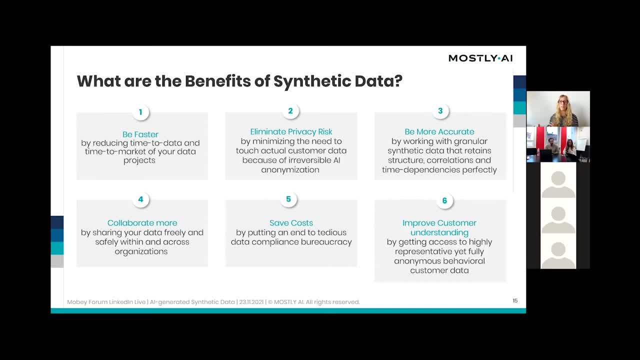 So synthetic data perform as good, sometimes better, sometimes nearly as good- as models trained on original data. One very important aspect of synthetic data is that it's super easy to collaborate on this data. It's not only possible to freely give people access within your company, but also to share data across borders. 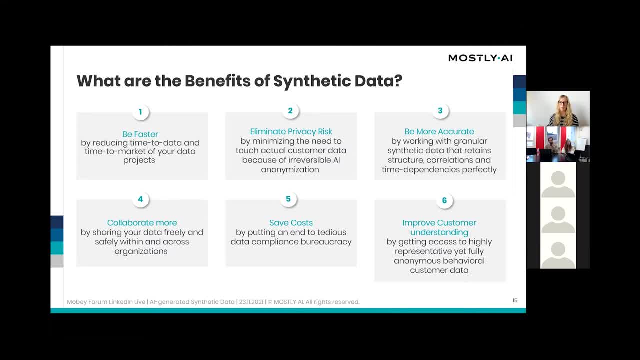 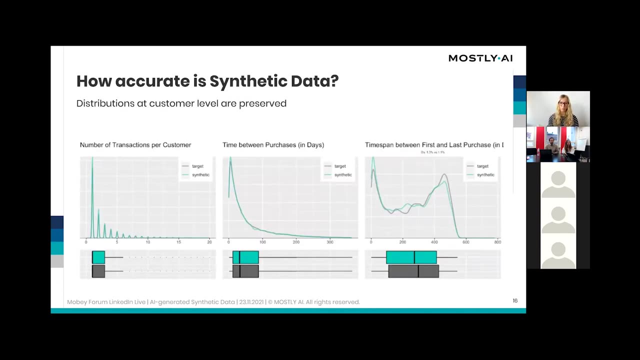 to collaborate with fintechs or with other partner companies, Then you also save lots of costs because much less human involvement in the whole process And since it gives you access to granular data, it's the basis to improve your customer understanding, Especially coming back to the accuracy. I just brought a few slides. 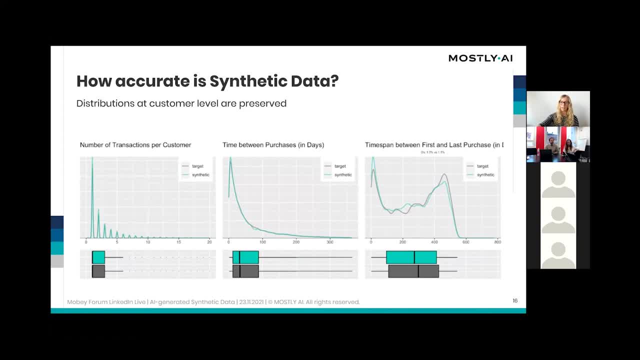 Here you can see that distributions at customer level are preserved, and you can't even see the gray line, which is the original data. You really have highly accurate data that's super granular, both on a global and general level, but also when you zoom into different synthetic individuals. 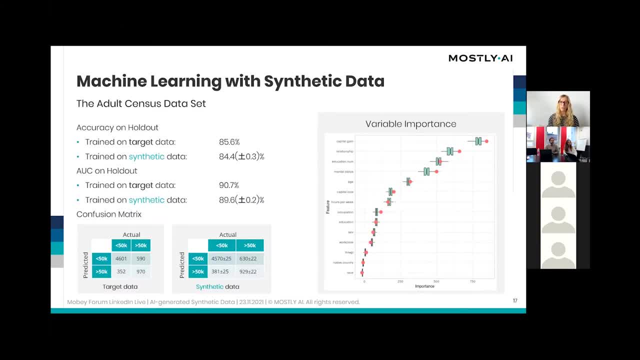 And, as already mentioned, you can use synthetic data to do machine learning on top and you can immediately then deploy the models that you've developed on your production data, because synthetic data has the exact same structure than your original data. So, for all those scenarios where you'd love to have training data available for your machine, 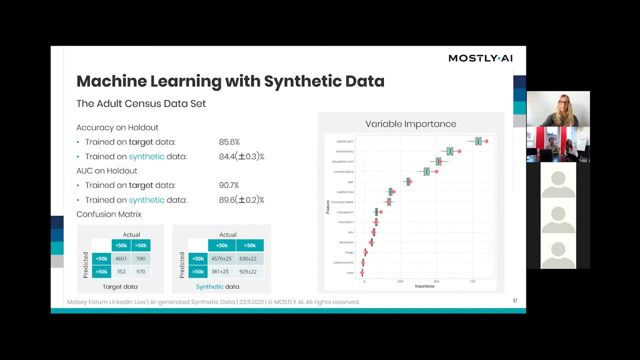 learning, but can't access it due to privacy reasons. synthetic data is your way to go, because it's out of scope from GDPR and can be freely used for AI training. When it comes to the privacy, synthetic data is more and more considered and recommended by. 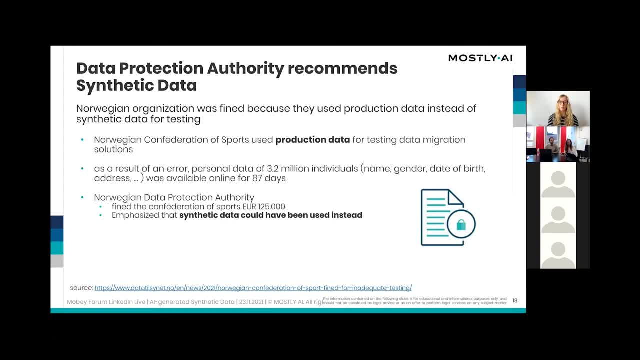 European regulatory bodies as one of the ways to go moving forward. For example, just in June this year, the Norwegian Data Protection Authority issued a fine to an organization that used production data for testing and explicitly mentioned that they could have used synthetic data as an alternative. But there are also many more statements about 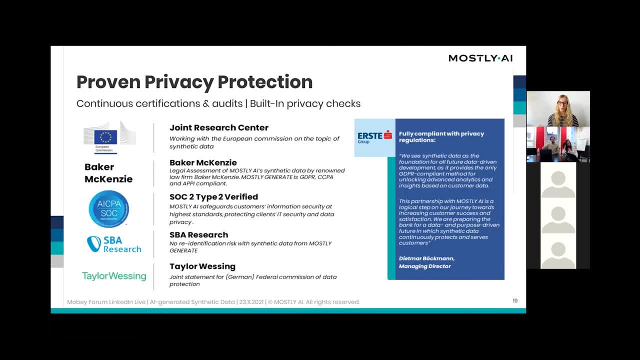 synthetic data. And then, of course, we as a company not only have our internal privacy experts who make sure that synthetic data can't be re-identified, we also work with global leaders, especially on the technical side, but also on the legal side, to really make sure that synthetic 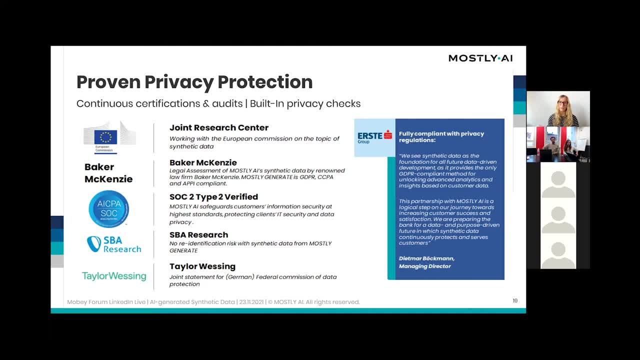 data is as good and as private as GDPR requires it to be, And also our customers. when they do their independent analysis of the technology- like, for example, you can see here Oersted Group- they come to the conclusion that synthetic data is their way out from many of the analytical 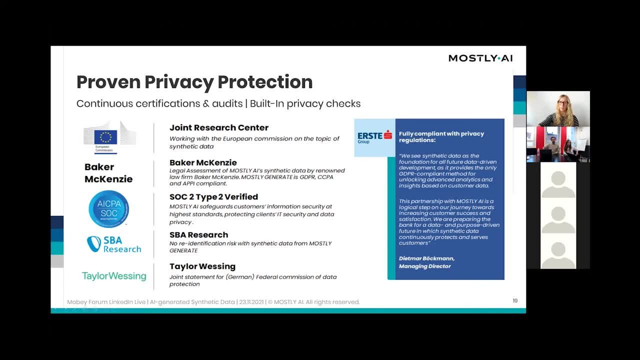 challenges that they have when it comes to privacy. So, for example, here we have Oersted Group saying that they see synthetic data as the foundation of all future data-driven developments, as it provides the only GDPR compliant method for unlocking advanced analytics and insights based on your customer data. So now the use cases that I 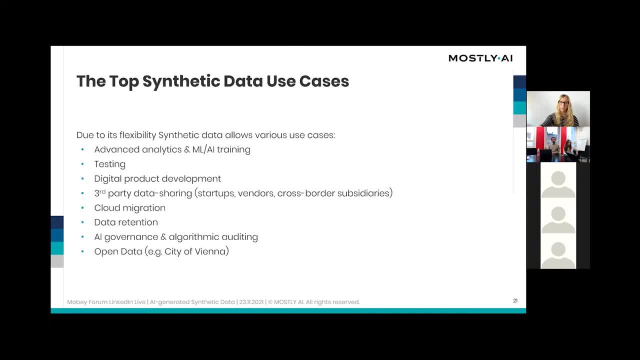 promised. What can you do with synthetic data? I would say the top use cases for synthetic data which we see with our clients are, on the one hand, AI, training and analytics. This is really one of the main application areas of synthetic data nowadays. specifically to the problems I described, 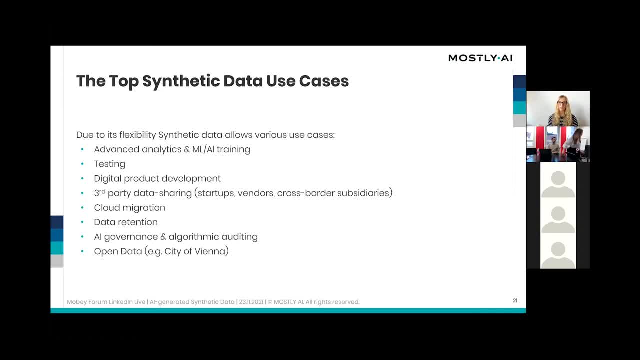 earlier that you need to do So. for example, if you want to do a lot of data processing, you need to have vast amounts of data for AI training, but oftentimes can't access this data due to privacy constraints. Testing is another very promising field, and we just had our new release where we 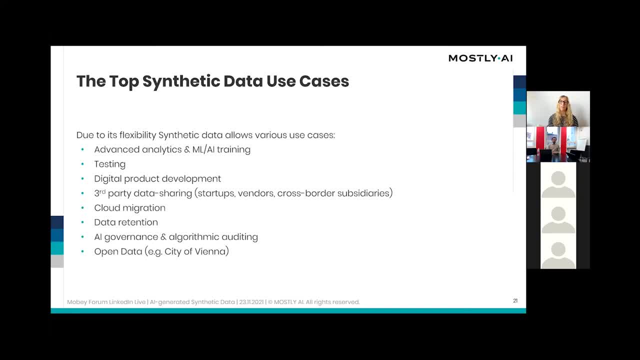 specifically introduced some capabilities that will make synthetic data even more useful for testing, Because with testing you need highly realistic- ideally- production data to test all different scenarios and edge cases. And production data, of course, is something that's not allowed to be used in low environments, So also here. 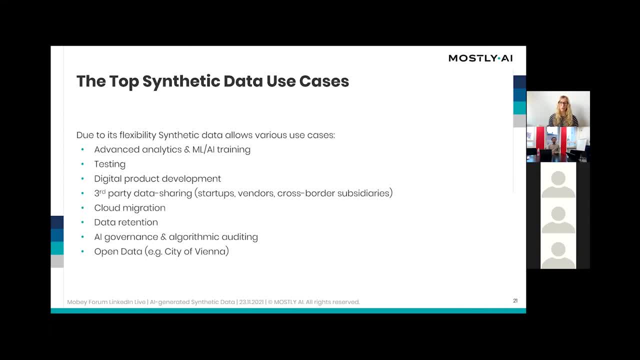 data can work as a drop-in replacement. Then it's for digital product development and also very interesting for data sharing being this cross-border data sharing with different subsidiaries of a bigger group being this to validate vendors, to move into the cloud or to collaborate with startups. I specifically also mentioned cloud migration again. 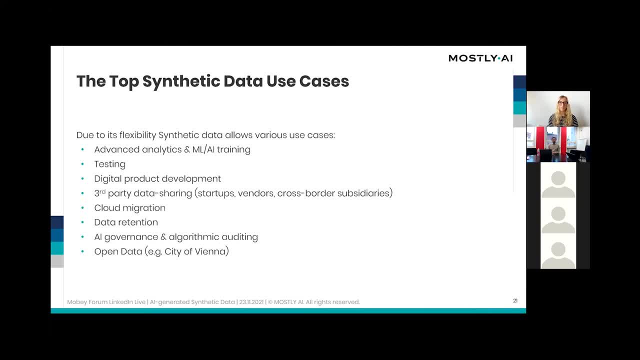 because this was one of the earliest use cases that, for example, a large insurance company, which is a client of ours, used synthetic data for. And then it's also for data retention, Because there are many obligations that require you to delete data at a certain point in time. 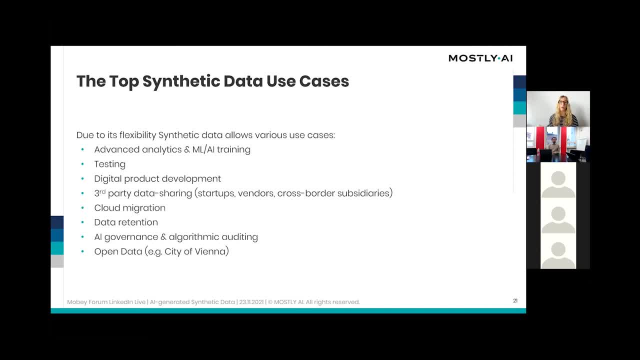 but with synthetic data, you can, in an anonymous form, retain all these insights over a long period of time, which helps to boost the accuracy of your models and also helps in areas of fairness and mitigating biases. AI governance and algorithmic auditing is a more new topic. 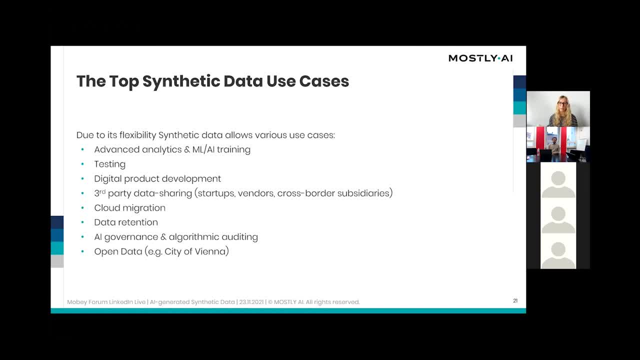 which is becoming more important now with this proposed AI Act in the European Union. And then we also have open data initiatives. For example, the city of Vienna set out to share synthetic data sets with researchers, startups, small and medium enterprises, in an effort to democratize the asset to data. 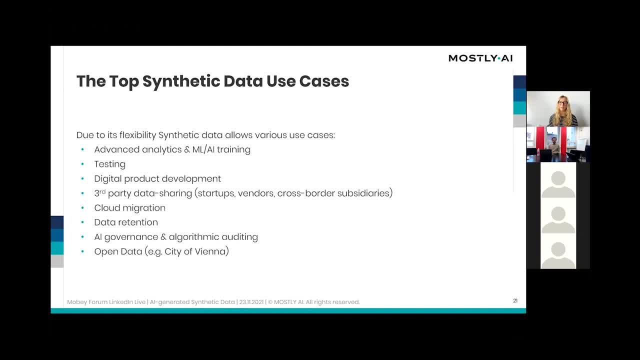 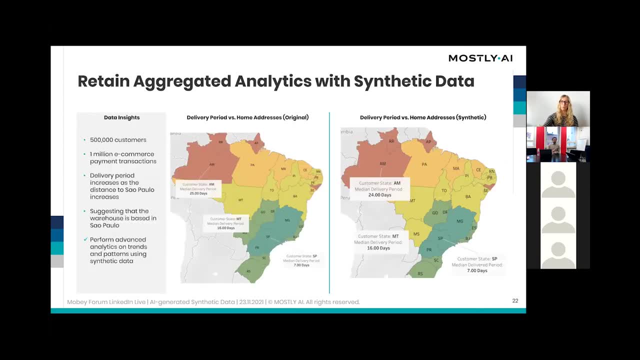 and make it readily available so that also the small players in the field, and not only the big tech companies with vast amounts of data, can innovate. And I have a more concrete use case here for you as well, which is of one of our clients who analyzed 1 million e-commerce payment. 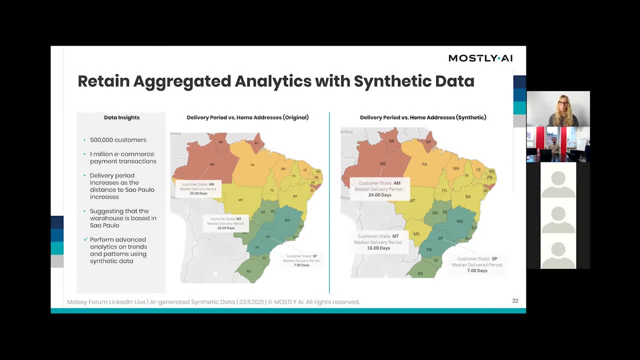 transactions of the client in Brazil and they wanted to use them for advanced analytics and also for testing purposes, And as you can see here that many details of the data set were perfectly retained on a more general statistical distribution level, So, for example, how long the delivery periods were from one area of the country to another area of the country. 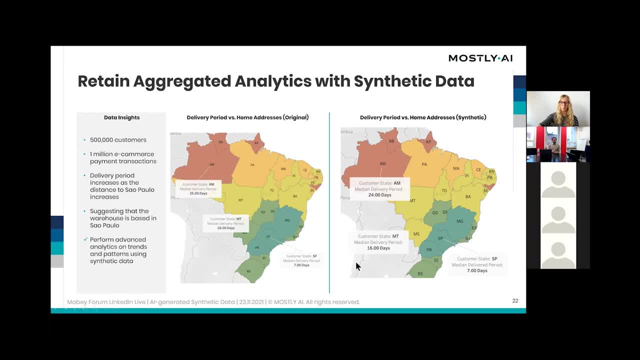 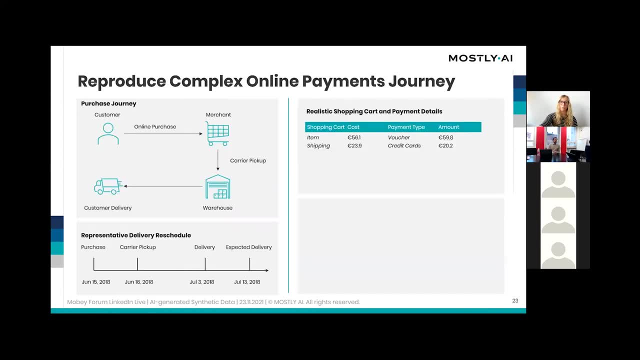 which suggests that the warehouse is somewhere based in Sao Paulo below here, But it's not a particular area of the country, but it is a particular area of the country that got the most data and is being used. It's not only the global statistics, It's really the granularity. 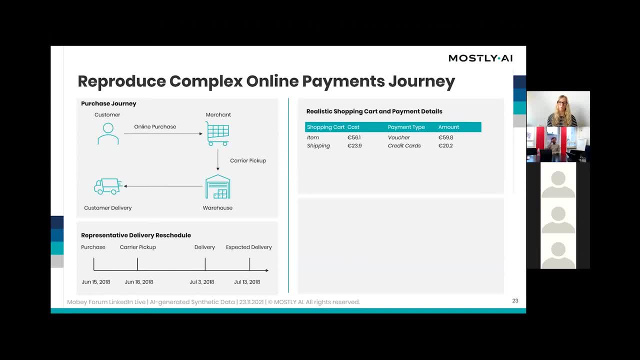 which is so important to understand customer behavior and make personalization happen. So what they really saw is that the data reproduced complex online payment journeys where everything was retained from, for example, what type of payment method was chosen, which items were purchased, how long different periods take, where some issues in the warehouse and 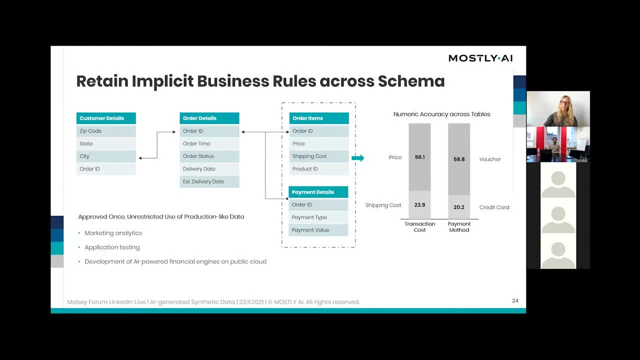 And one thing that's also very important, especially when it comes to testing, is that our platform is capable of retaining implicit business rules across EMA, which really also when you synthesize whole databases- is important to have feasible data for your testing efforts. 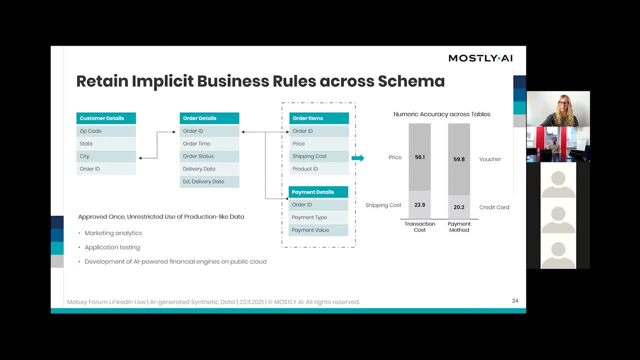 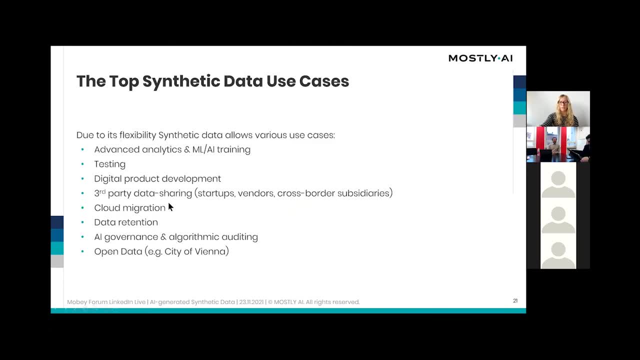 But this was just one example. Another example- I don't have any slides on this, but is coming back to this data sharing use case. A Fortune 100 bank has the need to, for example, validate over 1,000 vendors and also startups every year, which up until now led to significant costs and also time commitment from the whole team working on these initiatives. 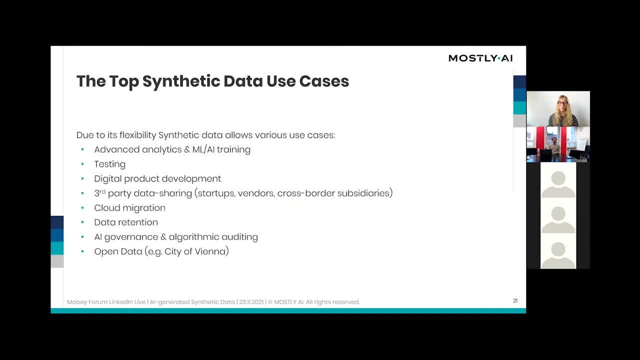 And with synthetic data, they were able to reduce the time it needed them to, or it took them to, share data by 70% And the costs associated with it By 80%, which, at the scale of this company, with 1,000 vendors and startups that they validate each year, resulted in 10 million of cost savings annually. 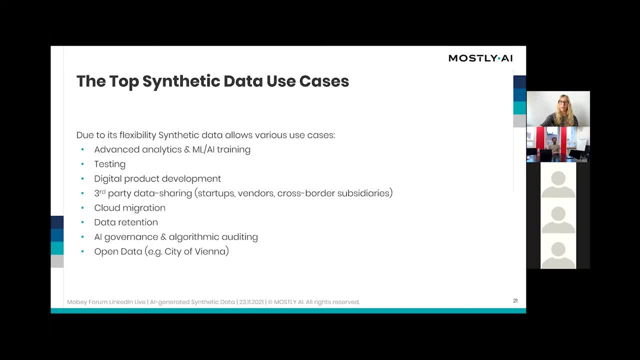 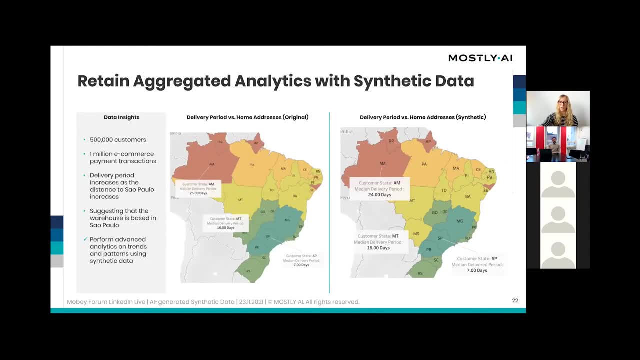 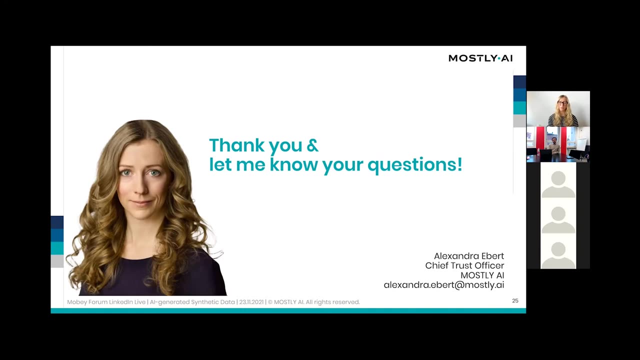 So just a few examples of synthetic data usage, but basically it's a technology that unlocks the data and makes it free to share, use or analyze for whichever use case you want to use it. So I think I'm out of time, therefore jumping to this slide and happy to take any questions about synthetic data. 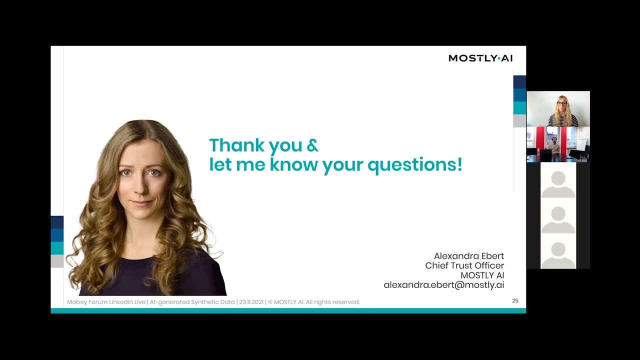 Thank you very much, Aleksandra. great presentation. I learned that legacy anonymization techniques are dead, long-lived synthesization, So very interesting potential And also, I think, many of our attendees. they know very well the pain of long data provisioning cycles of multiple months. 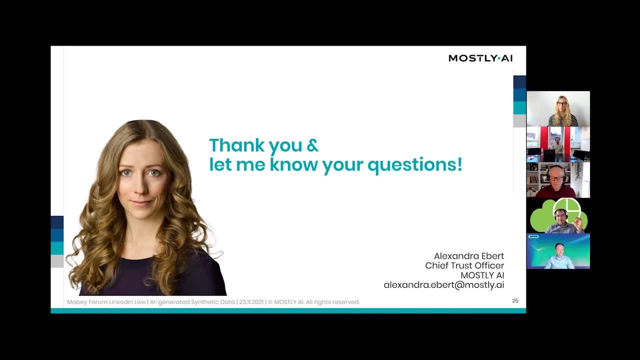 So this could be an interesting solution. Do we have any questions from the audience? Let's see. the computer has a question, but maybe if we have something, It's just, I think. thank you for the great presentation here. So the importance of synthetic data is also in any type of privacy. 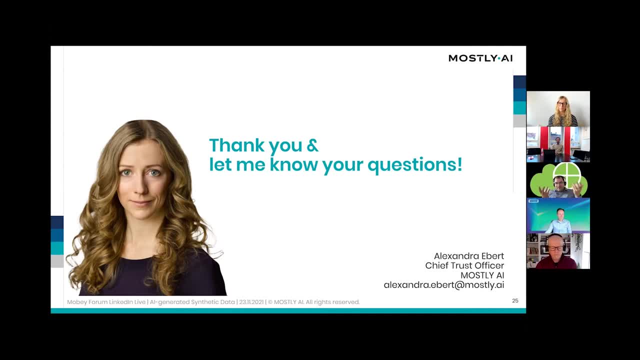 Preserving computing is around this concept of privacy budgets that we mentioned earlier Today. so if you just want to test a model on a given private real data set, then you have a limited budget. but for the actual model building process you need a lot of iterations, you need to iterate, you need to. you more or less need some data that you could like where you have a much bigger budget or like, say, unlimited budget. 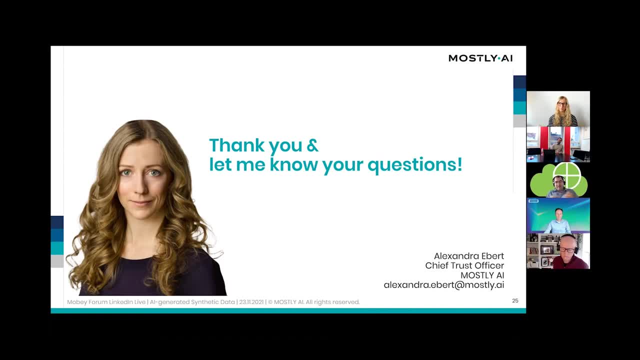 So synthetic data can be, the use of synthetic data there can be extremely important. So I think it's really valuable. I think so. so that's. Thank you very much, Dietmar. Yes, completely agree. So it's really about the explorability of the data, that like anonymization techniques. in the past it was always like: okay, we need column 3,, column 17,, column 32, and whatever to make one specific use case happen, which of course requires you to know in advance what exactly you will need. 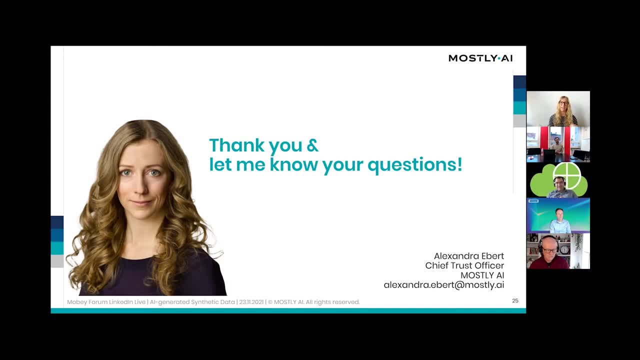 And this is definitely not how machine learning works. You want to have the access to all the 200, 300 columns available, And this is something that you can Unlock with synthetic data and really have data that's explorable and understandable by everybody. looking at the data. 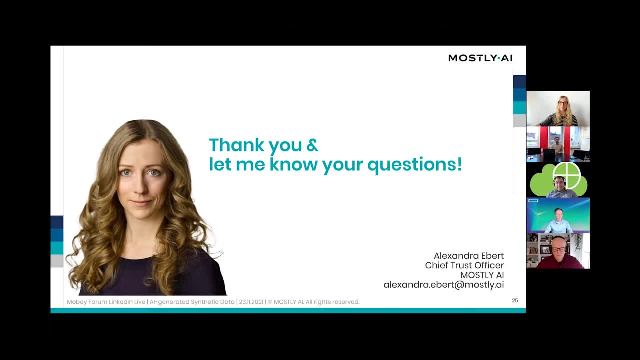 Maybe a question also which leads exactly to that. So how would you address data shift or model shift? to that Is this: have you had any recommendation how to approach it over time? You're asking for model shift when a model is developed based on synthetic data. 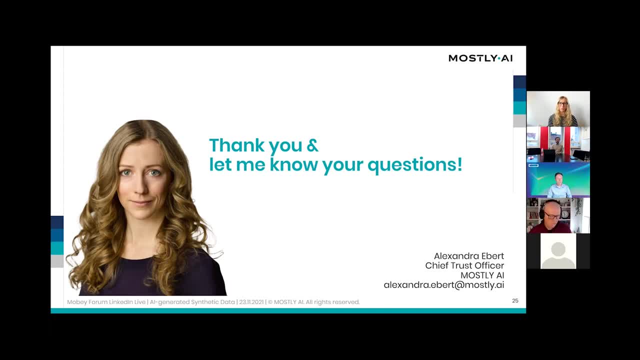 Yes, Basically the same as when a model is not trained on synthetic data to update Or basically correct the model every whatever you deem a relevant timeframe and resynthesizing data sets. So of course factors can change And if you trained your model two years ago and don't ever update in between, then of course you will have some issues. 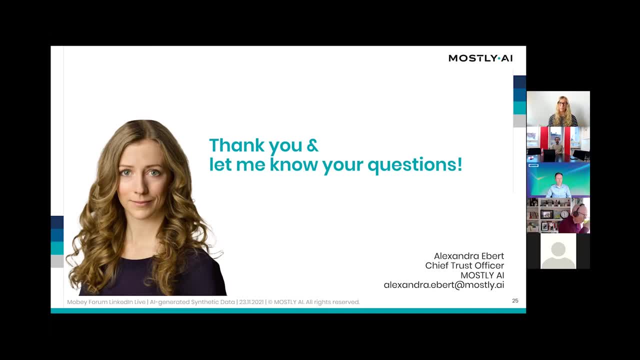 So definitely collecting new data, synthesizing this again and trying to mitigate this problem. Okay, Thanks. Also, I think the synthetic data engine becomes the part of your machine learning, I think a workflow as additional step within your data pipeline. that is, basically you're automating the entire process, end-to-end, and recalculating when it's needed to update your model. 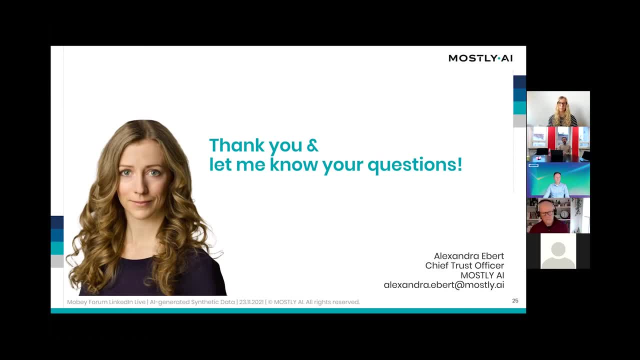 Absolutely. And then one other quite interesting aspect of synthetic data- didn't get to it in detail yet due to time reasons, but especially when it comes to fraud detection. we all know that it's a challenge for machine learning if there are not enough examples. 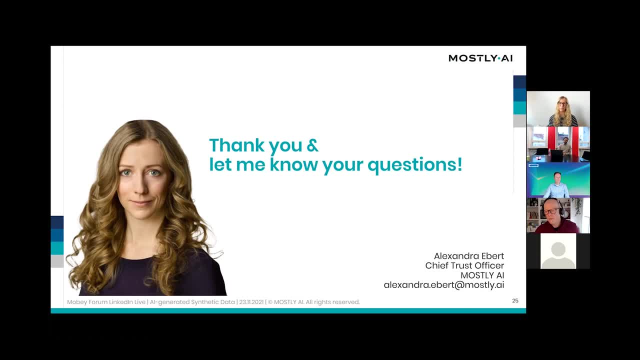 And one of the benefits of synthetic data Is that it can also be changed And, for example, you can boost or rebalance data sets and make more fraud cases in your example, which then help downstream models to train on this data to better pick up on certain patterns. 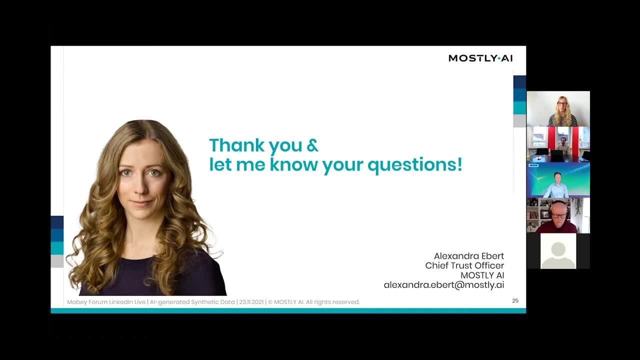 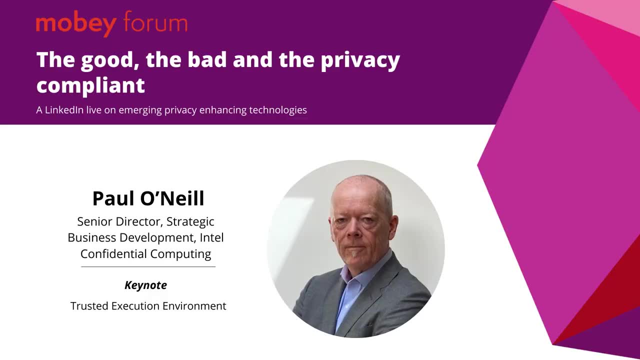 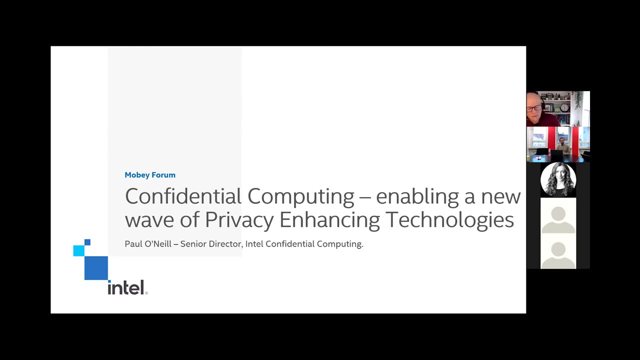 So this is also one of the use cases that is quite interesting for financial services clients. I work for Intel, which I guess most people know what Intel does, but I'm part of our security group here at Intel, what we call confidential computing. 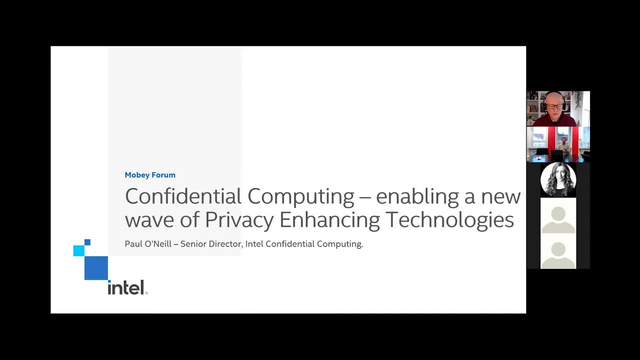 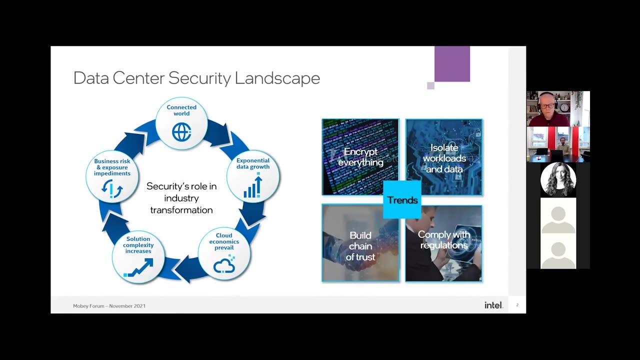 Everybody will probably have heard about confidential computing at this stage. it's a new paradigm and a new way of using hardware-based security technologies to drive some of the things that the previous speakers have talked about. I need to start at sort of our security view of the world. 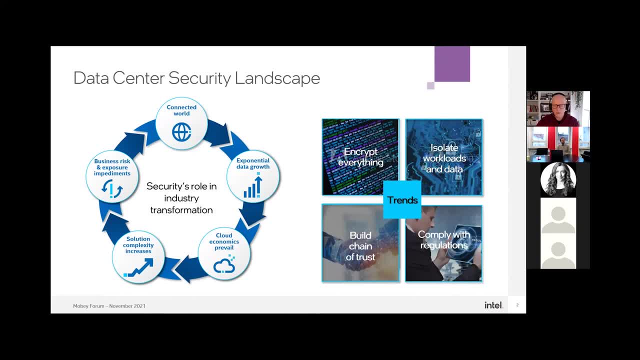 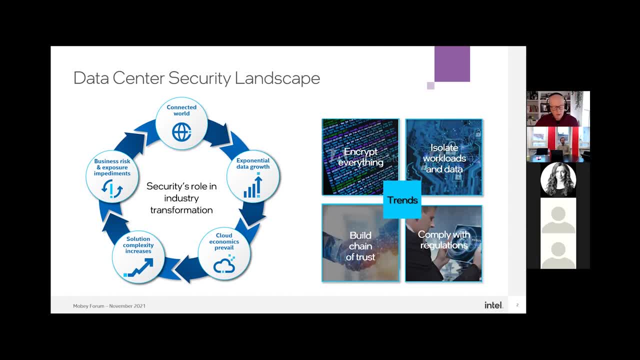 I'm really going to get down into infrastructure a little bit and build it up into what people are actually doing with this. But in order to sort of give you guys a view of what we're doing, I need to just take it back down to what our strategy is. 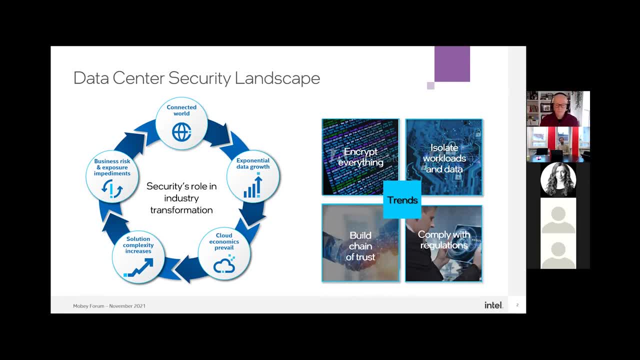 You know security is important. I don't think I need to tell anybody on this webinar that security is important. But what's driving the need? We're in a unique position in the world where we're seeing data centers built with Intel technologies. 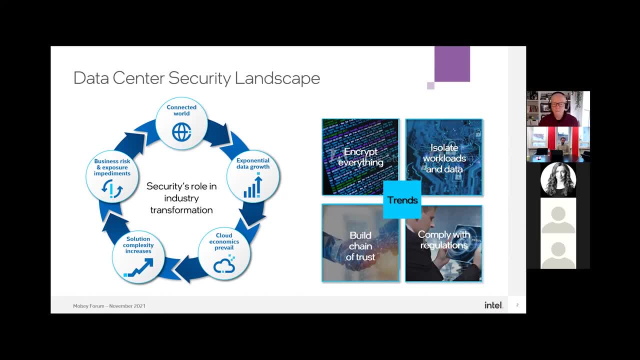 We're seeing what people are actually doing in the data science department, But you'll get information tomorrow. data centers: we're seeing the amazing amount of data that's happening. The world is becoming more connected. we're seeing this exponential data growth and in 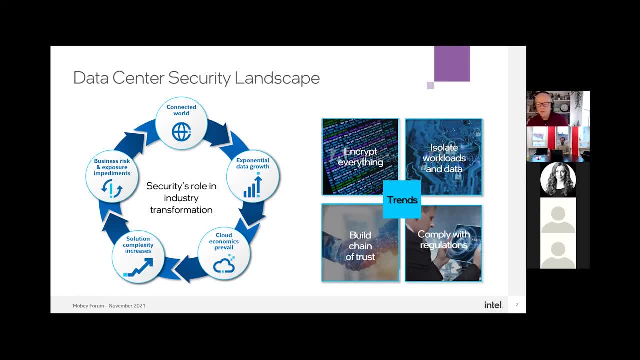 order to process the data. new computing opportunities, such as cloud and edge and analytics, are emerging, transforming business operations. There's a move to the cloud, as everybody else sees here as well, of bringing some very sensitive data sets to the cloud. These transformations that I'm showing here are driving big complexities for IT that are 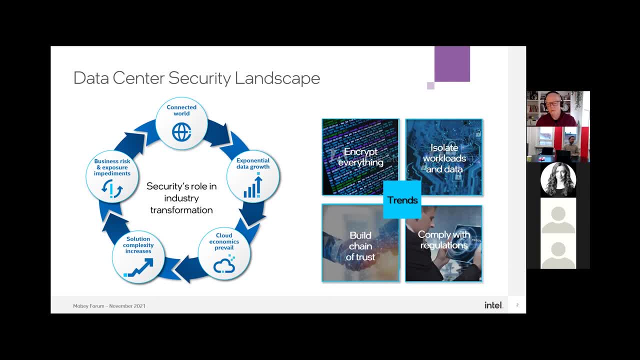 really increasing risks to business if the security part of this isn't addressed. So security goes hand in hand with this overall transformation, And the trends that we're specifically looking at here in this landscape that we're sort of relentless in our pursuit of is, first of all, encrypt everything. 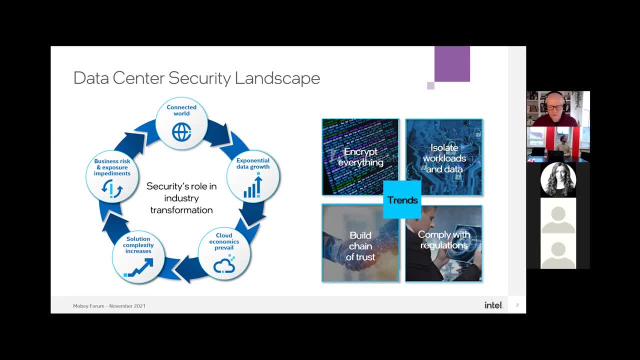 We want to see that everything gets encrypted and provide opportunities to do that. Keep workloads and data. Keep data isolated from each other. I think that's paramount- and we want to build a chain of trust that's rooted in silicon- and obviously our expertise is rooted down in silicon. 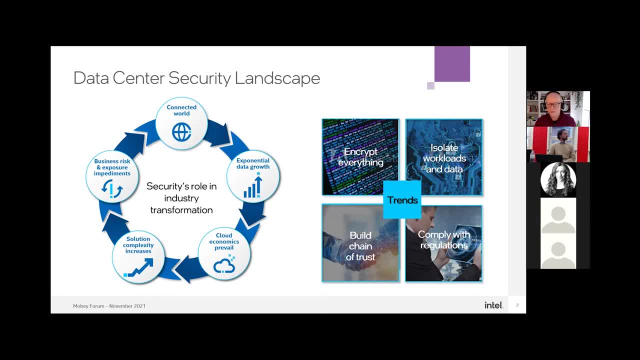 The biggest thing that our strategic customers tell us is that regulation and compliance with regulation is a massive problem for them. Compliance with policies and regulations generally- and I think the previous speakers have alluded to HIPAA and GDPR and now SHRM2 and all the other things that are going on in that space. 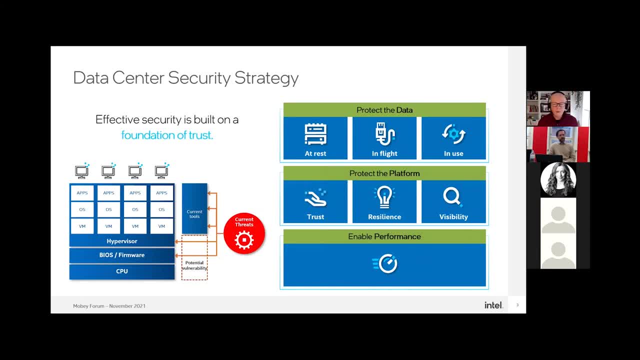 So security is only as good as the layer below it. You can have the most secure applications in the world, but if the operating system is compromised, it can spoof that application into thinking everything is okay And as the security and the software layers improves, attackers are generally looking to. 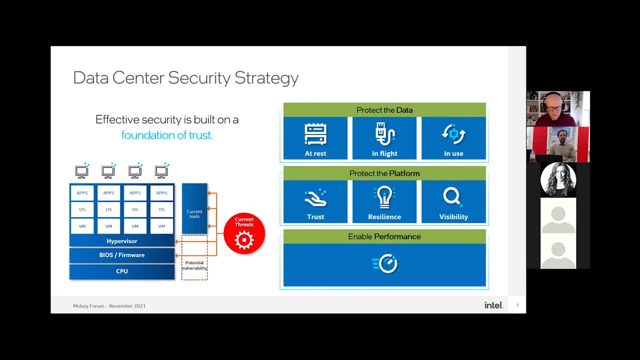 move down the stack to look for new vulnerabilities, And that's why we start with security at the lowest layer possible, right down at the silicon. Once the silicon is secure, then you can start to build solutions on top of that layer, And that's what we're doing at Trusted Foundation. 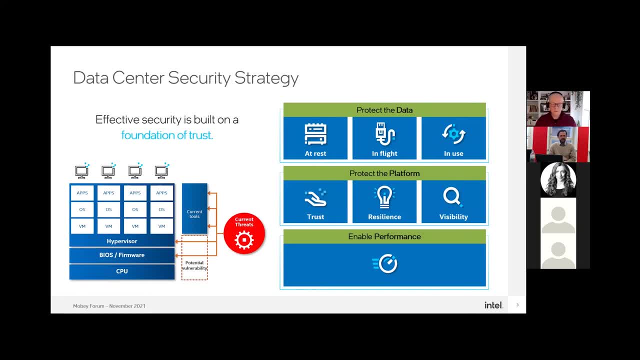 Now at Intel, we're focused on protecting data throughout all of its phases. Dimitar referred to the three phases that I'm showing here as well- at rest, in flight and in use- And we're helping to protect that platform by establishing a chain of trust. that's more. 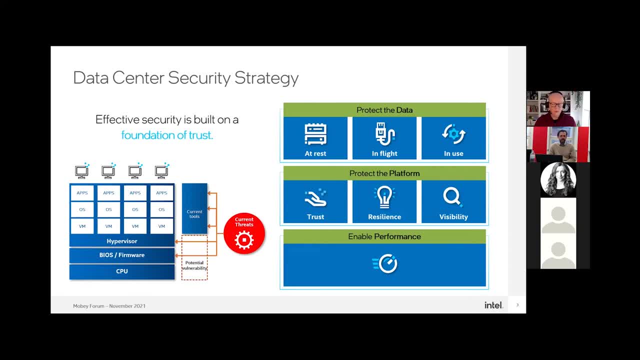 resilient against compromise, And the other thing we're doing is accelerating crypto functions to ensure that you don't have to sacrifice performance to implement security. A lot of the feedback we get from our clients is that security is a necessity. Performance is as important. 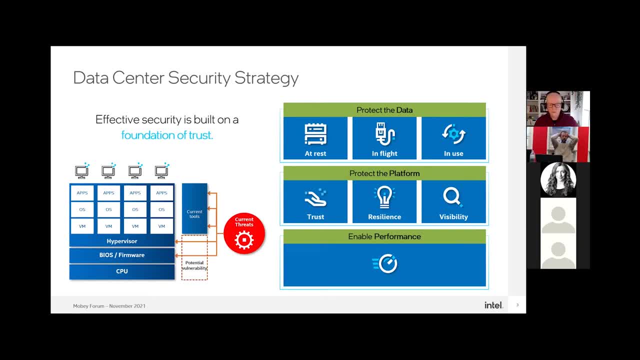 And the two are not necessarily the same thing. They want it cheap, but they also want it secure, which is hard. Now I want to drill in today into one of these in particular, which is the concept of data in use. So we've all long understood that data should be encrypted when it's been stored. 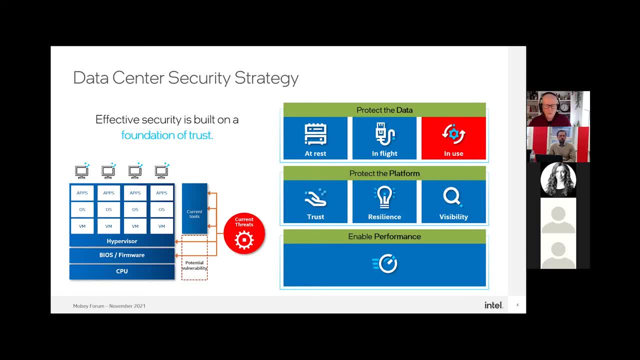 And we've known that you should encrypt it as you're moving it across the network. But what about when it's been actively processed in memory, especially today when systems are typically shared Or even operated by a third party And in that case, a cloud? 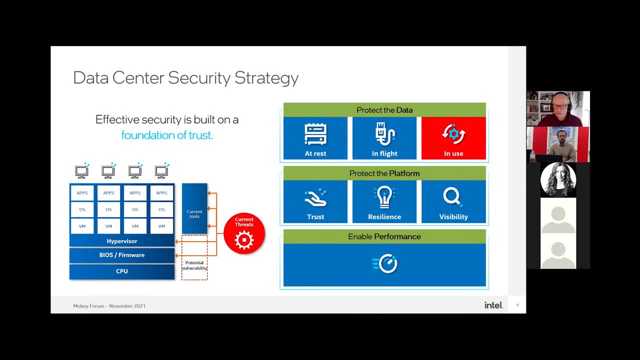 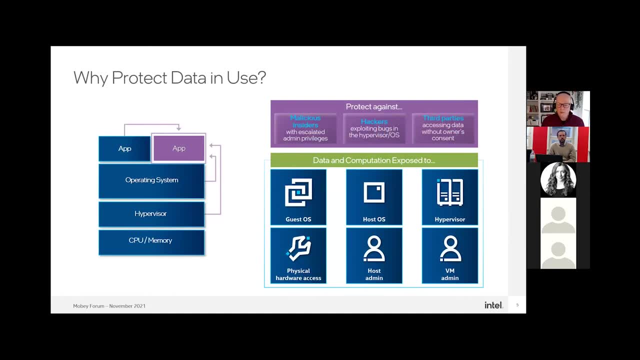 So doing operations on someone else's machine. So protecting and creating confidentiality for data in use is this new frontier that we call confidential computing here at Intel. Application data and even the code itself is under attack. So gone are the days when we can rely on sort of perimeter defenses alone to keep us safe. 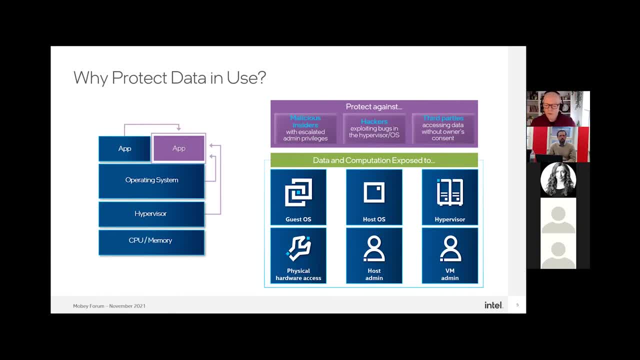 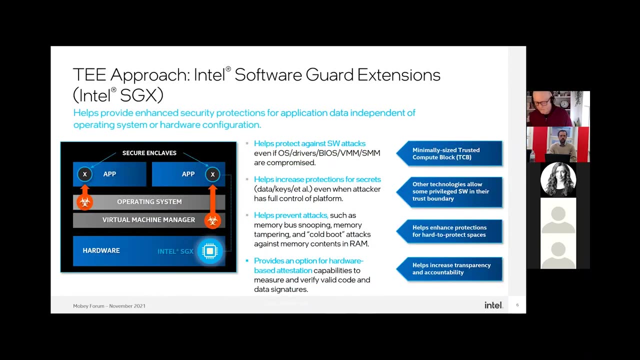 Attackers can be hackers or unauthorized third parties or even malicious insiders, And they can leverage exploits and other applications or privilege escalations or hypervisor layers. Sorry, got some technical issues here, Oops, Sorry, can you guys still hear me there? 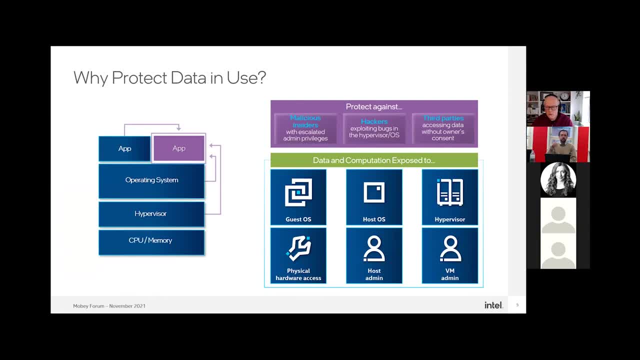 Okay, Seems I've lost my network. Okay, Could you guys hear me? I'm here. Yes, Okay, sorry, Yeah, apologies, I lost my network connection there. Sorry for a second. So we need this multi-layered defense in depth strategy to make it cost prohibitive. 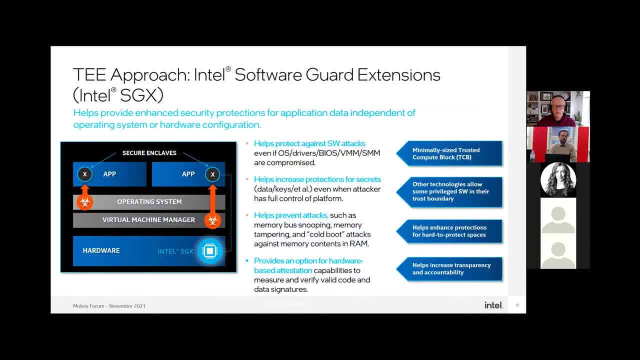 to execute this successful attacks. Now, in a few words, a trusted execution environment is effectively an isolated processing environment that runs parallel to the operating system. This provides several security features, such as the isolated execution of a program application, its integrity and also confidentiality. 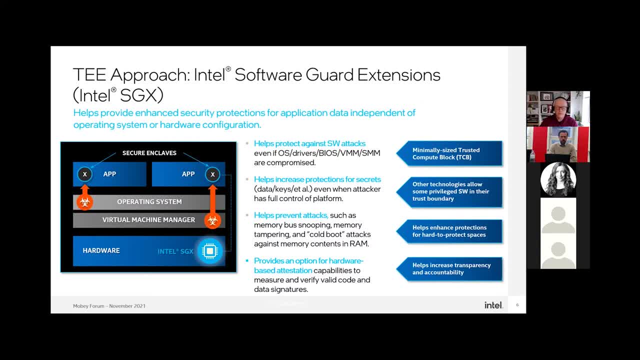 The data and applications stored in these trusted execution environments are protected cryptographically, And the interactions either between applications or with the user are securely performed. That is, it not only protects data, but also the communications with remote entities, and also enables trusted device identity and authentication. 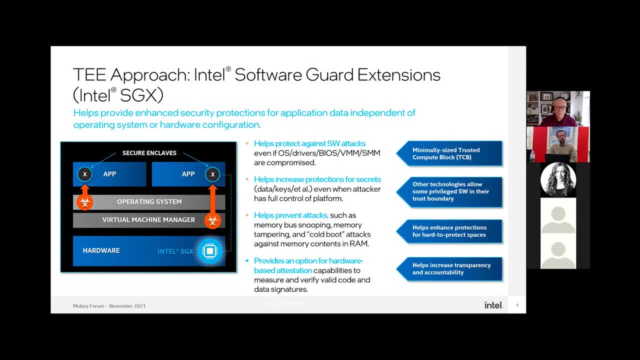 Intel software guard extensions, also known as Intel SGX, mostly in the market, has become the sort of preferred trusted execution environment for developers. It was nice to see Dimitar refer to it at the start of his presentation. So developers who want additional hardware assisted security for the application layer. 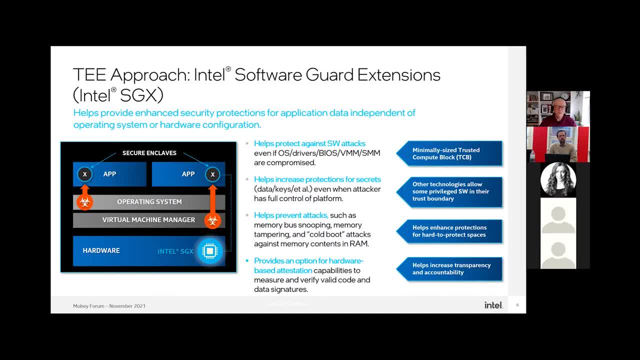 So, by definition, Intel SGX is a set of instructions that increases the security of application code and data, giving them more protection from disclosure or modification. So developers can partition sensitive information into enclaves which are areas of execution in memory, with more security protection. 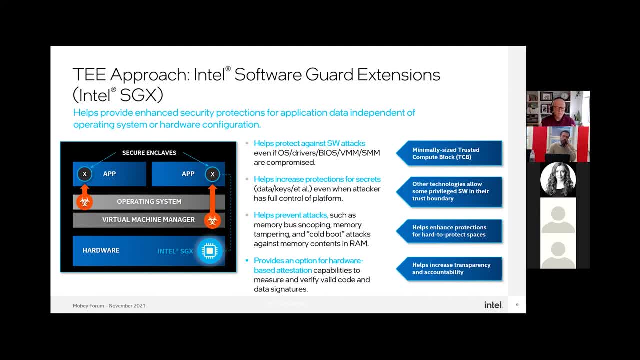 Developers are able to partition their application to two parts, trusted and untrusted. And the trusted part is what will be executed within the enclave or the secure hardware, or whatever words you want to use. The enclave is decrypted on the CPU and only for code and data running within itself. 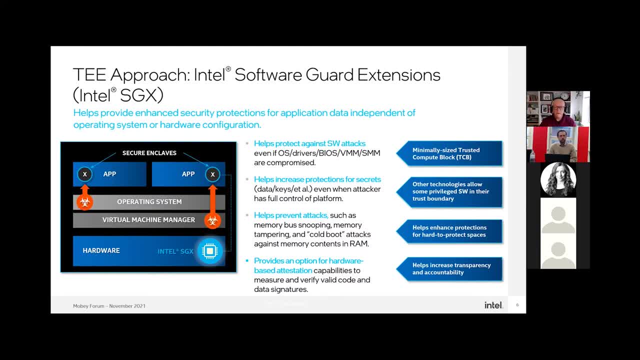 In this way, the content of an enclave cannot be read, except in its encrypted form, by any external processes, not even the operating system, or malicious insiders or whoever may be operating that operating system. Attestation is also a key feature of Intel SGX, and it can force the enclave. 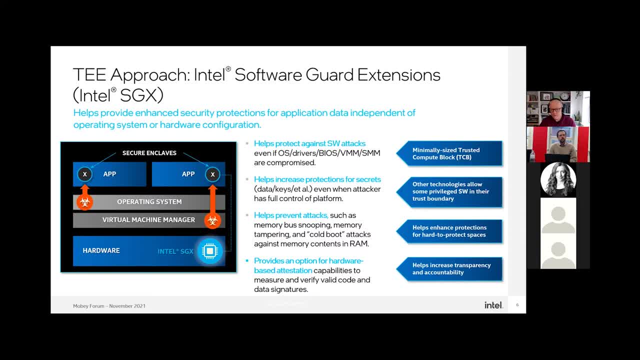 to prove its identity, prove that it hasn't been tampered with, that it is running on a genuine platform with Intel SGX enabled and that it's running at the latest security level. Also, we refer to it as the trusted computing base level, which is super important, if you're. 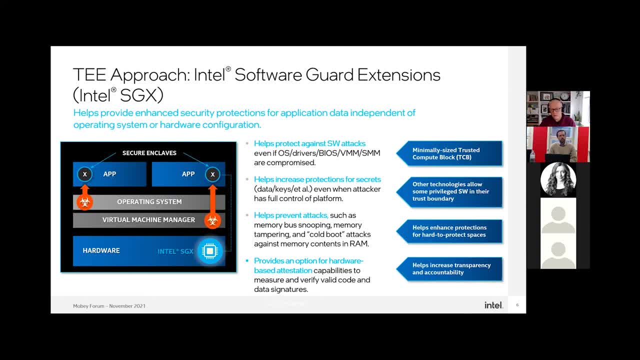 going to expose confidential data within those enclaves. Attestation can also be extended to confirm that a particular code hash is only permitted to execute within the enclave or to open an enclave. indeed, Attestation delivers integrity to not only the platform that is being used, but also to who and what can access your 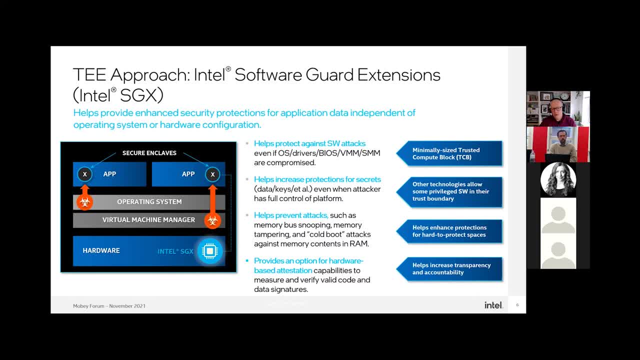 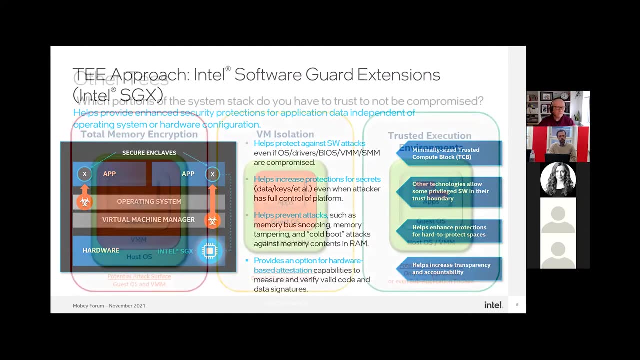 datasets, As Dimitar noticed, we refer to the combination of other technologies using hardware-based enclaves, and getting that attestation to prove integrity of computation is one area of real overlap. Now there are other trusted execution environments out there. They come in three formats. 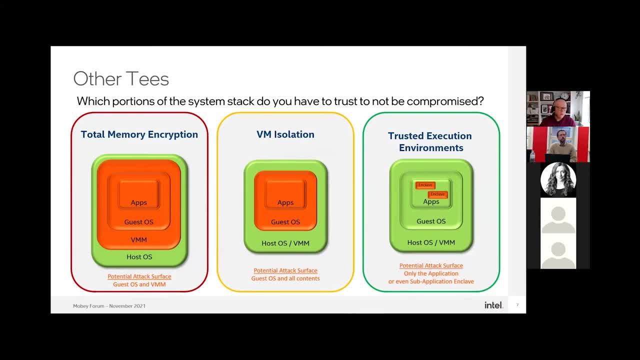 We've got one that is more total memory encryption, where you have quite a large attack surface. in those You've got the guest OS and the VMM inside of the attack surface. You've got others that are bringing VM isolation. You'll see that from Intel and AMD and lots of. 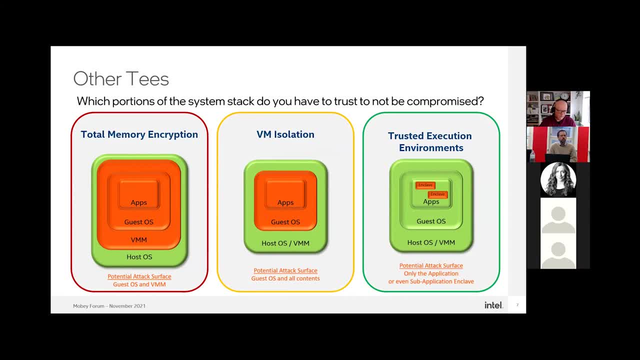 others, where the guest OS and all of its contents are inside of the attack surface. But only trusted execution environments really bring the application right down to, or sorry, bring the security right down to the application or even sub-application level down to even function, And you'll see them mostly from Intel and ARM with 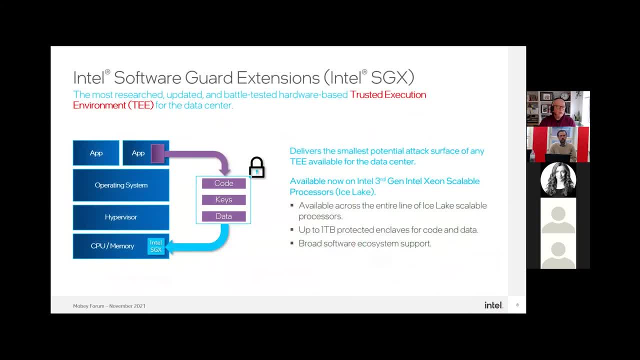 TrustZone as well. Intel SGX itself is really the most researched, updated, battle-tested, hardware-based trusted execution environment for the data center that's out there. There's a lot of research that goes into Intel SGX. We work with a lot of academia, etc. We have bug. 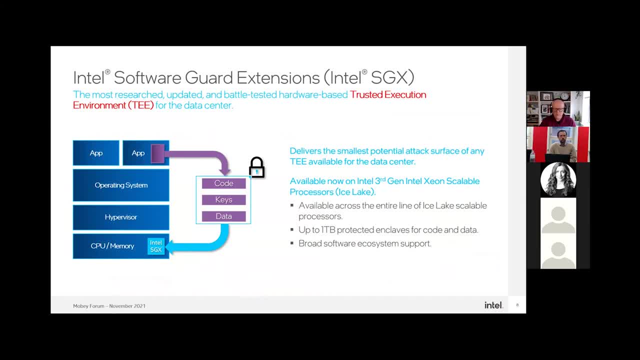 bounties and lots and lots of research going into what's going on with SGX. It delivers the smallest potential attack surface of any trusted execution environment available for the data center right now. It's available for the last six, seven years, mostly on the client side of. 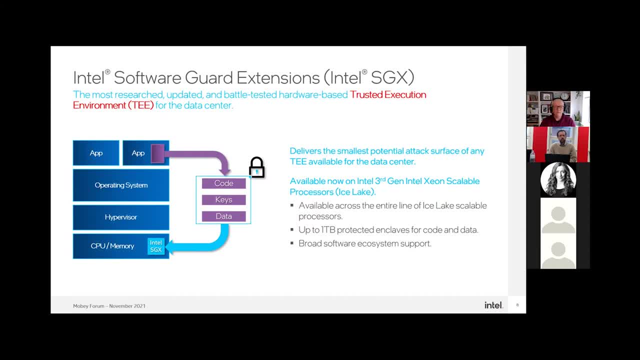 our house, And recently we've graduated into the data center with Intel's third generation Intel Xeon scalable processors that we call Ice Lake that released last year. We've brought them into the data center with enclaves that are available up to one terabyte. 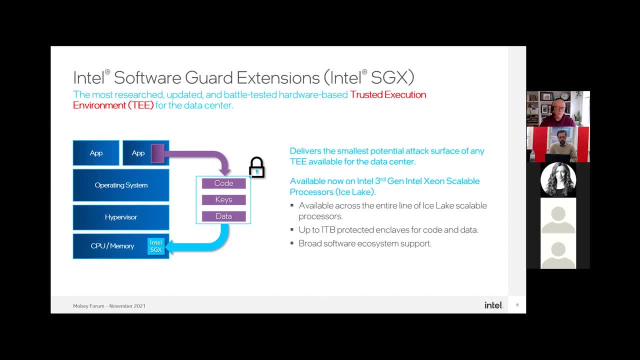 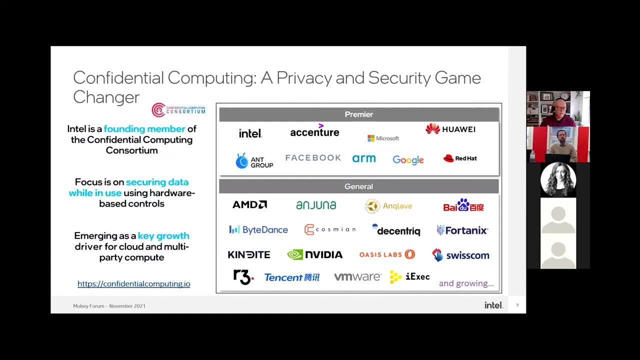 in size And that really opens up a huge area for interest for lots of different companies doing processing of video or genomics or other areas like that. Now, as we move sort of hardware-based confidential computing forward, we founded, along with a lot, 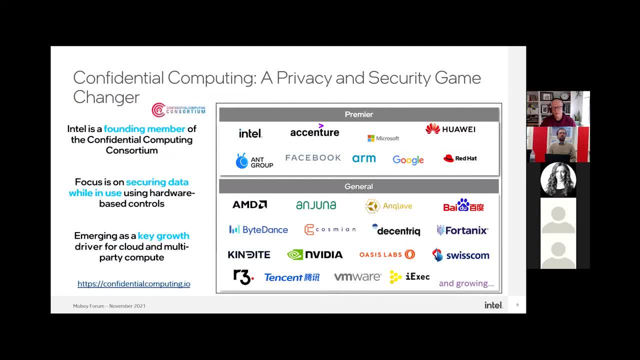 of others that you can see here- the Confidential Computing Consortium- in August of 2019.. The focus for this consortium is securing data while in use using hardware-based controls. Here at Intel, we spend a lot of time with open source. We do think open source is quite critical. 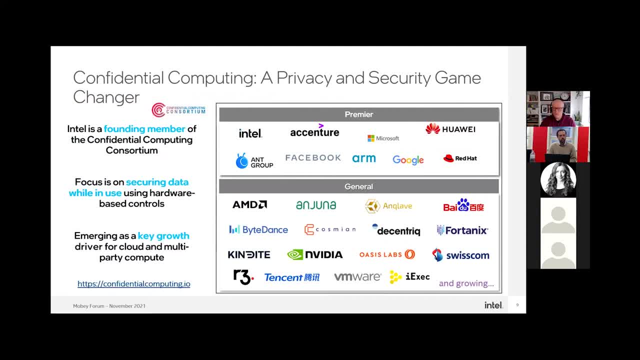 and that's why we helped to found and fund this original Confidential Computing Consortium. We want to accelerate the awareness and adoption of confidential computing as an infrastructure layer for privacy-enhancing technology to be built on Intel, SGX or other like-minded environments are to. 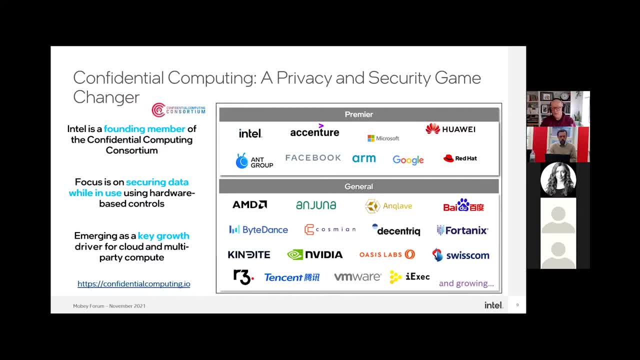 support and reinforce those. We want to build an infrastructure layer for privacy enhancing technology to be built on Intel, SGX or other like-minded environments, or to support and reinforce others that are out there as well. it's very much a growing membership um lots of interesting. 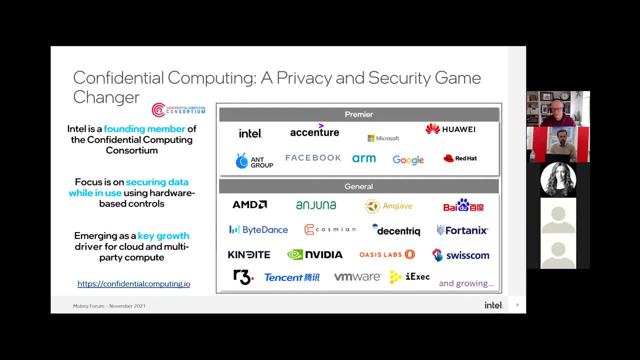 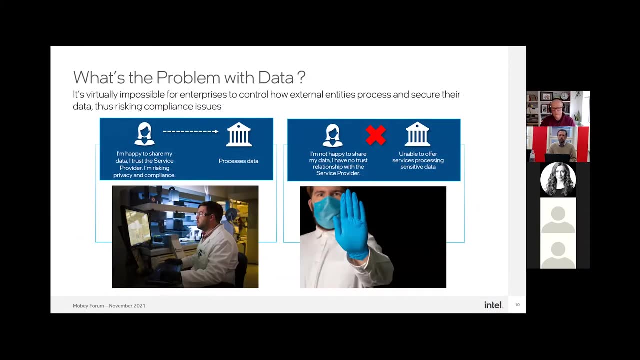 companies coming here, both startups and established companies that you can see on this list, and it's something that we intend to invest in over the next couple of years, as we sort of uh looked at, you know, when we built out our strategy around data center and intel sgx and why we would bring 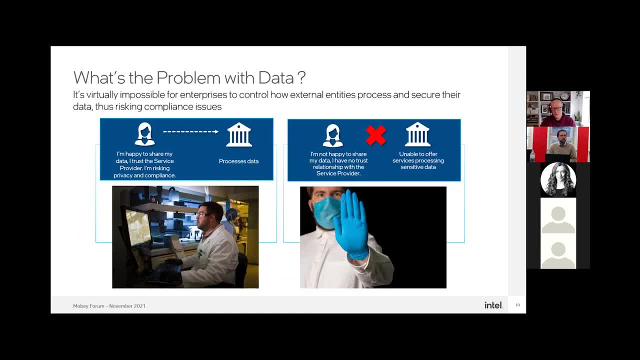 these large enclaves into the data center. we talked to a lot of our customers uh, financial services and healthcare companies mostly. um hartwood mentioned healthcare a lot in his presentation. we're working with a lot of healthcare companies on research at the moment as well, and our research really came down to a couple of areas. one is uh. 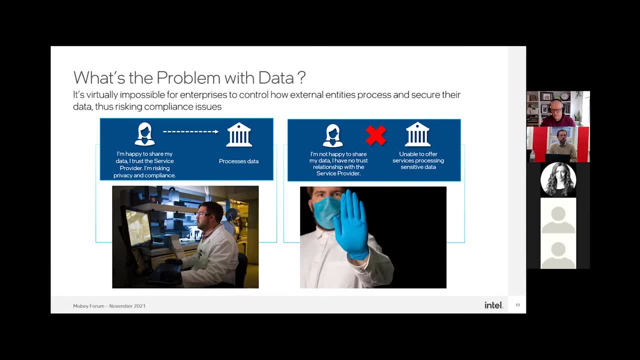 you know, i- just i- i'm terrified to share my data, but i want to share my data without going through different processes to do it. so in this case, you know, you could imagine that you're a data analyst in a bank who you're sitting on the submit button for uh to to share some sensitive data. 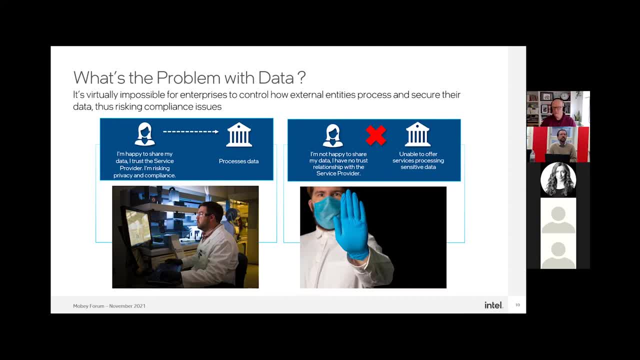 and when you click that button, some of your customers most sensitive financial records are going to be update, upload to a research firm which is performing an analysis in that data. you have the customers consent, etc. but they desperately want to help- anti-money laundering, for example, um. but you're still worried um what happens if a rogue employee at the intermediate? 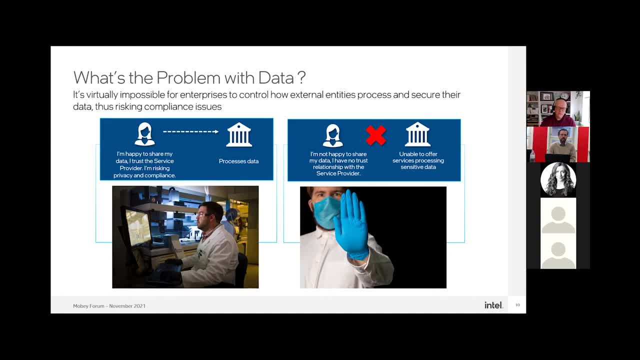 rate is going to be able to get the data and the data is going to be able to get the data and the reform stole the data. or what happens if the research firm is using your computer's data in a way that they didn't agree to? um, you know, they. that was the feedback that we're getting from a lot. 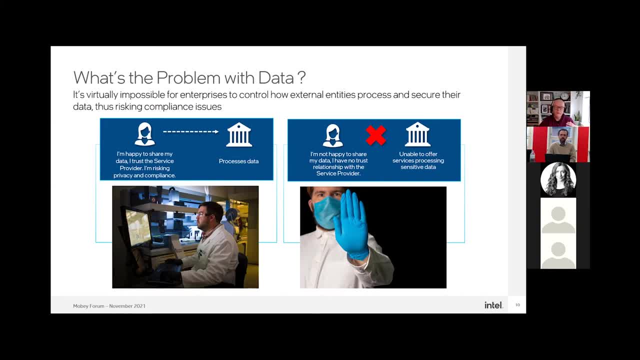 of our customers. it's not just financial services organizations, i said it's all industries face the dilemma every time. the mobility sector, for example, is another area that has big problems with sensitive data. the brutal reality is in a lot of these cases is that when you send data to somebody, 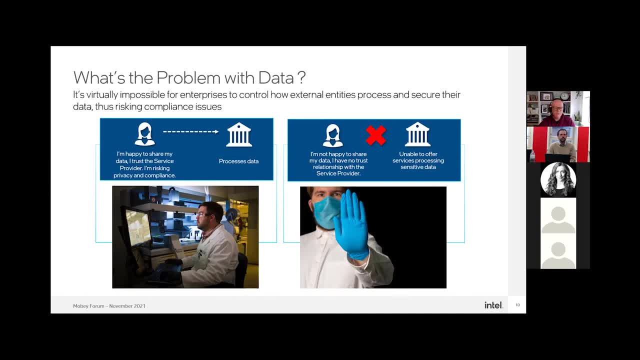 else. you've given technology, you've given over technological control of that. you're reliant on privacy policies or goodwill or contracts or law stuff that nobody kind of really reads. ultimately, when you send data to someone else's computer, you you have handed over all control. they could change. 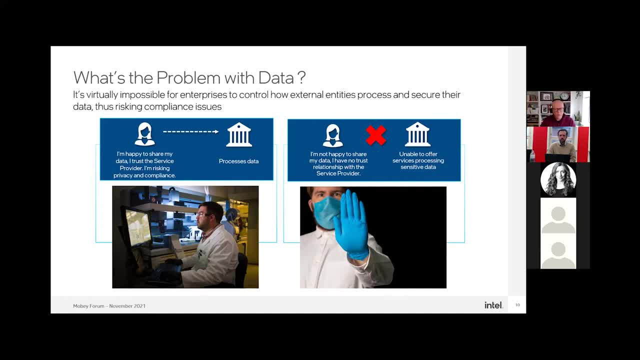 the algorithms that are running and you'd never know. they could take a copy of your data and use it for your own purpose, and you'd never know, or they could give you false results. even worse, and you would never know. as we look at you know building out confidential computing with things. 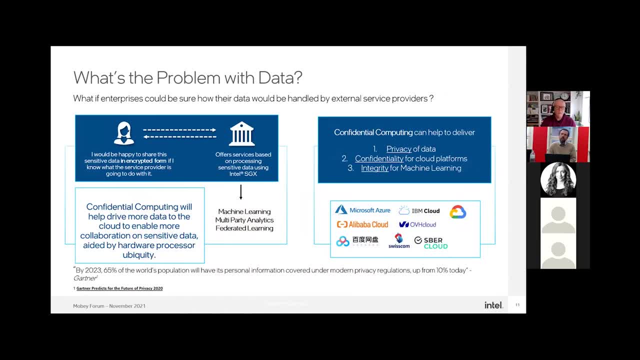 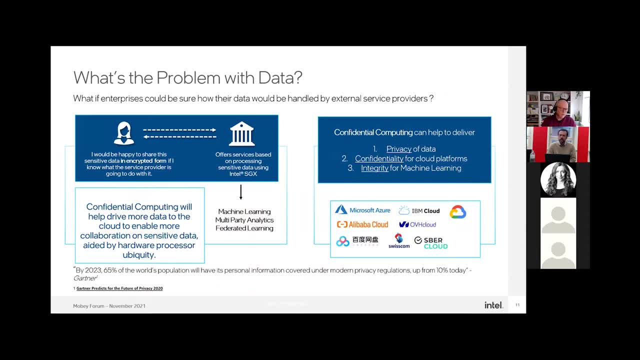 in the case of the bank analyst, um, you know what? if he could examine the algorithms that the research firm are going to use before they upload their data, if they can examine those algorithms, then he can be sure that only that algorithm can access that data inside of that trusted enclave, because that algorithm will have to attest itself. 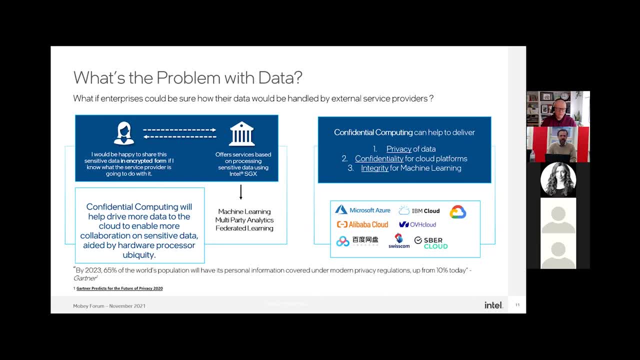 um. so i think confidential computing gives you that sort of view, um that you know for sure what will happen to your information after you you click that upload button and who you give it to. many of the world's biggest pharmaceuticals and medical research companies are looking at. 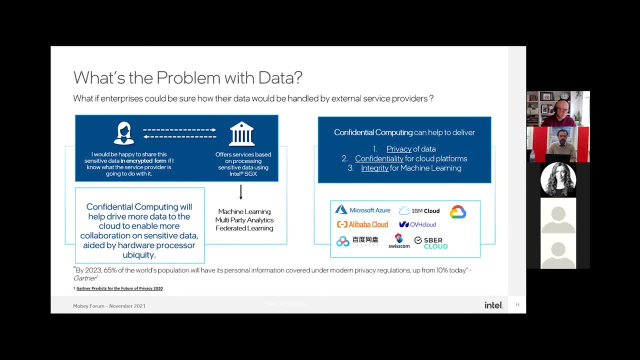 confidential computing techniques to build a sort of new data approach for real-time insights. both hartmut and dimitar are talking about federated learning, which i'll show a little bit later as well. but um, now we're starting to see offers: institutions offering services based on processing sensitive data using intel, sgx. 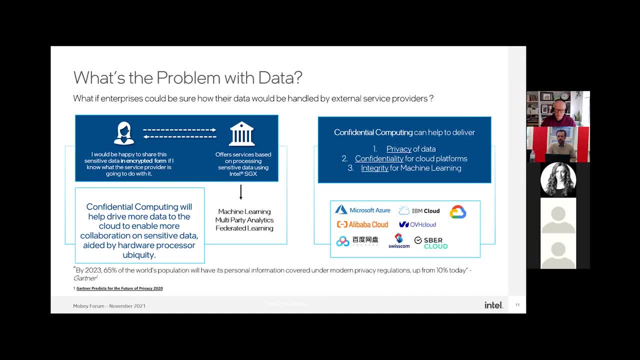 so the three areas that we're focused on with confidential computing and sgx as we move forward, and even its other technologies, is assuring privacy of data, or giving our data owners methods to assure privacy of data, to build confidentiality solutions that cloud platforms employ, and you can see some of those clouds there, for example, who are offering confidential computing. 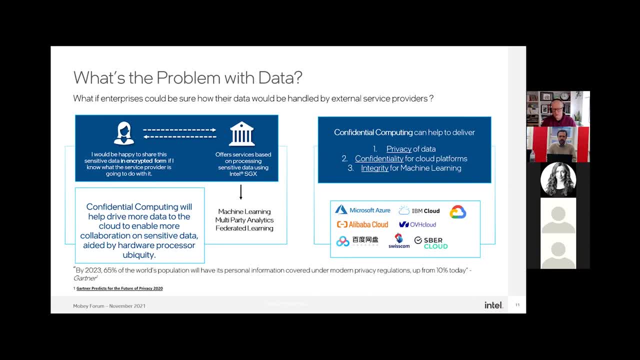 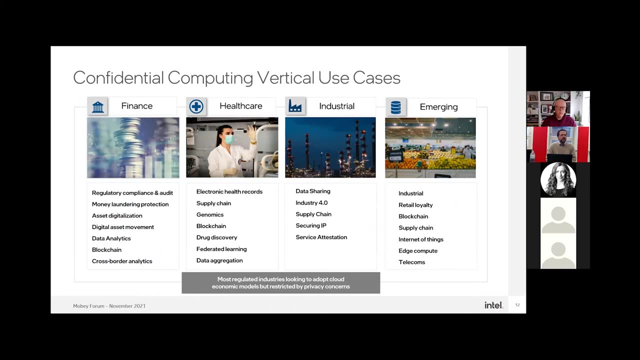 and integrity for machine learning, which really comes through attestation techniques and the ability to attest to who's doing what and attest that the integrity of the computing environment that's working on those data sets. now, as we look at, uh, where we're working with confidential computing, finance is really leading the way and i think the the reason there is that. 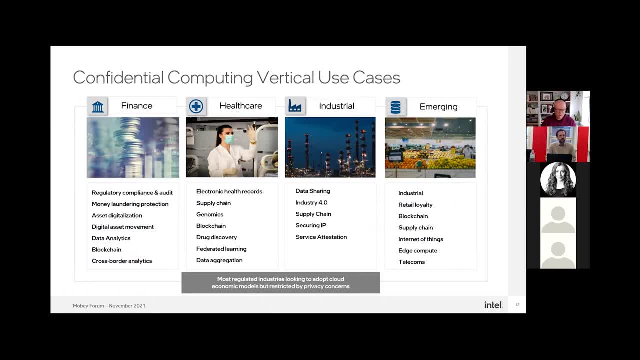 there's more money for research, there are more pressing problems. uh, i think everybody's mentioned some of these uh areas already: anti-money laundering- um you know, data analytics, a lot of up-and-coming work with blockchains, for example, cryptocurrencies defy as well, and the healthcare. 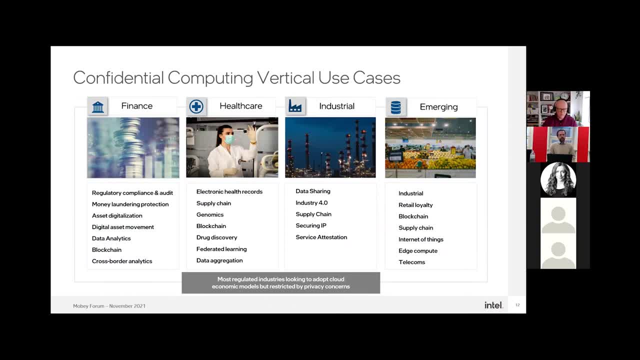 space. we've built large electronic health records, for example in germany around epa, e-prescription, all built on trusted execution environments, a lot of research with genomics happening inside of enclaves as well and industrial areas around data sharing, um gaia x was mentioned and sovereign cloud, etc. in that sense as well, the mobility sector is very 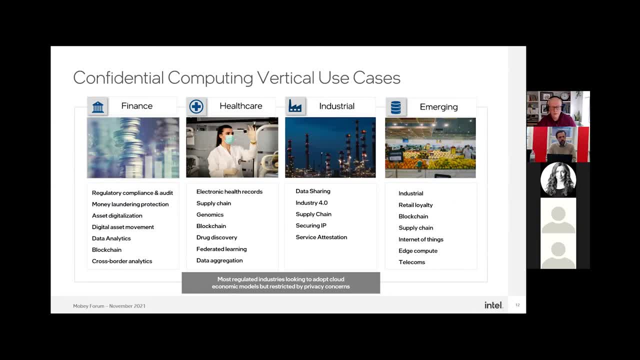 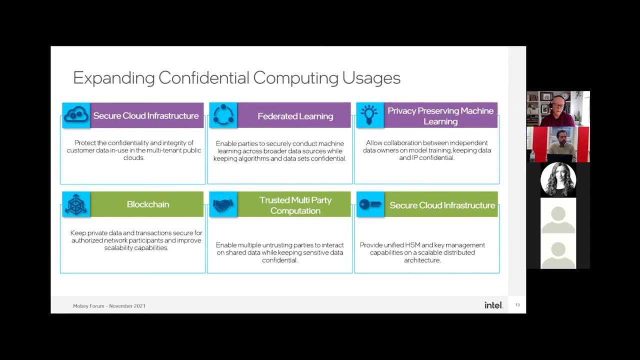 interested in using hardware-based um attestation techniques and trusted execution environments to monetize or release data in maybe even things like container x and lots of other uh emerging areas. but as we boil down uh some of the uh key uh points that were um our key workloads that we're 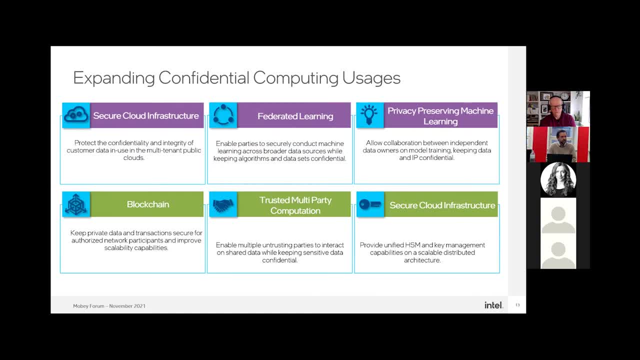 looking at. we really started this journey as a secure cloud infrastructure play right, the to protect the confidentiality of the infrastructure and the security of the cloud infrastructure and integrity of customer data in use in the multi-tenant public clouds. you'll see microsoft, google and others, as i mentioned in our previous slide, offering these confidential services and 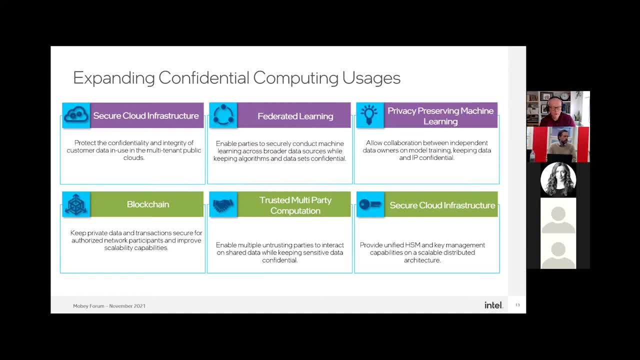 really, that's allowing companies to start avail more of cloud economics with sensitive data sets and to put their data to work inside of the cloud. we're seeing a lot of interest in federated learning, as others have said before, privacy preserving machine learning for collaboration and using a lot of data to help them learn more about the cloud and also the future of cloud. 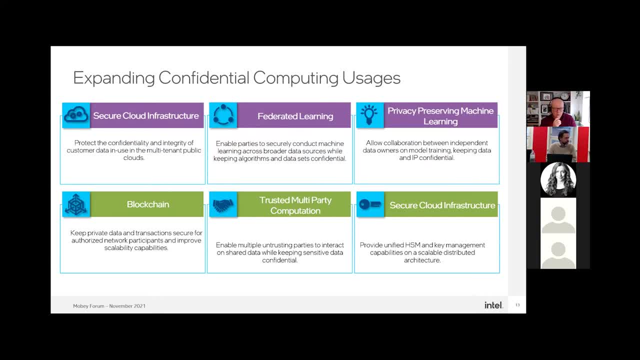 technology. we've seen a lot of interest in the cloud as well as the role of cloud at the weapons of cloud technology and um. one of the things that we've also seen in our project is that we've built in the cloud a lot of data on uh, data on the cloud um, and we're going to 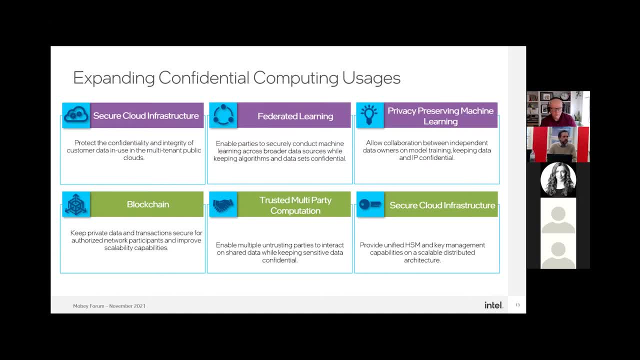 work with a lot of data on cloud and we're also working with a lot of data on cloud technology to support that on um, on internal data on the cloud, and so we're working with a large number of data owners on model training, um, people or companies who may not have implicit trust with. 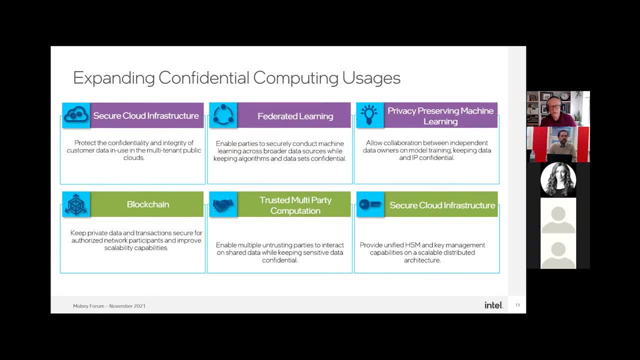 And trusted multi-party computation which people are starting to do in the cloud, and I meant to say secure key management there down the bottom right- rather than secure cloud infrastructure, But the concept and the ability to provide a unified HSM key management capability using SGX on a distributed architecture base. 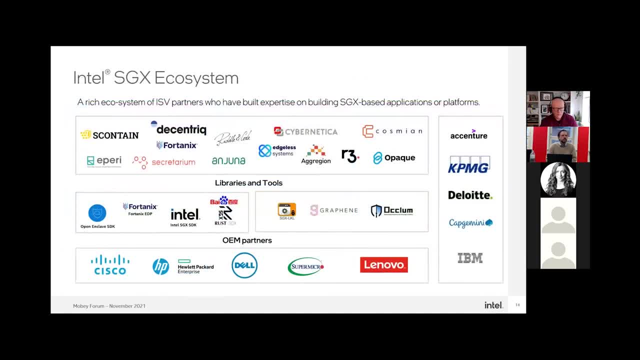 Now, working with trusted execution environments isn't straightforward. This is cryptography. You know there's a lot of companies that are using our technologies to build solutions, as I call them, our product. Intel doesn't do this. We are, as I said, at the top of this. we're enabling an infrastructure for a new wave of privacy enhancing technologies to come to play and to reinforce some of the ones that are out there. 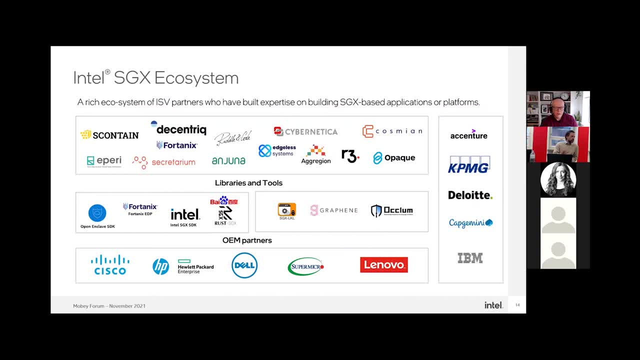 You can see some of these companies, for example, that are playing on this side of the world and they're building on top of libraries and tools That are available, you know, out in the market to build solutions here. At the end of the day, SGX has an SDK. the original Intel SGX SDK is there and that's how people you know build the most secure platforms with SGX. 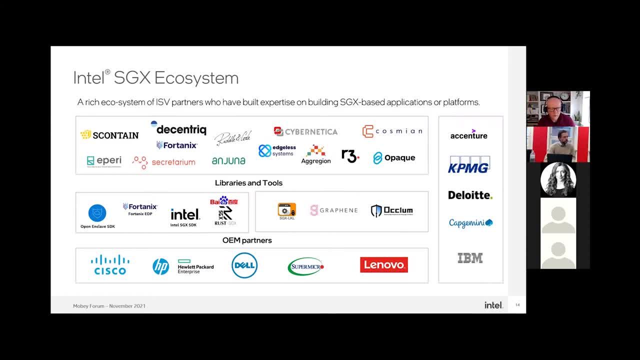 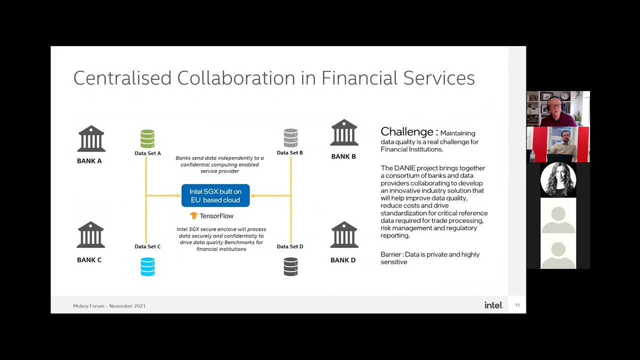 There are a lot of other things, like you see Graphene and Oclum there, for example, where people can simply secure containers with SGX, which becomes an interesting proposition for legacy code if people want to move that to the cloud. Now I'll talk a little bit about use cases. I can't go into the depth of others because I'm not an expert in the financial services area, but I'll do my best on what's happening with some of the other things that we see out there. 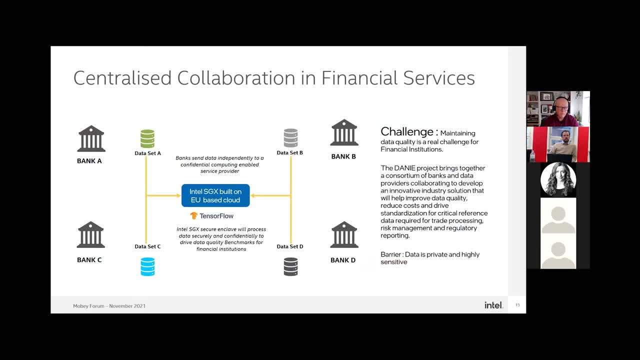 There's an interest in consortium, you know, to bring data together in a centralized manner. This is one project that's happening in Europe across 14 different banks, And the challenge really is around maintaining Data quality. so this consortium is bringing together these banks and data to. 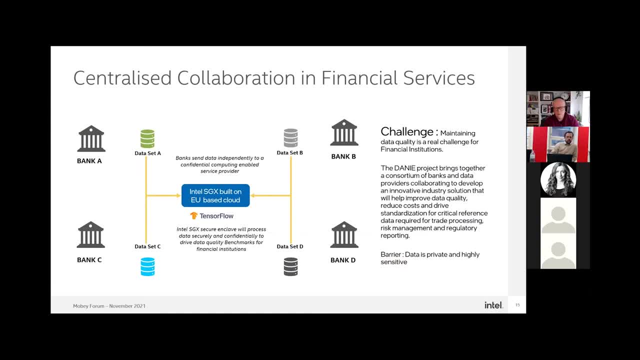 To do some critical referencing data required for trade processing and risk management and all the other regulatory reporting that goes on inside of financial services, And this has been built on a on a cloud, French based cloud, public cloud, where banks are sending data independently to a confidential computing enabled service provider, which is an ISD. 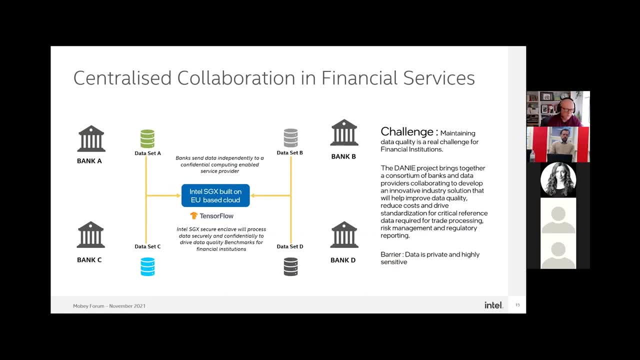 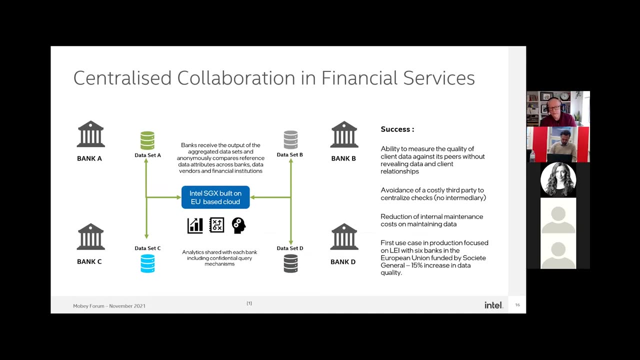 In this. in this case, they're using a tensor flow to Securely and confidentially drive data quality benchmarks for financial institutions. This is progressing quite well, You know. the banks are receiving the output of aggregated data sets and they're able to anonymously compare reference data attributes across banks, etc. 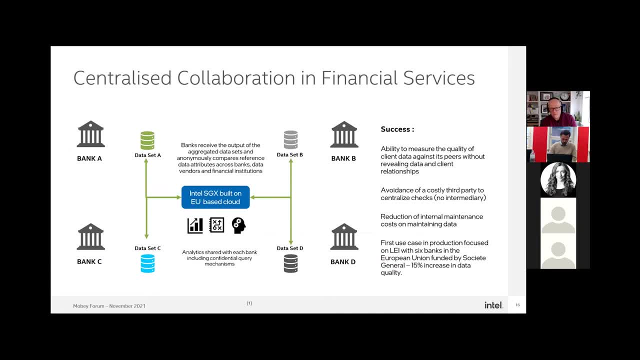 The analytics are also shared with each banks, and what they're looking at from a success criteria here is the ability to measure the quality of client data against peers with each banks, and what they're looking at from a success criteria here is the ability to measure the quality of client data against peers. 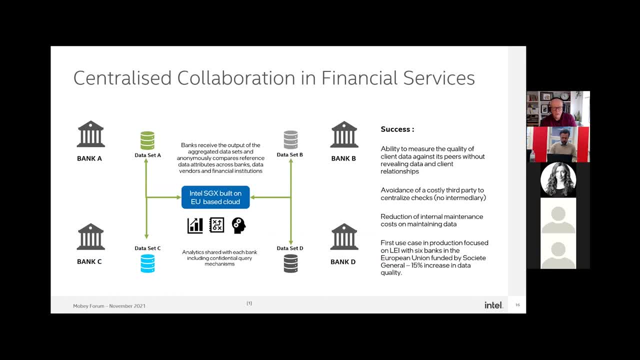 that revealing and he said- sort of data sets, obviously, And the avoidance of costly third party intermediaries that are doing centralized checking for this particular consortium at the moment. So there's a reduction on internal maintenance costs, Also on maintaining that data set, and the learning and training can happen as and when needed on a regular basis. And the first use case in production here is focused on early I, with six of the banks in this consortium, all EU based banks. 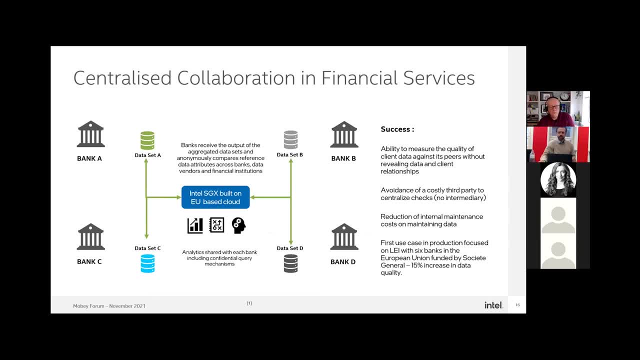 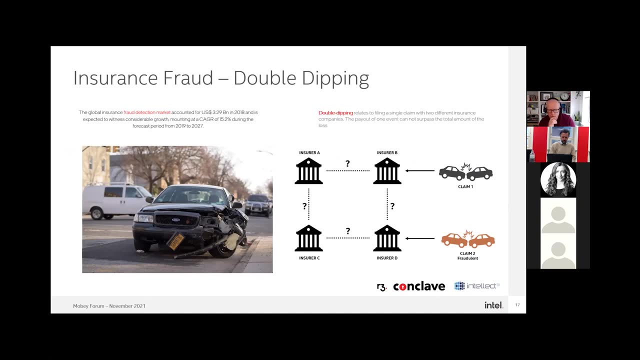 funded in this case by society general. they've seen already 15 increases in data quality and they hope to move this into a bigger consortium, uh, the early part of next year. um, we see a lot of interest in fraudulent claims as well. um, and i've marked some of the partners that we're working. 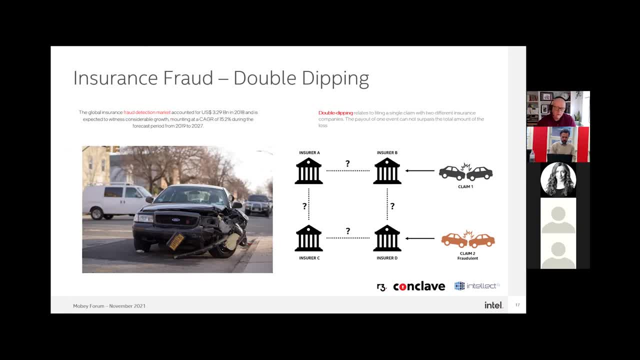 with here on the bottom of these slides, uh in the in insurance. uh, i think insurance are investing pretty heavily in fraud and fraud prevention mechanisms, uh leveraging newest technologies. uh, in this case, this is a fraud detection platform built uh on azure, microsoft azure with intel, sgx. 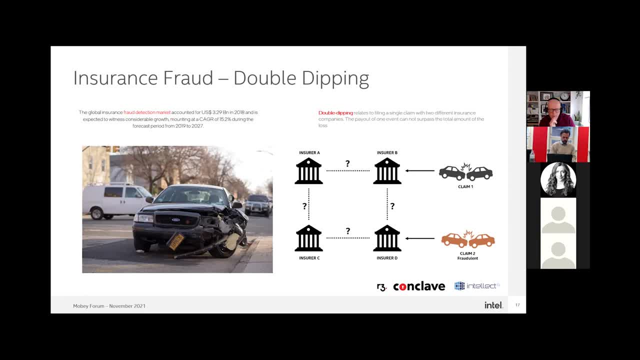 where this company claimshare by intellect to use, is separating claims in a public and private data and uses sort of fuzzy matching algorithms to identify suspicious claims um where that are suspected of being fraudulent- or double dipping, in this case, um once they're, the fuzzy matching sort of happens. 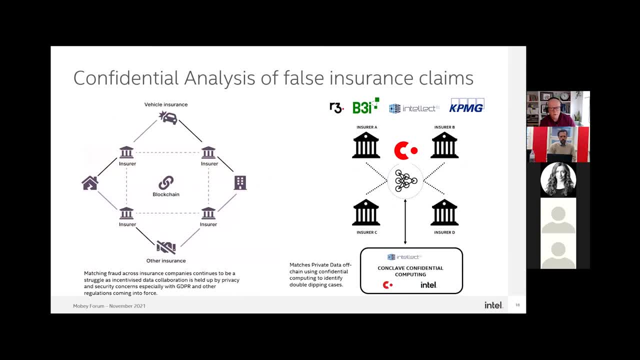 they're then taking the data off the chain and doing the computation between the two to figure out whether that duplicate claim is in fact coming from the same vehicle, that happened in the same spot, etc. etc. so it's matching that private data off chain, uh, using sgx, uh, and this will. this has 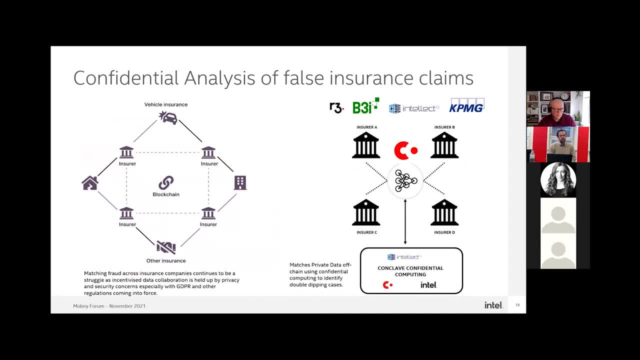 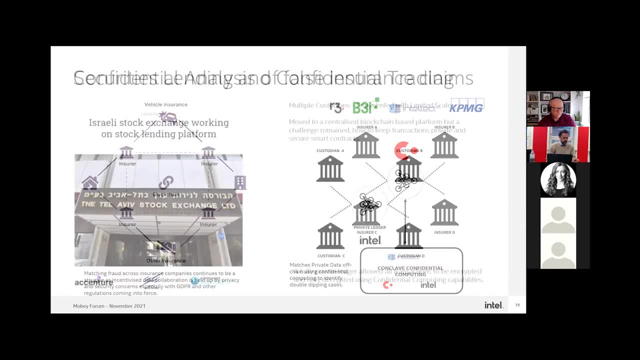 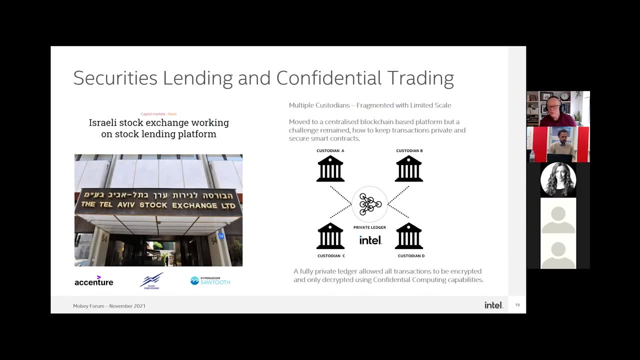 been launched across a couple of big insurance companies, uh, here in europe, um, and picked up a couple of big insurance companies like b3i, for example, the big blockchain insurance consortium in uh in israel- again looking at sort of capital markets and, uh, there's currently no central. 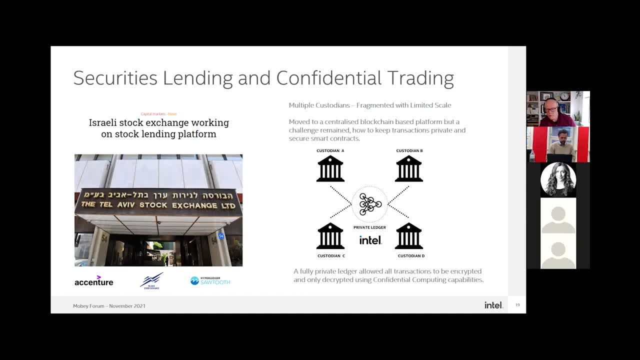 securities lending platform in the israeli market, for example. so securities lending is at present executed in the capital market primarily using interbanking mechanisms within and, if necessarily, outside the banking group limits. so, in this case, the use of uh dlt as the basis of the 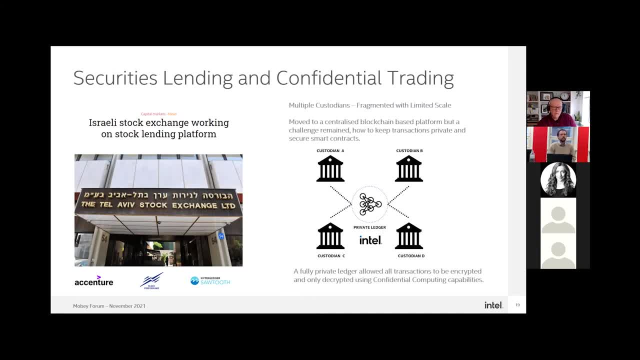 this sort of new trading platform is harnessing some of blockchain's primary advantages and features, such as direct peer-to-peer transactions, smart contracts, enhanced security through immutability, etc. And this is also then using SGX to encrypt transaction data as it goes across the chain. 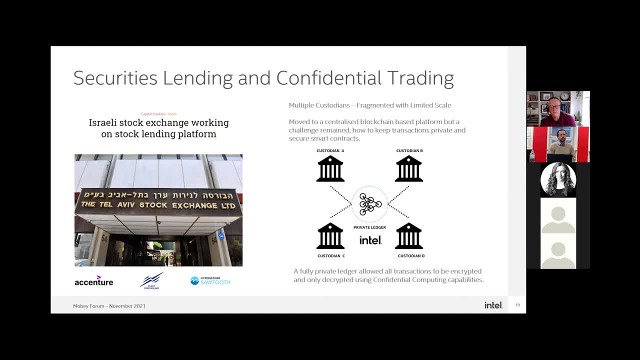 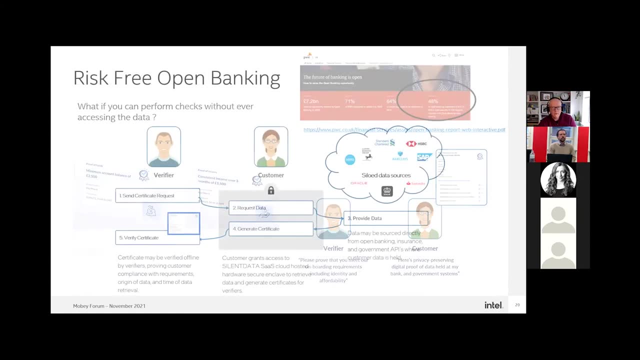 So it's keeping private data or data private amongst the transaction participants and provides closed DLT platform members with additional confidentiality capabilities, and this has been rolled out very successfully across Israel. I'll skip a couple of these because I know I'm tight on time. 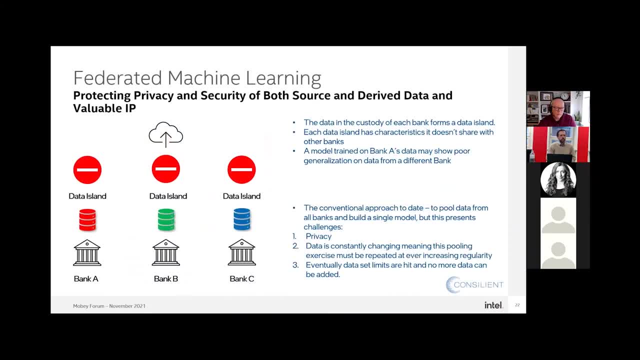 I wanted to just dip into federated learning a little bit as well, seeing as everybody else did, So I thought I'd throw in my piece on federated learning as well. A lot of our work is with the cloud providers, but we're also seeing a lot more. 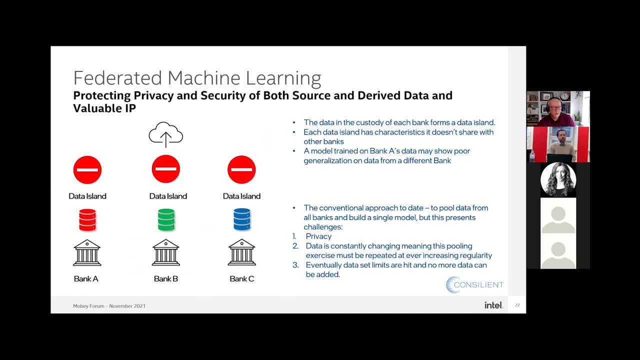 Federated learning requests and desire for federated learning to happen for many reasons: Privacy or data constantly changing, data set limits happening and people don't want to double their threat surface by moving some data to the cloud, and we're seeing a lot. 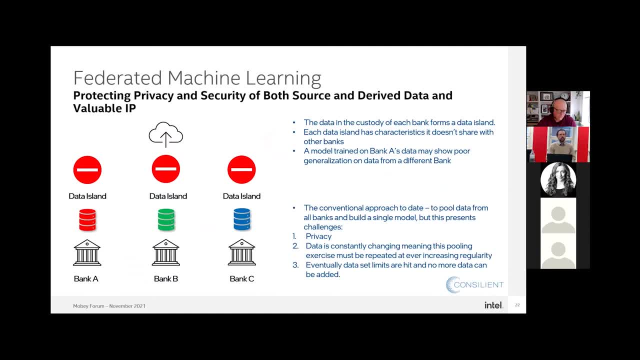 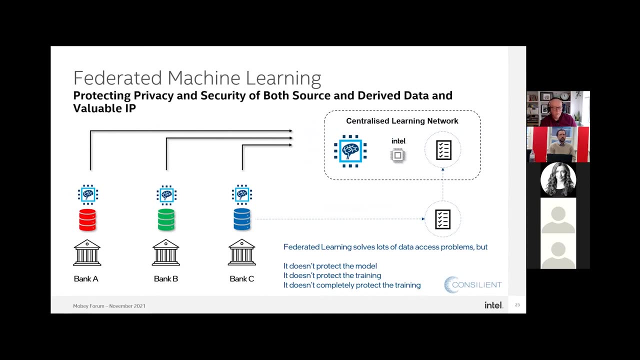 of this in Europe and also in the US, and not just in financial services but healthcare and also the mobility sector as well. Many different, disparate data sets in the bank. but ultimately, as we look at federated machine learning, We see- and I think others agree- that it doesn't protect the model generally and it doesn't 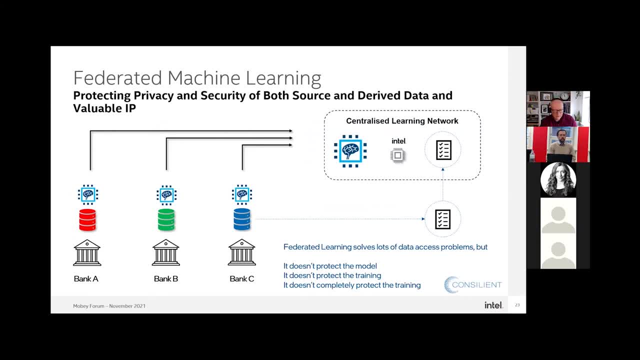 really protect the training. It doesn't protect the data completely either in that sense. So we're working a lot with- in this case I'm showing Consilient here, a company that's working across a lot of the big banks in the US building a pilot for centralized federated. 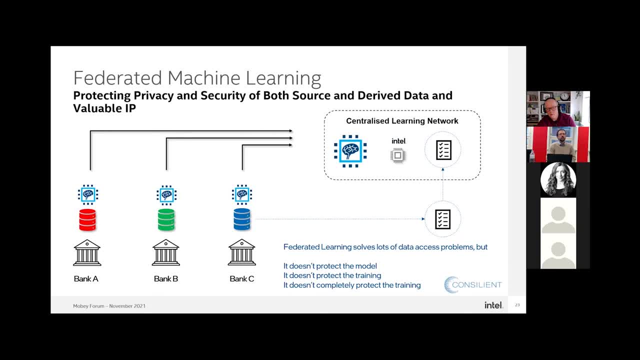 learning, Sorry, centralized learning. Yeah, It's a learning network that's building federated models to allow banks to get involved in this type of federation. And in this federated case, the centralized model has been developed so we can initially use synthetic data or sample of data to create the initial model and then get into a sort 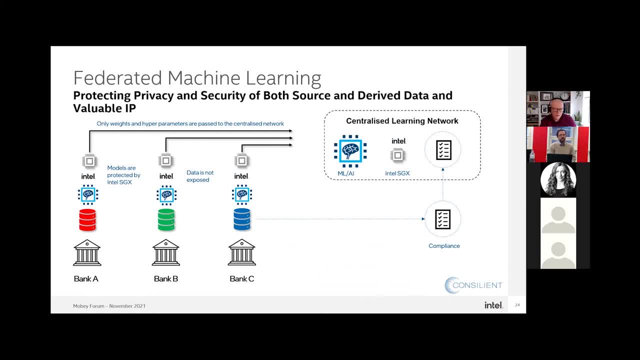 of round robin situation where algorithms go to bank A and bank B and bank C. There's no direct access to the data. The models are protected by Intel SGX. In this case, the biggest fear from a Consilient perspective was the model being stolen or 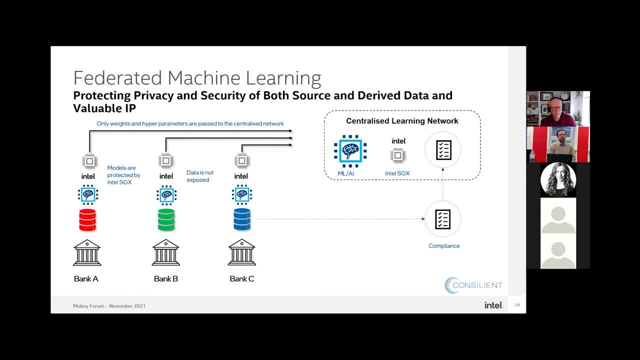 somehow manipulated, The data is not exposed, so the data owners are happy and only weights and hyperparameters are passed back to the centralized network. So the trusted execution environment here is really doing all of the protection. But not only that, it's providing two things. 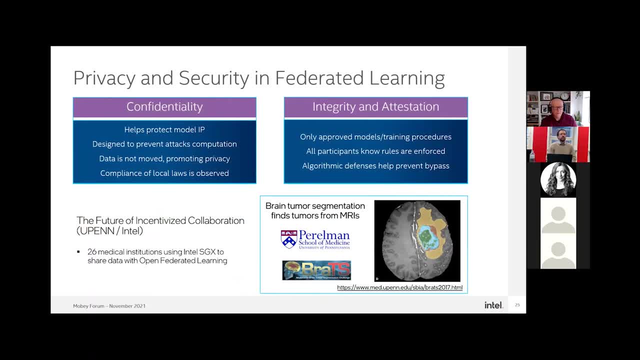 One is confidentiality, The second is integrity and attestation. So the confidentiality part of this helps to protect the model. It's designed to prevent attack computation so data is not moved, promoting privacy and legislators of wherever those local laws are. But most importantly, integrity and attestation is confirmed that only approved models and 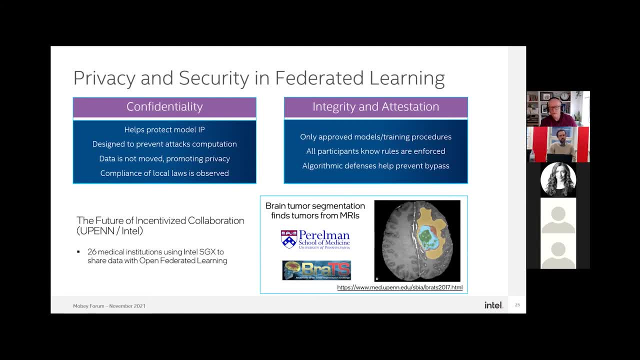 training procedures can happen within the federation and all participants know that the rules are enforced and algorithmic defenses help prevent a bypass to solve some of the poisoning, et cetera that Dimitar mentioned earlier on, And we've actually done this ourselves in the medical care area, where we've built federated 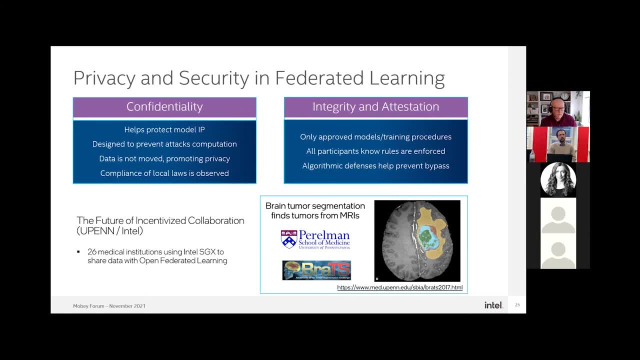 models to do brain tumor segmentation across 26 different medical institutions across 11 different countries and proved, with similar to some of the stuff that Hartmut showed, that it's as effective doing this in a federated way as centralizing models and as data starts. 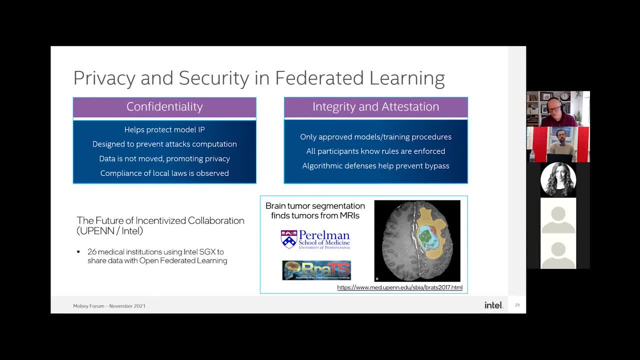 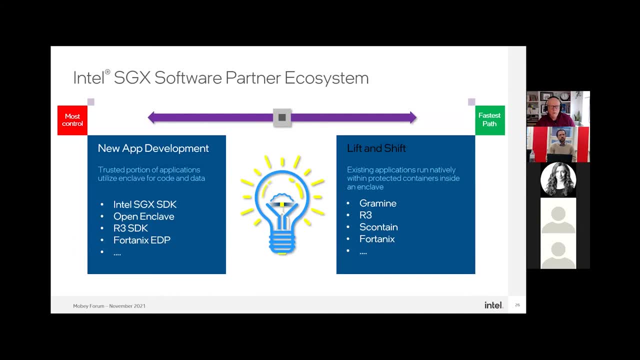 to grow bigger and bigger and more is generated. The federated approach to, especially to large data sets is likely the one that works out in the end. You know a lot of people say hey. you know, trusted execution environments are difficult. 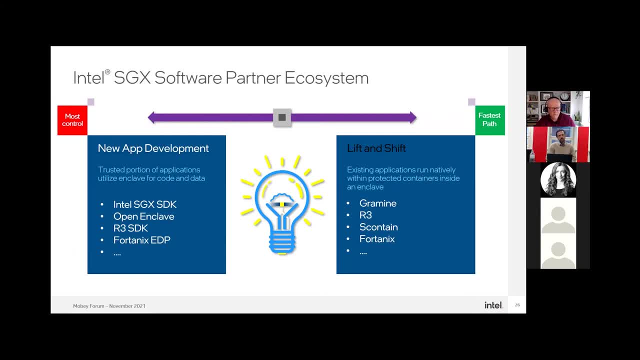 to work with. Well, they're not easy. right On the left-hand side, if you want to build trusted execution environments, well, you've got to know a little bit about cryptography and what you want to do. but by utilizing the trusted portion of applications and building down at an application or even function level, 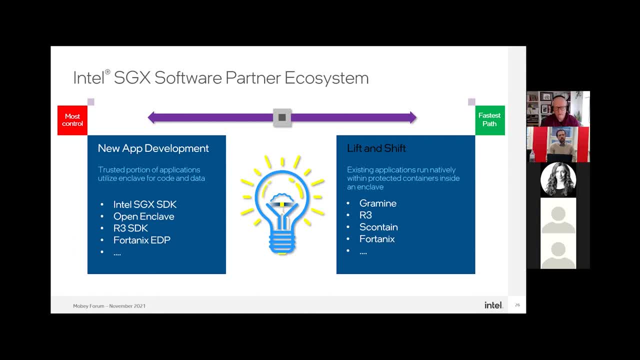 you really are garnering the most control. There's also the fast path to using trusted execution environments, where you can take, you know, runtime encryption environments or libOSes or items like that, and you can take legacy code and run them inside of secure containers, for example, which people are 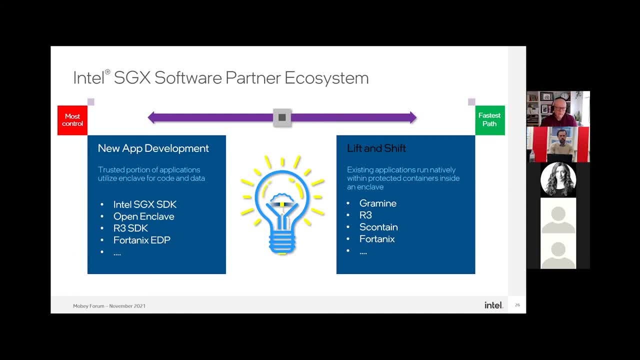 doing with things like TensorFlow and stuff like that. So that's where legacy code can be ported to the cloud or brought to the cloud using trusted execution environments. where Docker containers or Kubernetes can be ported to the cloud, These containers can simply be lifted and shifted. that's why we gave it that name. 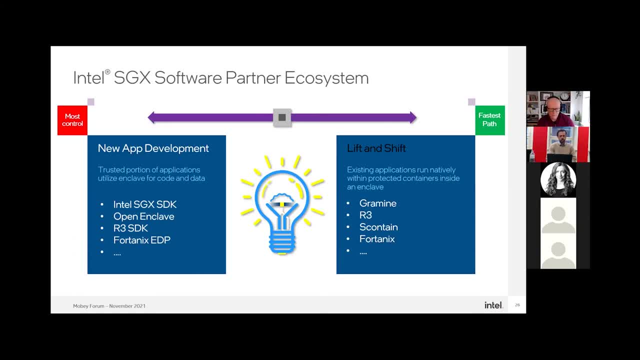 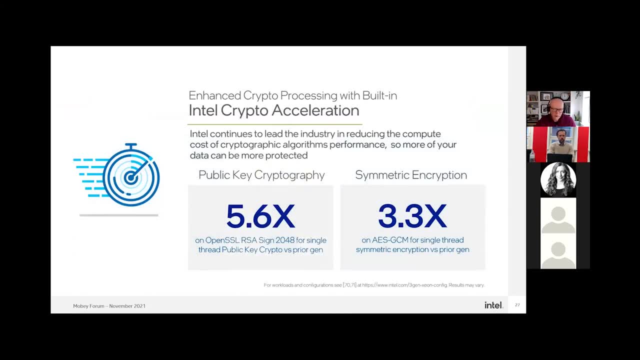 to the cloud as well, and we see this in the federated model as well, as we push secure containers out into federated nodes. Acceleration is very important for us. We're doing a lot of work and research into making stuff faster. You can see some figures there. 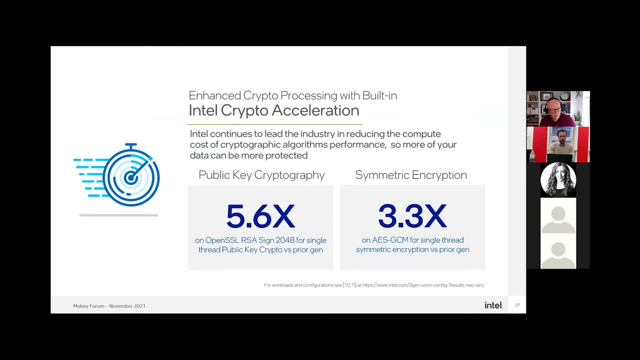 Our home office encryption team are working hard to address some of the scaling problems that are out there with home office encryption. So we see HE as something that's going to be very important for us in years to come. So attacking that scaling issue with home office encryption is something that we are 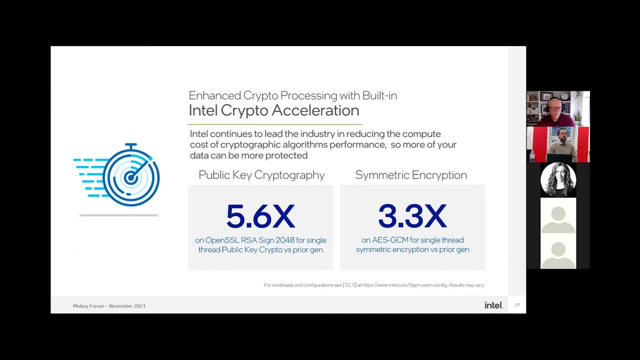 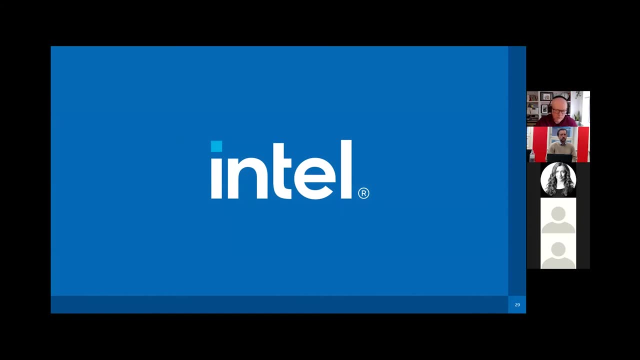 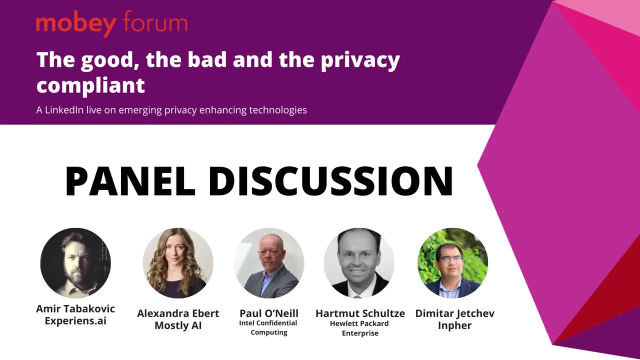 pushing hard to do as well. over time, We realize that performance is as important sometimes as security from a business perspective. Again, that's feedback from our direct clients out there. I think I'll finish there, Amir, if that's okay. It's a topic we could talk about for quite a long time. 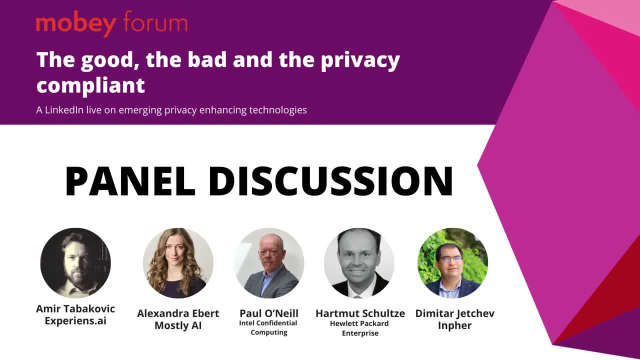 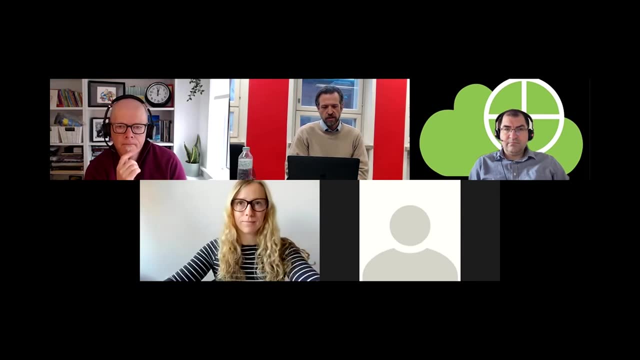 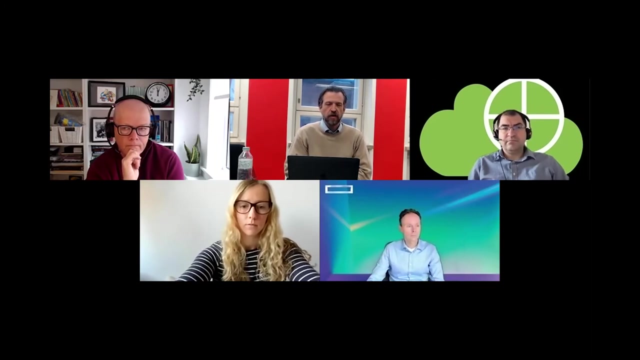 Amir Duggana To quickly introduce or reintroduce a little bit. Amir Duggana. Thank you very much for the panelists. So we have Alexandra Ebert from Chief Trust Officer of Mostly AI with us. We have Paul O'Neill working at Intel, Hartmut Schulze, Hewlett-Packard and Wigter Jetschek. 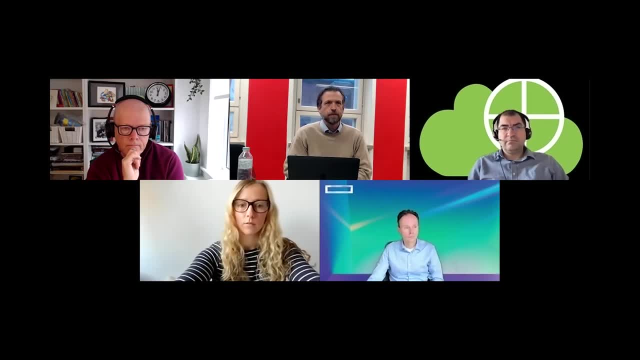 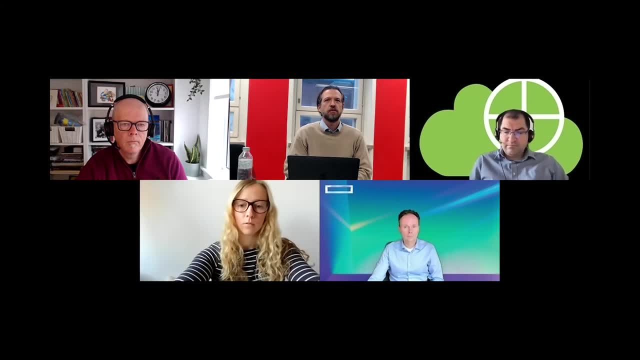 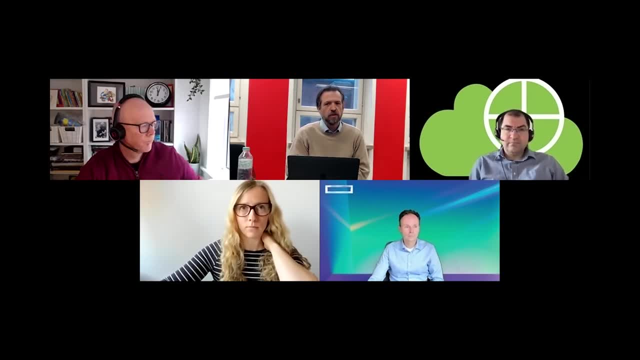 My first question to all of you panelists is basically that, something that I just received as a comment from one of my friends who is following here, and what was interesting about the results. what he says as an expert in digital banking is rather a technical event for Mobile Forum. 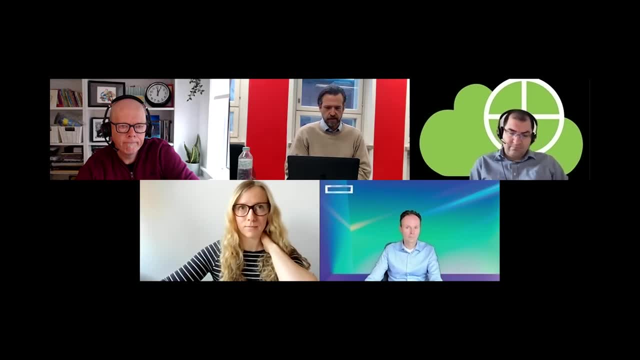 So the impression from non-privacy experts in the bank is that emerging privacy enhancing technologies are very complicated. There are many of them. all of them kind of seems to emerge in the same time. It's very difficult for a non-privacy experts to keep up. 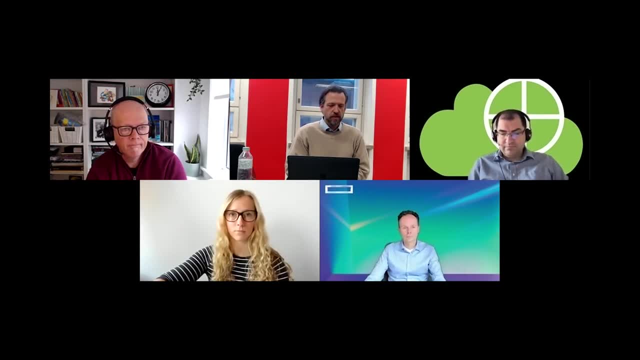 although there is a high need to have a privacy by design applications within the organization. So what are your favorite tricks or analogies that you use to explain to non-experts, your favorite privacy enhancing technology? Maybe, starting with Alexandra, I would say my new favorite one. 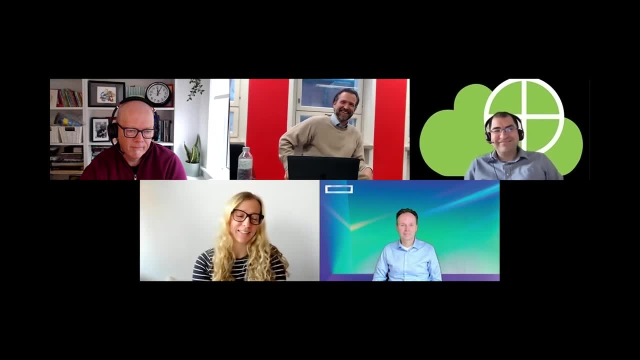 is the one we just heard today, with creating the necklace in the box. But for synthetic data, I mean, if it's very high level, then some of the analogies that have been used in the past where, like, imagine it's a super rich cake. 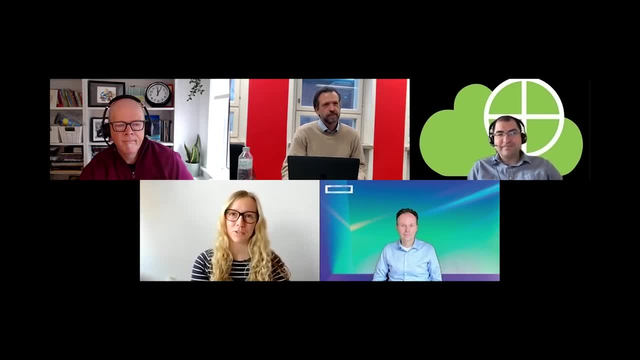 but without the calories. So you basically have the data, but without all the privacy pitfalls attached to it. And then, of course, the image example that I also included in my presentation usually helps quite good if you're talking to the not that technical audience. 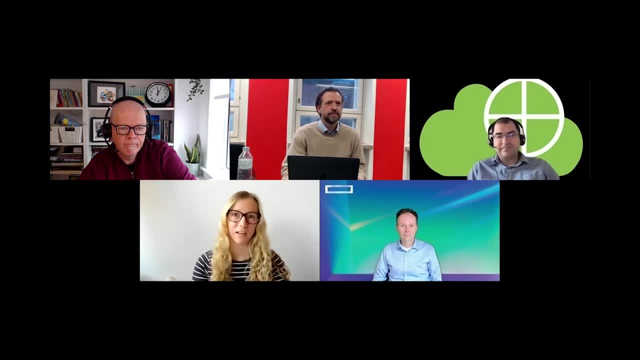 because you can easier assess that an image looks realistic, as opposed to looking at millions of tables of your customers and millions of rows in the table and see whether they are as representative and realistic as the original customer base. I think you're still muted, Amir. 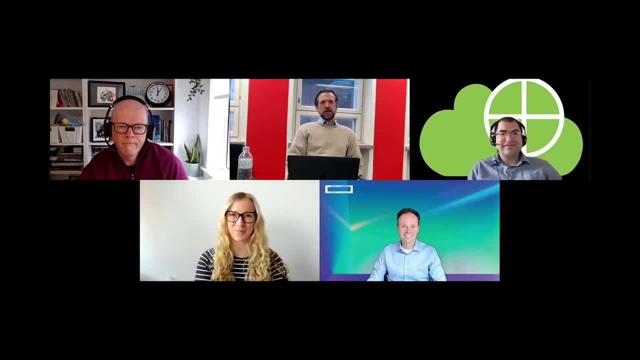 So, unless I should pick the next person to answer No, no, Thank you for reminding me. So, absolutely Yeah. I mean I've seen your presentation and you were not the only one using the analogies: Dimitar was also coming up with this box of gold. 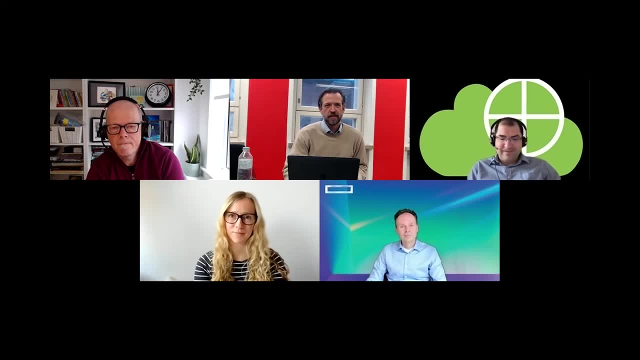 So interesting. take on that. Hartmut, what's your take on that? federated learning? Yeah, federated learning. Well, a lot of people have just the notion of: well, I need to share my data unless I can analyze it and learn on it. 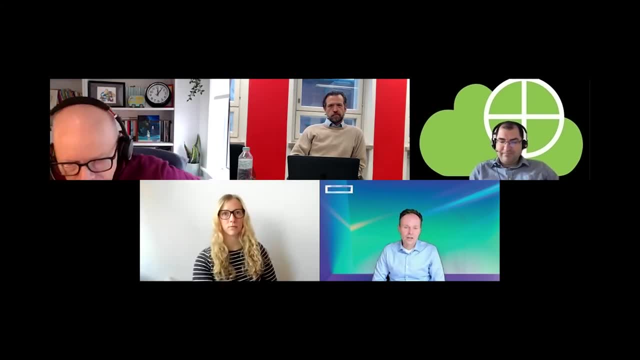 And that is basically not necessarily true. And there's this notion of: well, let's start with the problem. What is the problem? I would like to analyze And then really think through a data flow, more or less, So say: okay, where's the data? 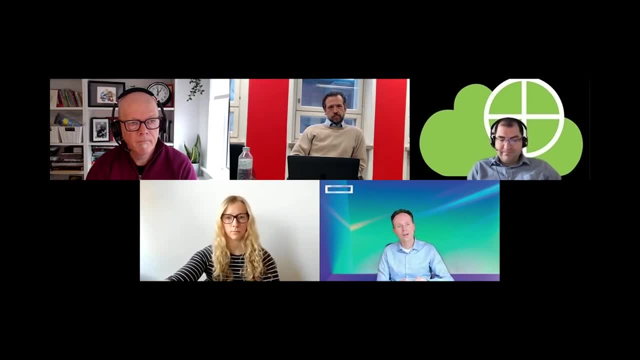 Where do I have to analyze it? Is it something really I need to bring together? Can I bring it together? How do I have to split it? Who are the parties? And then really to go on. well, sometimes maybe it's not even necessary. 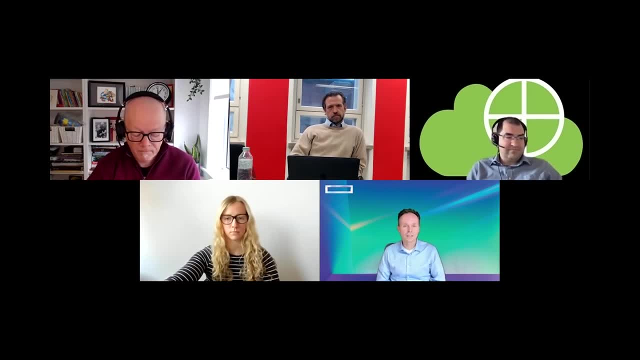 to get the right information out of such data, For having PII data as it is regulated like using synthetic data, for example- then have a subset first to a, as you said before, a filtering on data for preparation And then to say, okay, when I did the preparation. 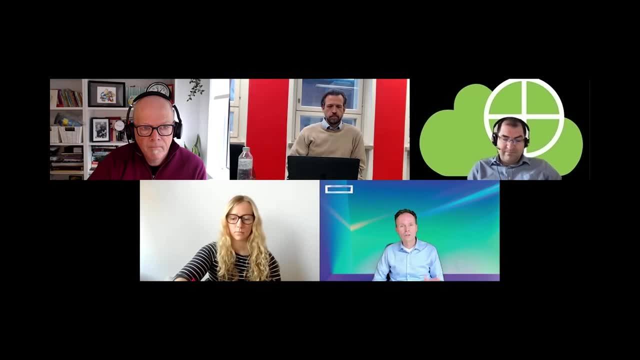 then I can learn the patterns and then I do the life cycle. And let's be clear: to have a combination of all these different notions, because we do need you know. to have a combination of all these different notions because we do need you know. 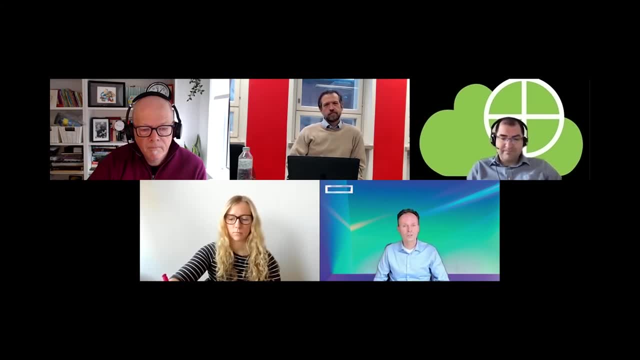 we do need encryption at certain points. We do need federation in certain points. We do need have some obfuscation or synthetic data And we do definitely need some to have the trusted execution environments. But the combination is always as good as the problem. 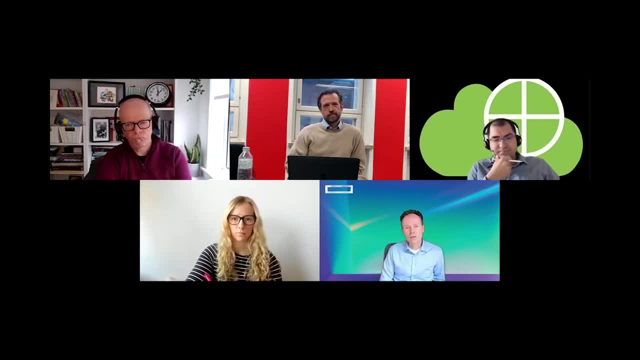 if I can describe it well, And a notion. what I see a lot is that people strive for going for the overall. I want to have all the data And I would say: well, the data is better. Think about the problem, Think about what you try to reach and then segment it. 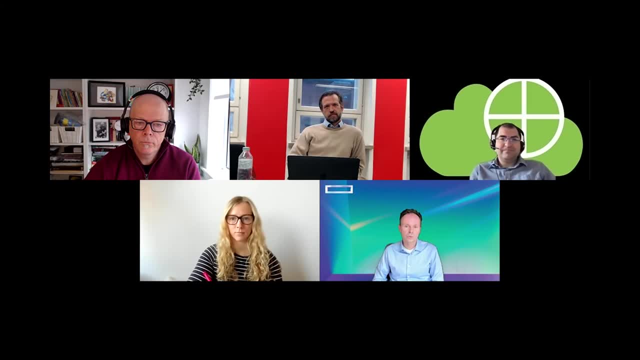 in the right way. And well, we have the tools. I would say It's possible to do so And we can share and can work together without really sharing, And that's how I would approach it. Sometimes, people are even benefiting already. 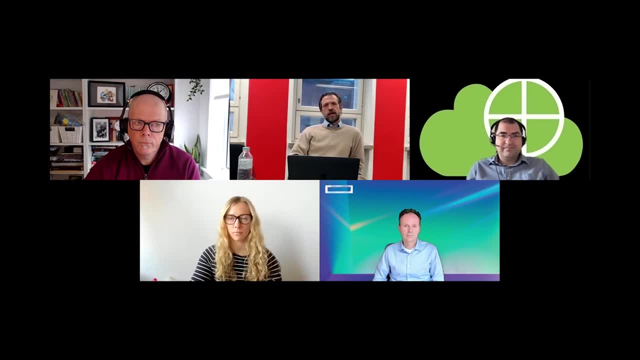 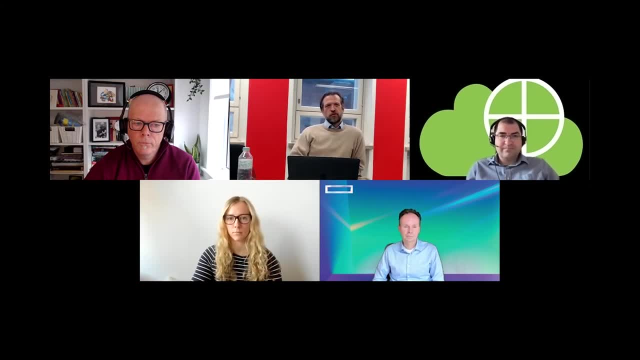 the you know, the you know, the you know. the keyboard is actually also based on federated learning. So it's those. you're already kind of, you're already exposed to this technology, you just don't know that. 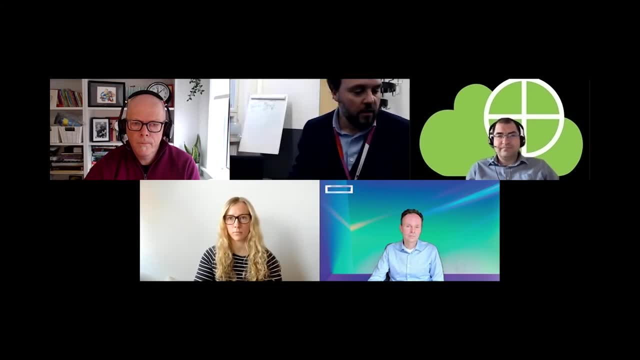 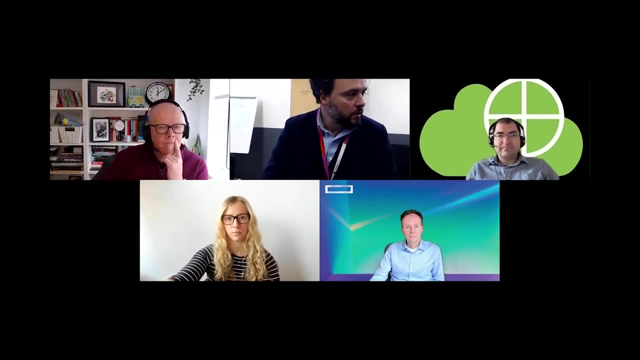 I have a question, then, on this. My question would be, as Amir just mentioned. I mean, today we saw you presented a lot of new technology and you're probably pioneering in each of those, But he just he just said something that came into my mind. 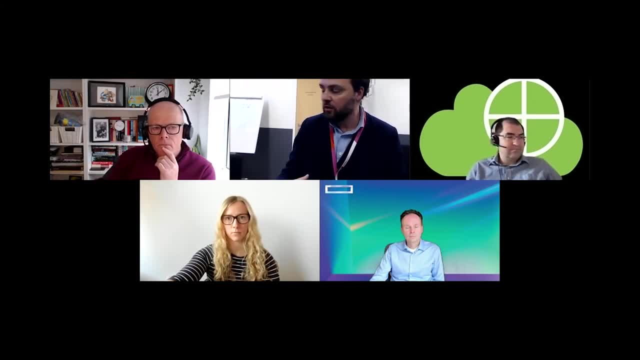 like you know, a use case which probably each of us are using every day and no one of us know that has been built with some of the technology you are you are presenting today. So my question would be: can you guys give some example? 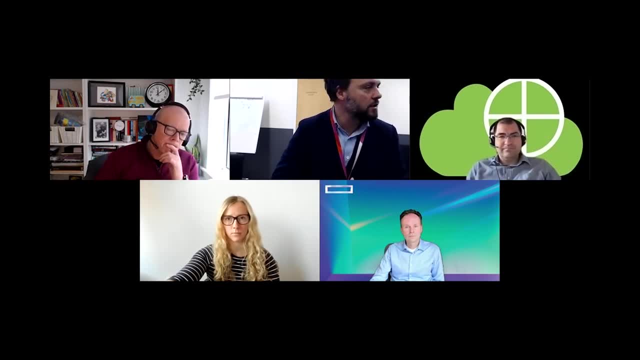 not on some research project, but something that lots of people are currently using, And and and. actually there there is one or the other of the technology you talked today, but we don't know about it. So maybe. so, Dimitar nodding, maybe you want to take that. 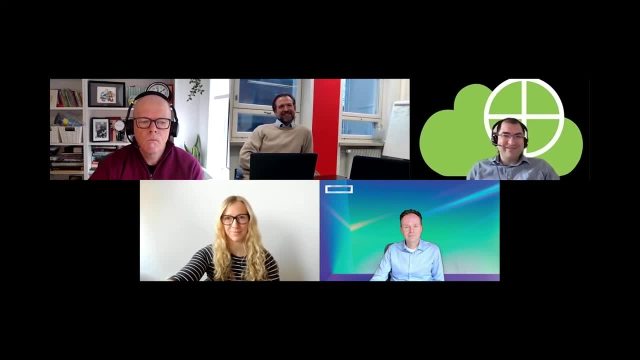 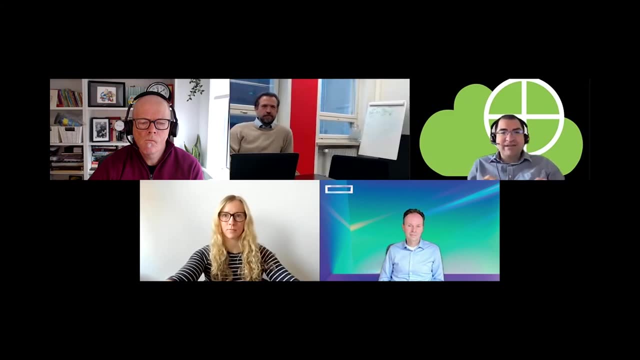 because we already saw your box with gold, So you're already trying to answer the other question. Maybe you want to take this one. Yeah, exactly, So getting to this one, what could be better than a show showcase for the multi-party computation? 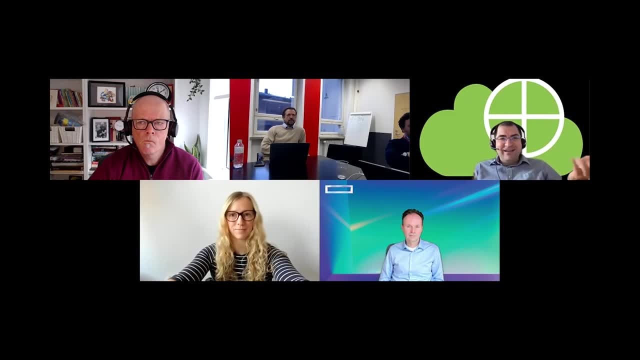 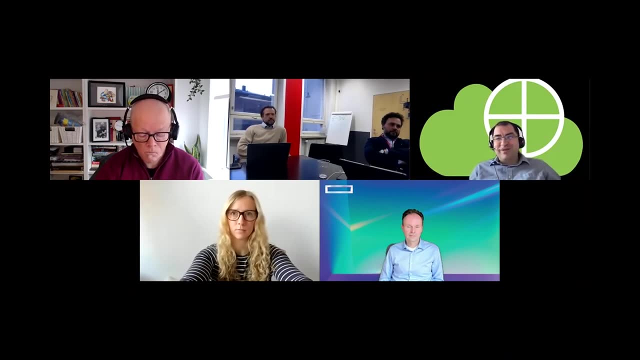 than the simple millionaire problem. So you have your salary, I have my salary. How do we decide which salary is bigger, Bigger, without actually revealing the salary, So revealing only one bit of information? That's for me, at least in the context. 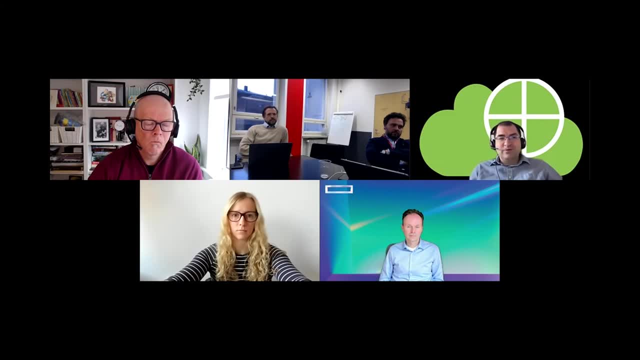 of multi-party computation. that's one of the simplest visuals, or like problems, that you could show to to to everybody. So, that being said, I would go to. obviously visuals are important, What we saw in a lot of the presentations today. 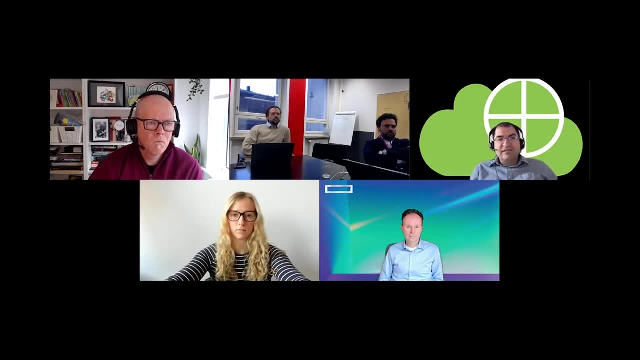 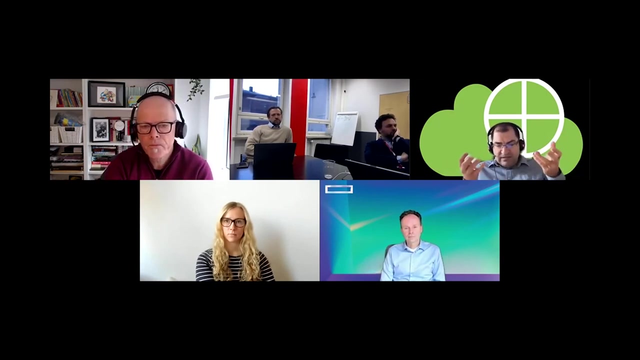 I think that that helps explain to non-privacy experts the the, the concepts. I should say that also presenting really basic use cases. So one one basic use case that goes in all of these machine learning models is non-machine learning data pipelines in privacy preserving. 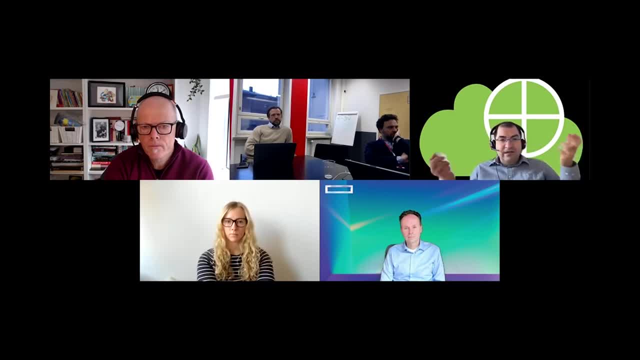 is actually the very first step, which is the data integration. So how do you actually integrate two data sets, two private data sets, Without revealing information? So that's the privacy preserving data integration inner joints of tables and databases. So there are obviously a lot. 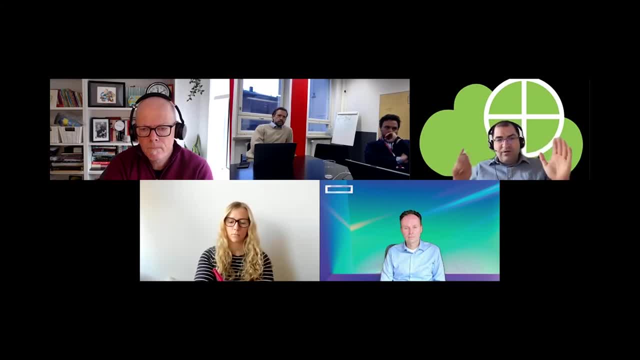 of non-trivial cryptographic technologies underneath. but you could. you could just show the the problem. You could show like an Excel spreadsheet on one side where you don't see the numbers and another Excel spreadsheet where you don't see the numbers and you show how you could. 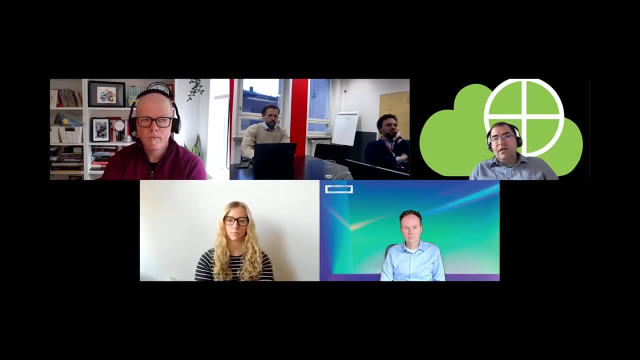 you could integrate them. That's your first step. before you, you go down the machine learning pipeline, Also intuitive APIs. that's very important. So when we build demos or products, it's really important that data scientists are not changing their flows. 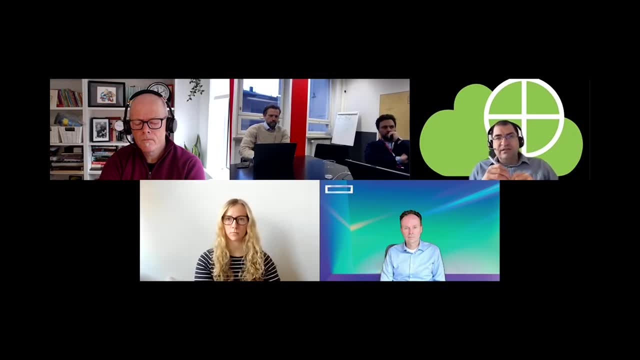 They can see how how these technologies can be used within their existing flows. So graphical, graphical APIs or programming tools there. these are going to explain a lot, the use of how these technologies can be integrated. Yeah, Yeah, I think let's make one point here. 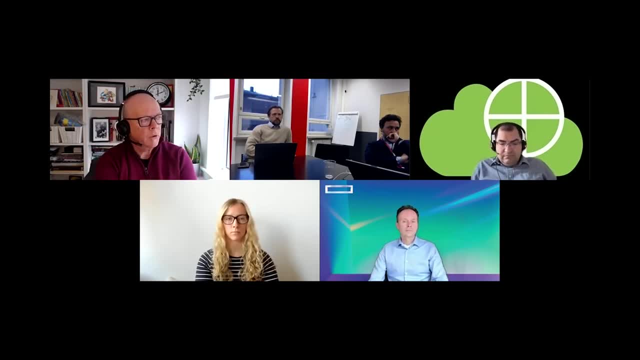 You know I get to speak to a lot of large enterprises pretty much every day and you know you can go along to a big bank and in that big bank you've got a team of people who are supporting secure multi-party computation. 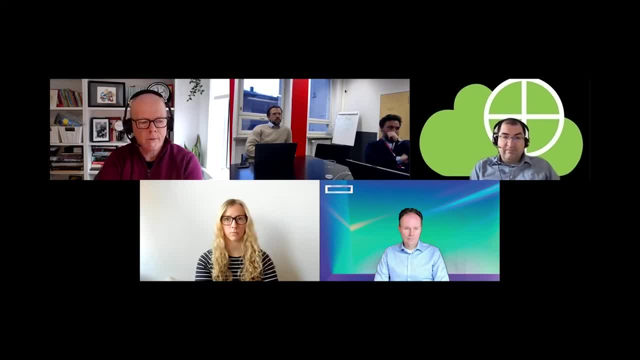 You've got a team of people who are supporting trusted execution environments. You've got a team of people who are who are supporting HE and they don't talk right And they don't come together and they're making it super complicated for that bank to make a decision on that. 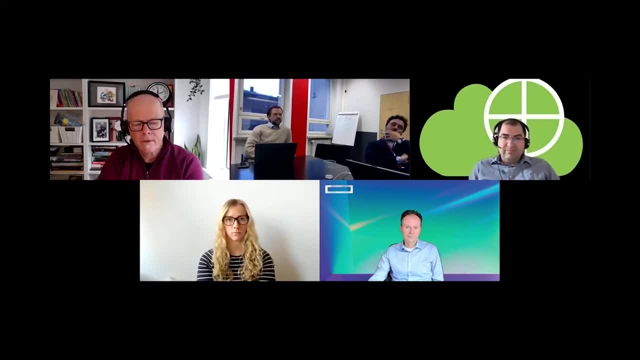 I think it's incredibly important to break those barriers down and show how these technologies work well together. You know: homomorphic encryption and trusted execution environments- potential match made in heaven, right So? you know, secure, secure execution environments, securing computation and securing integrity of computation- right so those two things so that to 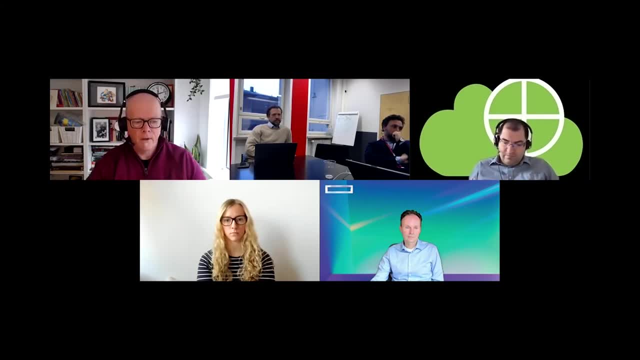 me is one of the mission statements that we are on at Intel is to show that you know we're not. we're not entering the pet space, we're building this environment. so privacy enhanced technologies can thrive in both a centralized cloud perspective and a federated model as well. to me, that's super. 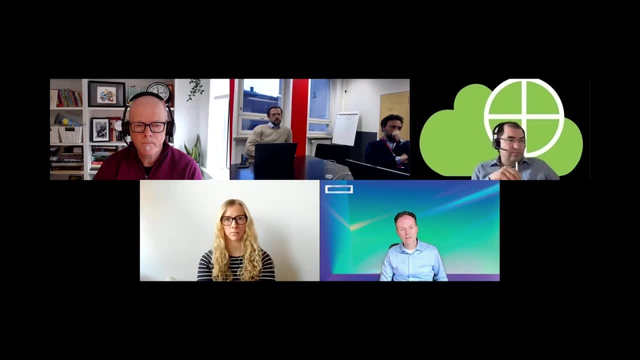 important and maybe, maybe, to add to that. uh, I think it's, it's important that we have all the modules, I would say, and there's no one size fits all solution. it's always the, the issue, the problem the customer tries to solve, and then really to go to the, the minimum part and to extend over time. 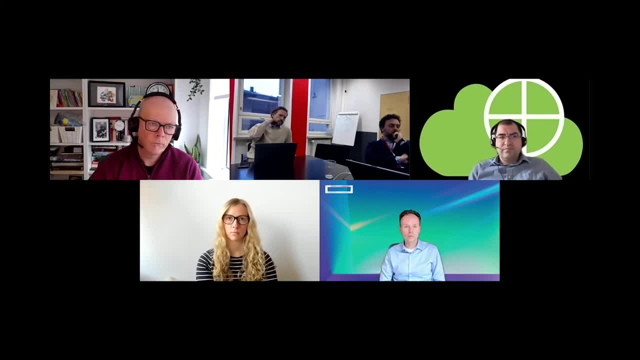 and I'm pretty sure that we have the technology already in in hand- not in the right combination, though, uh, in in the beginning, and it's not a one size fits all, that's, that's for sure. but we can build this together, because the modules by itself are getting better and better and working better together, as, as Paul. 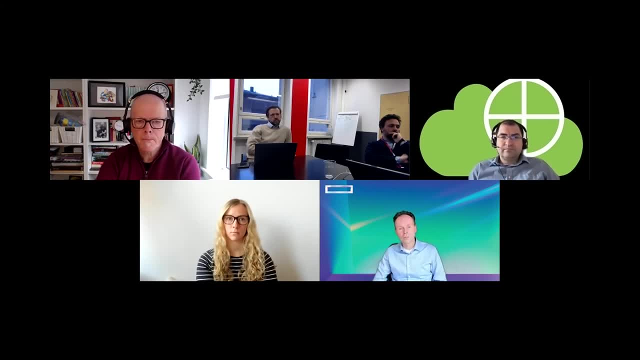 was mentioning going open source, going in consortias, going on. how do we actually build this? together is the only way to to make it happen, to build up the ecosystems. uh, for what Dimitar was was beautifully showing in getting the AUC to one is the ecosystem I mean we need. 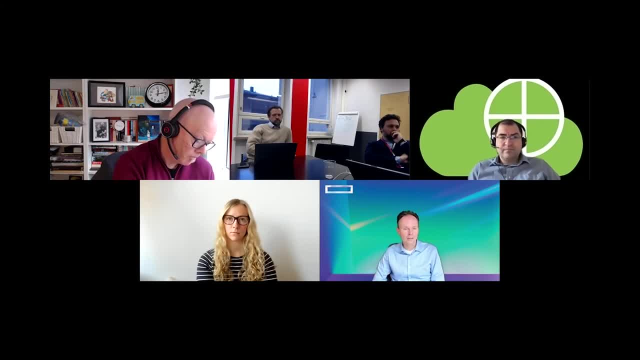 to do that: building modules, take, take the different things and uh at at best, talk to the, to the people. so I find this extremely important: what you, at mobile, do, uh to bring those people together and think about what is from maybe different domains, what is the solution. 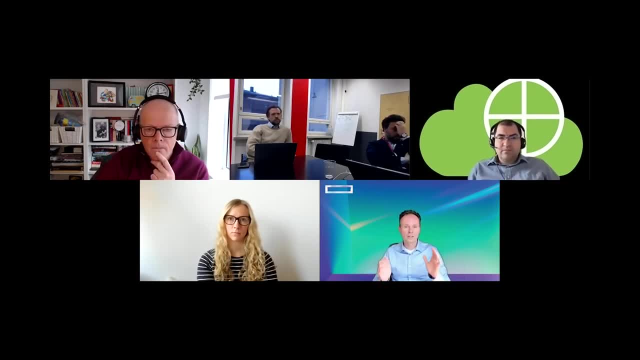 approaches. what is the real, real problem? for example, histological data. there's no private information in histological data. if you split of the metadata and it's agreed that you can analyze this on computer vision, so you circumvent it like you do it with with since, since that's what you're. 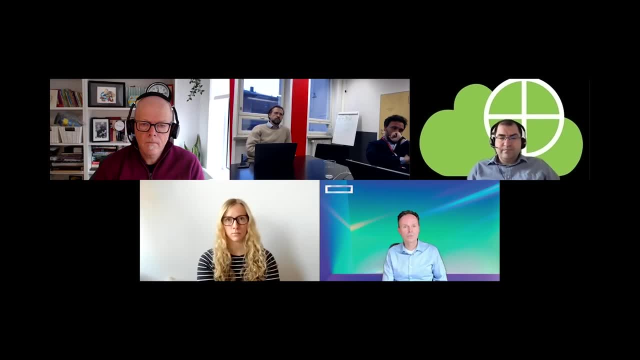 doing with static data. the principles, though, is the same. you, we approach the problems and say, okay, how quick can we circumvent good regulations? sometimes because none of us obviously wants to know a complete tracking of all our PII data, but, of course, talking to other domains as well, 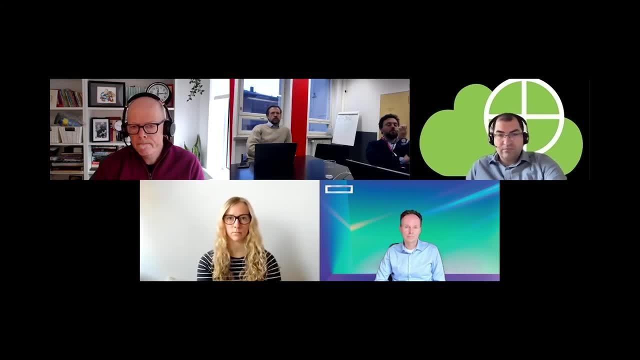 is helping a lot and therefore we we need to work together. yeah, what you mentioned, uh, regarding mobile forum, uh, how come it's interesting to follow? you know the the history we were dealing, for example, you know we're looking at at building uh mobile wallet ecosystems 10 years ago and and that was also the that brought in different 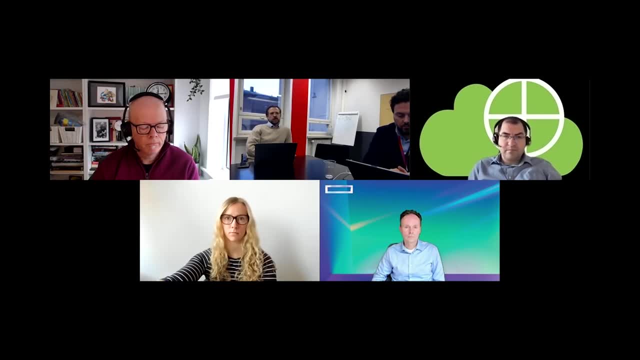 stakeholders coming up from different angles with different Technologies. we we had to identify different control points to build a mobile wallet solution. interestingly, that was 10 years ago. we identified data as one of the control points, but we didn't know at that time: is that even? 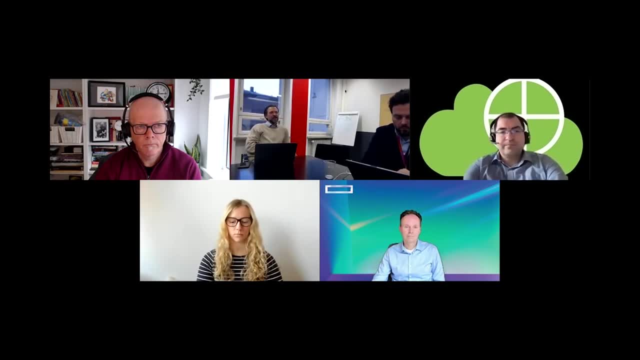 this control point has further controls points behind, and the privacy is probably one of them that we have that we didn't pay attention in 2013, when we're publishing these kind of papers. so so this is a learning curve. this is a journey where I think we all can benefit from this kind of exchange. 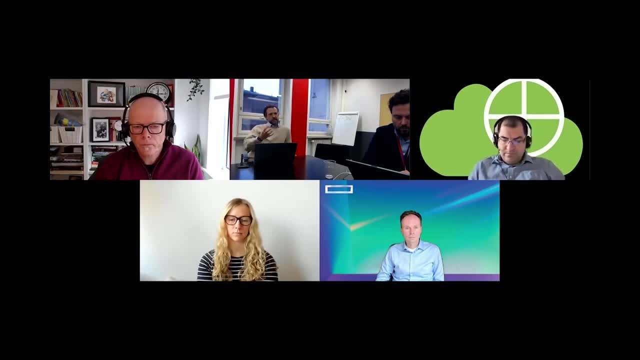 what I'm wondering is: when you're coming from the, from the technology side, and you're approaching non-experts who are maybe, you know, subject matter experts in banking and retail banking, um, how are you basically, how are you able to track their- you know their- pain points, their, uh, the 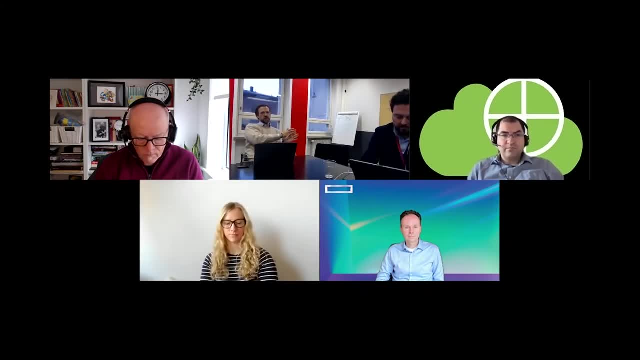 business value to your specific technology, because obviously there are different alternatives. you can go with this or that technology, you can um, you know, how can you? how do you approach that? uh, let's start with Paul. this time he was yeah, I think. I think the challenge for us was a little. 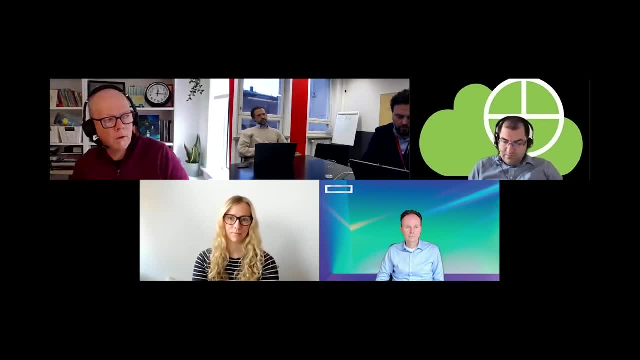 easier than than the others, right, and maybe, uh, maybe, it's the same for Hartwood. you know our customers wanted us to help them move to the cloud, right? so they just said, hey, you know we can't continue to, uh, do some of this stuff in data center. we've got to move it to the cloud, and that was the. 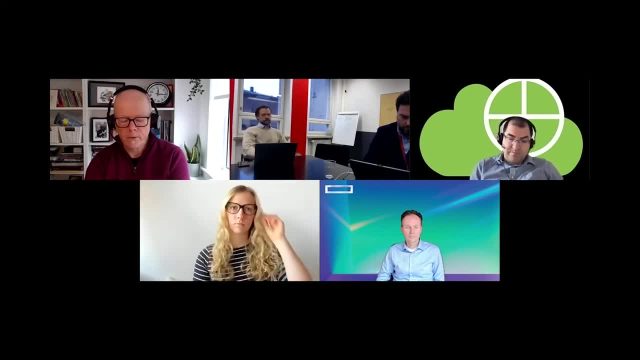 problem that we had to, that we had to solve for them. now, you know, by using trusted execution environments and bringing that confidentiality, integrity and privacy into the cloud- the three things I mentioned there earlier. on SGX and our trusted execution environment is effectively a developer toolkit. I was open about that. 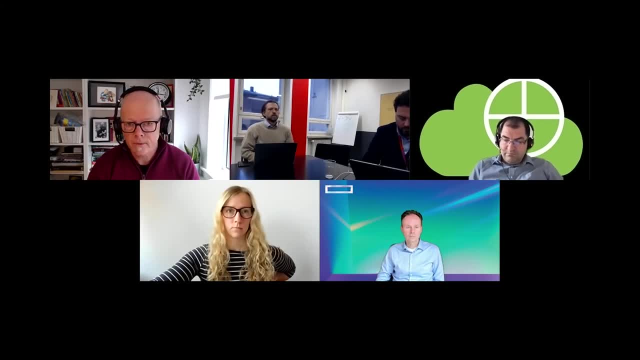 so the only way that we could help our customer base was to sort of grow this ecosystem around us. so with our capital arm, Etc, starting to invest in companies to raise, to try and float all boats around bringing privacy enhancing Technologies to the cloud. but we've always seen this as a cloud. 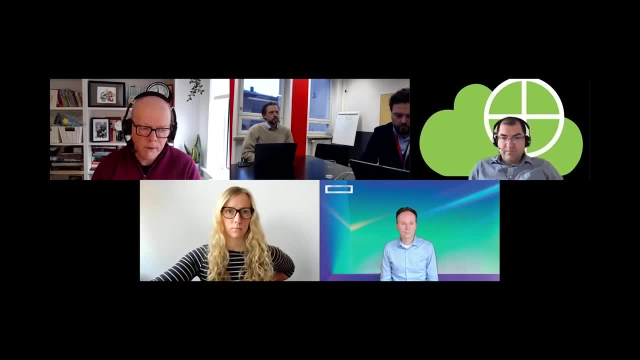 play, and it's only sort of more recently that we're starting to dip our toes into more of the federated learning work which we've done a lot with with the HP uh, also as well, but for us that's how we sort of um moved it in and that's how we brought our customers. let's get to the cloud and get you. 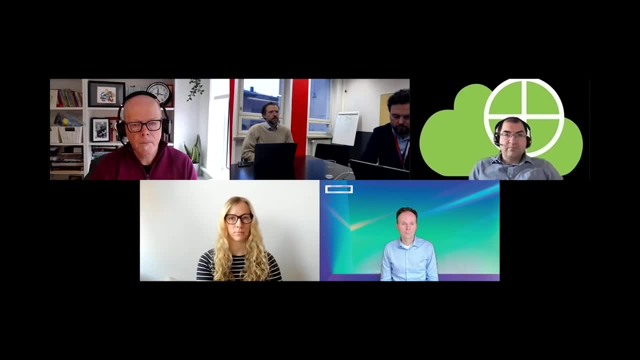 guys playing with that cloud economic models with sensitive data sets. thanks, Paul. how about you, Dimitar? how are you facing this challenge? yeah, that's a. that's a great question. actually, that's uh. so here I'm going to talk about two different aspects to two different scenarios. so the first scenario is we all talked about. 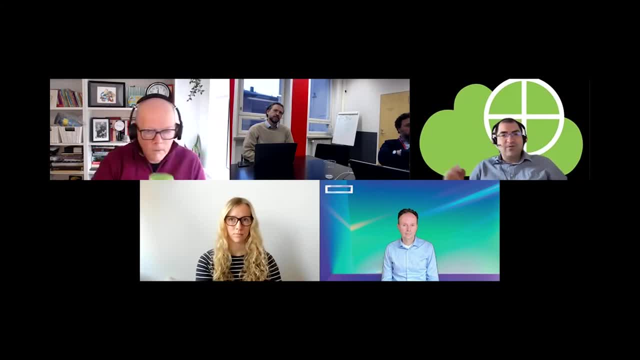 improvements. so we say we can improve accuracy by 20 percent. uh, for credit scoring. so that doesn't mean anything to a business owner on a customer site unless you have a solid return on investment model that could convert this into actual, like money that you're saving. so uh, for example in 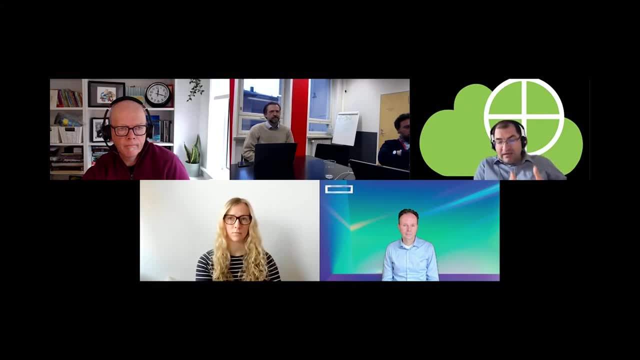 this particular case, like the picture would be incomplete if we don't have the uh credit risk model and saying, okay, if we improve uh the detection of that default credits by 20 percent, then that is going to translate into um like X amount of dollars less for the bank and then a. 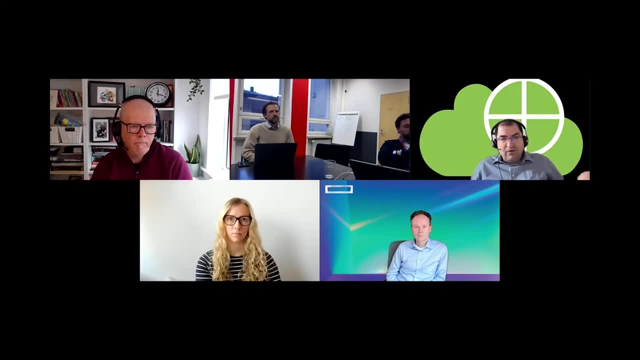 business development uh person who, who doesn't need to even know anything about machine learning, could, could, could- see the actual value. so the other uh scenario that I wanted to talk was use cases that actually did not exist before, that were not possible before without this technology. so this technology is obviously an enabler for newest cases, not just machine learning model. 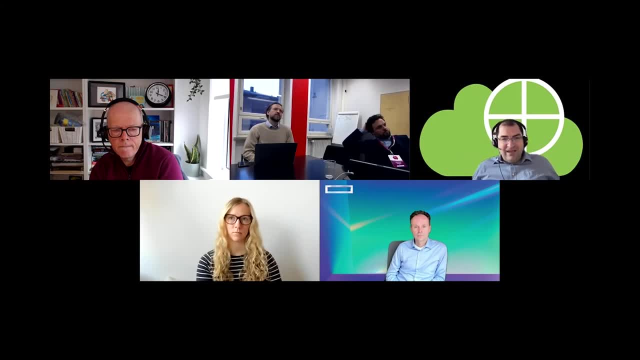 improvements, but you're not even able to run the model due to GDPR if you don't have it. so that's the example, for instance, with uh cross jurisdictional compliance. so in that in those cases the business value is more clear. they are just like forced to. so the 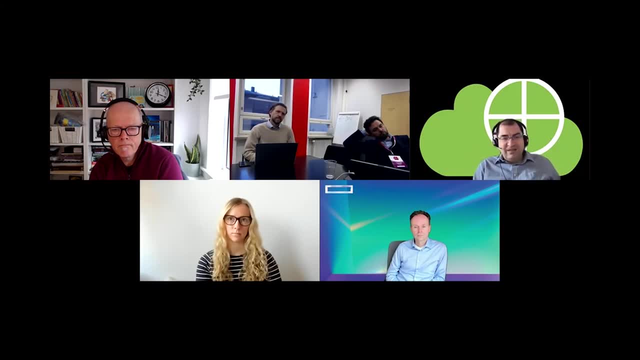 user uh needs to uh, uh needs to have a solution that enables this use case. so this is typically our approach in these two scenarios. there are other scenarios, obviously. coming back to the second approach, isn't it challenging? because you're, basically it's a two-step approach. first, 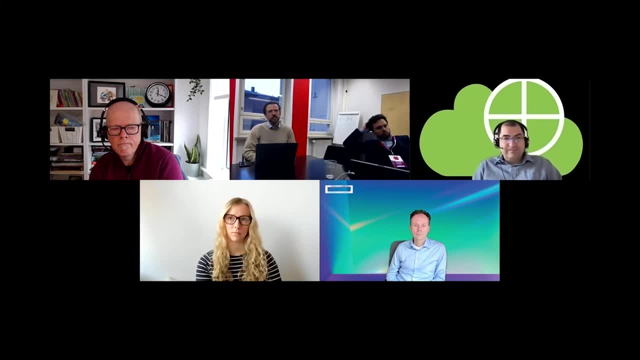 you have to sell them, you know a use case for itself, something that they believe is not possible. so you're basically, you know, entering the world of, you know, retail banking practitioner and are convincing them that they should start using AI, machine learning, for something that they believe is not possible to do without mentioning 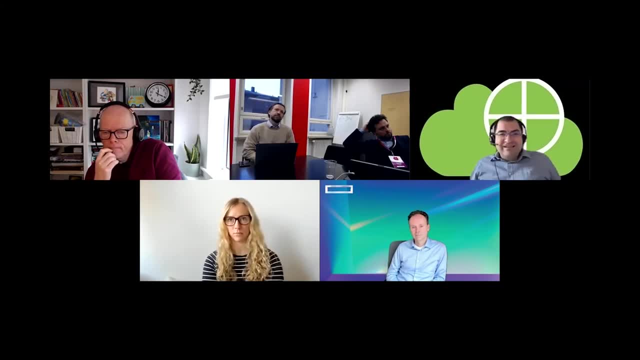 actually, you know your, your technology is coming in the second step. so so that that was true in the very early days of the market. I agree with you, Amir, so that that was what we were seeing in the early days. but as the market matures, uh, the banks are starting to. 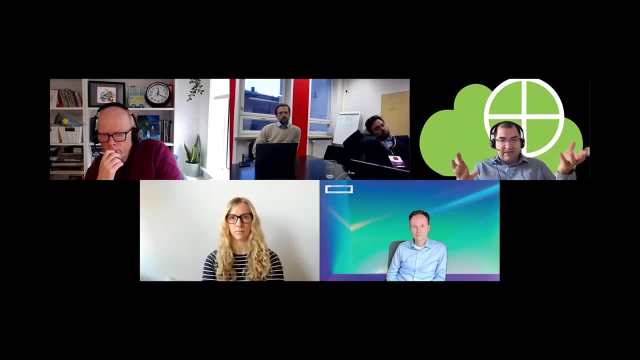 actually realize the use cases by themselves, which is the, which, which is really a good indicator of the market, exactly where we want to be. and then they said, okay, we cannot support these keys because we don't have, uh, privacy preserving technology or privacy preserving solution for the computing. so 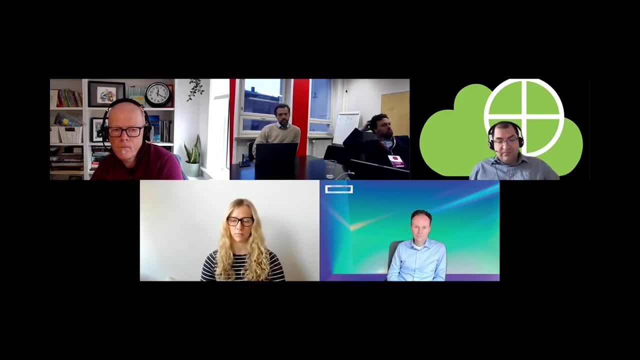 are you able to provide us this solution? and it's, it's done when we step in. so this is the much more clear uh uh indicator that the market is really maturing. what about you? are you sharing this opinion? what's your take on on the business? how to get? 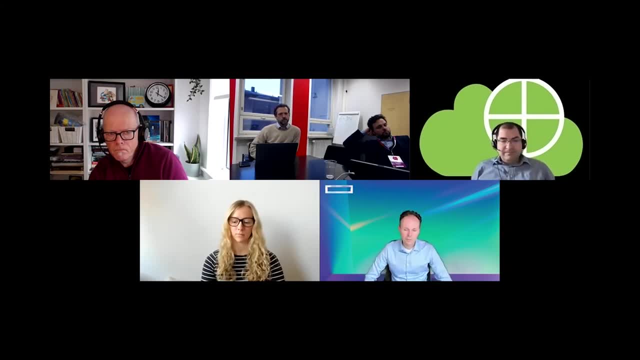 the prove the business value. yeah, that that comes a bit from my history. I I come out from the account management and do business development, so actually I was listening to the customers all day long. uh, so what is your problem? how do we actually solve this and what is the technology? 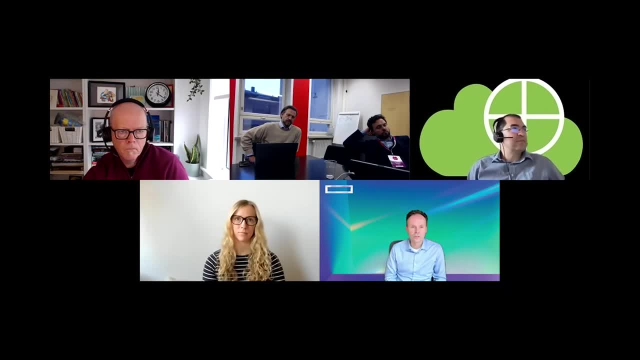 to be deployed. and the interesting thing is: uh- and that's that's what I typically always do- is listen, just listen. listen first, not not thinking about a solution. move off the solution how it's how we say it all the time. move off the solution, listen and then prepare and say: okay, what is the 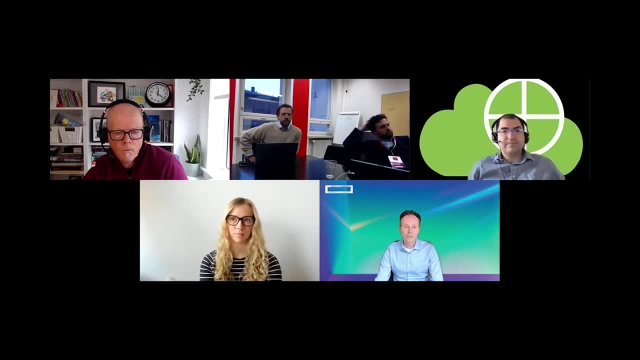 different components and what we actually will try to solve and, as you will just mention, the innovation dilemma of crossing any Chasm we have here on the world. how did we deploy it? yeah, we need to educate the people. we need to make proof points. of course, we need to make proof point that 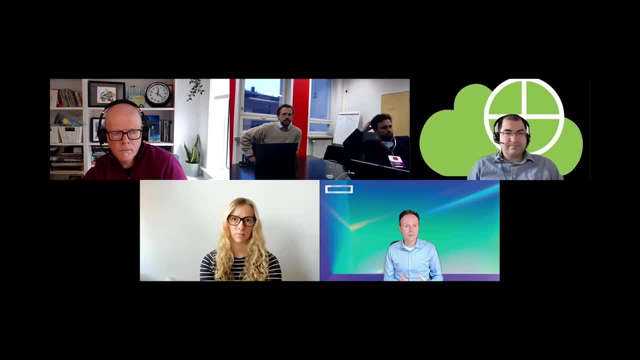 something is possible, something is happening, and then these modules build out and somehow I have the feeling- at least that's, that's that's how I see it, but of course this is a bubble in in which I live as well. uh, knowing a lot of Technologies, now, uh, to build these together, and only the 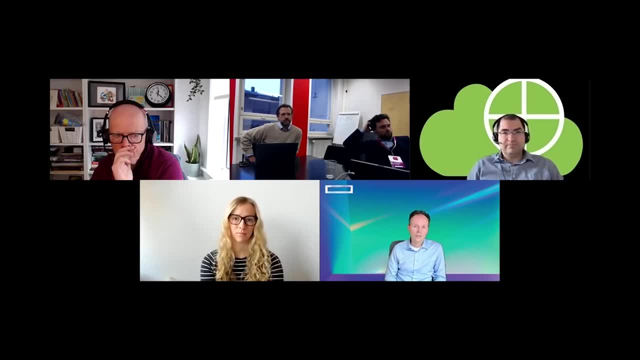 combination of those are really bringing it to to value them. looking at business problems typically, as the major was just mentioning is it's it's. at the end of the day, uh, there needs to be either a cost savings or a a revenue generation and additional services which we can provide, but then the way to get there is is different. of course it's it's. 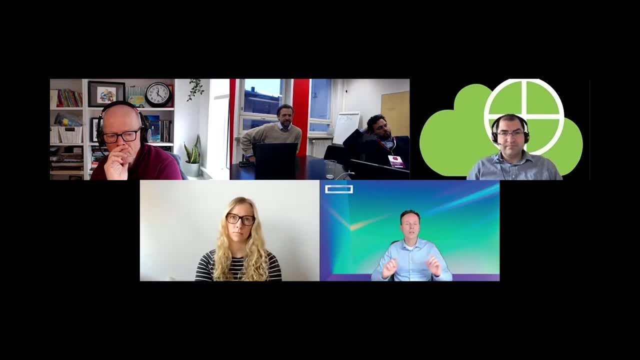 centralized, it's decentralized, it's it's different parties, it's organizational, it's processes, whatever. and then to have these, this, this bunch of topics, what we actually have to try to to to solve for, but still come to this very much and specific problem the the customer has, and that is then 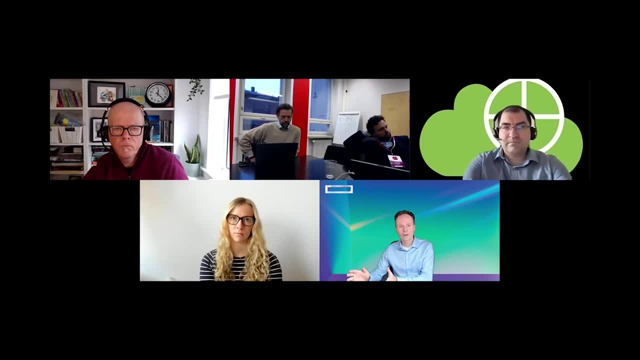 for example, as was mentioned uh by Paul, fraud detection in uh car accidents- and then to say, okay, which data do I need? and then it's the data pipeline. so start from listening first and then try to figure out with the experience with with a group of people, of course, because nobody and 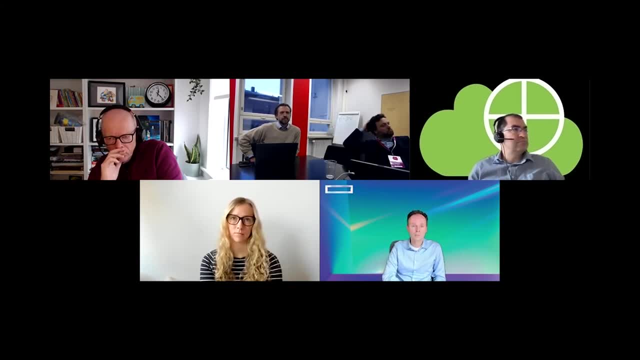 I'm absolutely convinced that nobody of us can solve everything by him own, by by themselves. it's not possible anymore. and, uh, it's. it's a combination of these people coming together and then think about it and and find the right solution. yeah, it's an it's. 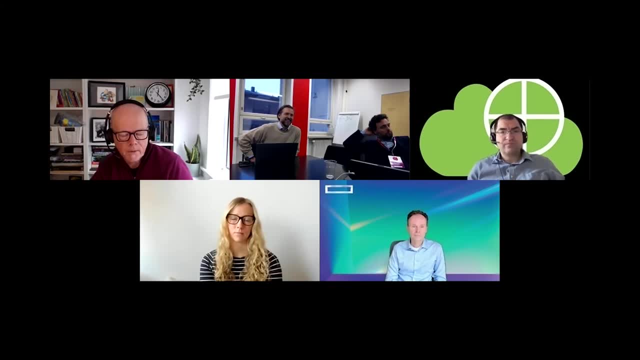 an early Market still. I don't know whether uh Alexander and dimitar agree with that, but it's an early Market still. really, we're looking at uh people who are doing digital transformation. maturity is still in a sort of innovative stage. privacy and security is proactive. they 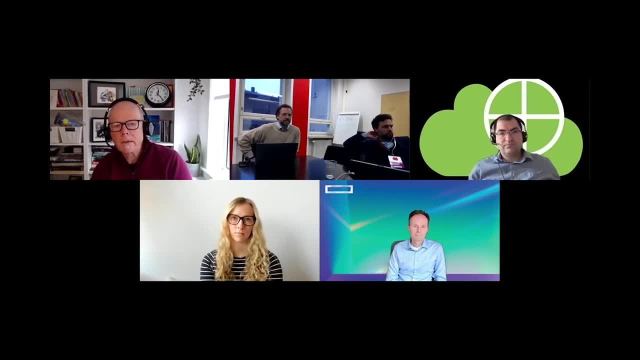 recognize that there's some problems that need to be solved and they'll likely know how to do it, but it's still working with early adopters and visionaries. um, as far as I can see, yeah, great, yes, how about you, Alexandra? where do you start? do you start explaining the difference between? 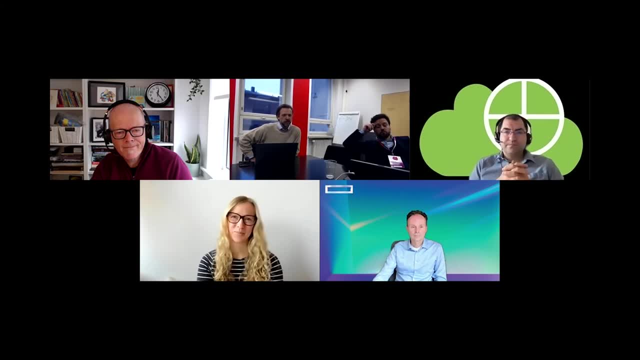 anonymous and pseudonymized data, or you know, is it, or already? are the customers so mature that they know what? uh, what is it? what is the benefit? that? that definitely depends to whom you're talking to. some people already know, but I actually start the same way at hard mode does with listening, and then usually it is rather 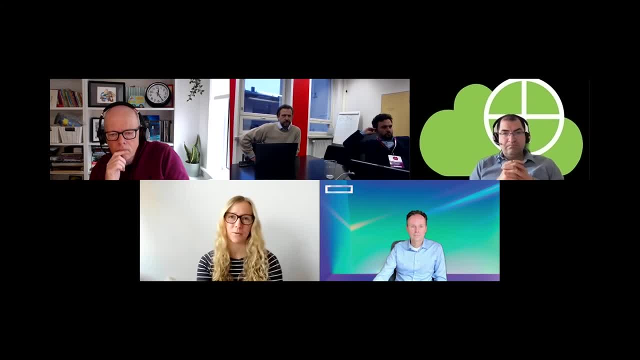 quickly that it turns out whether, for example, data sharing cross-border is one of the biggest pain points for the counterpart, whether it's AI training or in which different areas uh synthetic data could play in. but I can only second what Hartman said. uh listening first, I think, is the 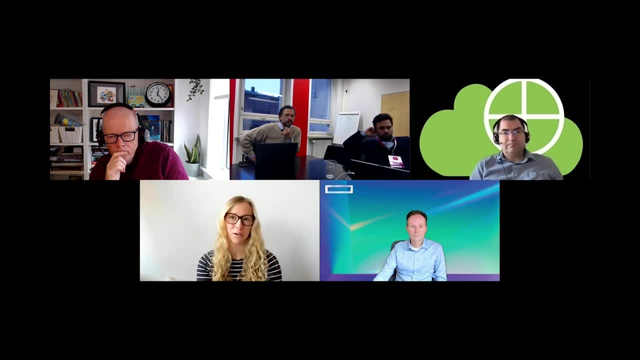 best way to go and he also shared that on the one hand, you don't want to have a cost reduction or an impact on the bottom line. more and more I also talk to people for whom it's really this overall risk minimization because with the GDPR finds and the proposed AI Act finds we're really reaching. 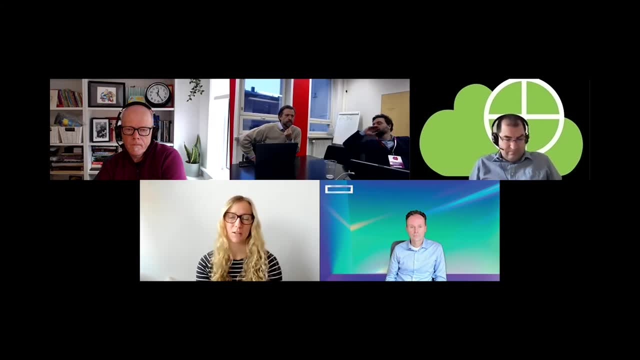 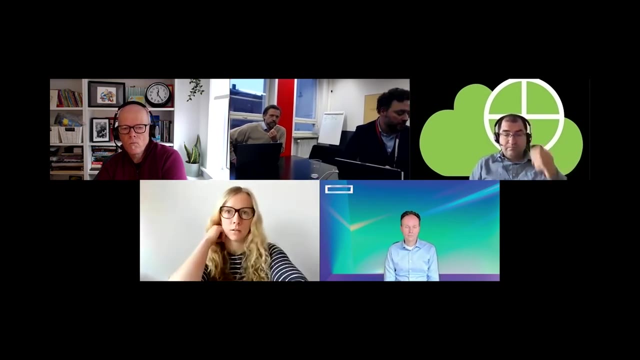 very sensitive amounts and therefore risk mitigation also is something that's a concern, depending on which department you're talking to. okay, I have a question. so, yeah, I have a question. um, um, looking, looking at the big Global Company that apparently having their business model built around data- you know, Facebook, Google, all the 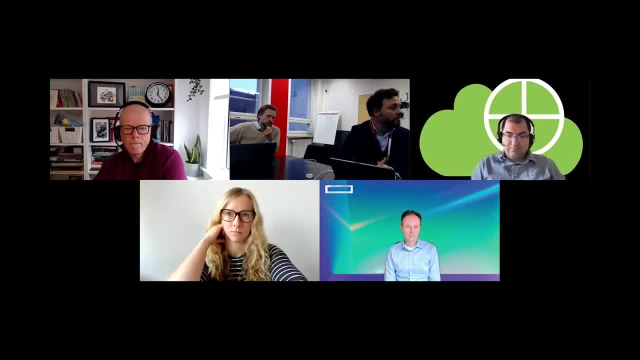 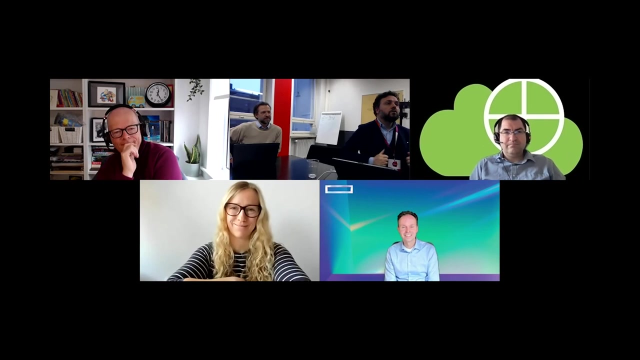 huge Global Company, which one, in your opinion, is the most advanced on the topic you just described to us today? and on on which part of that business may I ask a question? in what respect? in respect of technology Advancement or in respect of ethical and trustworthy uh? 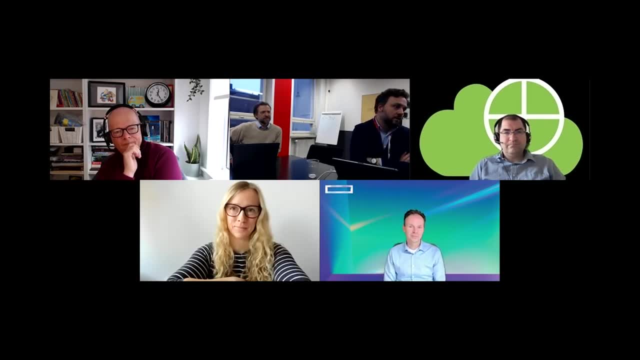 uh, uh, uh uh in respect of trying to be compliant with the privacy and, at the same time, continue to generate value out of data, because that's what they are doing, right, they are most of their money, especially the one dealing with advertising. they're dealing with data, and so I guess they have the same privacy. 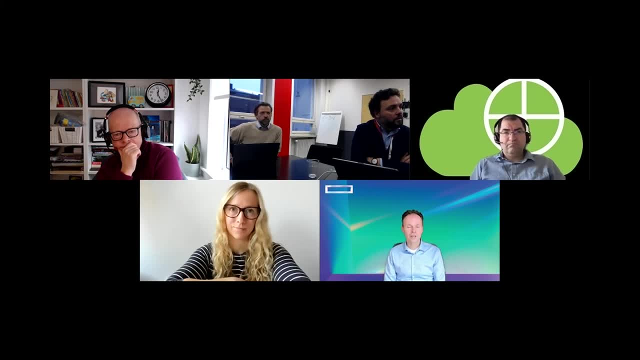 issue that anyone else has right, or you think that they don't? uh, they don't act like that. I mean, Neta is the best example on that. uh, so any any Monopoly which is going in that direction, which is now getting into a potentially political discussion? 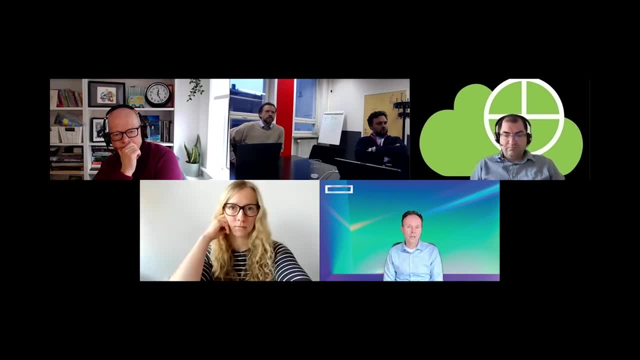 but nevertheless, any Monopoly is not going to strive for that. so we need this regulation in a certain way on safeguarding our privacy, and the technology is there, but it needs to be applied ethically, and I'm extremely convinced about that because, uh, we, as humans, we have so much bias with. 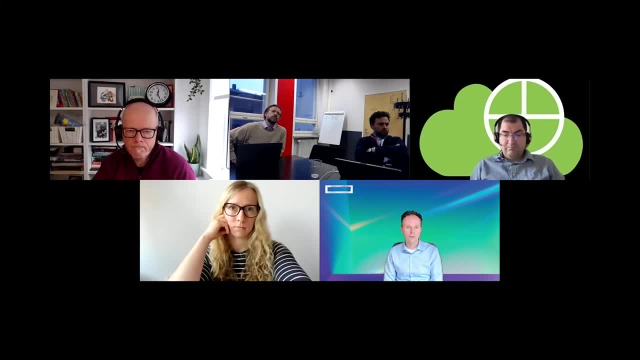 within us. so we must also take the right measures of getting that bias out, and that is something we have to really do, and there's- there's- only the society who can actually work on that. uh, it's not the technology company. so I don't, I don't believe and I don't trust any Monopoly or 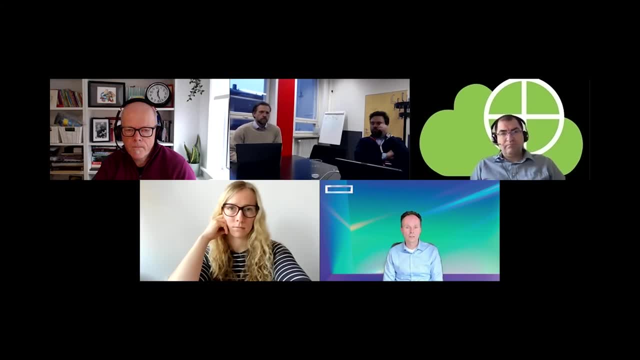 any kind of technology Advancing, uh, without doing that, and let's face it, I mean, these are the, the big ones, uh, and it's always a a strife of getting how. how big is good, of being system relevant or to be the well regulated and then, uh, hindered to apply and deploy technologies which might be counterproductive. 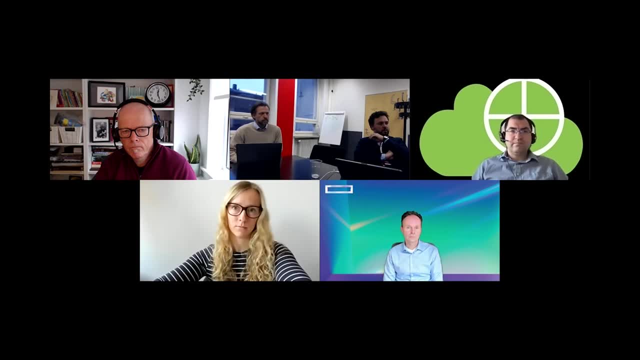 so what you, what you are saying is that the big player, the big global data driven company, are not working with the technology we were discussing today, mainly because they don't get up, they don't care about privacy or they are in a Monopoly situation where this is not the point, that that's not what I'm saying, but you just take the, the meta. 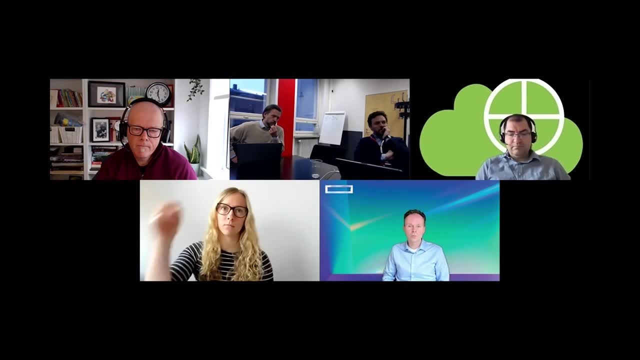 discussion we currently have uh right about how much. what is, what is their primary North Star? where are they leading to? are they deploying technology for good or are they deploying uh technology just for exploitation? and uh, I I mean there's different companies uh who have uh a technology Advancement and do great stuff, but still have this struggle within a a large let's. 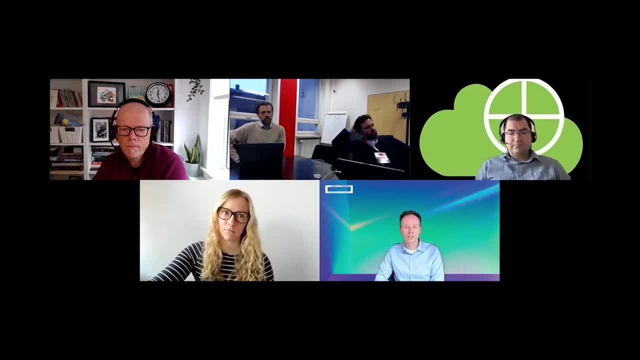 take our hyposcalers, let's take in in different jurisdictions if we go to China or Americas. we have different approaches here. this is, this is always this leveling out, and what I'm absolutely convinced is that the overall getting bias out. it needs to have a certain ecosystem working. 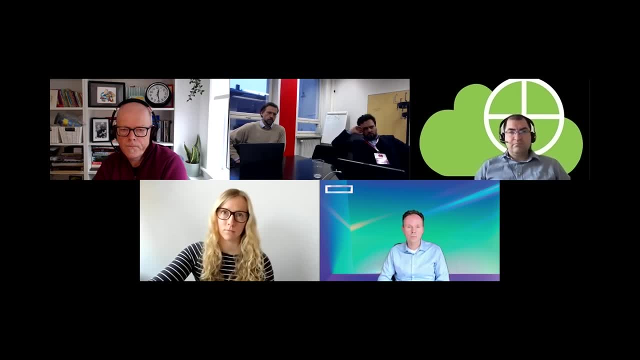 together and it's not a one can take it all or must be the central custodian somewhere. that is something which we need to uh well prevent. and there I come to the open source. I'm very much in in the open source space also, or I'm a believer of the open source, that we have the right connections. 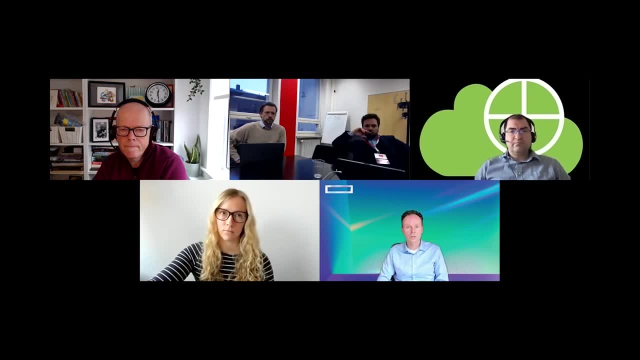 have the right combination of people and organizations working together to actually get the insights out of that. maybe the uh sorry, Alexandra, please. thank you, Paul. maybe to add to that um and to tomorrow's question. I know that two of the players already mentioned uh working and looking into synthetic. 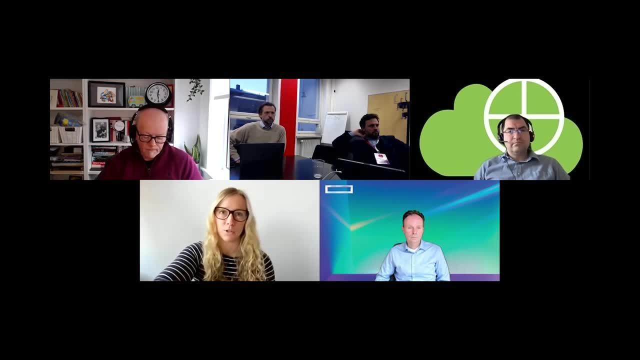 data. I'm not an expert on the other emerging Technologies that were discussed today. from some conversations with members of this company I know that they're looking in some Technologies but have diverging opinions within the organization in general. your question, I think, is easy to answer because from the 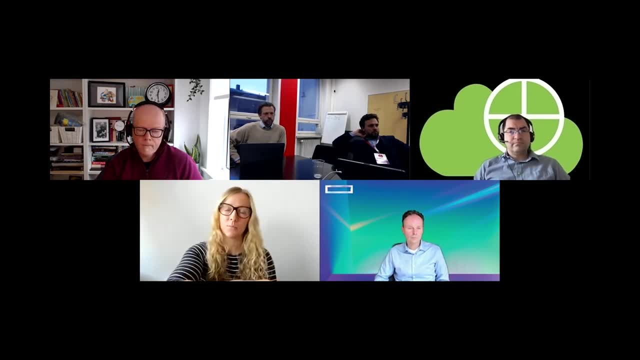 players. we have a few companies. they're not that dependent on exploiting customer data is the other. so, for example, the business model from Apple and also from Microsoft puts them in a position where they can actually use privacy as one of their USPs and competitive advantages versus Google. 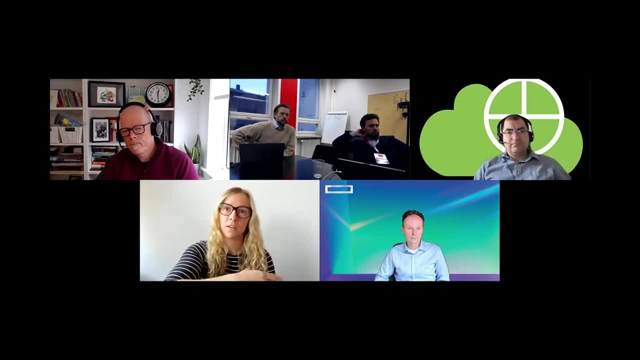 Facebook are maybe slightly differently positioned. so definitely for Microsoft with gdpi and this increasing regulatory complexity. we tremendously benefited from this landscape because it is becoming so complex that cloud providers are now in a much better position than any other small solution providers to make compliance easier for large companies. so I know they're looking into some of 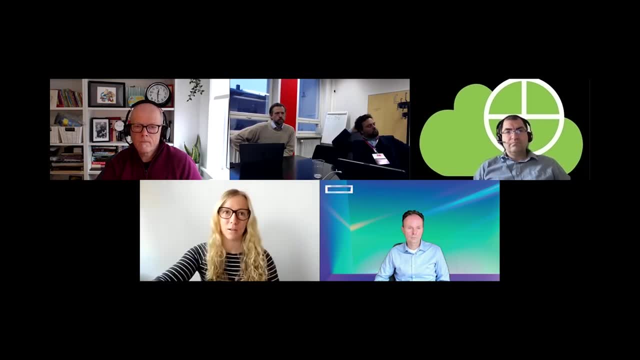 the emerging Technologies, but up until now I haven't seen any one of them going full steam ahead on any single one of them. maybe to what Paul says- the still emerging field- and they're also evaluating and looking into them. yeah, I think. so I was going to make the same point. 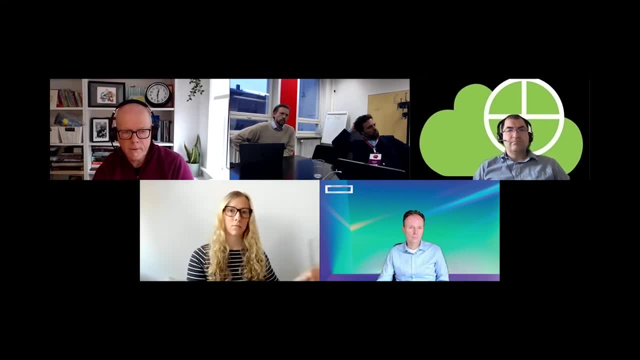 about apples and stuff. but but I can guarantee you that they're looking at all of these. it's absolutely guarantee you. they're looking at all of these Technologies. there's no doubt about that. but you're trying to turn an oil liner. uh, you know, you're not just going to turn that quickly. 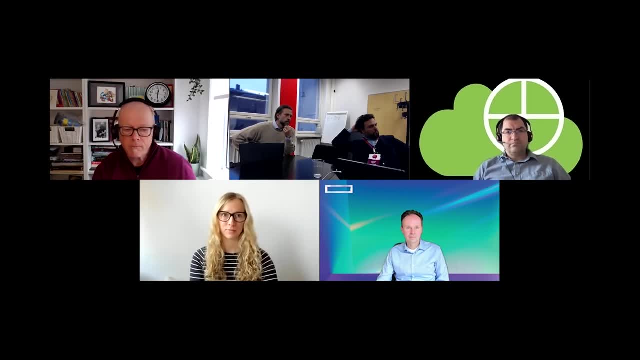 it's going to take time for this to happen. um, we talked about Sovereign Cloud earlier on. to me, this we've we've entered the decade of Sovereign Cloud. this, this is it right? I think it's right in front of us, uh, and I know Google, for example, are doing incredible work on Sovereign Cloud in Germany, for 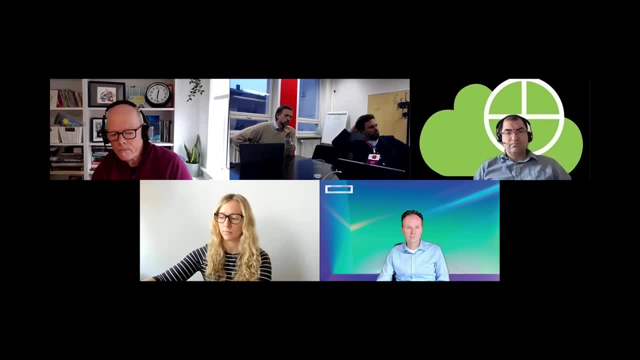 example, for industrial cloud and stuff like that. so these companies, although they have two-sided business models, uh, privacy is becoming a thing. uh, here in Ireland, we're super proud because uh, WhatsApp got fined here a massive amount of money recently as the first fine- on the shrimps too. so, uh, you know some. 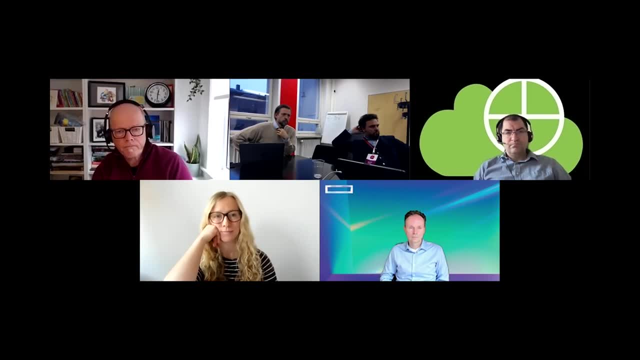 of this stuff is starting to come down quite heavy. um, so more of it, please also uh, and basically extending their existing ecosystems to to provide, to basically provide this privacy layer as a part of their existing technology stack to to their customers is probably something that will uh develop in the same way. like it. it came, for example, machine learning applications, where they 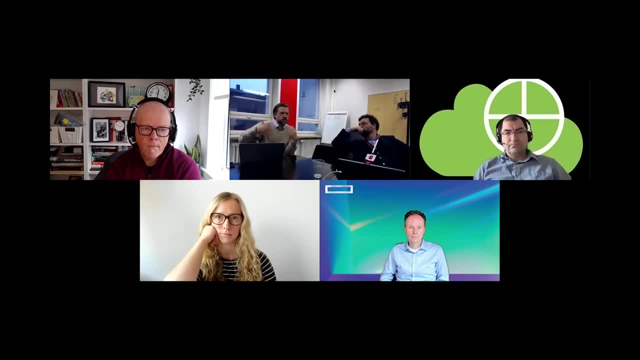 just understood that analytic, the machine learning, is just additional layer on there on top of the infrastructure, so they came up with their own platforms just to support that. I I expect them to come up also with some privacy layer so that they can keep their uh customer within their 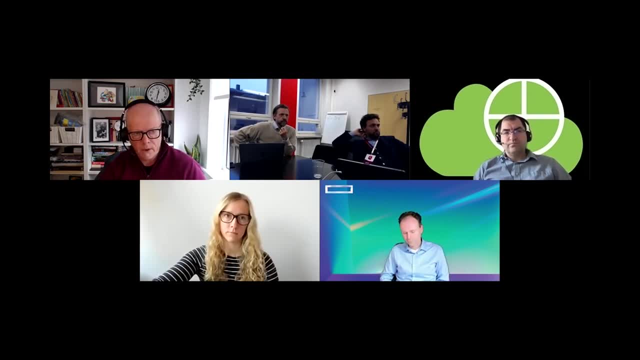 yeah, from the cloud perspective, you know they need to be providing Zero Trust. you know, just because you're taking your data to a cloud, you shouldn't have to trust that cloud at all. you shouldn't have to trust that. you know they can see your data or do anything with your data. you 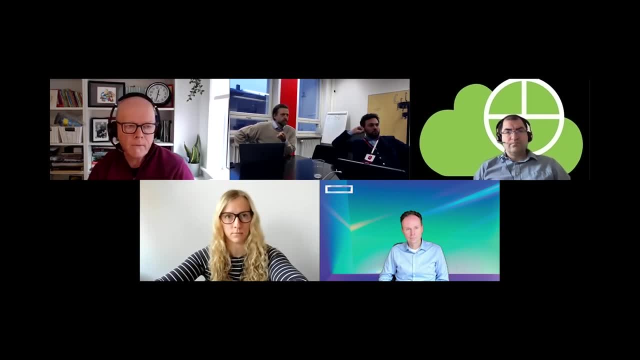 shouldn't even have to trust that the integrity of the computing environment, that that trust comes from them as well. that's the future, and if we're going to build sovereign clouds, it's got to be around those principles, I mean. so so so I kind of agree with the earlier comment of 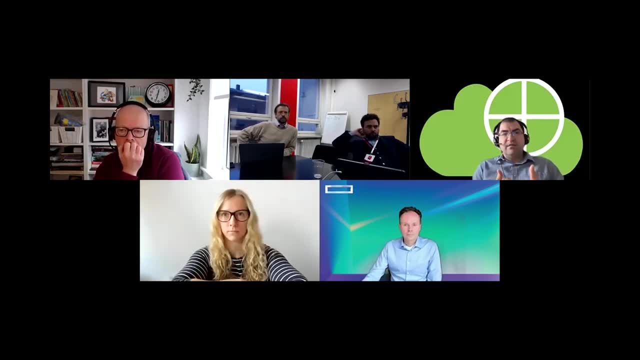 the comment on the use of these technologies. so, first of all, the big tech companies. true, they've they've had the top level experts in, like they've definitely had top level experts in these areas, no doubt about this. do they have use cases for these technologies? yes, they do. so the question is, uh? 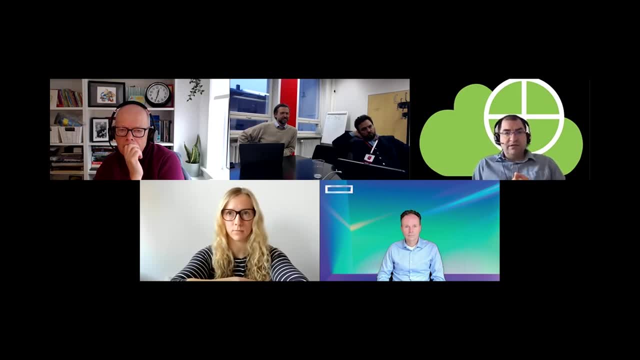 like: what do they do about the ethical application of these technologies? and I think this is going to be a increasingly uh, important so undoubtedly, the technology is there and they look at all these different Technologies for sure, absolutely agree so, especially with responsible AI. many of these big players realize now, also with the proposed AI Act from the European Union, that they won't. 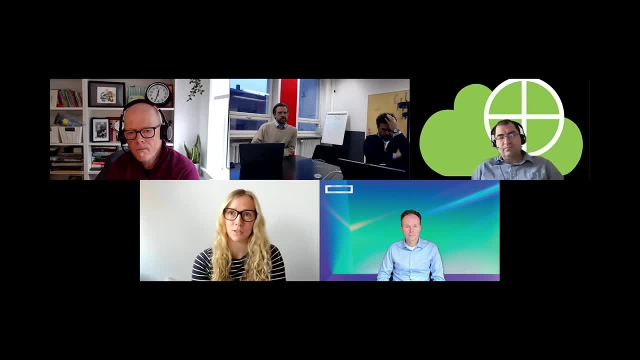 be able to make lots of business if they don't have tools for responsible AI. so from the conversations I had and learned that they're currently really thinking hard on how to actually build products and put it into all the product pipelines because, of course, they have world-leading researchers in. 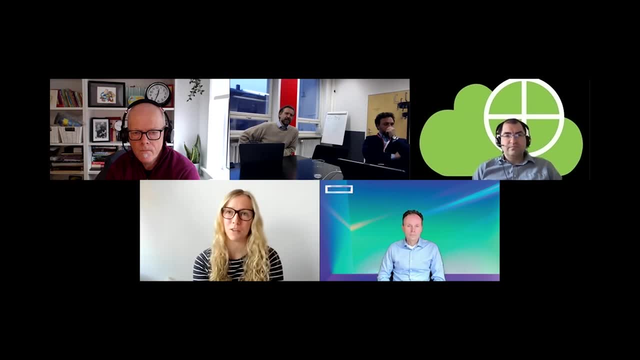 all of these fields, but they don't yet have the full suit of tools needed to actually make it happen. so I think they will see quite a lot in the next two, two years, potentially. on the willingness: no, or the willingness, like the the Google ethics uh example shows so. so sometimes they're not even. 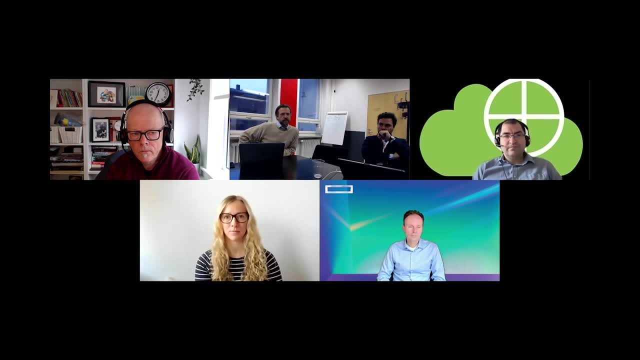 in line with the, the results of their, of their teams, research teams. well, uh, we haven't touched. I would like still to um, to conclude this uh panel or file with a with a question about hybrid uh pets. so we were actually uh, the the good thing was is that all of you touched in. 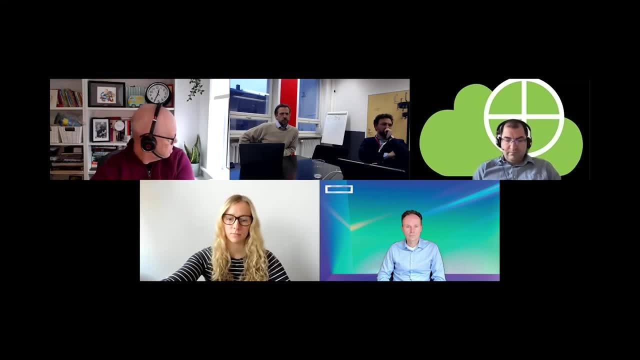 one way or another, this idea of combining different, uh, privacy and attic technologies together. um, there is, I think, uh, there is many, many, if you look at the, the Gardner, or or or Forester, all of them. they also tend to agree that that this is kind of the way to go, so they're. 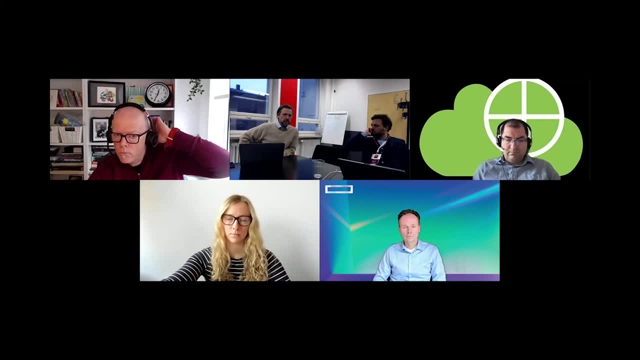 in the market. there is kind of the common understanding that this will come this. so my question to all of you is: what kind of, what combination of privacy enhancing technologies, what hybrid approach do you see the one with the most potential in the short term? I know it's a bit provocative question, but uh, and probably difficult to answer, but still uh. 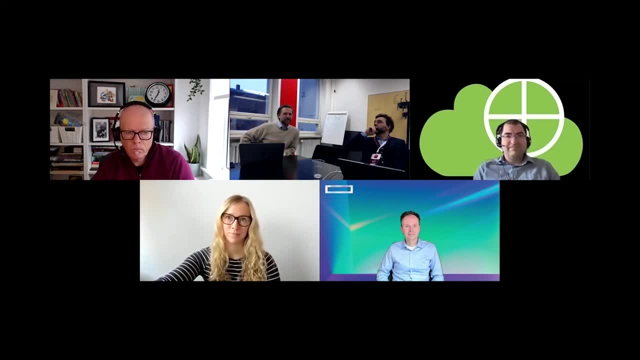 let's. let's hear your thoughts on that. who wants to start this time? well, I, I can start. um, I, I would always go to the use case again because it's too broad, otherwise uh. so, for example, if I do not have the necessity, uh on, or I have a large data set, uh, which I can. 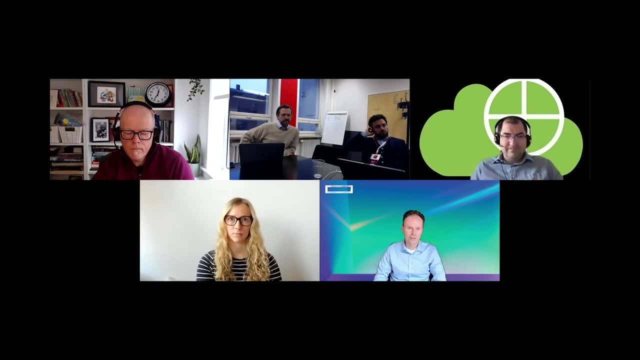 potentially uh. completely anonymize in the beginning. example histology data of uh, of um. if a tissue, no question uh. I would not by homomorphic encryption, because it's an additional layer of performance, complexity, 100x, whatever um. this is an impact I don't need uh. if I, though, have 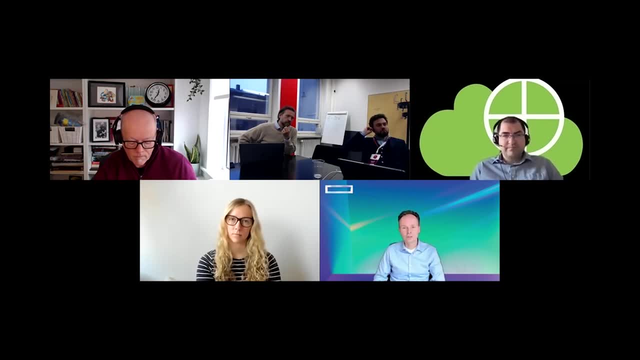 a combination of banking data with uh anonymized data, then of course I would combine that uh and do a secure multi-party, but leaving data at the edges, uh. so. so it really depends on the use case, uh on on how I would actually combine those and- and it's it's I- I would potentially always uh take. 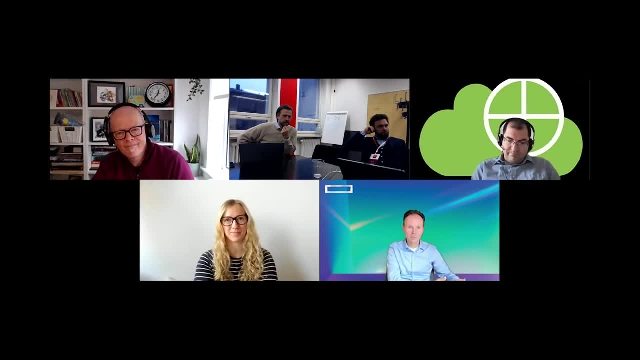 the TEE. so, Paul, I would always take yours, because that's what we need is to be, and maybe even go into the supply chain on the silicon by itself, so that we can ask to state that the the computation which has been done in the silicon is right. nevertheless, I would go always up and say I need the identity. 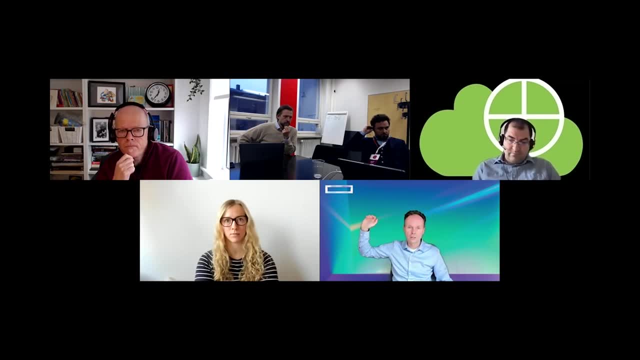 uh, that's the question which came before the SSIs, which are then be given out by either a self-sovereign identity or a government which is trusted only for giving the identity. so we have the complete chain from in silicon until the the the end. so the architecture is fine, but then to define really. 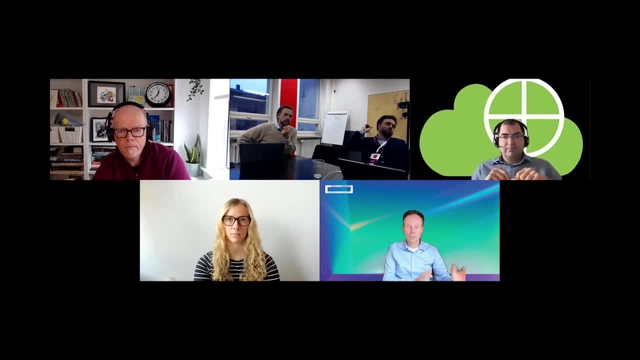 depending on the use case which I need- and I come back to the synthetic data- I would potentially start with synthetic data for usage to get the right seed model, the ground truth, somehow, and then to extend and also deploy additional things. but always it has to be in a common sense at the beginning. 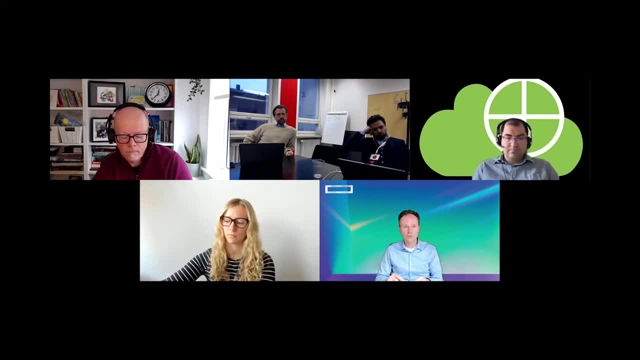 already to have the right architecture that all these different aspects can be used and should be used. that's my target. so to define the target and then, step by step, do the approach and what to employ in with which phase and in which, which size and and spread and scope. 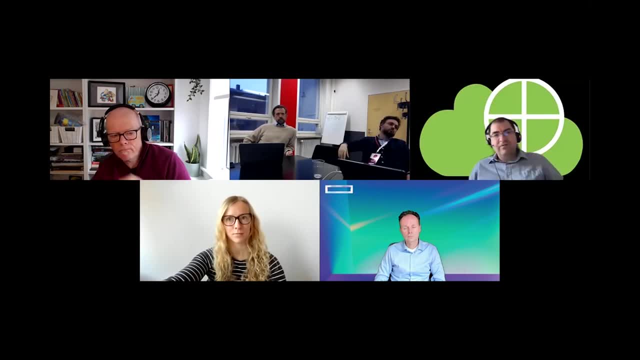 so, uh, maybe to add to that the the question of what hybrid combination is the most suitable for a use case. I should say it depends on the use case. so that's, that's the first step. so if you're doing it's one thing. if you're doing model prediction, it's another thing. if 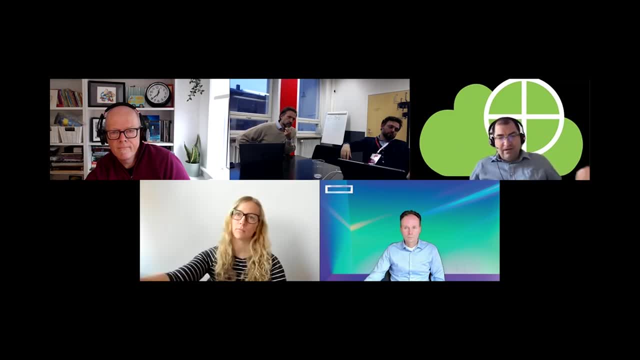 it's a training K model, so these two use cases would require a completely different combination of privacy enhancing Technologies. actually, something that I saw recently which caught my eye was an online simple questionnaire where people are trying to classify according to your problem or use case: so what kind of technology or combination of Technologies could give you could. 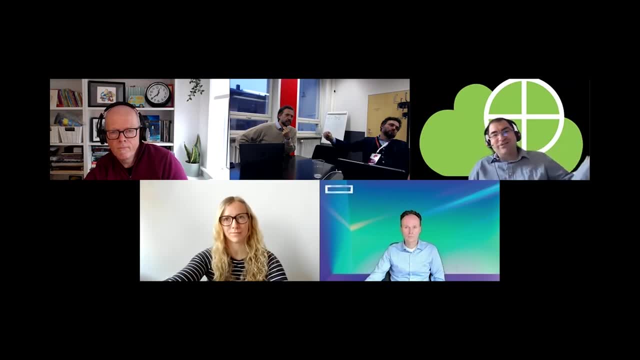 solve your risk case just based on questionnaire, simple like the covet questionnaires that we are doing online to classify whether, like, the patient has covered or not. but uh, so all of these tools, they are going to be important now to make us like to make this happen from a technology point of view. we obviously need 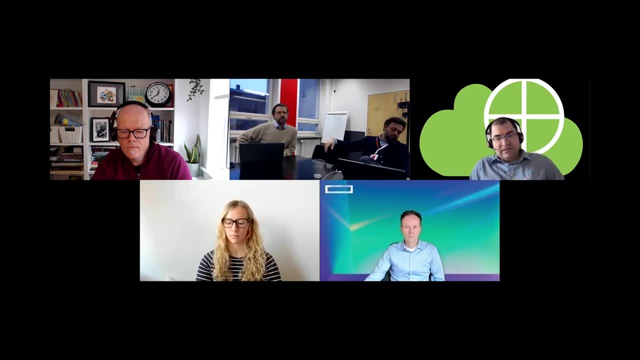 like very solid and intuitive development tools. uh, i mentioned this a few times in my talk as well. so, uh, deployment, orchestration are important, but making sure that, for example, you could chain part of the computation that uses fhe with part of the computation that uses npc or trusted execution environment within the same programming environment. that's that's going. 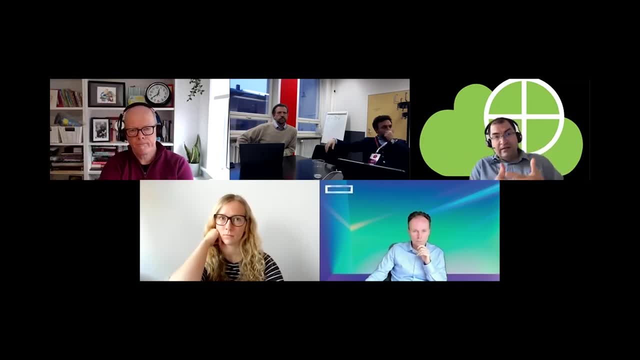 to be very crucial, and that's a non-trivial task. also, making sure that you could validate your program from a security point of view, making sure that you don't exceed your privacy budget to prevent you from using the same programming environment, and that's a non-trivial task. 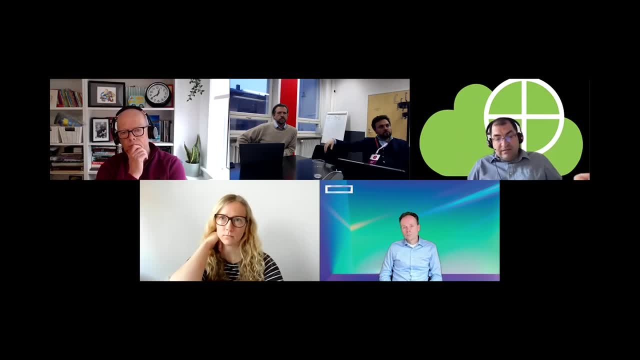 compute on the data and uh like, last but not least, very important during your model development, the use of this uh, of the synthetic data that we? uh, we mentioned. so we still have a long way to go, even if the technologies are already there to build this entire ecosystem to to allow that data data workflow. 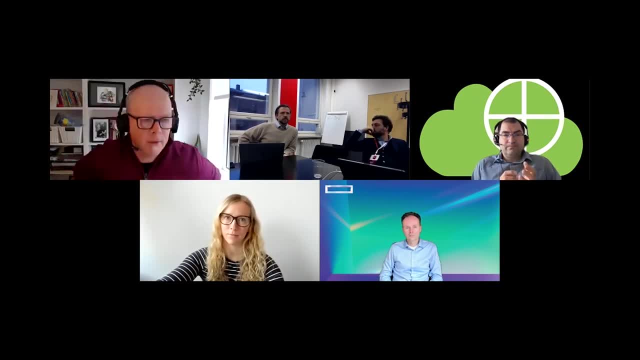 uh, so, um, sorry, i'll just- i'll just add that quickly, uh, to that. uh, amir, i think, um you know, we want to build an environment where all these pets can live happily, right, um, you know, so we can take things like homomorphic encryption uh, build it into trusted execution environments to provide. 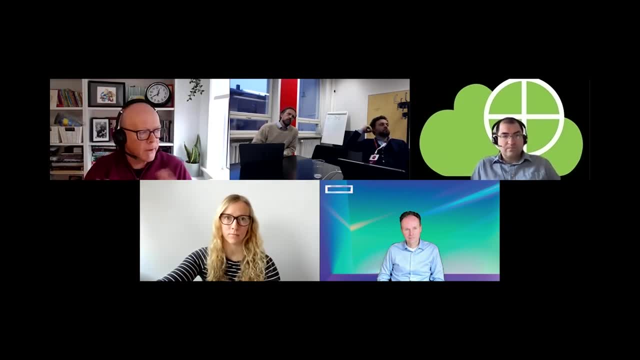 integrity of computational data and all that sort of stuff. or we can take- we're already running uh- pseudonymization engines inside of the system and we can take- uh, we're already running uh uh, uh uh inside of trusted execution environments in the cloud for that extra ring fence of uh insurance. 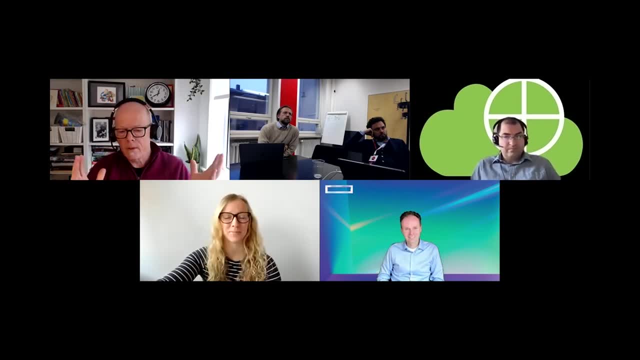 uh, we should do that with mostly ai as well. obviously, alexandra, at some point. but ultimately, you know there's the vision should be that you know, uh, there's a devops person who has some data sets and that devops person has a marking on that data set that says this is super sensitive. 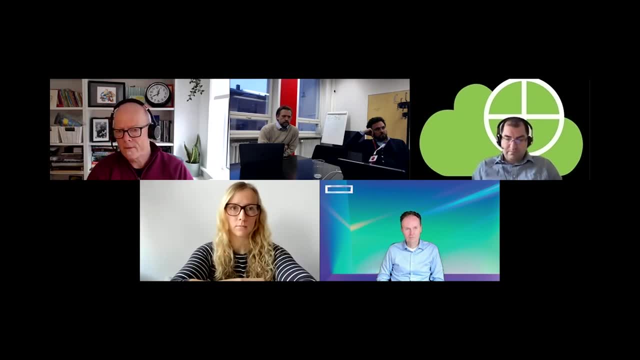 and they should press a button and, at the end of the day, they shouldn't have to worry about which cloud it goes to or which technology takes care of the data that they're using. so that's the vision. um, i think for sort of confidential computing embracing all types. 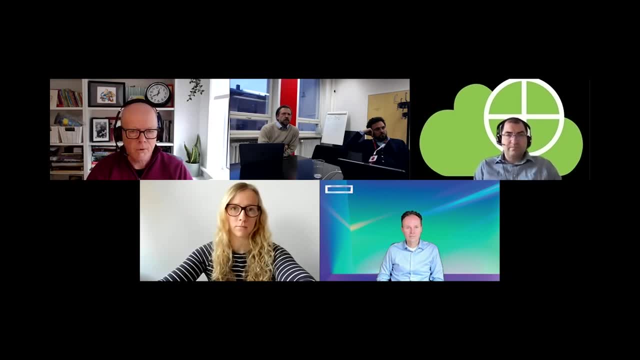 of different um technologies. we're way away from that yet, but that's the journey that we need to go on over the next five to six years to enable that. so that that was actually my follow-up question. right now, we have a feeling that this is a no, that's not the thing that, uh, right now we have. 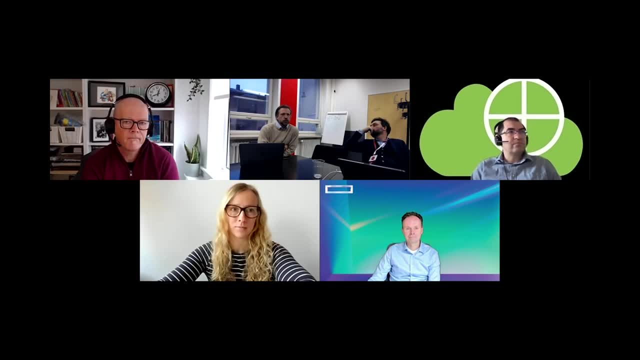 the feeling that this is still custom built solution. every, every use case is a custom built solution. so that's the vision i think for sort of confidential computing embracing all types of different technologies is a bit, especially when we tap into a hybrid solution. it's a kind of custom built. 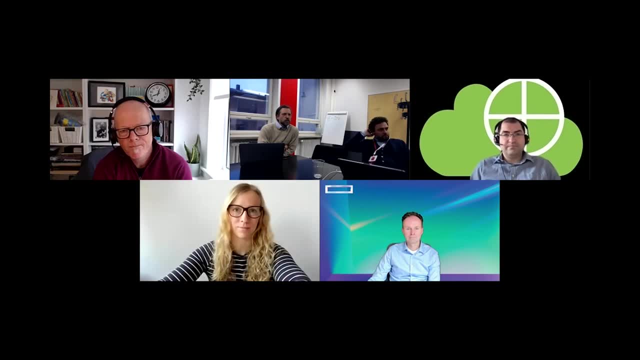 solution. so when do you expect to have products that you know, the out-of-the-shelf product, that do exactly what you mentioned, paul? just basically understand the complexity, the, the privacy complexity and then combine the different approaches together. i think the answer could be in dimitar's magic box at this stage. i don't think we know at this point, but there's two crucial parts. 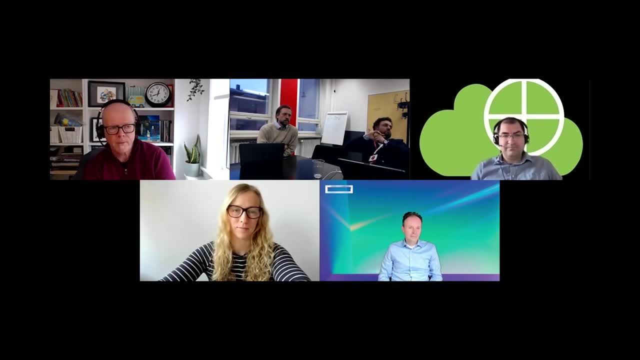 of this. it's not going to get done by companies like intel. we'll build the infrastructure to enable it happen. the plumbing, if you will right. it's the ecosystem that's going to drive that. the second part of that. i'm a firm believer that open source will lead the way here right, and that, uh, you know working with open source. 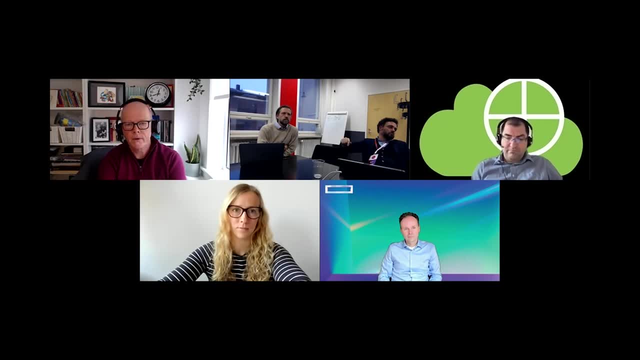 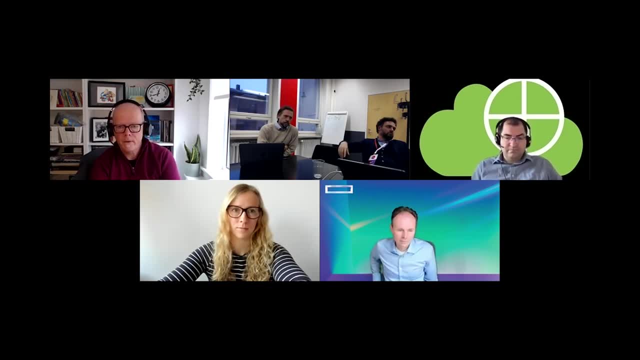 it's going to be something that has to be open source driven. if not, standards will fall by the wayside. unless we get into open source, it has to be standards and certain ways of doing things, attestation protocols, etc, etc. if we don't go there, it'll just end up with loads of different privacy. 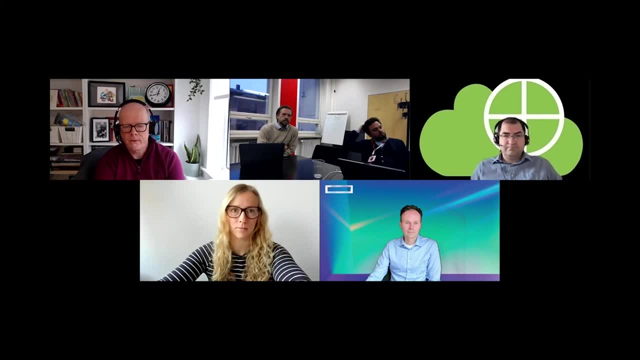 enhancing technology companies competing with privacy enhancing technology companies and for data owners, that's a nightmare. yeah, maybe that's that's the, the notion. standards: that's that's where we need to get over. if we have standards- and, uh, the standards deployed on data quality and privacy, on on requirements. 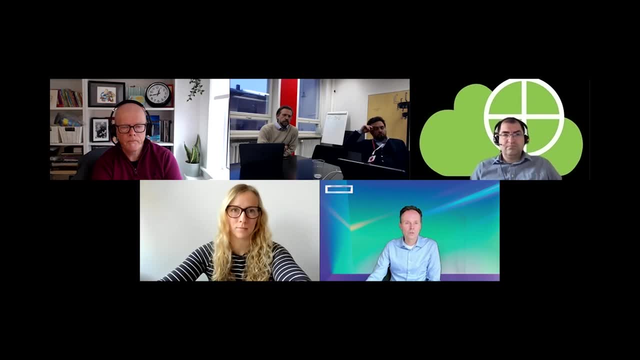 which have to be employed or are easily employed, then so. so each base and founding product, which is then one of the modules to be deployed in a vertical solution, is then having already this within and- and that's something we have also to work on- based on open source, and then coming to 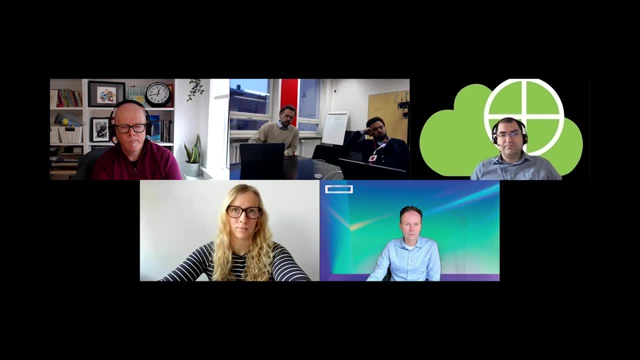 standards. so like, like service descriptions, uh, in, in, in gaia x or something like that. that also the the notion of what is private data? um, what is the classification? how do we? we treat it if, if classification type two needs to have a te of further standards, and that is something which has to be built out, so standardization is uh. 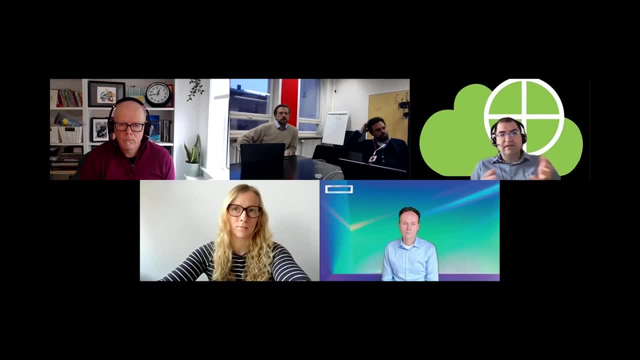 definitely very important. i agree here with hackmuth and back to what paul said earlier today. so what we see nowadays is a lot of standardization efforts, but they are segregated by technologies. so there is a homomorphic encryption standardization effort. there is uh standardization effort for, say like, multi-party computation or trusted execution environment. 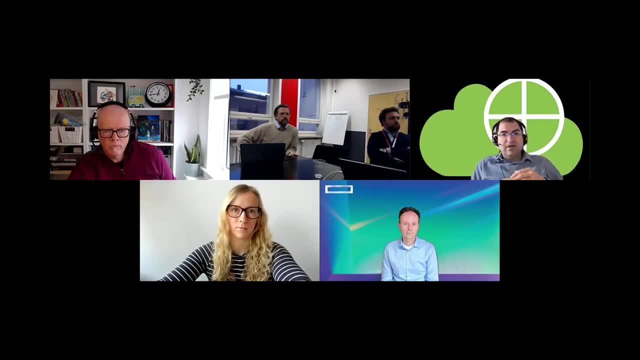 somehow, what's missing is the intertwining of all these technologies. so, uh, we, we also need to work towards that, and this know, uh, in the confidential computing sense. you know, when i showed the slide where all the logos, we're starting to work on standards without a station, so that other hardware providers can. 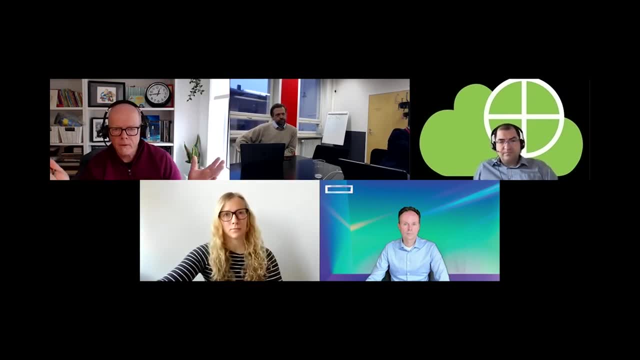 attest to our hardware, for example, to open that, and what that starts to do is open up a cloud to edge, where some t's may be better at the edge than we are, for example. then you're getting into integrity, you're getting into provable data, you're getting into provenance of data, etc. etc. right, and 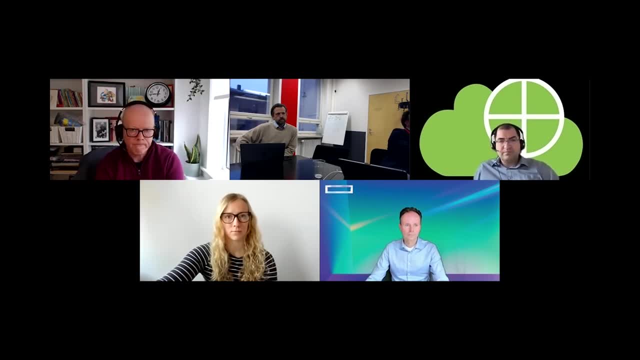 that's why standards are so important and it is doable um to do this type of thing, um, so fingers crossed, so so mobile forum. actually, i hope we contributed not only with this event but also with this panel, to point in in the direction that that also banking industry will, will, basically, will be. 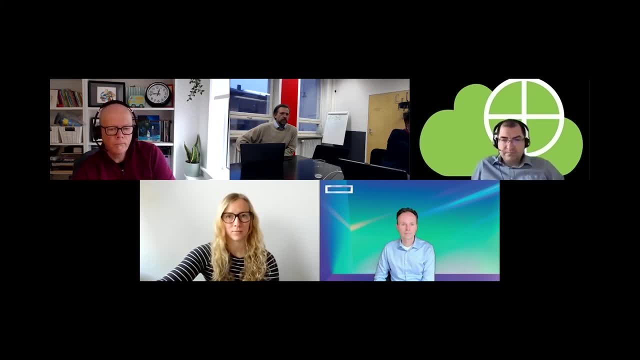 very will welcome this kind of standardization where where we can um come up with the use cases and then, uh, then, enjoy all these kind of technologies, um, and and are being able to consume this, and i i'm really happy that we we were able to spend this time together in this great panel. thank you very. 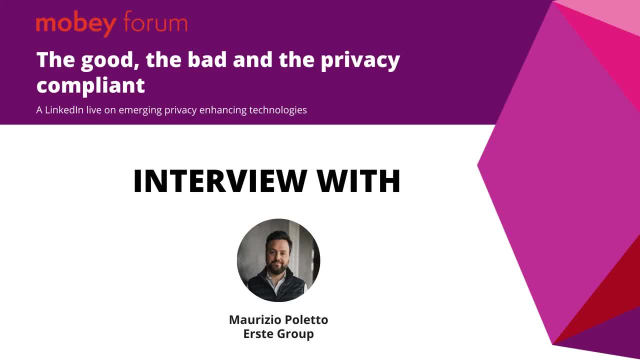 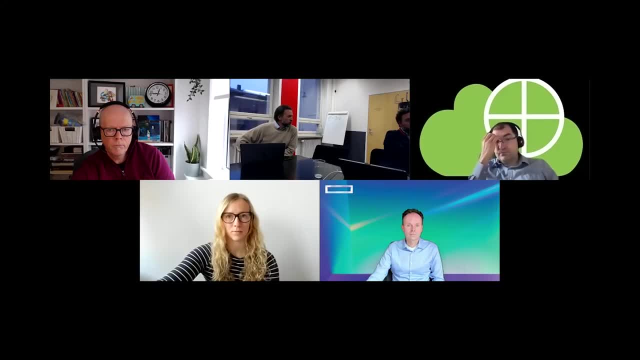 much for that. and uh, who is also can? can we talk a bit now from a decade perspective? what is your, your take on on this? uh, on the issue of privacy, how you see. well, first i have to say i really enjoy the panel. i understand half of the half of the things you guys talking about. 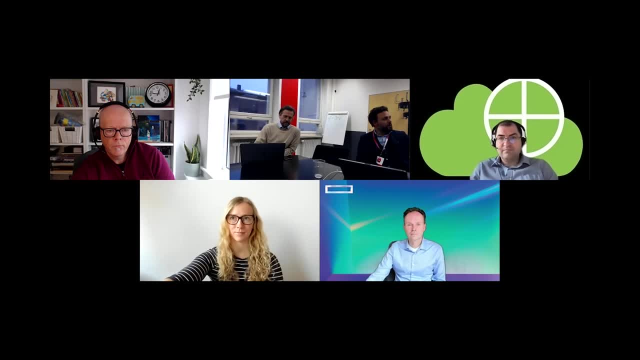 but on the other side, i also have full trust of what you're doing and it's going in the right direction. so when i asked the question below before about what the big tech player doing, it was not cynical. it was just trying to understand: uh okay, if they don't drive this, or if some of the big tech don't drive this, who else should drive this? 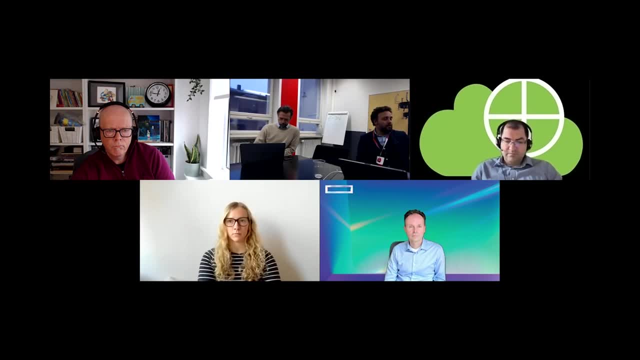 because it makes all the sense right and i think, uh, in general, regulated entities like we are as bank are probably the most, uh, the it's an industry that needs to go into that. i mean, if you're not doing it, who else? i mean, if you're not applying privacy and and um properly, we are uncompliant. so 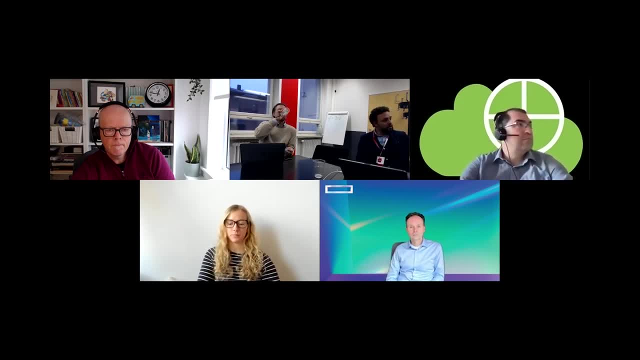 we're going to have trouble. so there is. we don't have any alternative. let's put it that way. and as actually i believe that the future is about also, for banking is about really trying to make the best out of the information we have. i think we need to find a way to do this in the most compliant way. can you share anything from? 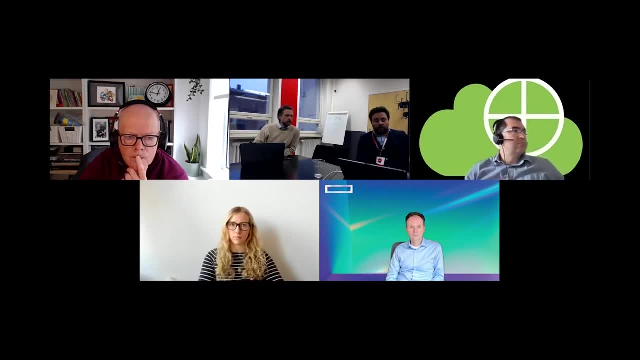 your side. what are the challenges that you're facing? look looking at. i speak for my banking group, where i'm working on, and uh, which we are located in different countries. uh, we have operation in different country and we have different maturity in different country, though the challenge for us is basically to make use of the gigantic amount of data we have in our systems. 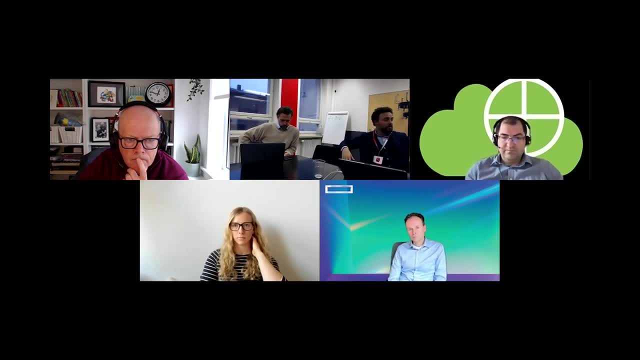 it is true that bank has tons of data. what is really true is that we have tons of unstructured data, and the way to make use of these informations is to structure them first. and unfortunately, in many cases, we store information but we don't structure information. so 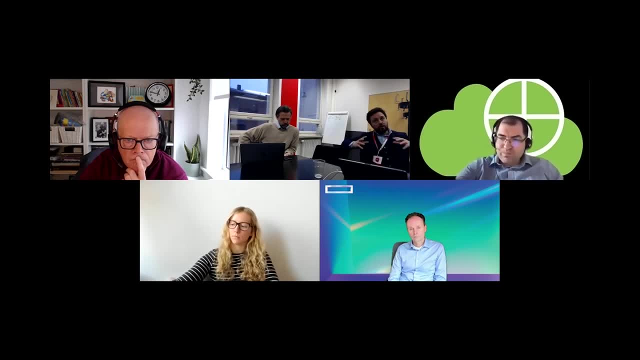 with lots of data saved, like just by looking at погsh. but we are sustaining the data wireless network where um things like a data pool program, orasaki or something like that power takes the information from the everybody else manually. so we our development of theomme system up and then, when we get our data, we are using this. we. are that and we also have tools. we have support tools that we had- some sort of Feuer trails and computer wings for audience education and geoscience issues, for example, and it continues to grow from the now now for a lot of the Taylor layer, but also data is changing the way we work anytime in the future. 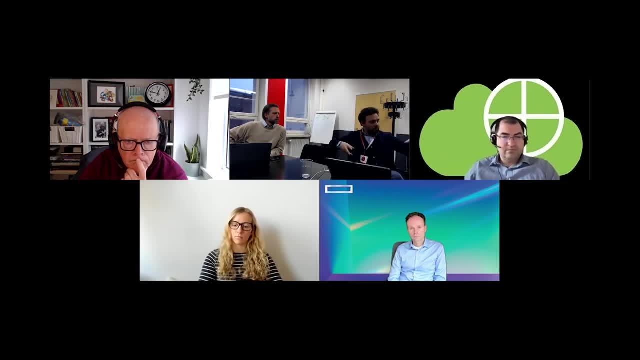 but they don't talk to each other, they don't share experience, they don't share models, they don't discuss, they don't leverage each other's work. This is the reality in many large banking organizations today, And if we solve that, if we break those silos, 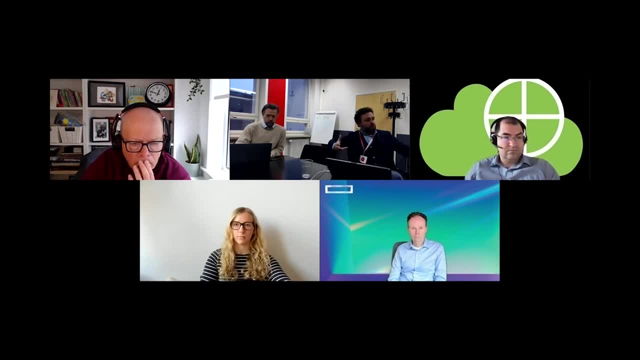 probably there is a much higher chance that value comes out of those experiences. This is not true that there are no great data engineers in banks. There are. We had some very good projects. We're having a very good risk model, for instance in Sears right. The point is: 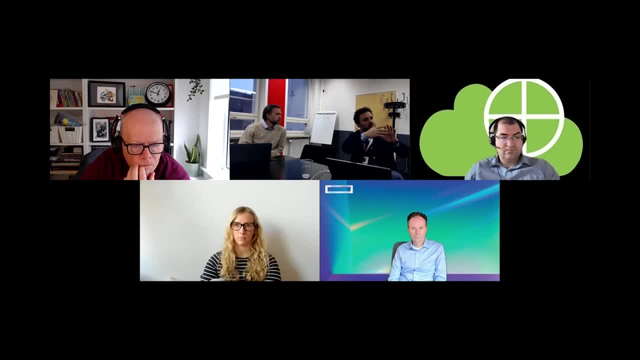 they're very restricted, within a very specific vertical They are normally. if you look at how those projects are financed, they're normally driven by a sponsor which is only interested in one output and is not interested in any other output. If I'm sponsoring a project, I have 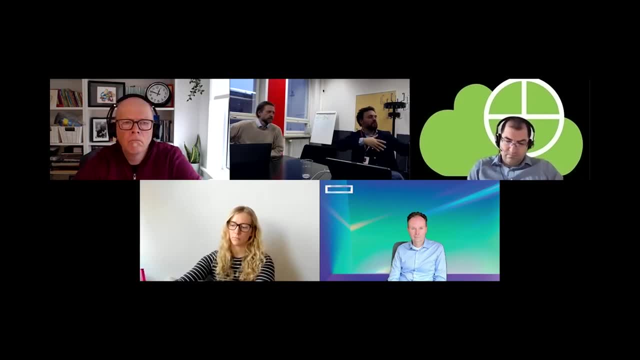 tight money. I want to get the result I want and I'm not interested in. my team is looking left and right or sharing with someone else. We need to break this thinking and try to go towards the direction where you say there is a bit what we call in some of our exercises. 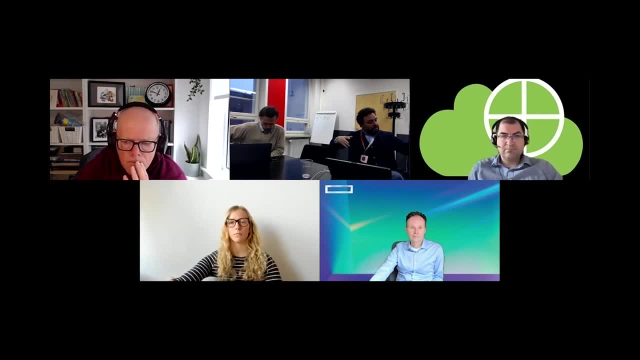 within an organization, data as a platform. So someone who takes care about the core data we need to structure, keeping it alive, maintaining it, making sure that everyone can use it in a various manner. So that's one of the things that we need to do. The other thing that we need to 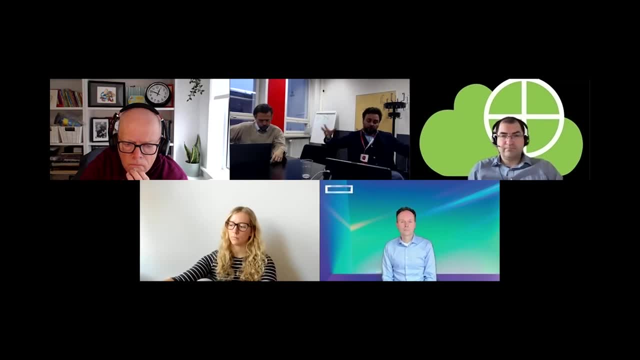 do is we need to make sure that it's shared across different divisions And, yeah, that's the direction we're currently working on. It's not easy, but we think it's the only way to go. But this is only one part of the story, So what I mean is this is solving the technological access to the. 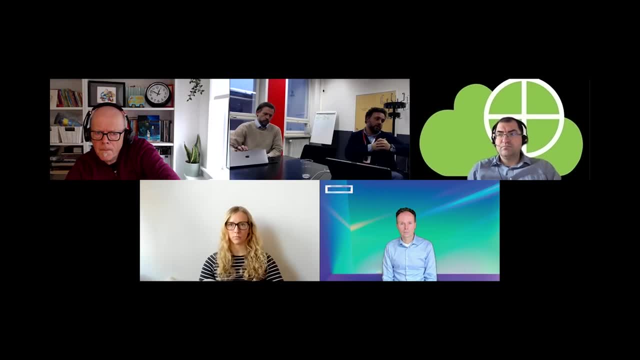 data information, but it doesn't solve the complete picture. The other big problem in large banking organization is that there is completely different attitudes towards data access and data utilization. You're going to have the data platform or the data officer who will tell you. 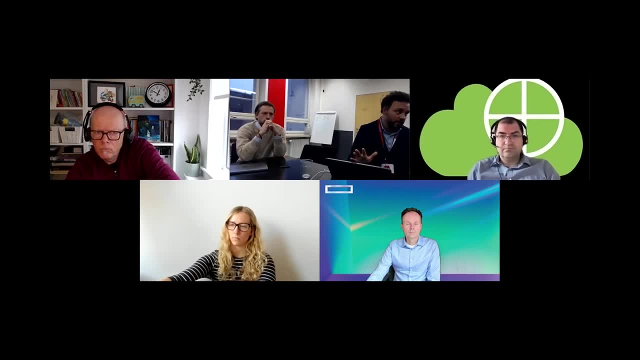 don't touch it, You will have the guy from business who say, well, touch as much as you can, You need to give me something out of it, right? And then you're going to have the legal guy say, well, if you touch it, it costs us millions of euros, right? And then you have the CEO say, well, 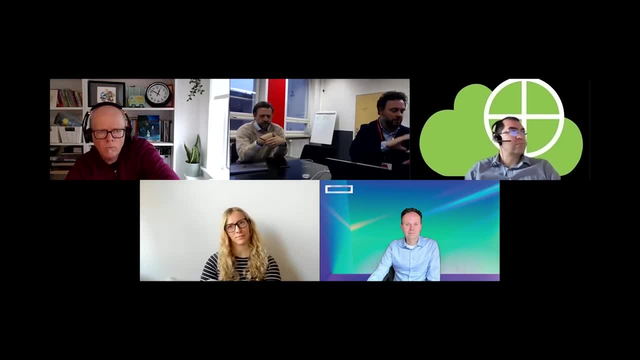 give me this table. I tried to calculate the risk- reputational risk, operational risk and so on- And then I decide if you can touch it or not. And I think- and each of these people are basically looking at the same regulation and interpret those regulations in a slightly 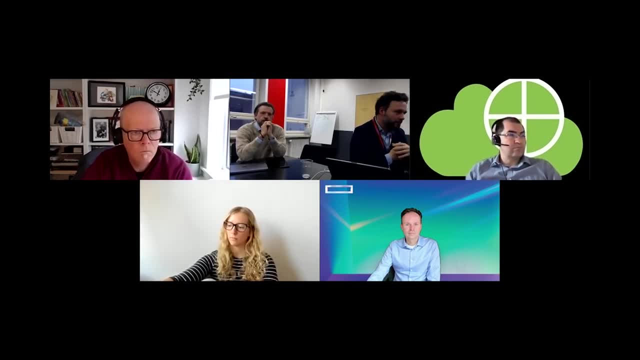 different way Because they've, you know, regulation not really written beautifully in this sense, or they leave lots of space for gray zone And so each of them has slightly different interpretation. So the other big elephant in the room that needs to be solved. 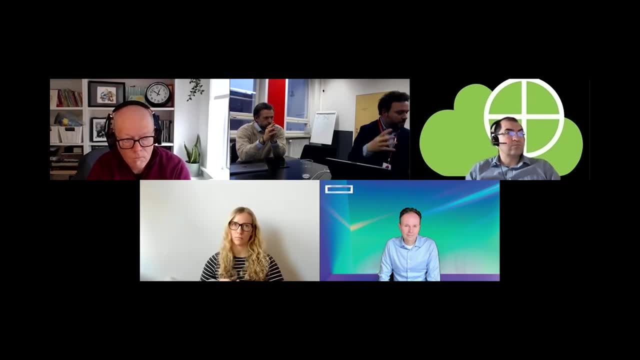 beside the technological access or the technology, the technology spec. how are you going to make data engineer really working on data rather than working on access to data is to solve the understanding of, so the purpose, So every company, in my opinion, should have a clear, documented purpose. 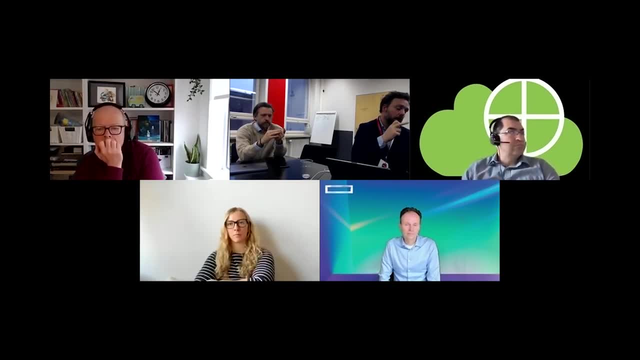 which data they are collecting, why they are collecting it, for which use cases they can use it, because it's their legitimate purpose For each use case they can only use it under a specific explicit permission of a customer, And for which use cases they will never touch it, no matter what Right, And so this should. 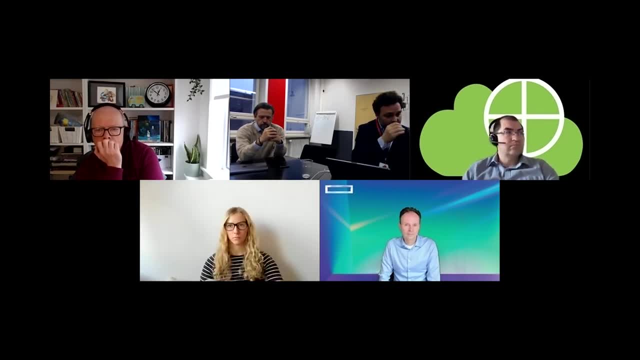 be structured, documented. In my opinion, it should be very precisely written into. we call it a data charter, you can call it a policy, whatever doesn't matter how you're calling it. You need to get these undersigned by the management and the management of risk. 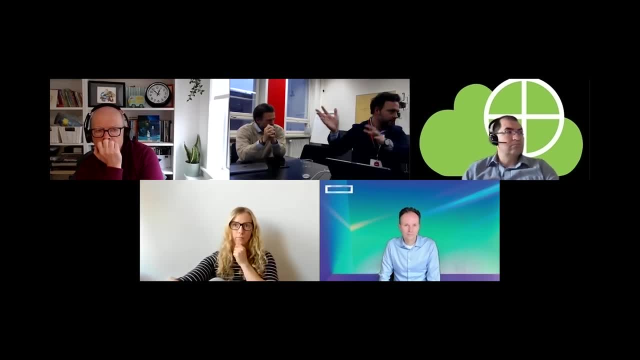 the management of business, the management of legal and compliance, etc. etc. and once this is agreed, then you can share this around your organization and tell and tell your uh, your teams who are dealing with data, say, guys, this is, this is the bible, that's what it is, that's. 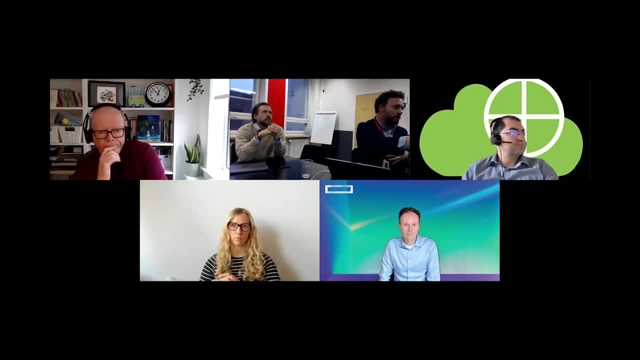 where we can. this defines where you can go, where you cannot go, where you need to ask permission, where you don't need to ask permission, what we allow to do it and why we allow to do it. that's, that's the second pillar. without this, even the technological solution will not help us. 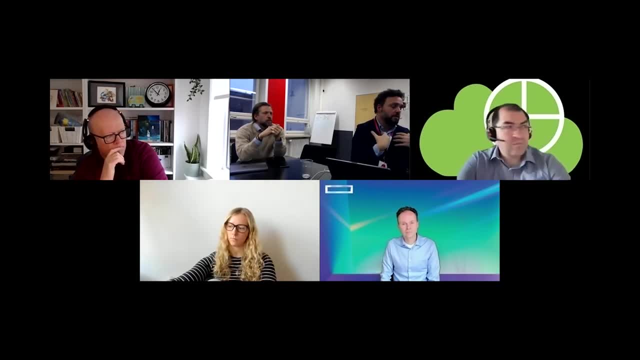 you will still have fights within the organization. because i'm business, i say, well, i can do this, it's pretty normal, it's my legitimate purpose as a bank. then you go to legal and say, well, that's, that's your opinion, our opinion is different, so this needs to be solved. we were discussing before and 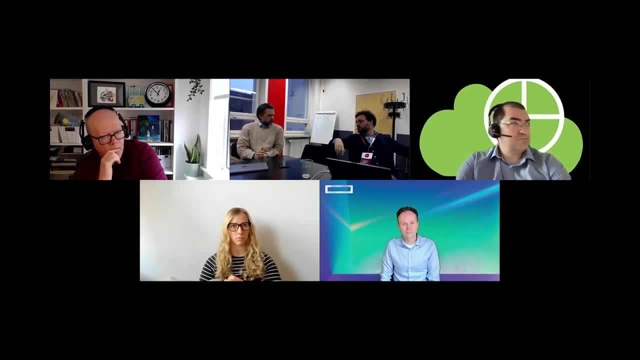 maybe it's just the wording. you know we were discussing this iterative approach to that. oh yeah, do you think that the bible is the, the best uh uh expression, how to name it? because it? i think it's also iterative. no well, it should be a living document, exactly i meant. bible, from the point of view, is normally, if you're religious, if you have. 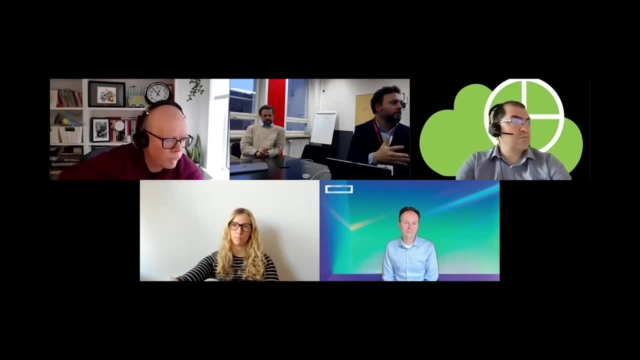 a problem. you open the bible, you find a solution in there, right. so same story here. i'm a, i'm a team. i want to solve an issue with data. i open the bible. i should find the guidance how to fix it, right. um, but what we discussed before, you're completely right. i think that, uh, what we are. 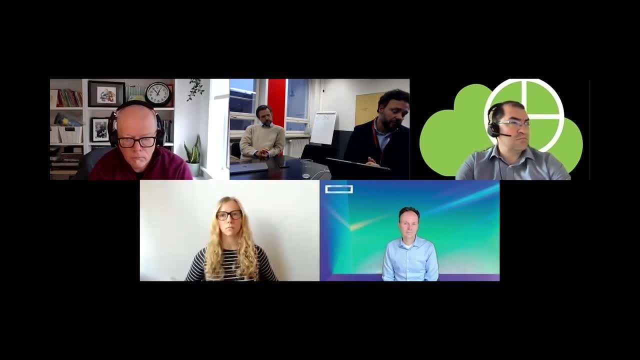 missing in in large bank organization are, for instance, lawyers that are it expert too, so technical lawyers, so it. we have a lot of very good, uh, banking lawyers. we have very we have many lawyers coming from the regulatory side of you. but what we are missing in many of the organization a lawyer with a deep 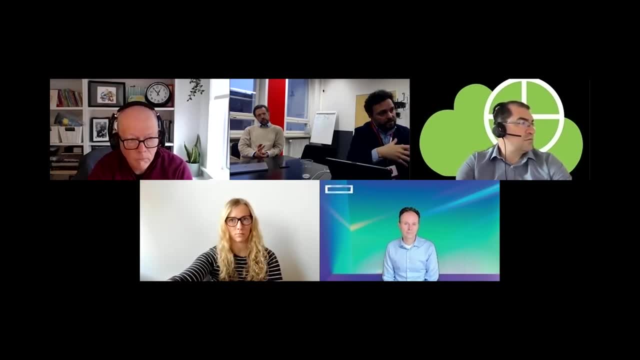 understanding of technology. that's what we miss in banking on one side- and i mean we are we- we try to get better there by training our existing lawyer, but also hiring specialized lawyer on that topic. and the second problem is um- and this is what i am not just mentioning here, i also 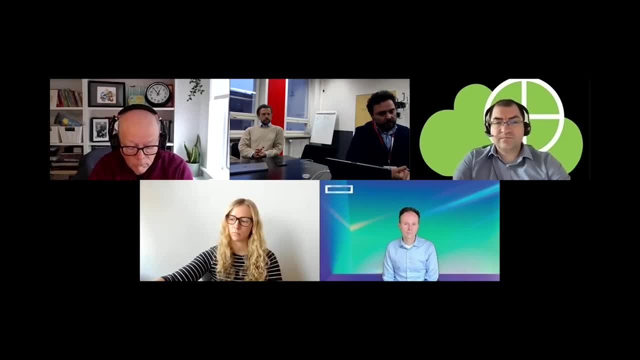 mentioned in my exchange with the regulator. i think, uh, regulators should learn making better regulations. most of the regulations that are in place today they tend to be uh they. then, because of the current situation of the business, they're very tech, technically driven and therefore, in my opinion, 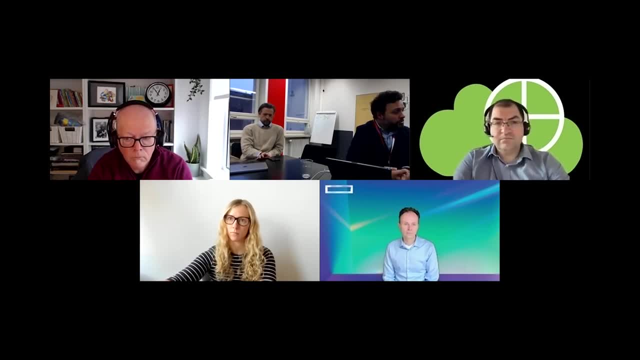 regulation are mini technical projects at the end there is a lot of technical reference into that and um. and if you look at how regulations are done in europe, for instance, in other countries, the europe, the regulations have done like it projects have been in banking have been done 15 years ago. 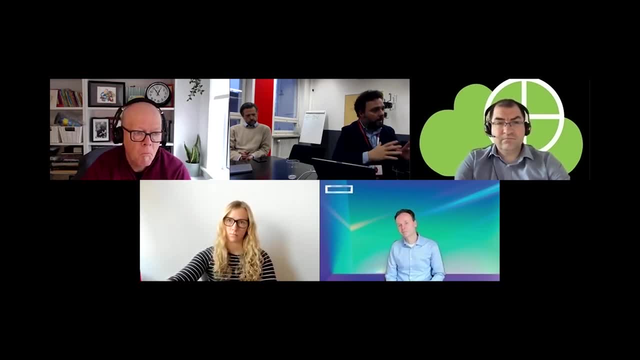 so you spend three years trying to get golden plate. everything tried to cover all the use cases. try to think about any possible, any possible edge case. so three years of really hard work and then, after three years, you issue the paper and you think the job is done. but the job is never done. 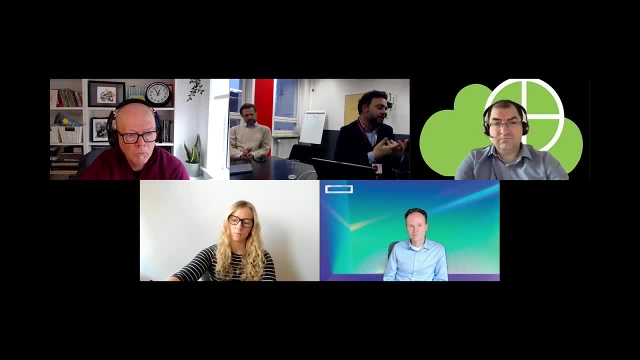 and so, i think, also building regulations. it's something that we need to be really careful about. Building regulations should be an iterative project. You start small, you pull out the first version. you see how people react, you listen to them, you get feedback, you tune, you issue an extra version. 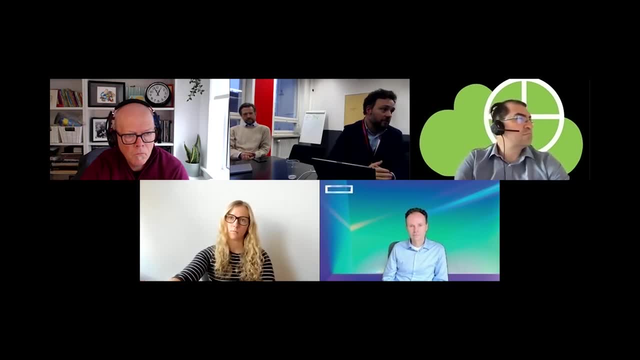 but we are not there at all. If you look at PSC2, it took us five years to issue PSC2 and we are still at version one UK. they have version five or something right, And they did it more iteratively. 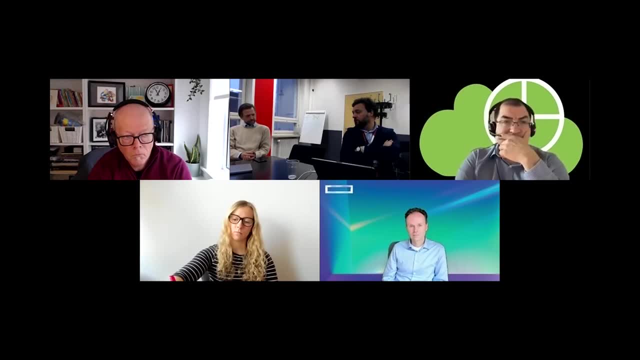 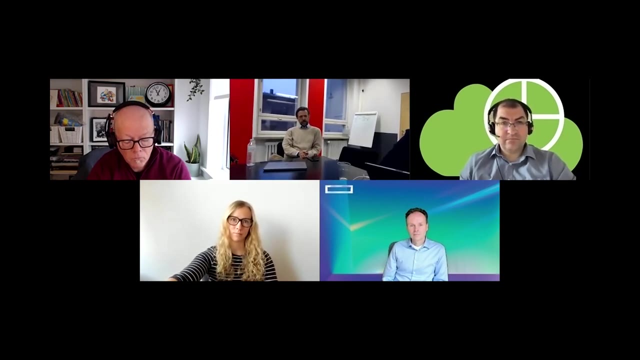 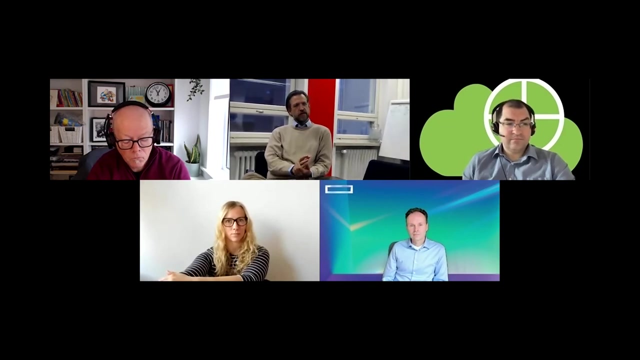 So I think there is lots of improvement to be done, also on the regulatory side. Yeah, that's my view. Thank you very much. Thank you, Mauri. We are close to conclude, after three hours of very insightful presentations, panel and, at the end, even the opinion of the customer. 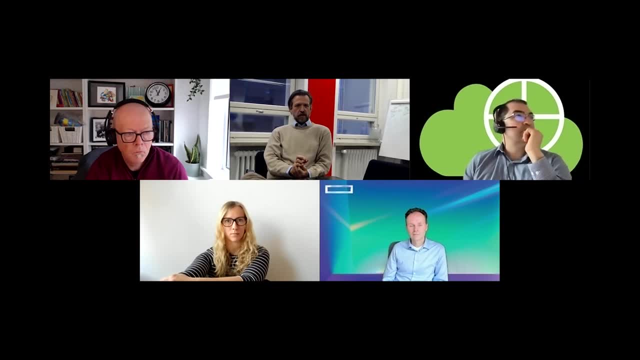 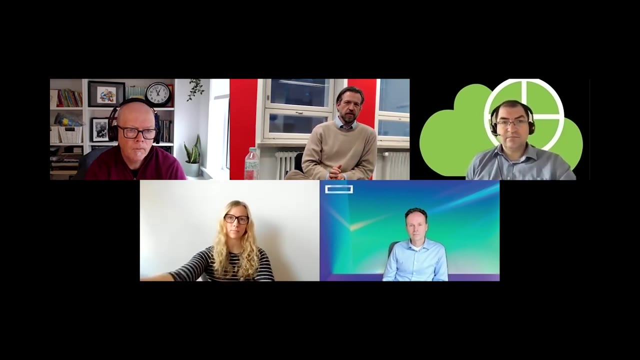 We are coming to the end of this event. I would like to finish with two things. The first, The thanks to experts who joined us virtually here in Helsinki during our expert group event and, really enriched with your insights, our understanding of privacy-enhancing technology. 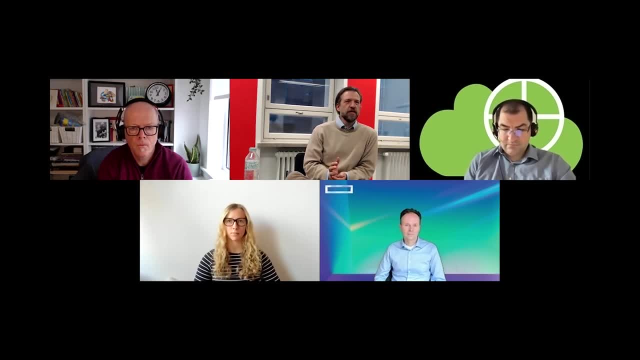 I hope that this kind of collaboration will continue in the future. And second, I would like also to just provide a few news. I think it's very important, Thank you. We have some questions regarding the results and output of our group. So we already mentioned that we published the first report. 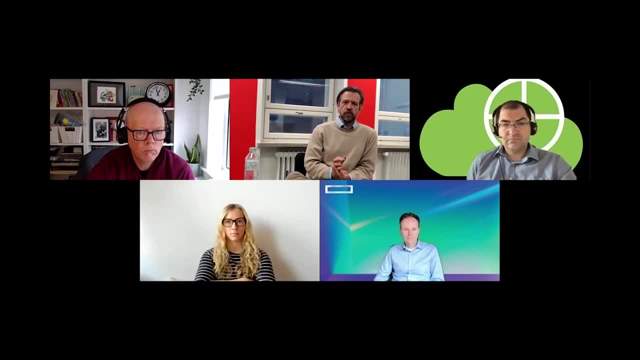 in June of this year. Next year, in the end of January, we are starting with a series of small reports on each of those technologies today mentioned. So we will publish them quite frequently, And it would be also great to involve you, as experts, in the finalization of these reports. 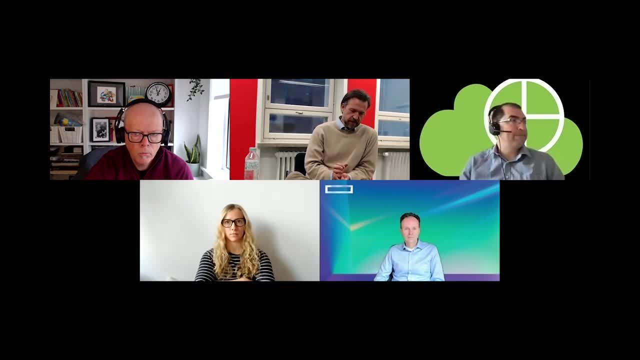 And for the Q2 of next year we are planning to publish the report on hybrid approaches. So exactly the topic of today, I think, in our view, is a very worth of dedicating entire report only to this aspect: How to combine different privacy enhancing technology into something that is of value to banks.